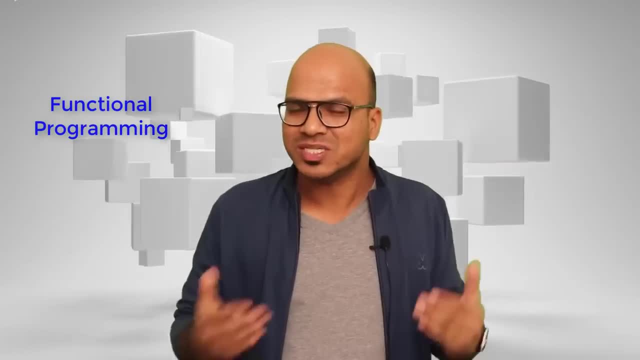 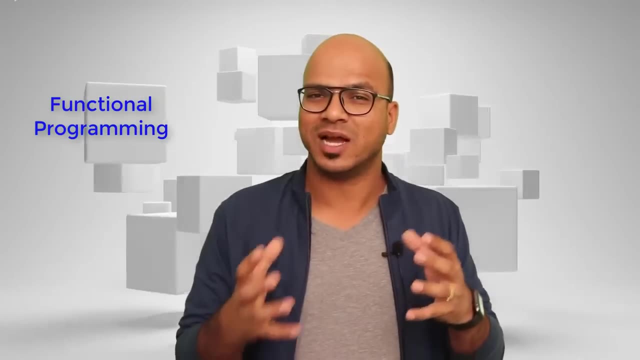 can achieve a certain task. implementing functions as a mathematical functions, where you will not complete a data, which is instead of changing data, you will still accomplish a task, One of the ways you can pass a function to a function. you know, we have seen this again. we have a very 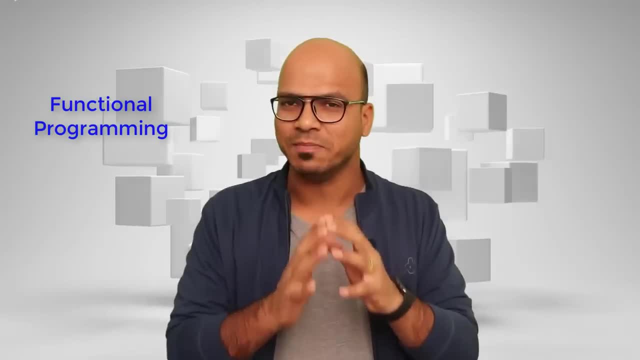 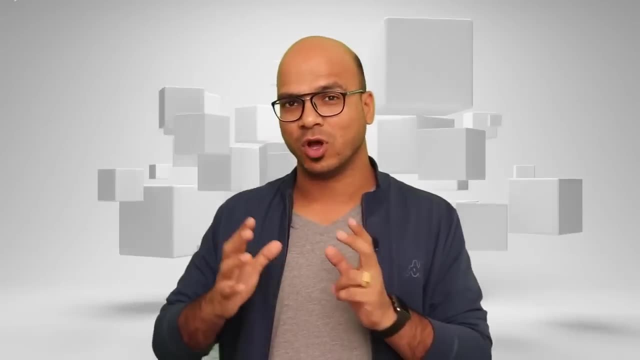 deep concept of functional programming- we'll talk about that later- but time being procedures and functions, which is something we have already done with, example, Lambdas. Now we are going for a concept of oops Now which is very famous in the industry. you know so if you are working on big 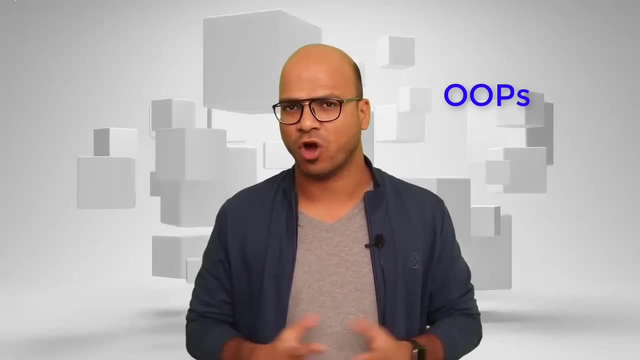 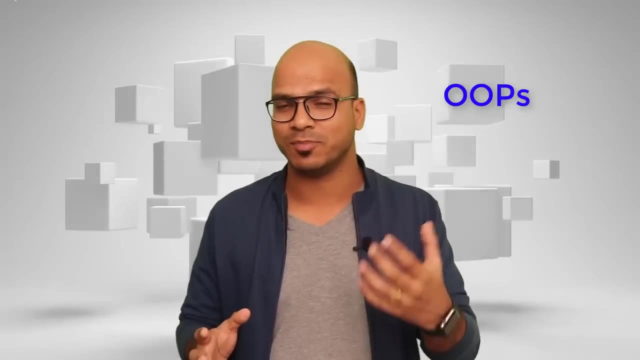 software enterprise projects. you need to think everything in a format of objects. Now you are thinking, why objects? We were happy with functions right Now. see, even from start itself I was: I'm talking about objects, right? Maybe in some programming I said, okay, this is. 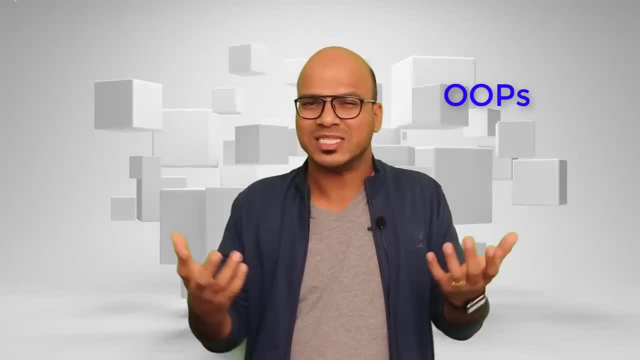 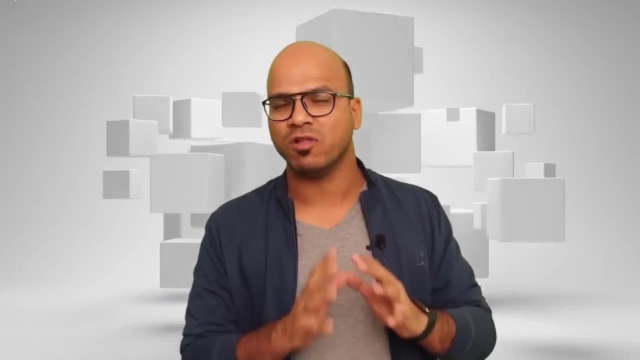 an object. integer is an object, but then we were skipping that part. What is object and why it's so important? See, ultimately, if we talk about programming world, what we do is we try to solve a real world issue with the help of virtual world solution. right So example: programming. 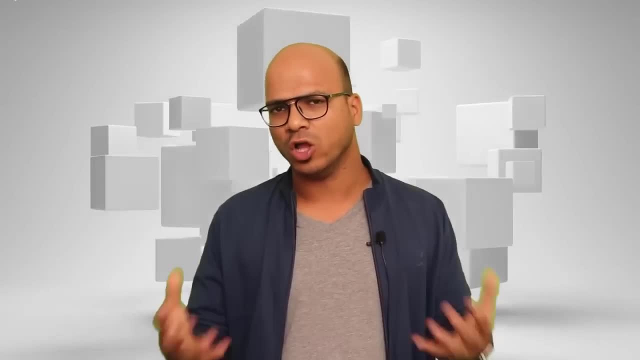 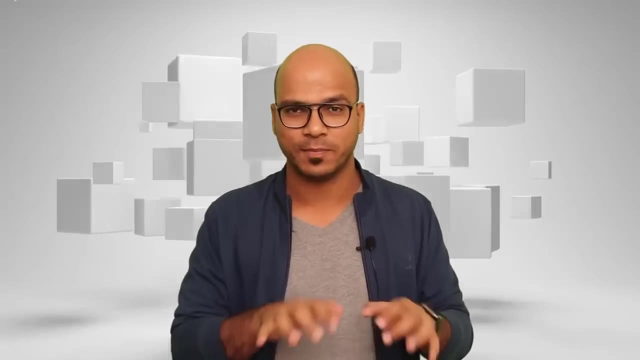 softwares, everything is virtual world. Now, in real world, we all use objects right. Example: if I want to record this video, I need a camera, right. If I want to call someone, I need a phone. If you want to type a code, you need a laptop, right. So for everything. 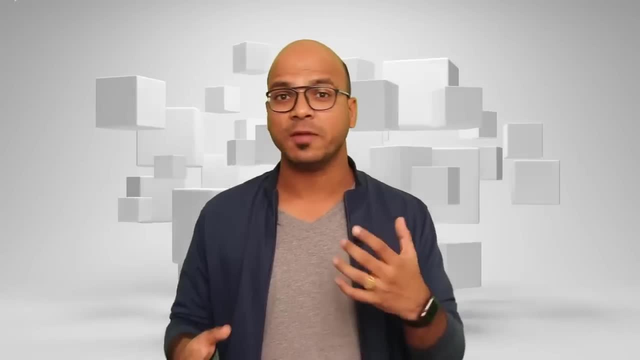 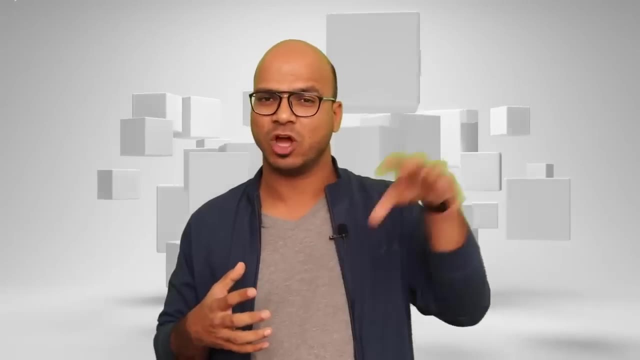 you need object. So in real world everything is object, In fact persons right. Example: if I have a company, if I want some work to be done, of course I need employees right And for me every employee is an object right. So an employee object is using a laptop object. So 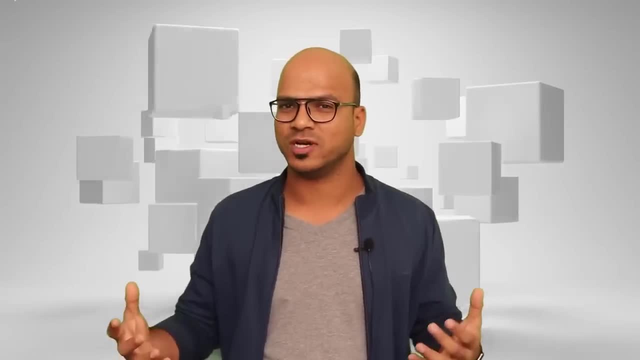 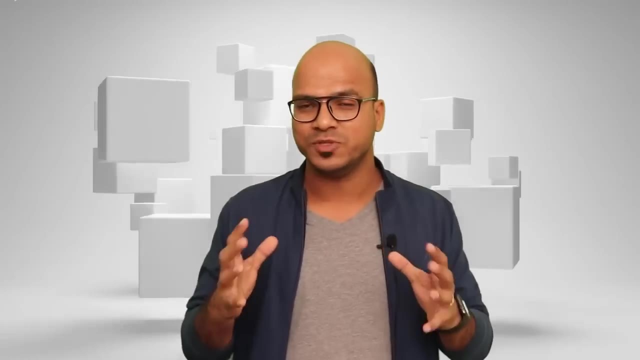 some employee object needs a AC object. right, That's how thing works. Everything is an object, we treat them as object. Now, what object will have? Object will have two things: Every object will have certain attributes and every object will have certain behavior. Now, when I say 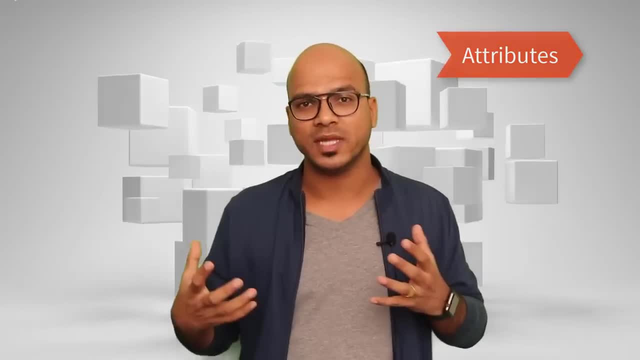 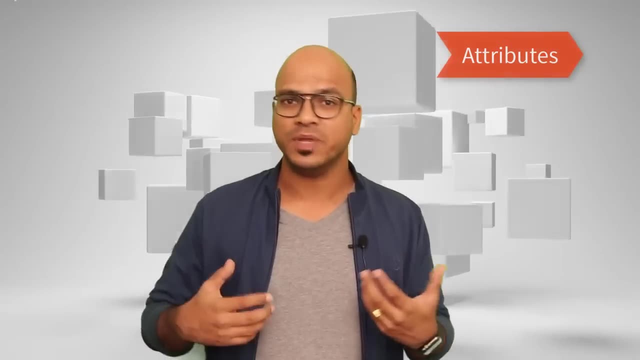 attribute. you can imagine them as data or you can say properties. Example: my height, it's one attribute. My age is one attribute. My name is one attribute. The company I work for is one attribute. right, Everything is those things are attribute. And then comes my behavior. I'm 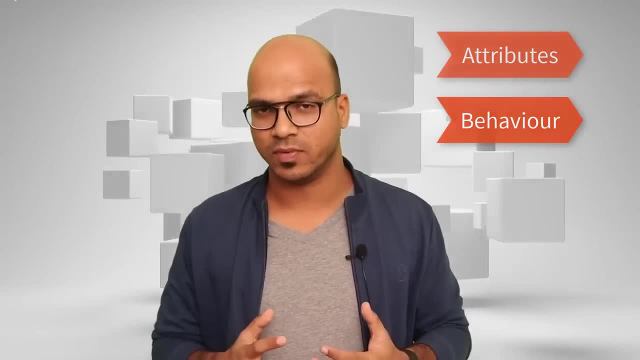 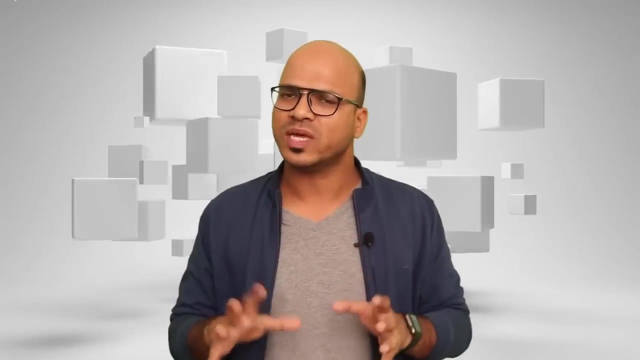 talking, I'm walking, I'm dancing. All these are behavior right, And then comes my behavior right. So our actions defines our behavior, And then we have attributes which we know. In other terms, you can say: as an object, I know something. As an object, I do something right, So I do. 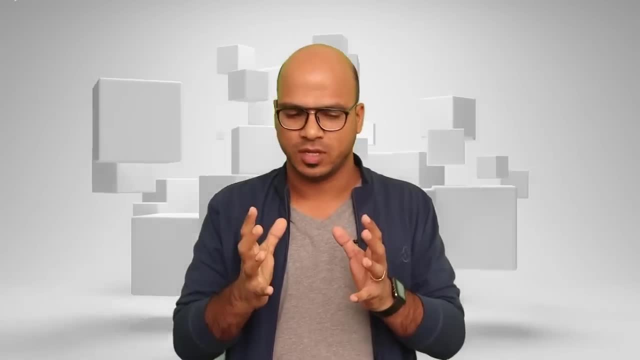 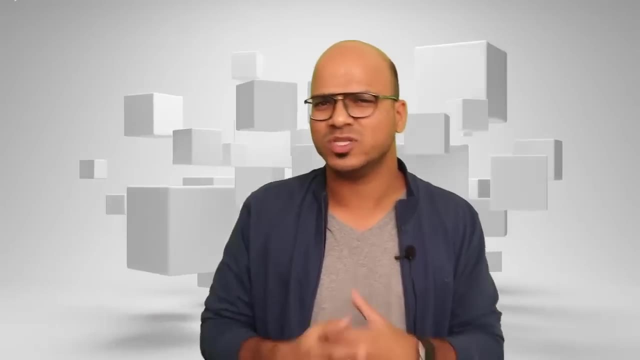 something based on something which I know right. So this is object. Object will have something where you can store data, and object will have some behavior. Now, this data which we normally use, those are variables. right, We have same variables. So if you want to store something, 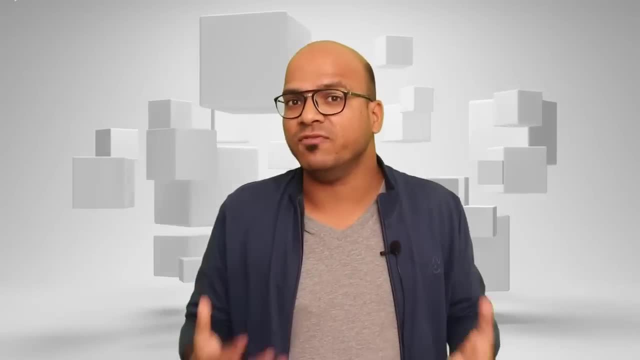 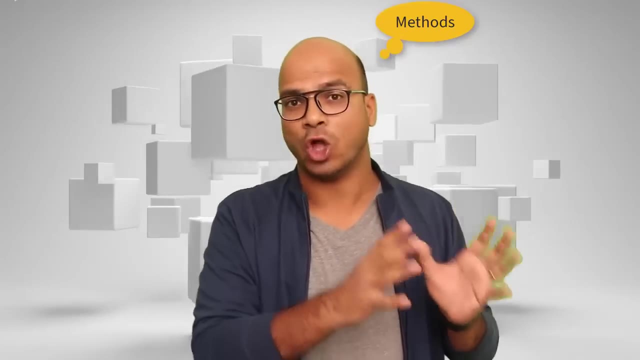 in object, we need to define variables. If you want to define the behavior, we need to use methods. Oh, that's something new. now What is method? We have done with functions, right? So functions in object-oriented programming they're called as methods, right? So so simple. 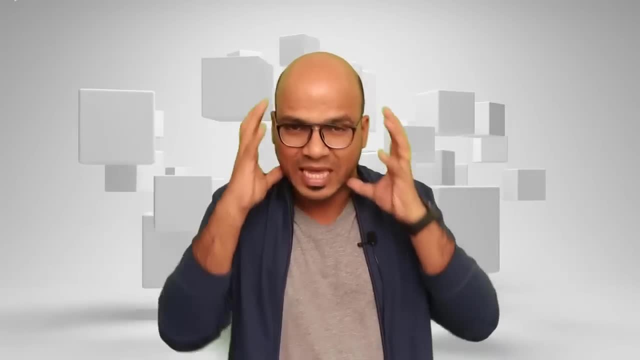 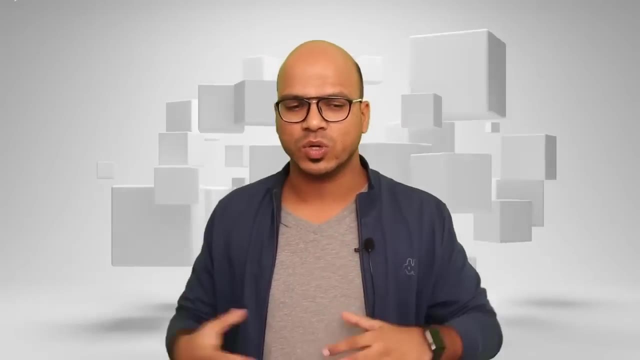 We have done all those stuff. The only change we have now is we need to think in an object term, See, object-oriented programming is not just about different syntax, It's also about the way you think. So now, if you want to achieve anything in programming, you need to think about. 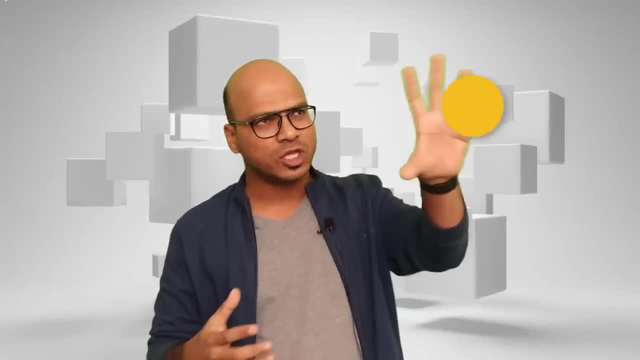 objects. So the moment you say you have a complex problem, think about the object, Think about multiple objects, Think about the object, Think about the object, Think about the object, Think about objects. and how can you connect them right? Because in OOPS we have so many concepts: One: 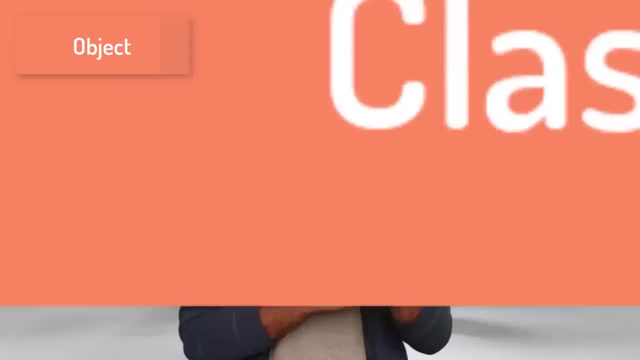 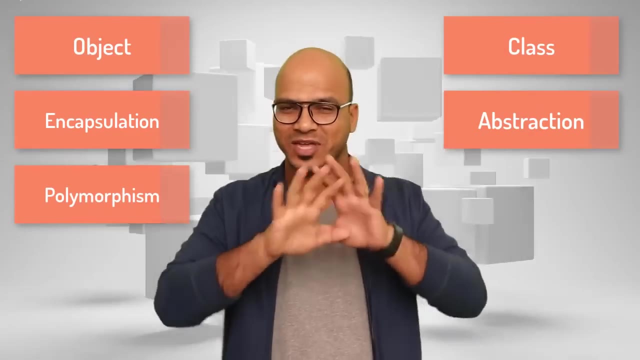 of the concepts is object, which we're going to see now. We have a concept of classes. We have a concept of encapsulation, abstraction, polymorphism. I know weird words, right, But don't worry, We will be covering everything in detail in the subsequent tutorials. So there's. 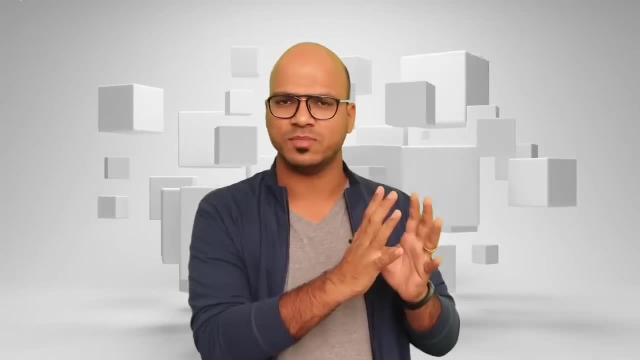 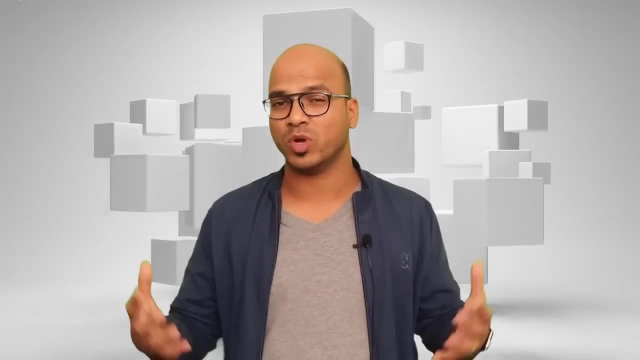 one thing which is important to discuss here about classes, because we have an object and we have a concept of class. It doesn't matter which language you work on, maybe Java, C++ or C, Sharp, whichever, whatever language which uses OOPS concept. You know, we always use this thing which is object. 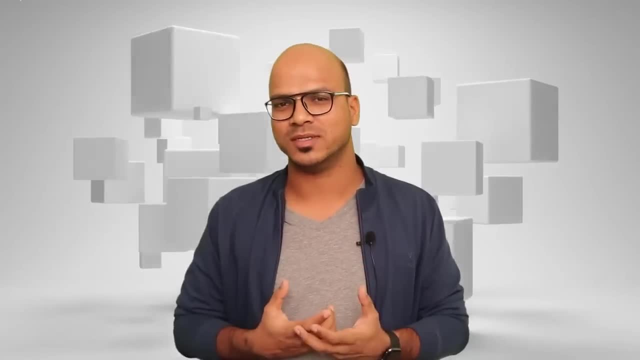 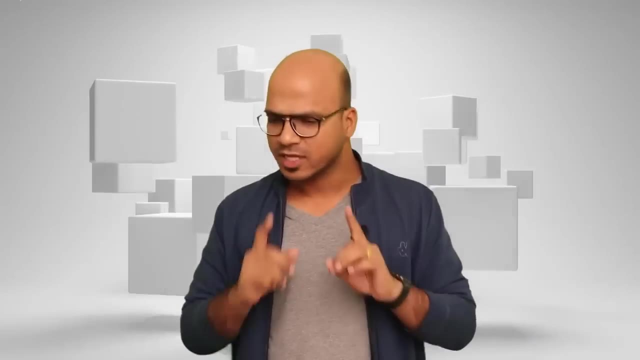 and class together. But why? Why they are so important? Of course, objects are important, because whatever you want to do can be done with the help of object. But why class is important? Now think about this When you want to see an object in real world- example, this camera. 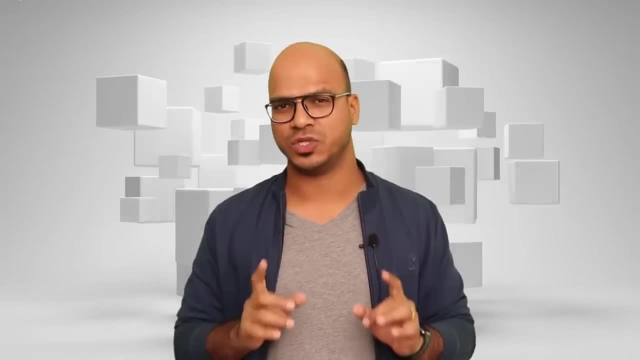 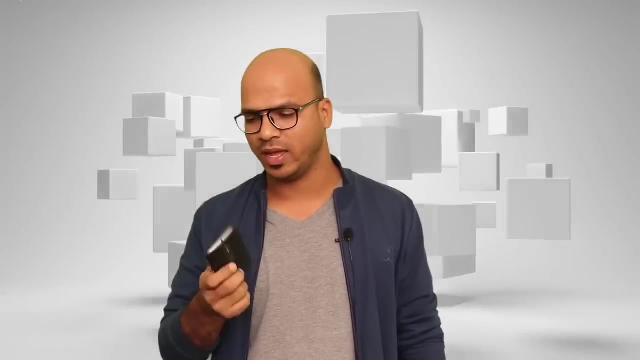 a fan or a clock, right. All these things are manufactured, right? So in some factory they have been manufactured. Or maybe you can talk about a phone Now. look at this phone. This is a Moto G3, okay, Now, it's not the only phone available here, right? So a lot of people. 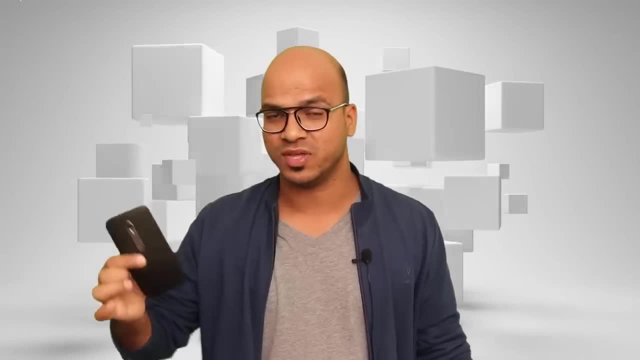 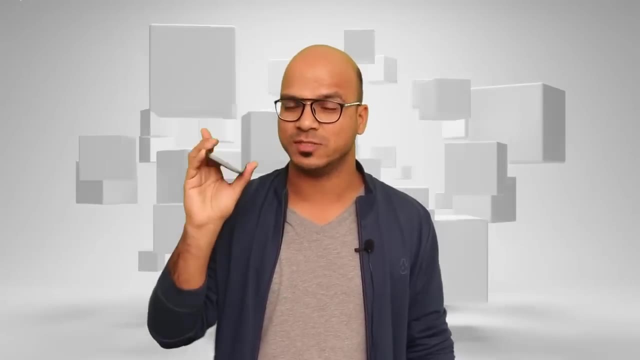 they have this phone. So that means we don't have one object of Moto G3. We have thousands or millions of objects. I'm using any number here. So imagine we have 5 million of this type of phones, which is Moto G3. Now, of course, someone must have designed it right And all. 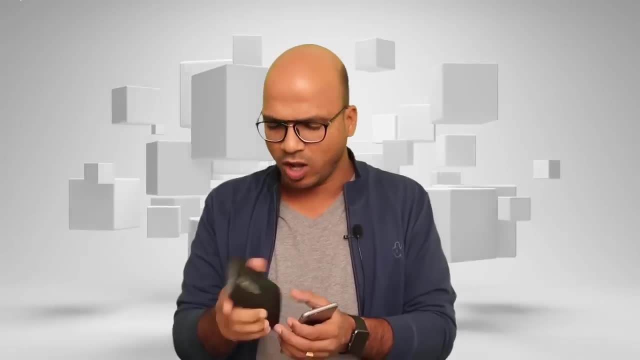 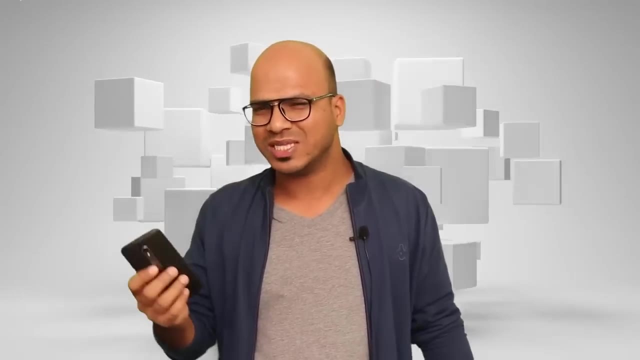 these phones have been manufactured somewhere. Maybe you can say: all these phones are made in China. okay, So we have a factory in China who is producing all this phone, But then Motorola says: this is a China phone. right, Of course. we don't say: this is a China phone. We say: this is a. 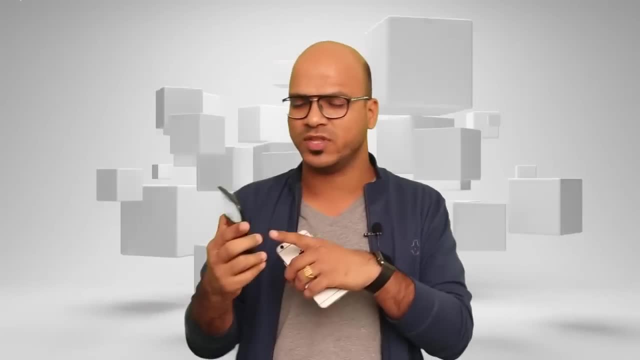 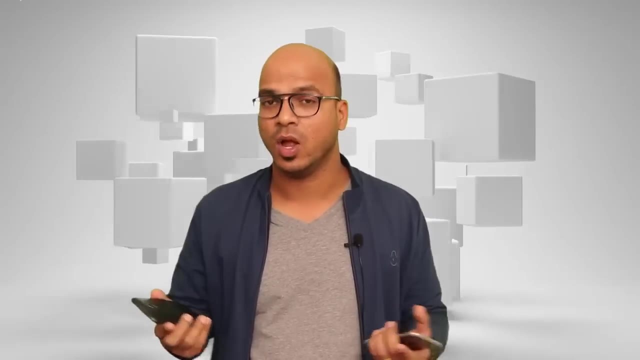 Motorola phone. Or we don't say, let's say the manufacturing is in India. We don't say it's an Indian phone, We say it's a Motorola phone. Why? Because manufacturing is not important. You can manufacture stuff anywhere. What is important is where it has been designed. okay. So this is. 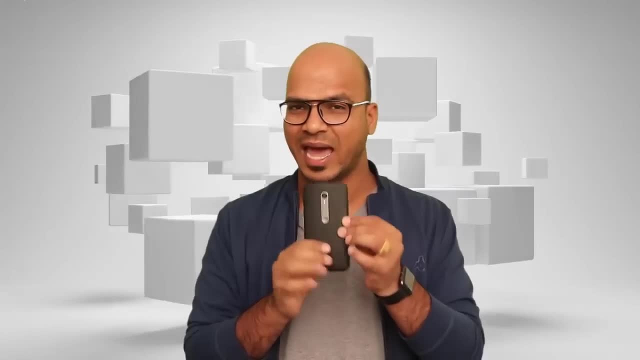 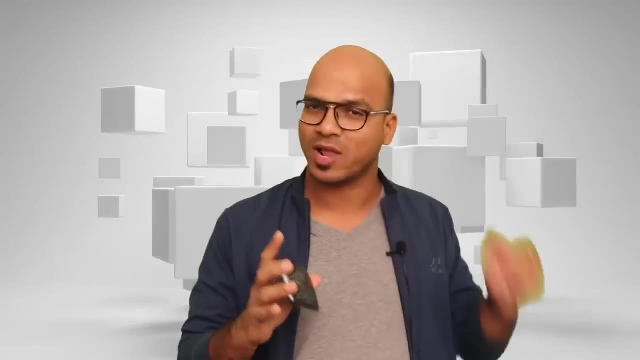 designed by Motorola. But even if you talk about this phone, this has been designed once and then they have manufactured multiple times. And that design in programming or in OOPS, we say class. So in a class you will write a design of the object. Imagine there's some factory. 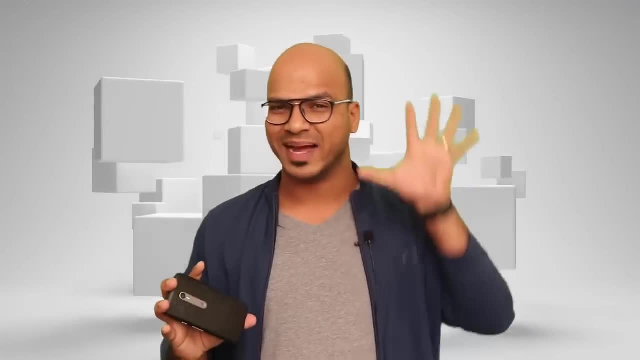 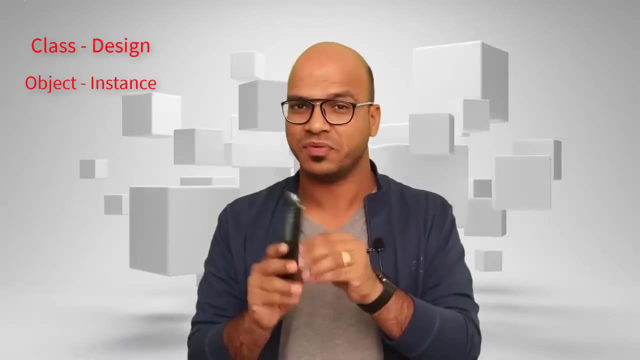 in your machine. who will create these objects? okay, So you have to provide a design so that you will get the object. So that means class is a design and objects they are real stuff. right, They are real entities. you can say, Or you can use another term called instance. 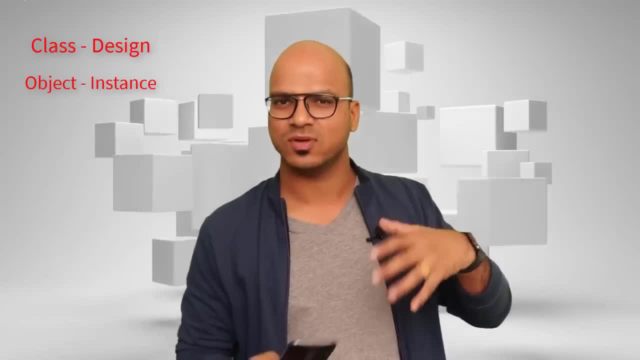 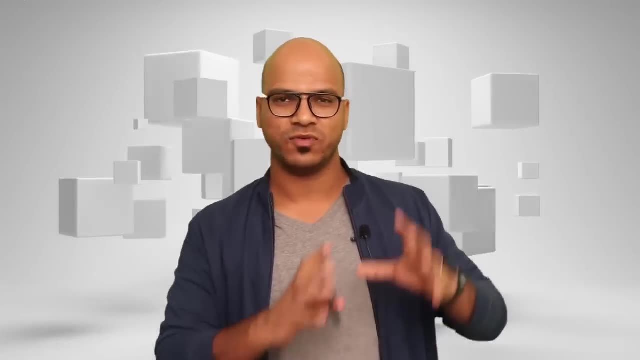 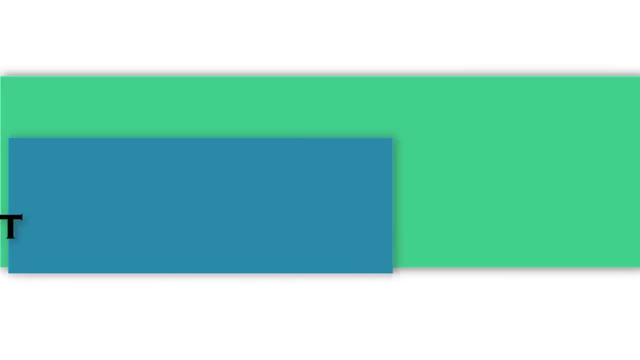 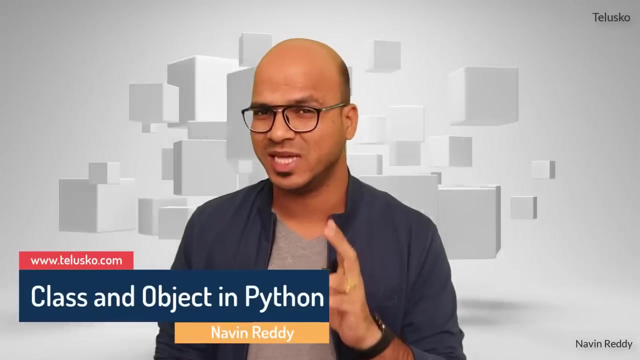 So you can imagine. this is an instance of a class. That's awesome, right? So point to remember: if you have a class, you can manufacture thousands or billions of these devices. So that's about class and object. In the last video we have talked about the theory of objects and a class. 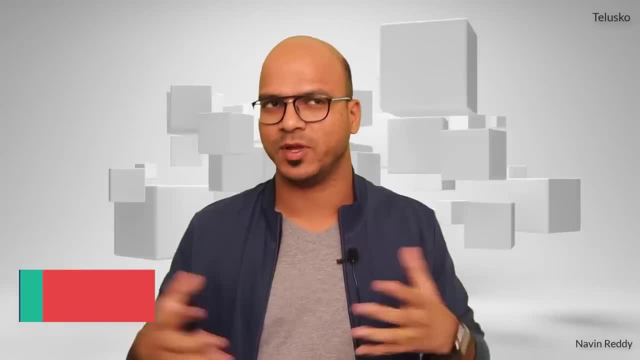 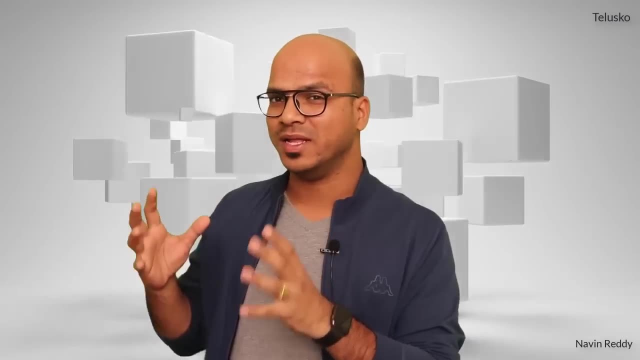 right? So, of course, before creating an object, you need to create a class, right? Because class is a design for the object, And if you don't have a design, how can you build something? In fact, even before building a tower, you need to create a blueprint of it, right, And that's. 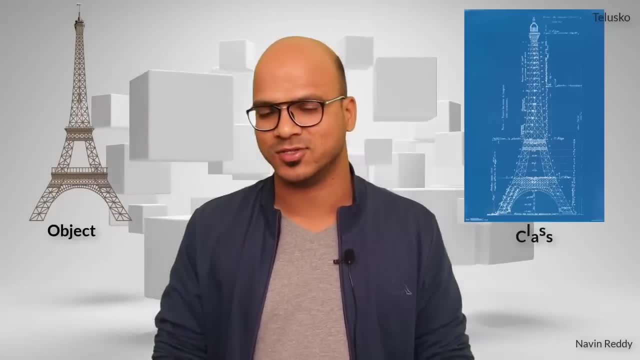 the same case here. So if you want an object, you need to create a class. So what I'm talking about is, you know. let's say I want to work with computers, So I'm a person I want to work with. 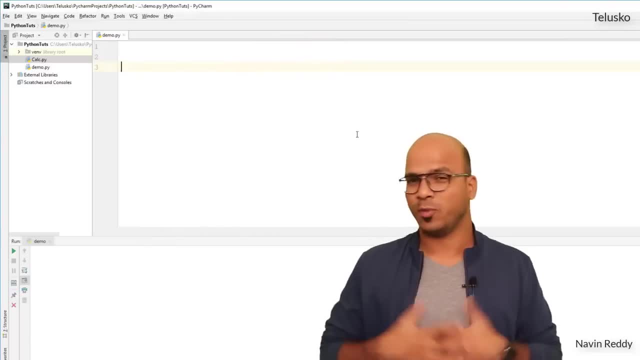 a computer. So of course I want an object of a computer, right? So let's say I'm a programmer and of course I want to work with a computer. So I will say comp1.. So this is my computer. 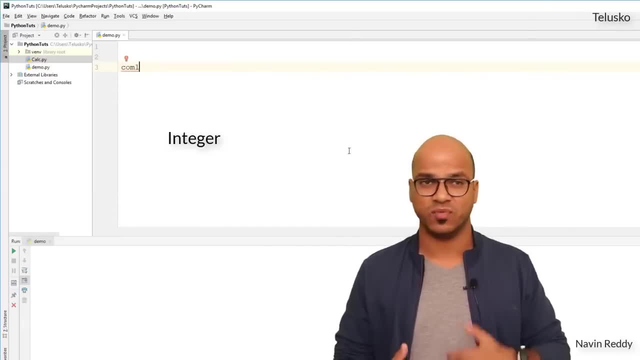 But see, the thing is, till this point we have worked with integers, we have worked with float string. Now all those are inbuilt types. right, We don't have any type as computer, So of course we need to create our own. 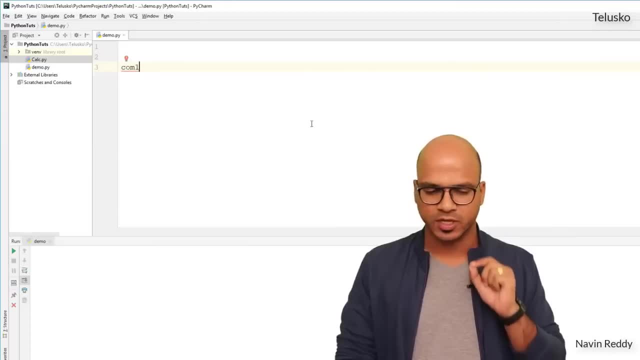 So we have to get our own class for it. So if you want to use a computer, you need to define a class here. So how do we define a class? The way we define a function is by saying def and function name. The way we define a class is using a class keyword. So we have to say class And 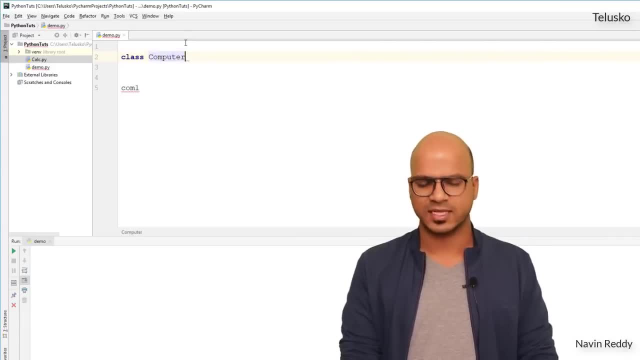 this class will, of course, have a name. In this case, I will use a name as computer. Okay, Now, this is how you define a class. You have to specify a colon. Now, after colon, this is your suite, right? So this is where you will mention your stuff. Now, what stuff we can put in a 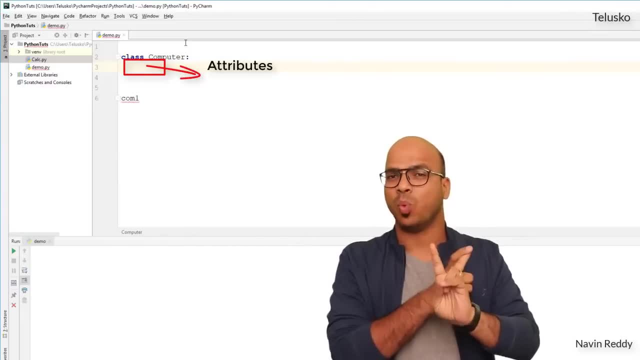 class Two things: The first thing is the attributes, The second one is the behavior. Oh now, when you say attribute, it is your variables. okay, The way you create variables, And the next thing we'll be having here is behavior, which is methods. What is methods? 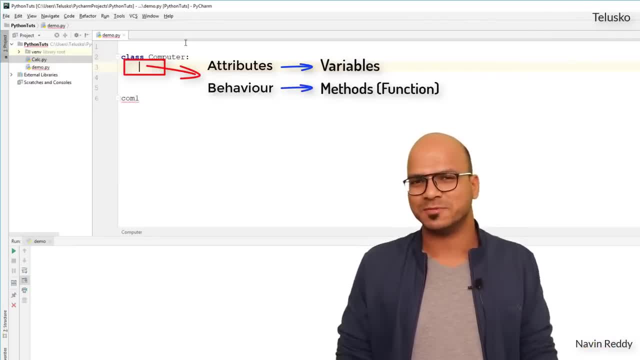 Functions. So now the functions which we are using from a long time, but here we call them as methods. So next time, when you are calling a function, but that function is a part of a class, instead of calling them as functions you have to say methods, right, Okay Now. 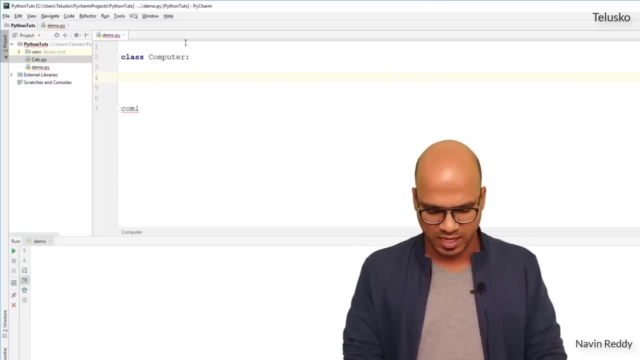 let's define some methods here. Now what method I'm talking about? let's say, let me get a method here. I will say config, because every machine has a configuration right. So I will say config. We got that self keyword there. That's weird. What is self? Because, see, I'm not typing it. 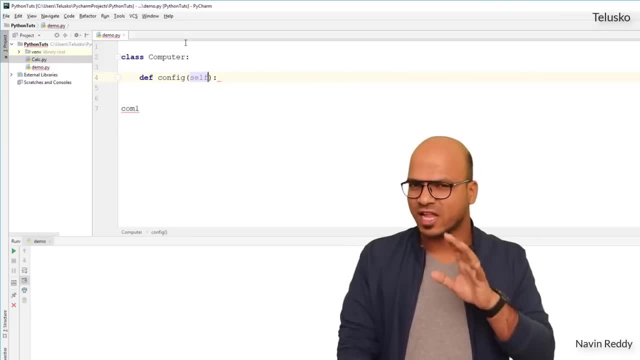 okay. So I mean the moment I say bracket, it says self. We'll talk about that self later, but time being let's keep it there. You can imagine we don't have any self here, okay, For time being. imagine we don't have anything like self, Okay. And here we'll say we got a computer. 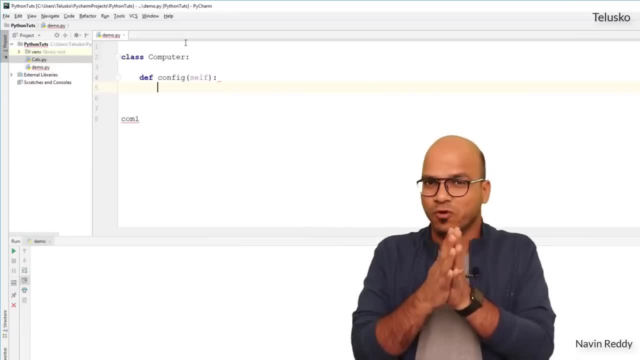 class. and then we got a config method. or you can say function, but try to move from that function term to method term, right. So we got a method here which is config, And here I'm printing the config of this machine and I want to say, hey, this is i5 machine with. 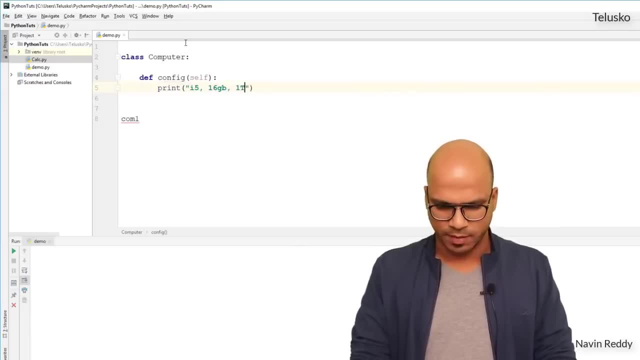 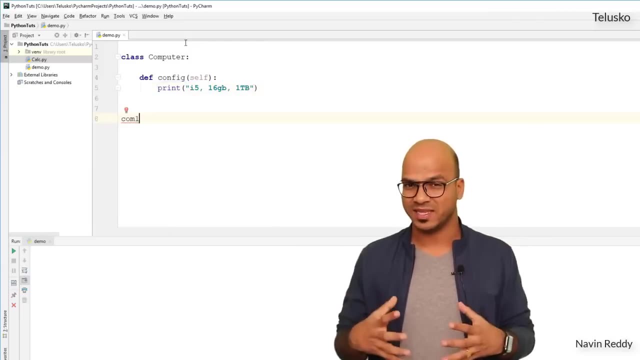 16 GB RAM and it has 1 TB huddle. Now, this is very common config now which we find nowadays right, And that's what I'm doing here. So we got a class computer, We got a method in that. 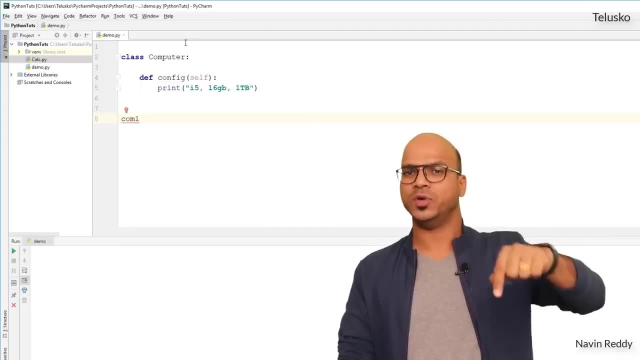 Example: here I'm saying comp1 is the object of computer. but we cannot simply do that right. We cannot simply say comp1, because no one will understand what this comp1 is. Example if I say comp1 is a variable right Now, since in Python we don't have to statically mention the type of 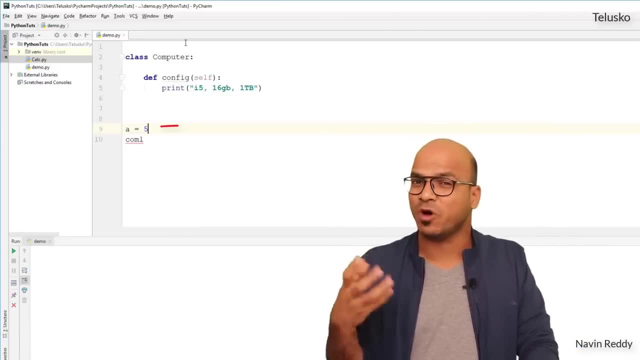 it. So what we can do is, when you say a equal to 5,, now the type of a becomes integer, right. If I say a is 5.5, the type of a becomes float. If I assign a value of string type, if I say 8, even. 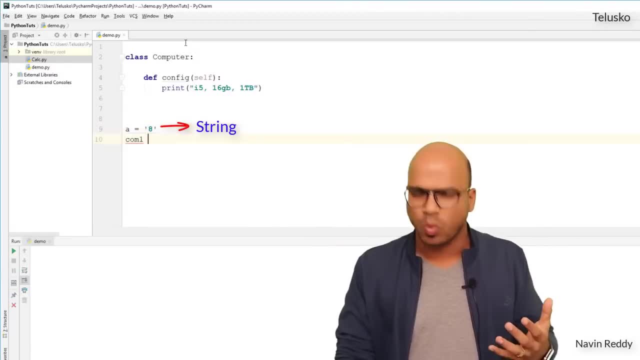 if that 8 is number, we are putting that in single code, right, That becomes a string. What about comp1?? Comp1 here don't have a type. We have to mention: hey, this comp1 is an object of computer. 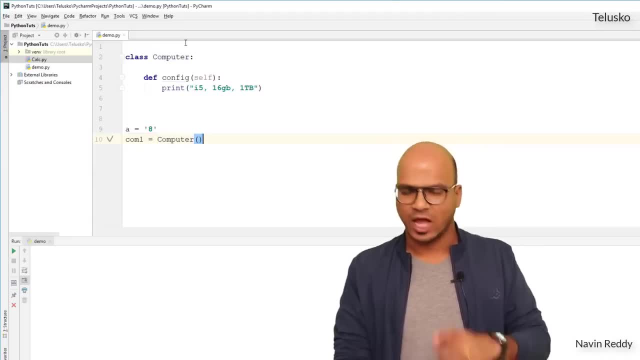 And you have to give this round brackets. Now, if you are coming from another, you know from different programming background, like Java C sharp, we have a concept of constructor right. So this is a constructor there. So this will give you the object of computer. Now how do I? 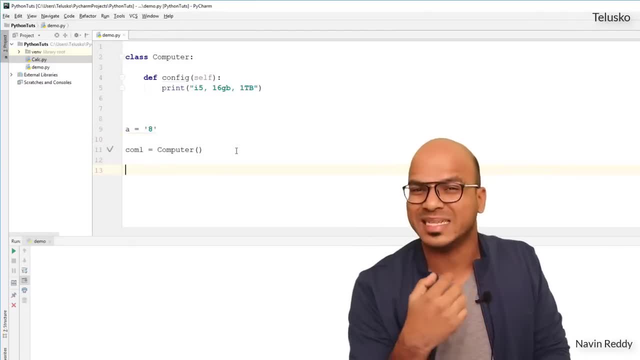 know that, If you remember, in one of the video we have talked about a type function, right? So you can use type function here. So I will say print, I will define type print, the type of comp1.. Let's see what happens, what it gives you. So if I run this code, it say: 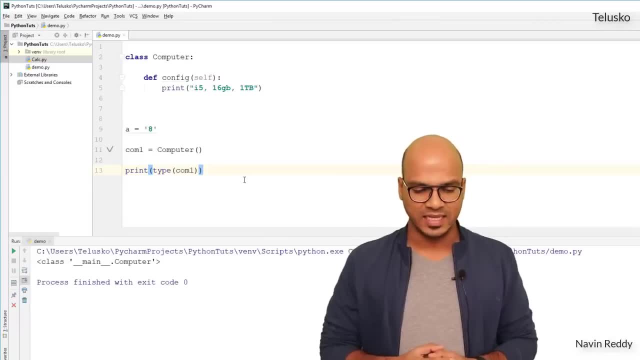 hey, this is a class. okay. Now we have a different keyword class and this belongs to a computer. That's important, okay? So it gives you the module name. The module name is main because we are running this code from here, And then we have a class called as computer. Now 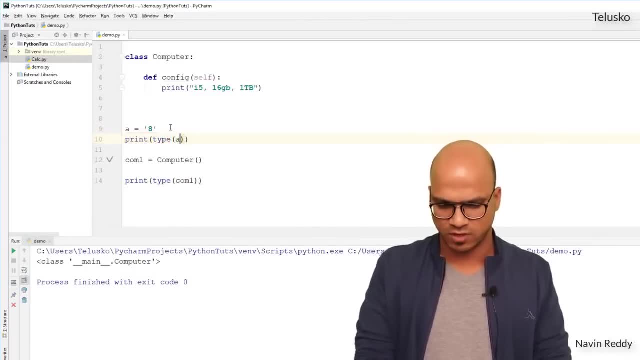 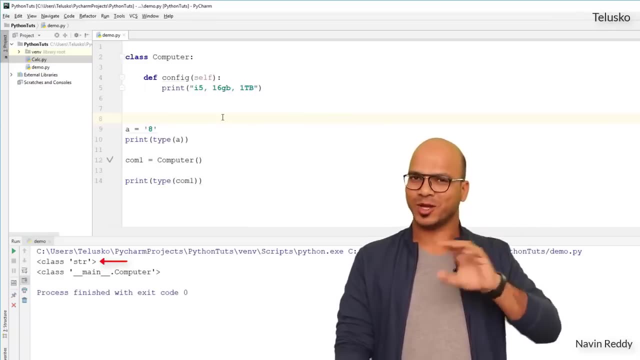 if you remember when we worked with string as well, string gives the same thing. So if I print the type of a, it also says the same thing. Can you see that It says class str- right, So we are using this concept from a long time, but this is where we are defining it now. 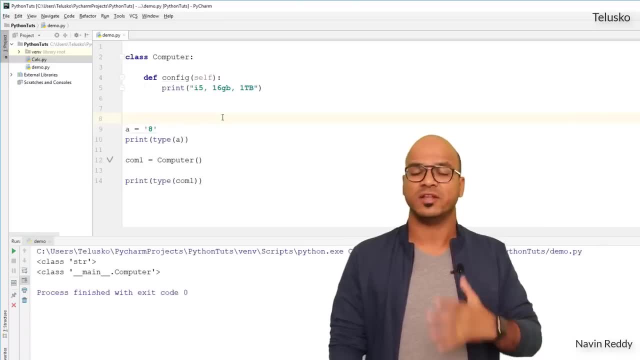 So string str is also a class, The same way computer is a class. The difference is: str is an inbuilt class, Computer is our class. okay, That's how you define it. So you say class computer and then we have dev config. 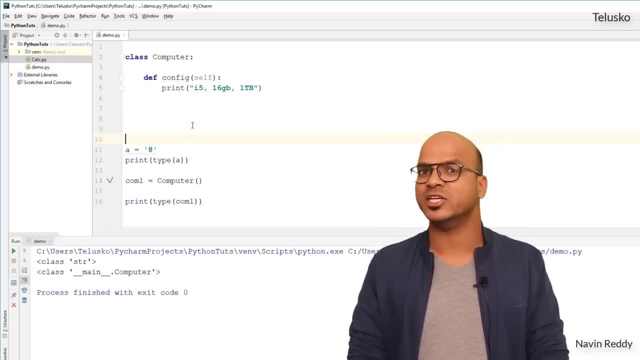 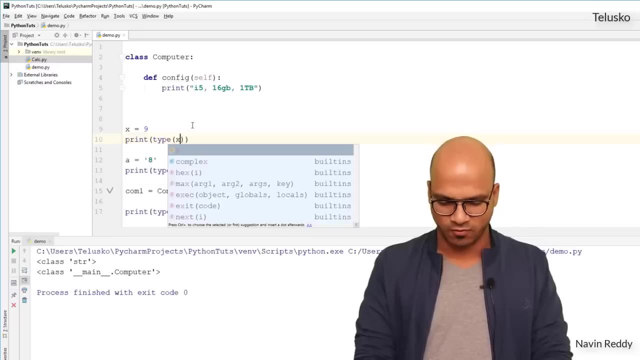 In fact there's one more thing. If you remember, when we worked with integers, we have also said that integers are also object. Let's try it here. I will say x equal to 9 and let me print the type of x. Can you see that When I print the type of x it says class int. So even this integer. 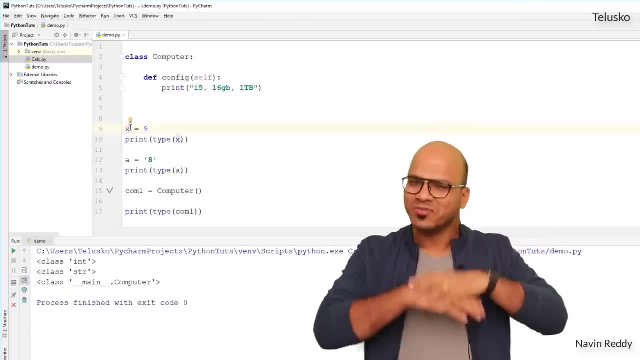 this x is an object of integer. now, right, So everything is object in Python, right? So there are some inbuilt objects and there are some objects which we create. And the way you create your own class is by saying class computer, whatever class name. Make sure that you don't. 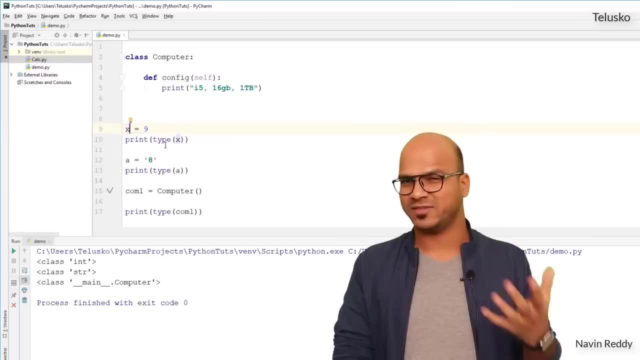 use inbuilt class name, because it will give you error, right, Or maybe you might face some bugs. So we have so in a class we are defining a function config, and then, oh, not, function method config, and then we are printing just a statement. Now question arise: how will you call? 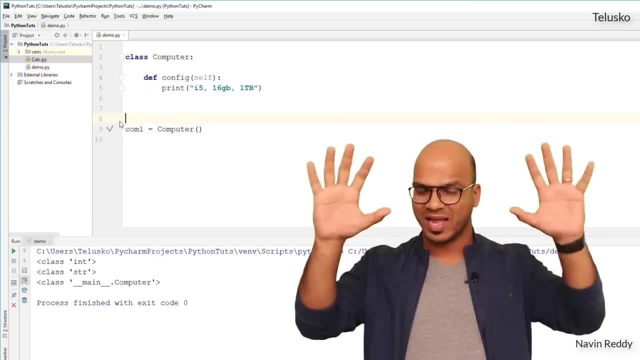 it. So let me remove this all Extra stuff which we are doing. So we got a class, we got the object. I want to call that config. Now what do you think? How will you do it So normally when you have a function? 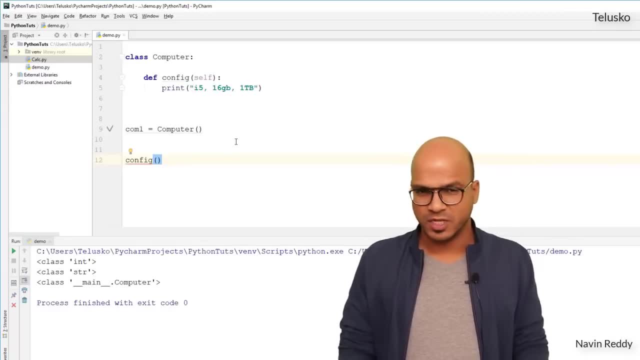 you mention the function name right Here. in this case it is config, But you are getting an error. Why error? So if I go back here, it says unresolved reference, or that's weird. What is giving you unresolved? Because of course, normally till this point we were mentioning the function as it is. 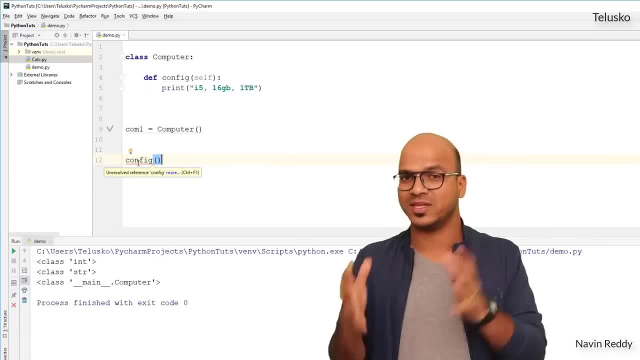 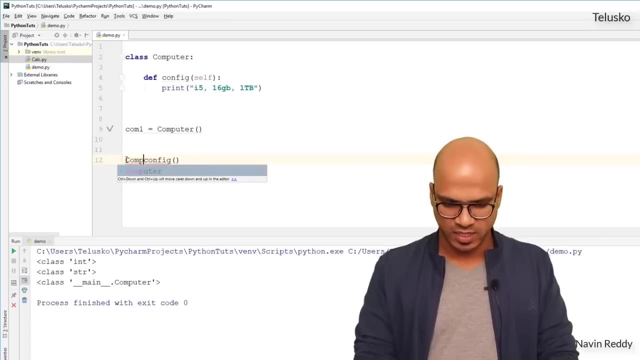 open. But now we have written that function or a method inside a class. So in order to access that we have to mention the class name. and the class name here is computer, So we have to say computerconfig, Important. So steps. remember the steps. You have to mention the computer class. 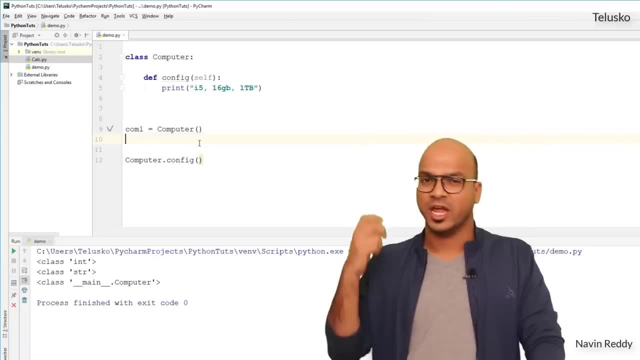 which is class name, and then you have to say config. So let me repeat: If you want to use a method, we have to mention a class name first, which is, I mean, where it belongs to computer, and then you have to mention config. And if I run this code, oh, we got an error, But why So? 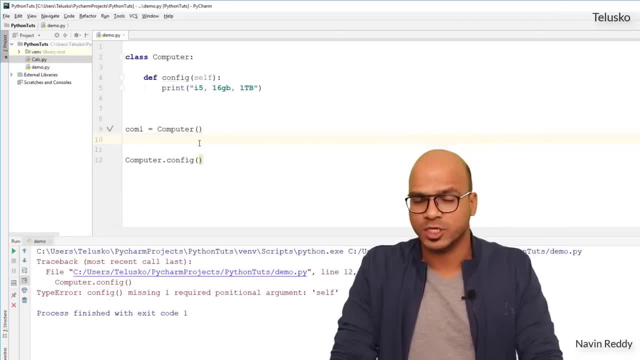 think about this: One class can have multiple objects right. One object, two object, five objects right. In this case, we are using only one object, which is comp one. The thing is, this config function or a method will change its behavior based on the object right, Because 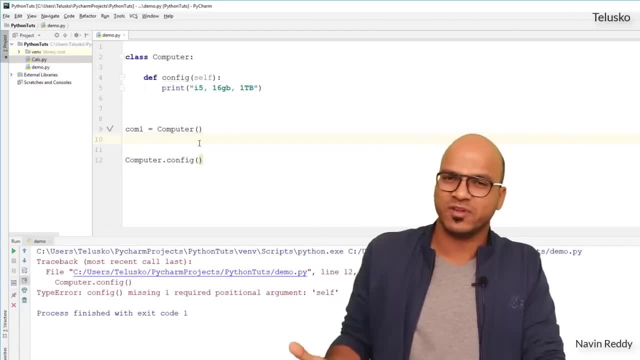 different objects have a different behavior because, depend upon what they know, they have a different behavior. See, in this case I'm not depending on any data, right, But maybe there's a chance that this config will depend upon some data and every object will have its own data. 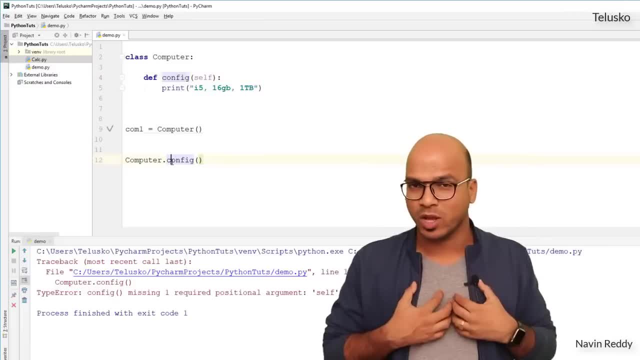 right Again, we'll talk about that later. But every object is different, right? If I'm calling object, I'm doing that. So if I say, hey, walk, but whom am I supposed to say walk? So I have to. 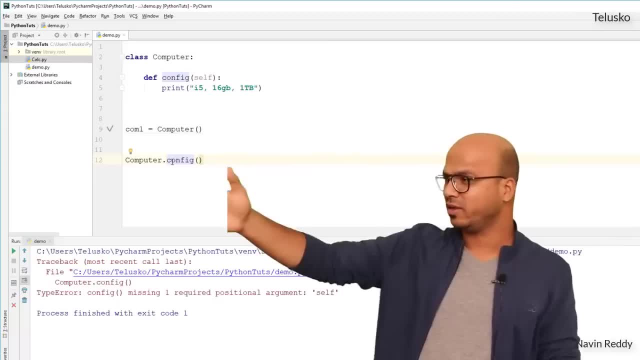 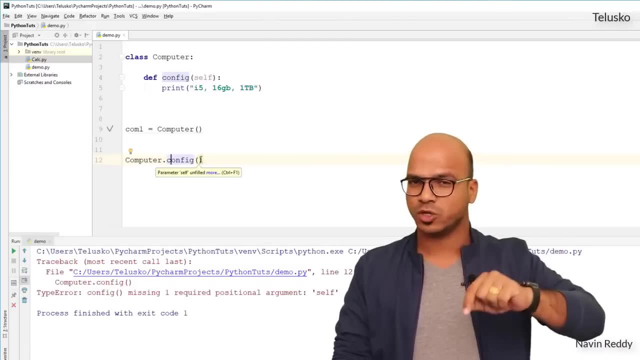 mention: hey Ravi walk. Hey Mukesh walk, Hey Kiran walk. So I have to mention the names as well. right, In the same way, when I say computer config, you have to also mention for which object. 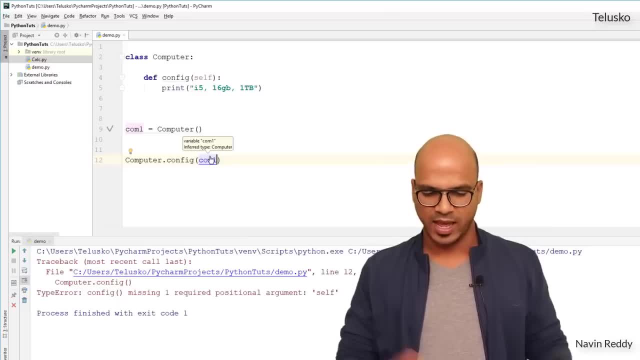 you're talking about, And I'm talking about comp one. So I'm saying, hey, I want the config for comp one. Now, luckily we have only one object here, So there's no confusion. But let's say if 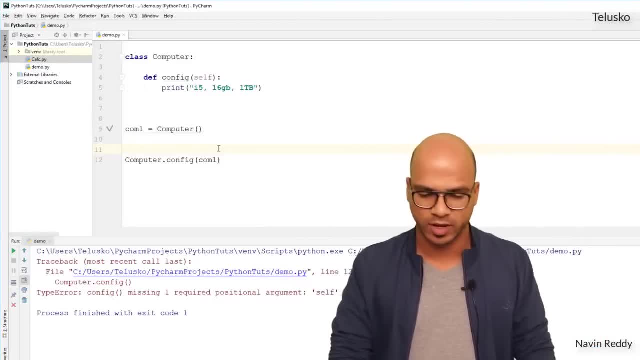 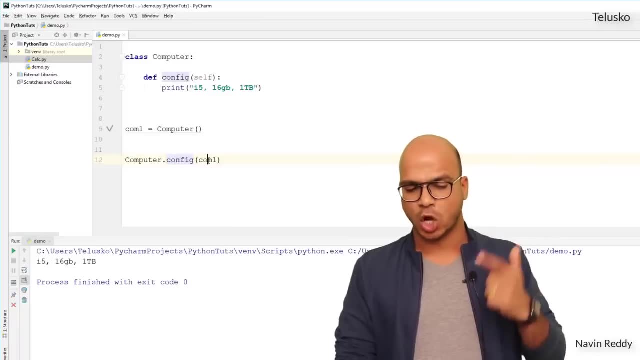 you have thousands of objects, you have to mention the object name as well. So we are doing comp one or it works. You can see that we got the output. So we are calling config and we are passing comp one. And this comp one is a parameter, right, It's an argument. So when you call config, 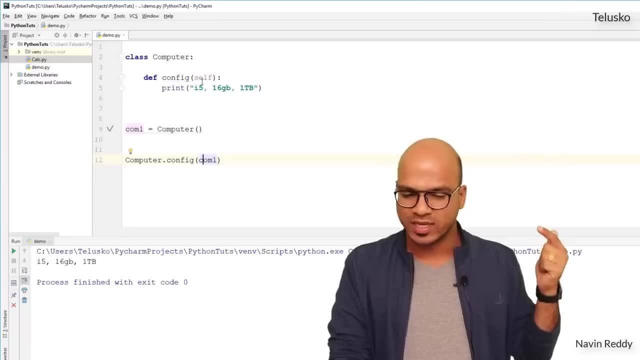 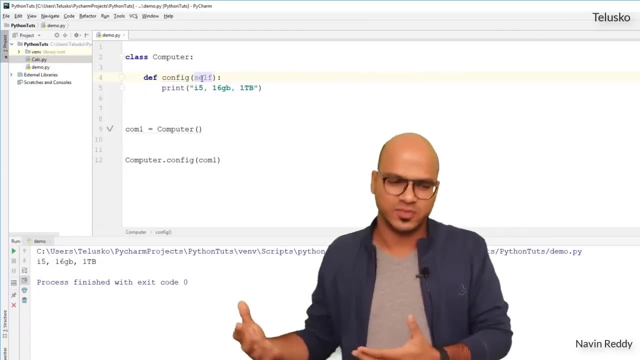 you're passing this comp one as the argument and it is going in self. So what is this self? Self is the object which you're passing Again. this thing will get more clear once you see further videos, right? So this is a complex concept if you're learning OOPS for the first time. 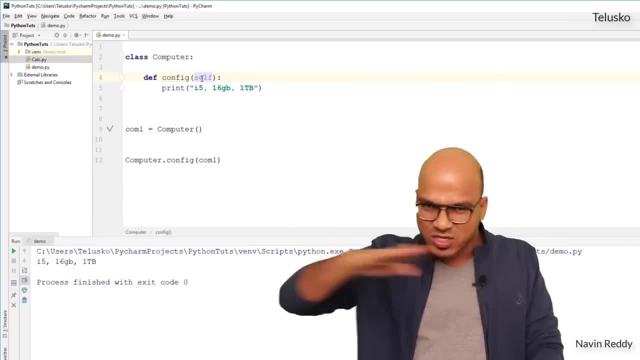 But, step by step, everything will go inside your brain. okay, So this is the first layer. Again, in the next video we'll talk about some more. We'll add more layers to it. We'll add more layers, and then I will make sure that you'll get. 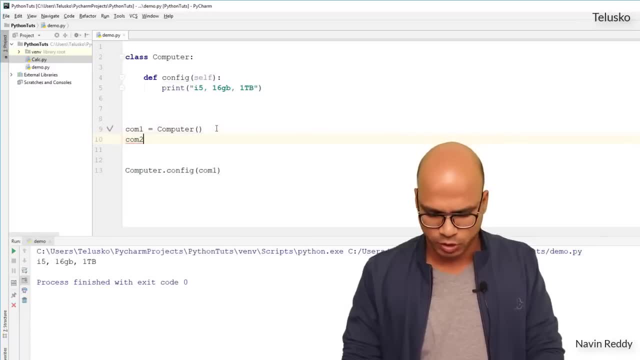 everything about it. Okay, let's create some more objects, okay. So I will say: comp two is equal to computer, right? So we got comp one, we got comp two. So in total we have two objects, which is: 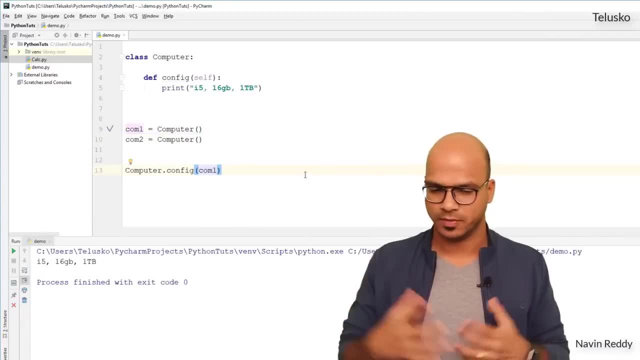 comp one and comp two, But we have only one class, which is computer. If I want to call config for comp two, what you will do? You will say computerconfig. and this time you're saying, hey, I want to call config for comp two. So in the first instance I'm saying: Mukesh, walk right Or I will. 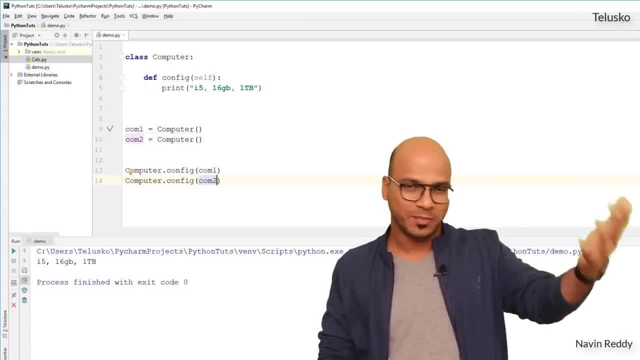 say: walk In bracket. I'm passing Mukesh, I will say: hey, human, walk In bracket. I'm passing Ravi, right In the same way. here I'm saying: hey, computer, show me your configuration, and I'm. 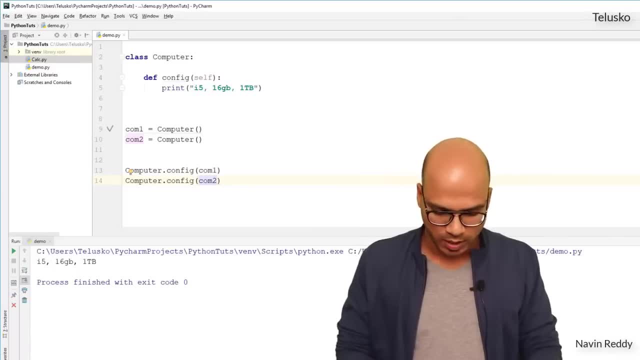 talking about comp one. Hey, computer, I want your configuration for comp two. So if on this code you can see we are getting same data, because at this point we are not changing data for different objects, We can do that later. So there's one way, right? If you want to call config, we have. 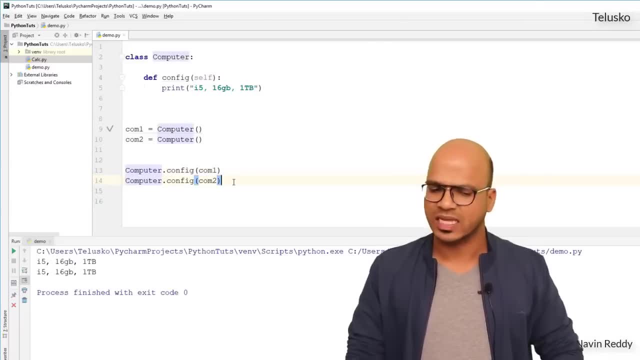 another way. If you think about this, this looks good, right, This looks clean, because we are saying, hey, computer, and then we have to pass the object name, which is comp one. But there's one more way. what you can do is you can mention comp oneconfig. Now, in this case, you are using the object itself. 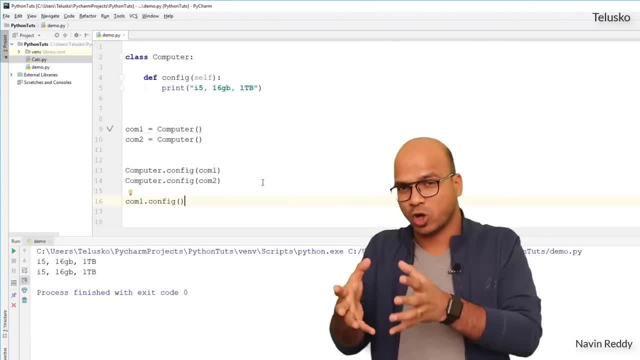 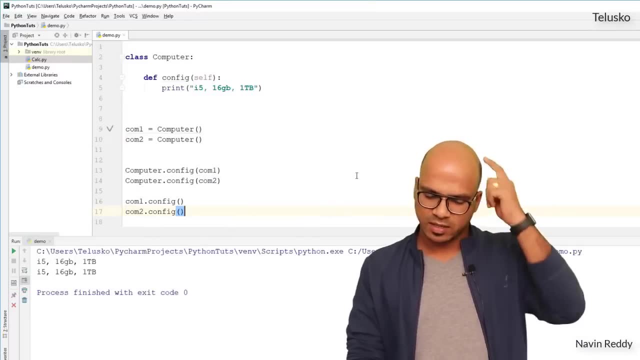 to call the function. So you're saying comp oneconfig, But question is: we are not passing it right. Example: let's do it for comp two as well. I will say comp twoconfig and you can see this time I'm not passing anything inside config and still it works. You can see the output. 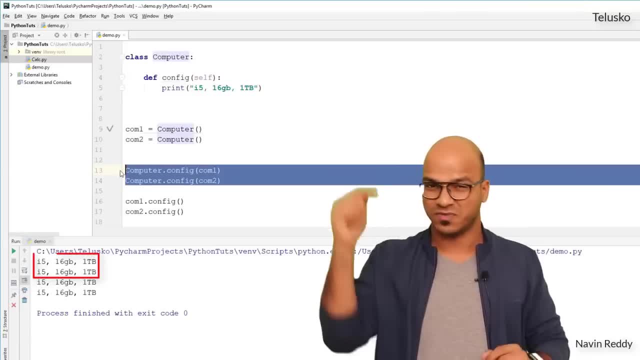 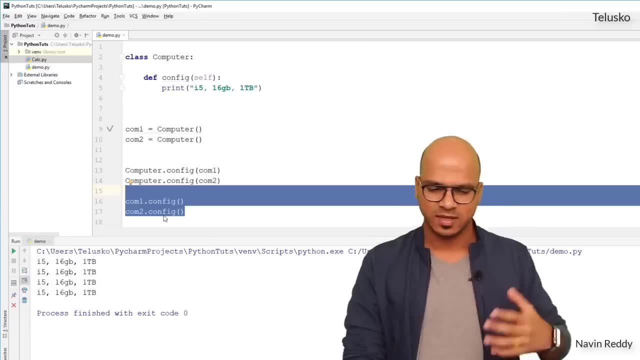 it works. We got four times the same data because the first two is because of this lines and the next two is because of this line. right, But why is it working? It's because this is another behavior of it. So when you say comp oneconfig, you are calling config. See, we are specifying. 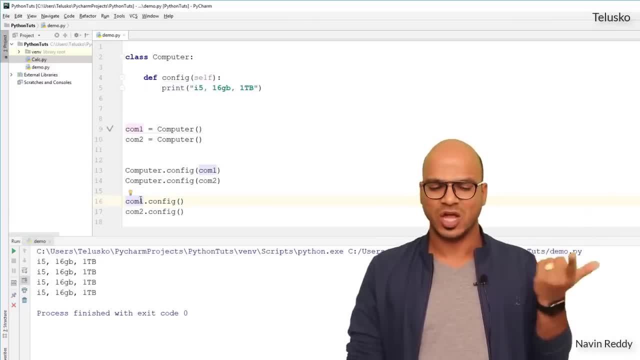 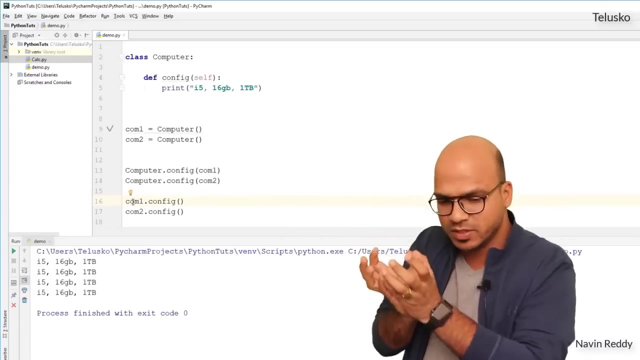 of which class. it is right. So comp one belongs to computer. So now we know config belongs to computer. The moment you say comp oneconfig, when you are calling it behind the scene, this config will take comp one as a parameter. So behind the scene config will take that comp one as argument. 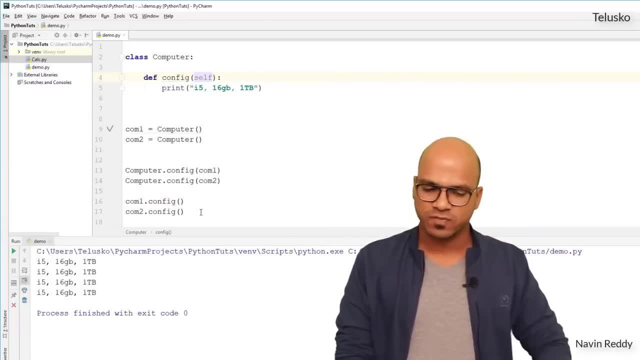 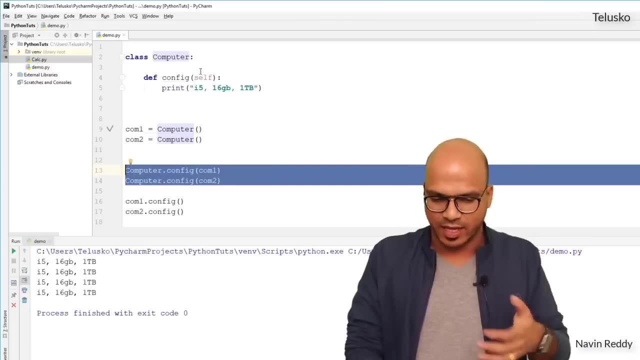 and it will pass that in self. okay. So in most of the code you will see this type of syntax, not this one. But I have done this just to explain you how this syntax link like. okay, So how this? 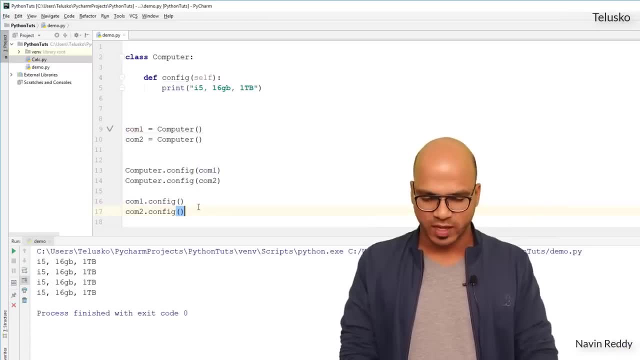 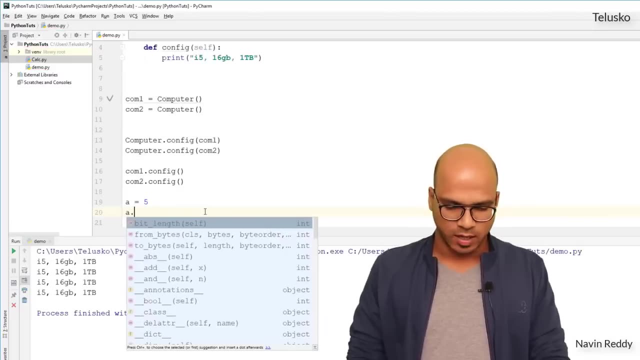 exactly works, But normally we use this syntax. the second one, And that's why, whatever we have done till now- example: if I work with a variable of inside, so if I say a equal to five and if I say a dot, so whatever function we use here, example- I want to know the bit length. Now, 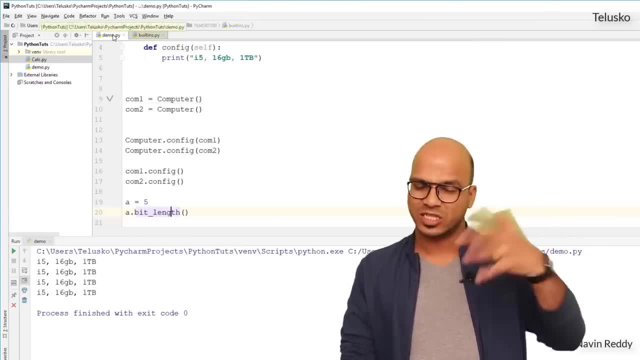 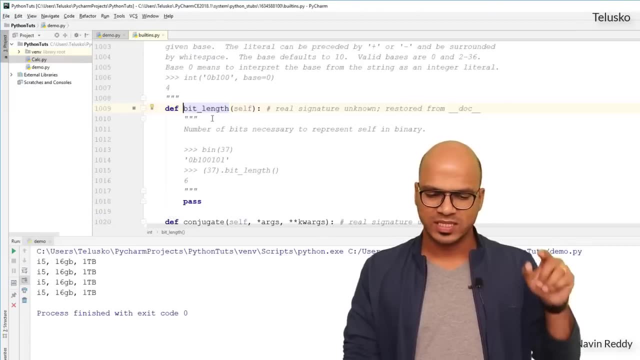 in this thing. you can see if I say control space, you know you can actually see the documentation by clicking on this control and click on the function name. So press control and click on the function name, You can see. it takes you to the function. It says bit length self. So 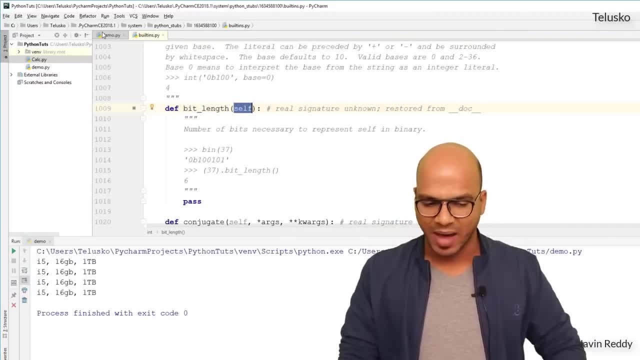 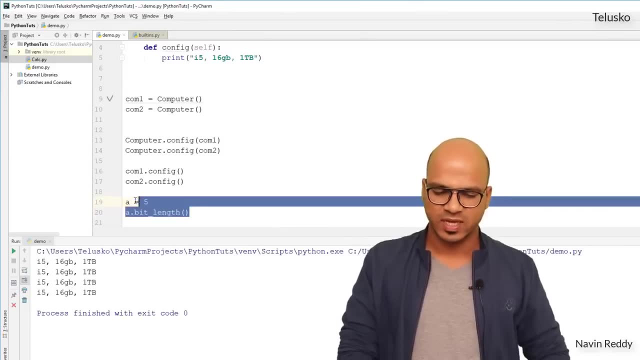 as a definition, it is accepting self. But when you're passing it, when you're calling bit length, we are not passing it. So this A is an object, right, It goes as a parameter. So self is the object which you are passing. We'll discuss more about that once we start with variables and then 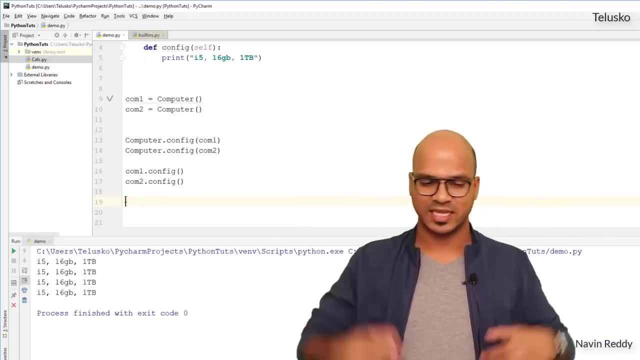 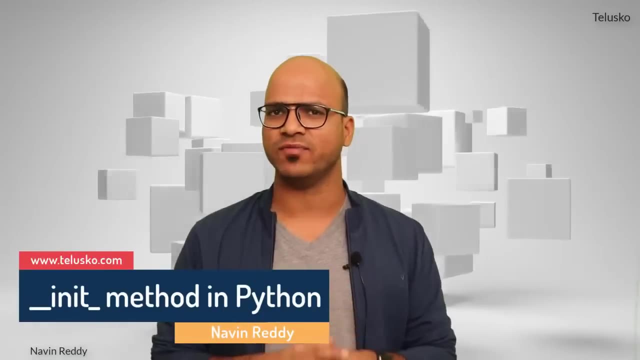 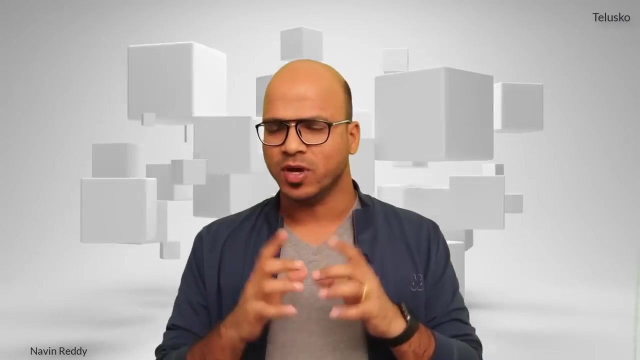 attributes, all the stuff, But time being, this is how you create a class and that's how you create an object. Now, in the last video, we have talked about oops, concepts. right, We have seen what is object and a class. Let's explore it more Now. if you remember when we talked about objects- object. 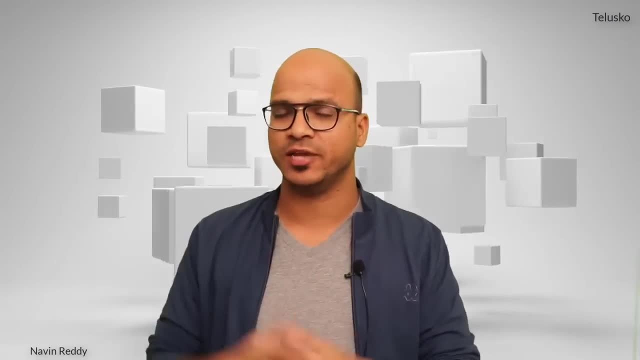 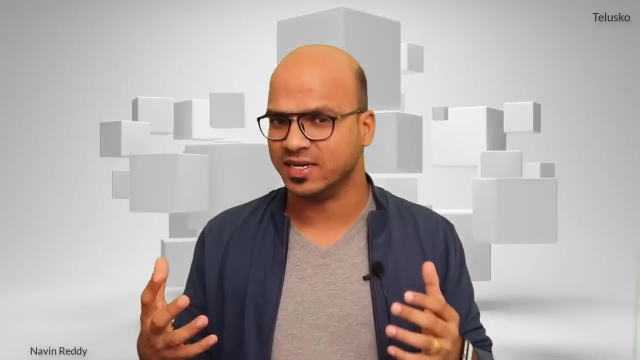 will be having two stuff right. One is it will be having some attributes and it will also have a behavior. Now when you say attributes, those are variables, right, We can create variables, and behavior is your methods, and then methods are almost same as functions, But in oops we call: 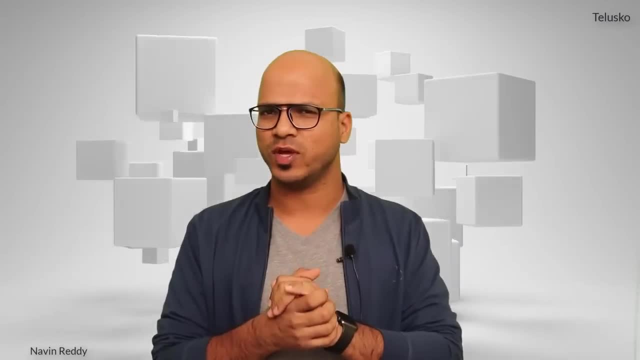 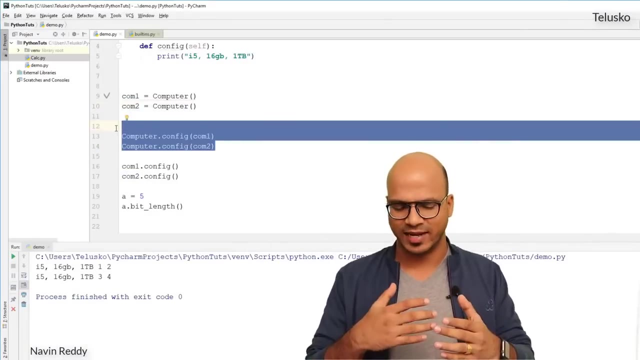 them as methods Right Now. here we have to work with methods. right, We have not worked with variables yet, So what I will do is just to demonstrate that. let me just remove this thing here, because we know that we can call config using the object itself, or we can call it with the help of class by passing the. 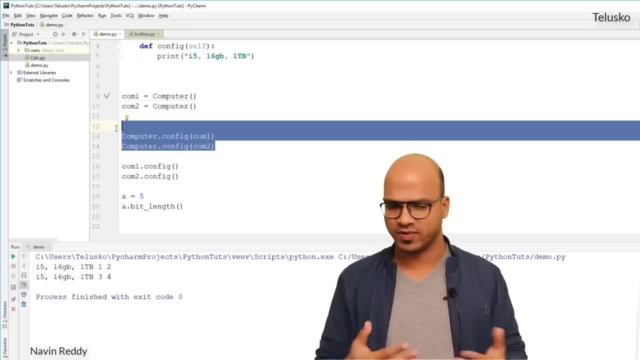 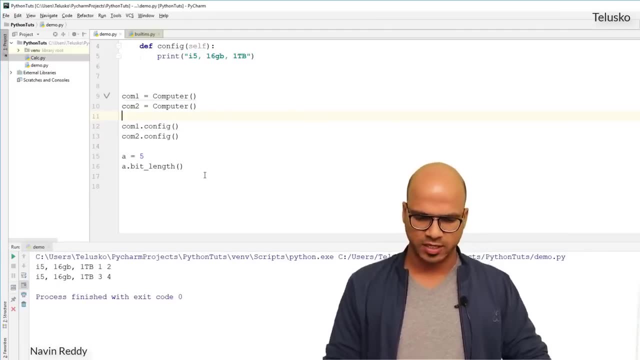 object. Now, syntactically, we normally go for the second one, which is calling the method from the object. It makes much more sense, right? So we'll remove that part. and so once we got the object, let's remove this A as well, just to clean it up stuff here. Now what I will do is: I want to have 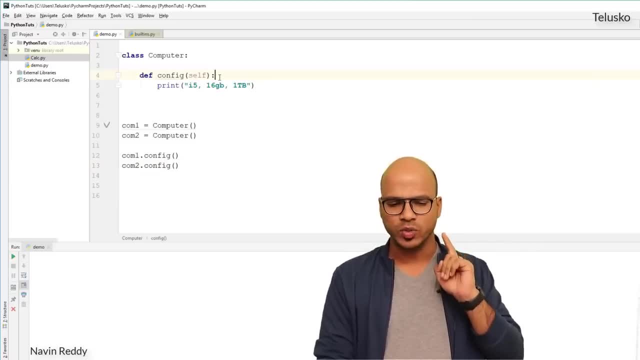 certain variables. Now, when I say variables, what I want to do is I want to have two variables: one which defines the type of CPU I'm working with and the amount of RAM I have. Example, if you talk about any computer, these two are very important, right, The CPU which you are using and 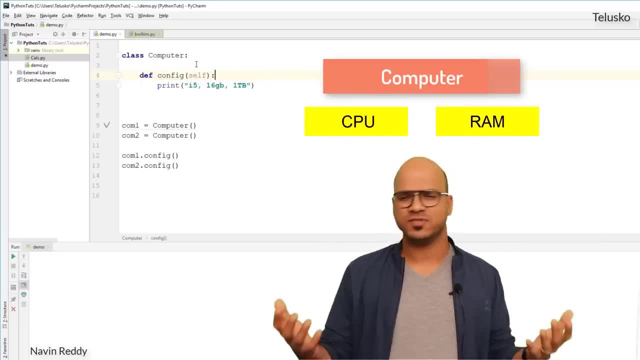 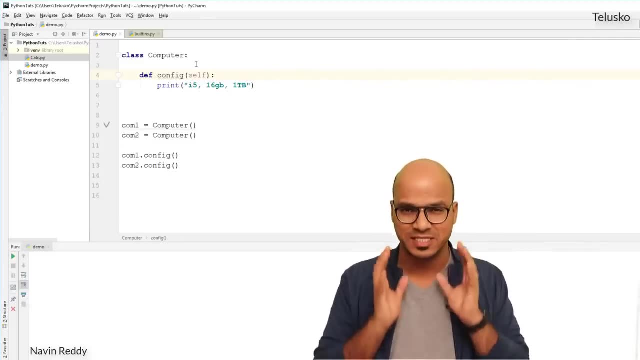 all RAM, maybe 8 GB RAM or 16 GB RAM, And in terms of CPU, we have, let's say, i3, i5, i7 or maybe some AMD series. Okay, we have different parameters as well, but just to keep it simple, let's only focus. 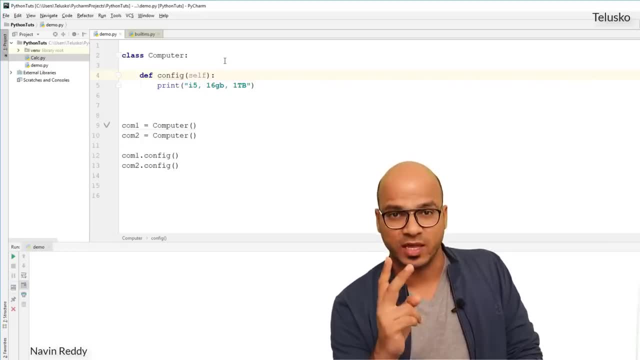 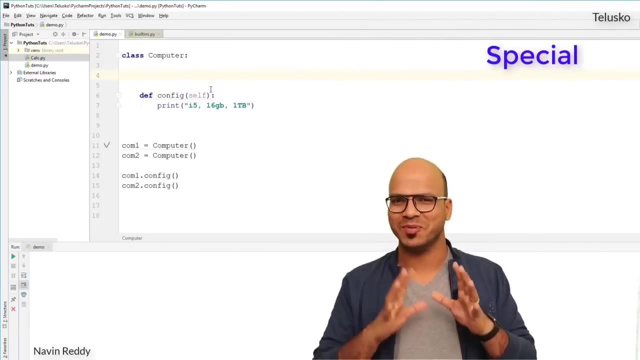 on two things: CPU and RAM capacity. Now when you say we have two variables- let's say we have two variables, where do you find that? So we can use a special method which is available in a class. Now when I say special, you know right. So the moment you say special, we have talked about 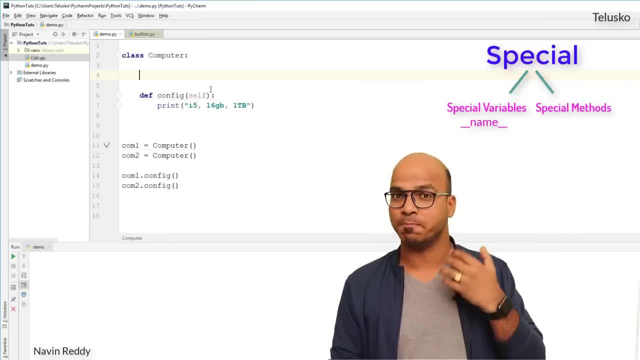 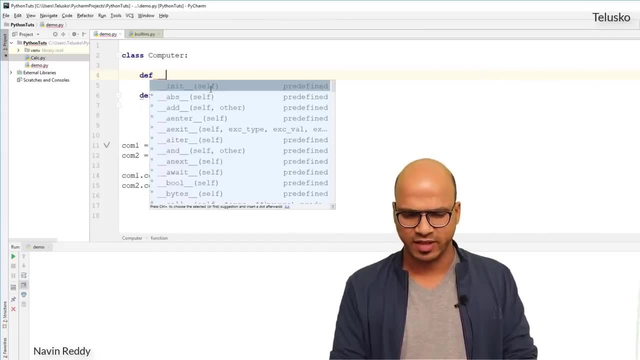 special variable which is underscore, underscore name. In the same way, we have special method, which is init, and when I say special, it will be having underscores as well. So let's define that. So we'll say: def- underscore, underscore, init. You can see that we are getting suggestions as well. 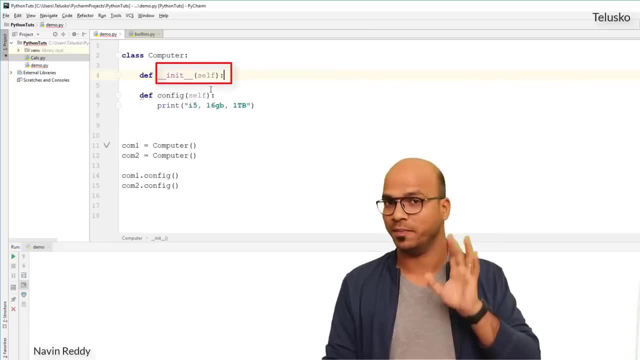 and the moment I say enter, you can see we have the function name or the method name as init and we are passing self. Now see, self is not something which I'm typing, that is coming automatically. So it's compulsory to have those argument: okay, which is self? And in here we can do something. 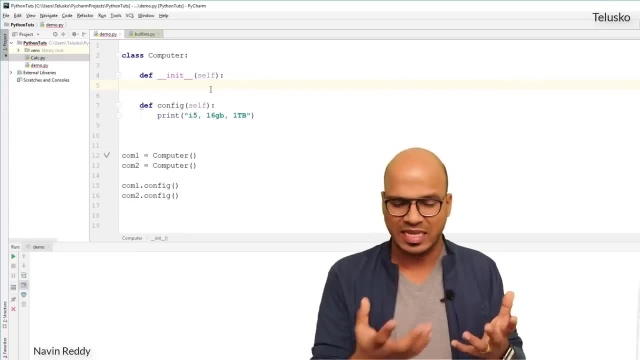 Normally we use init to initialize the variables. okay, And that's what the name itself init initialize. right Now, if you are coming from C, C++ or Java background, we use constructor, right, So you can imagine this is our constructor, but then it is init method. The advantage here is: 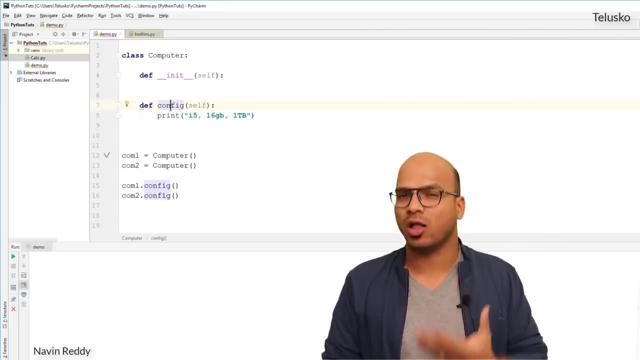 normally see. if you want to work with config, you are supposed to call config. okay, So it's compulsory for you to call config, Otherwise it will not get executed. The idea behind init is it will be getting called automatically. Example: if I go back here and let's say I want to print. 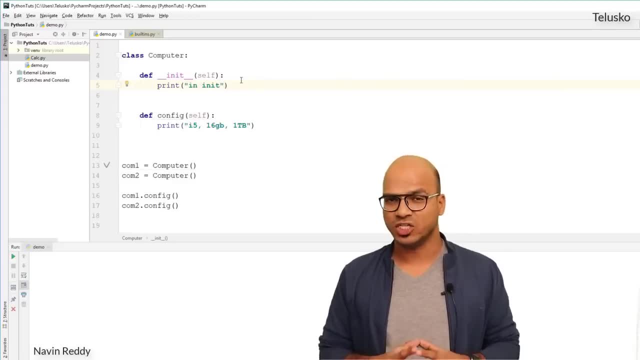 something and I will print in init. So you can see. I have defined a function called as init. I'm not calling it, okay. So anywhere in the code I'm not calling init, I'm calling config because I want to execute it. The moment I run this code you can see it prints in init, and that too it. 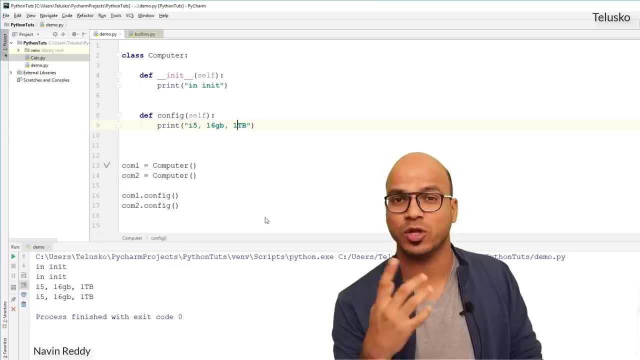 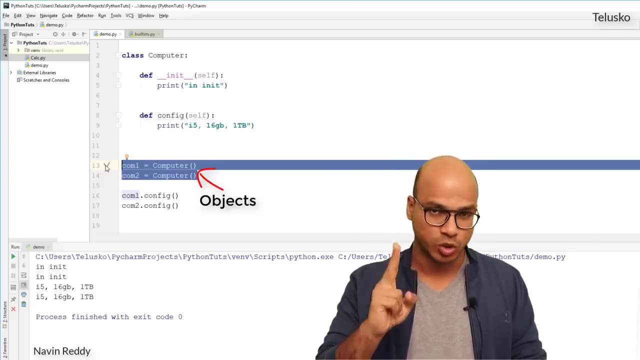 prints two times. Now why two times? Because for every object it will get called once. So you can see in the code I'm creating two objects: One is com1, one second is com2.. So we got two objects. 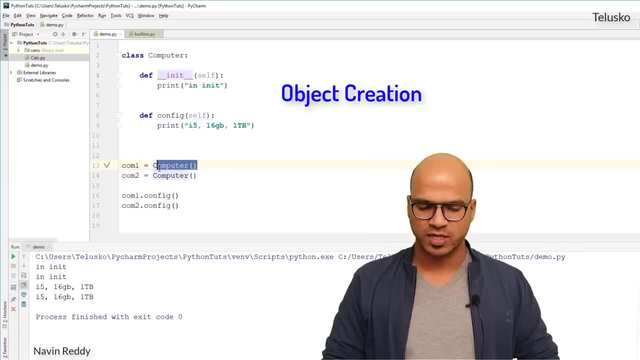 and it will call init two times. So this is the object creation. So when you say computer bracket, it will instantiate, It will call init for you. Now I want to pass some arguments. okay, I want to pass CPU and RAM So in the constructor itself. you can pass that So in the computer. 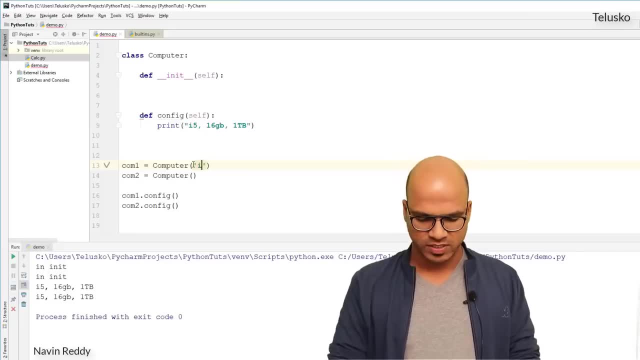 bracket itself. you can pass it. So I can say: I have a CPU here which is, let's say, i5 and the amount of RAM we have is 16 GB. The second computer we have, let's say reason 3 and the amount of RAM we have, let's say, 8 GB. So we have two computers with 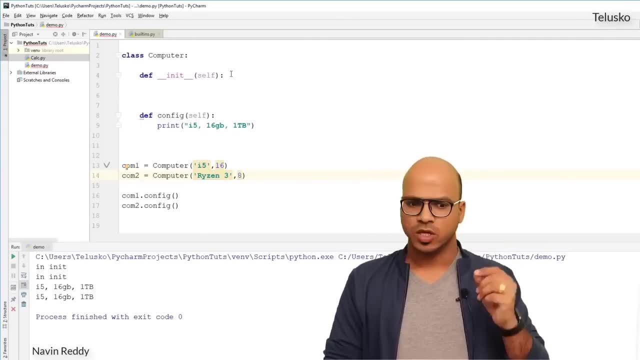 two different CPUs. right, And now how to accept these values. So of course you have to pass these values here, right? So you have to say self comma. you have to pass two values. You have to accept these two values. So you have to say CPU RAM. okay, That's how you accept it Now. 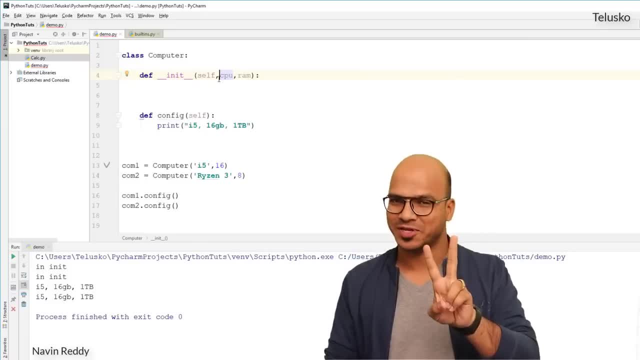 I know your question. Your question is: we are passing two parameters, right? Or we are passing two arguments: One is CPU and second is RAM, and we are accepting the arguments here. So the thing is, you are actually passing three arguments here. Remember we are also passing comp1.. The moment. 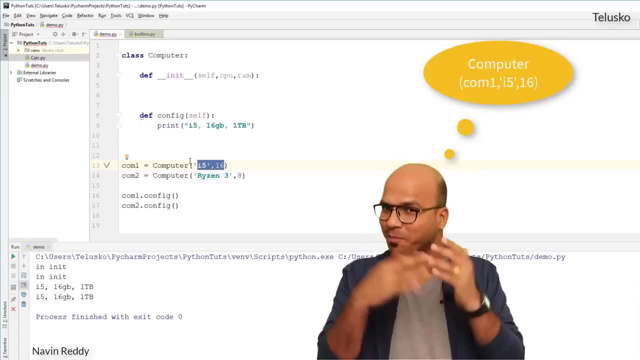 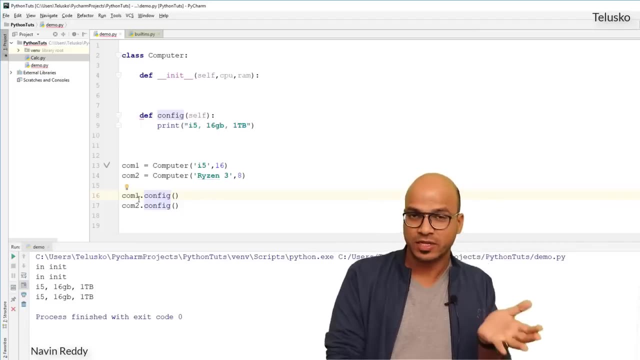 you say computer in the bracket, you are passing that comp1 by default. The same thing happened with config right. When we call config, we are not passing self or the object itself, but it gets passed automatically. The same way when you say computer, by passing two parameters, you're. 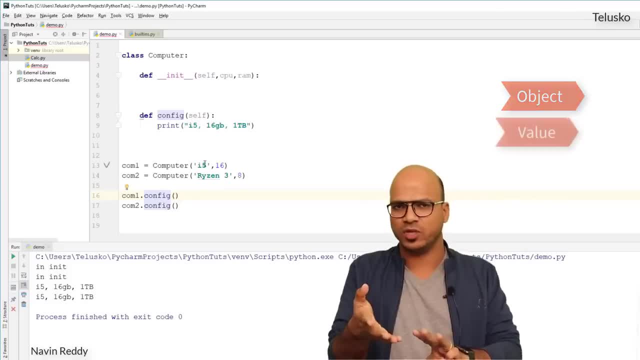 actually passing three. The first one is the object itself, the second one the value, the first value here, and then RAM. Okay, that makes sense, but will it work? So the thing is, every object need to have a value, because this is just an argument now. So CPU and RAM is just an argument, If you want it to. 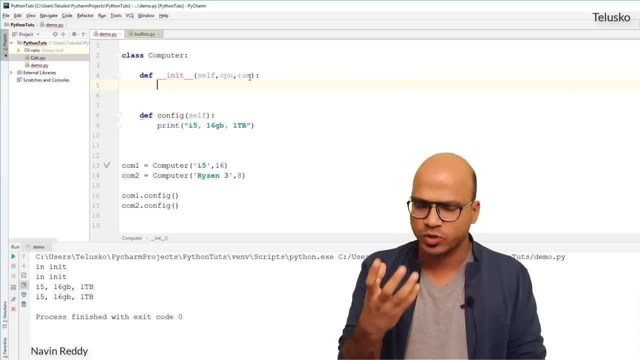 be a part of your object. you need to say because, see, we have to assign this value to our object right, And the object here is self right. So you have to say self dot, That's right, right. So 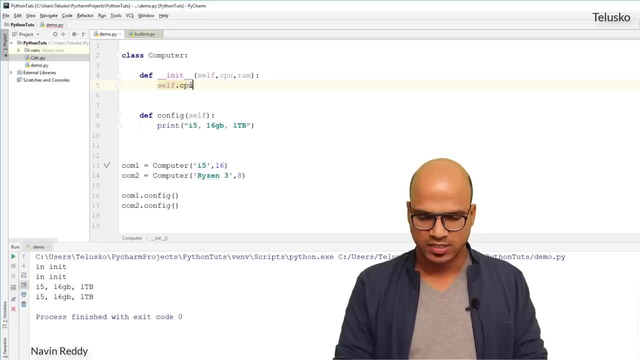 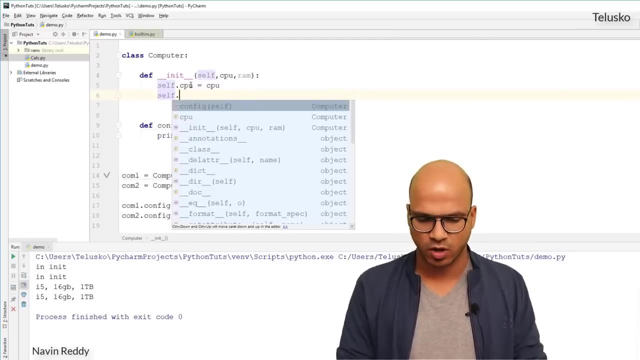 this comp1,. this is our object, right? So we have to say self dot CPU is equal to CPU. Again, there's no compulsion that you should be having same name. You can have a different name, That's fine. So you will say self dot RAM is equal to RAM. So whatever value you are passing, 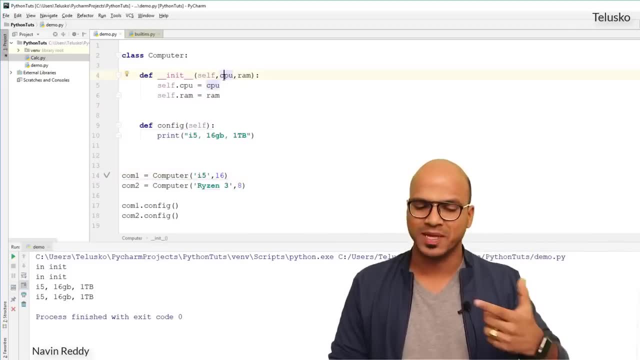 here, which is i5, goes to the CPU As an argument. it will be assigned to the object which is self. So the self you can imagine now. So in the back end you can see we have two objects here. So 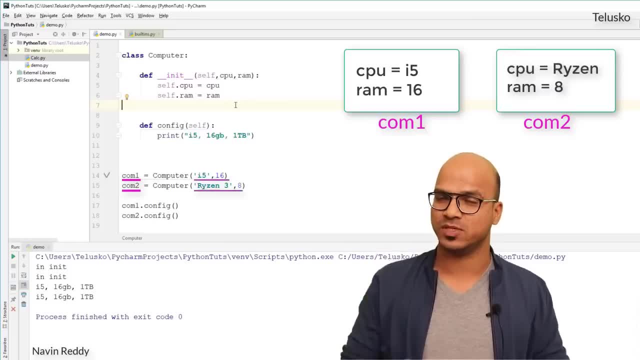 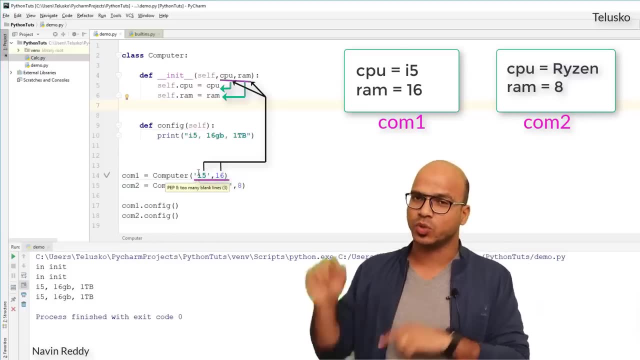 in total, we got two objects. Each object will have its own variables, okay, It will have its own CPU, It will have its own RAM and then whatever value you pass in the arguments, it will be assigned to those objects. okay, So we have two objects, two different values. 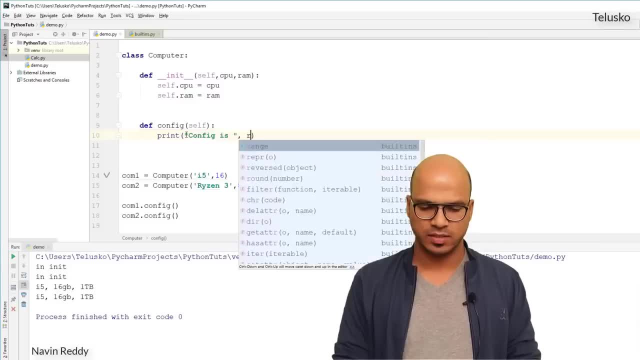 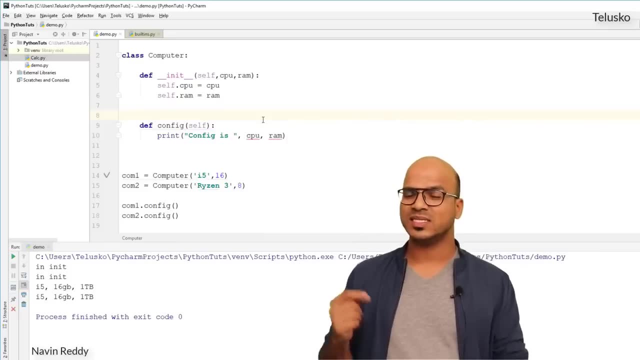 And now in the config, instead of printing this stuff, I will say CPU comma RAM. That's what we do. Oh, we got an error. What's wrong here? So the thing is, this CPU is not a local variable right. The CPU belongs to an object. And how do we refer to object? It's. 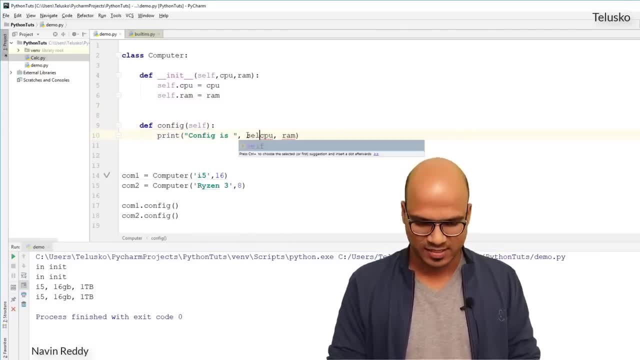 very simple. You have to use self right. That's why you are passing it. So you have to say self dot CPU and here as well, you have to say self dot RAM. And that's the idea behind passing this self right. We are passing self so that you can use it to fetch the values, So you can. 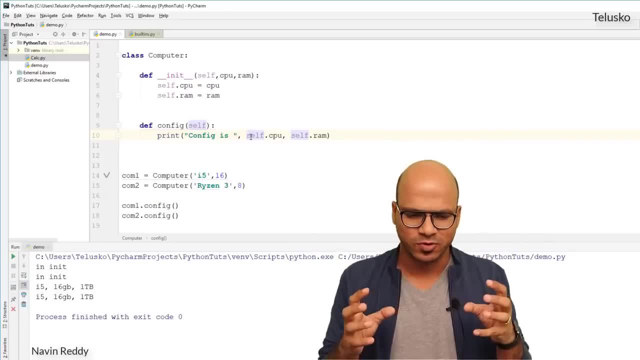 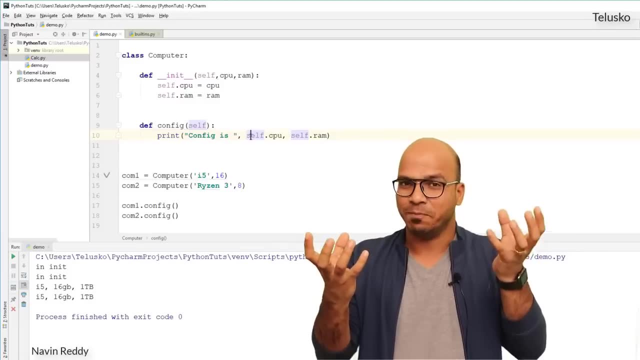 imagine your methods and your data works together And we have a name for this concept. Again, name later. It's a surprise, But we are binding our data with every method, So one object will have its own methods and its own variables. right, So they are working together. And now let's run. 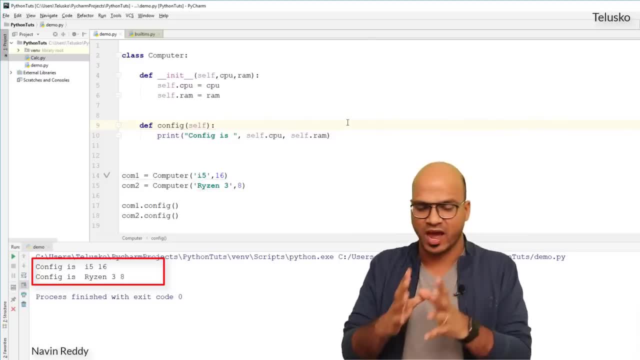 this code and let's see what happens. So the moment you run this code, you can see it says config is i5 16 and config is raisin 3, 8.. So that's the idea. That's how you create a variable. 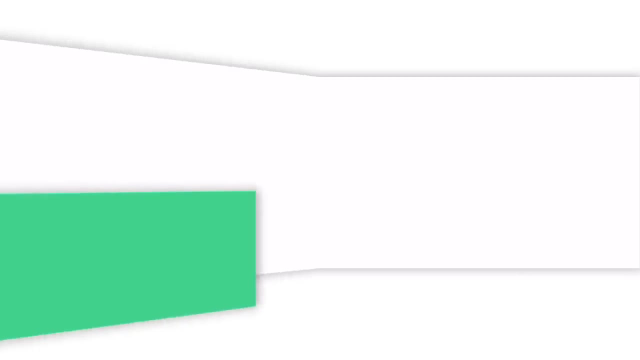 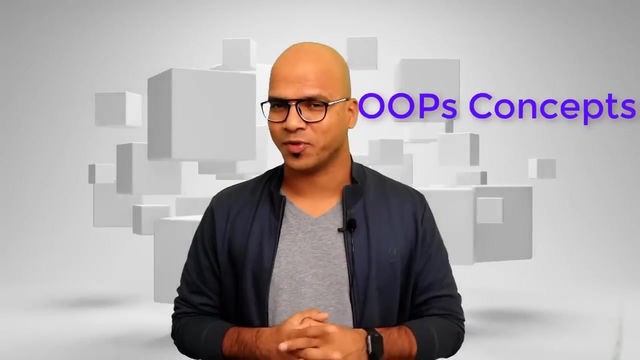 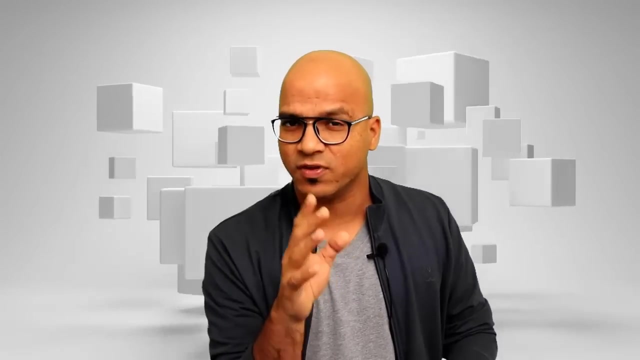 So every object will have its own values. That's amazing. In the last video we have talked about oops concept, right. We have talked about objects, We have talked about classes And then somewhere we have talked about init, right. In this video we'll focus on two concepts. One is constructor and self. But hold. 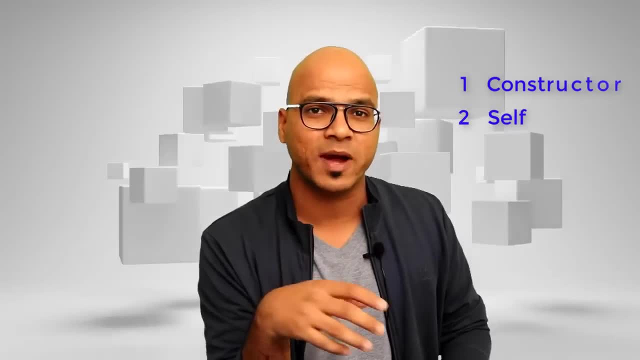 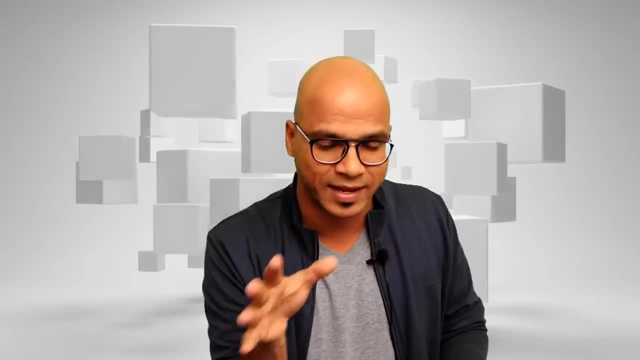 on. We have seen self before, right, But let's try to expand more of it, okay, Because self is something which is very easy to understand. At the same time, it is a bit confusing, okay, So let's talk about that. And then we also talk about constructor. Now, in the last video. 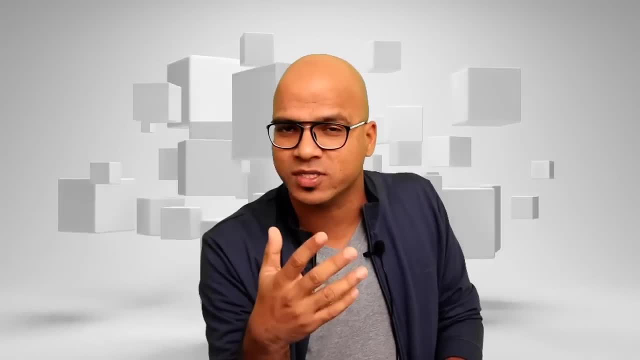 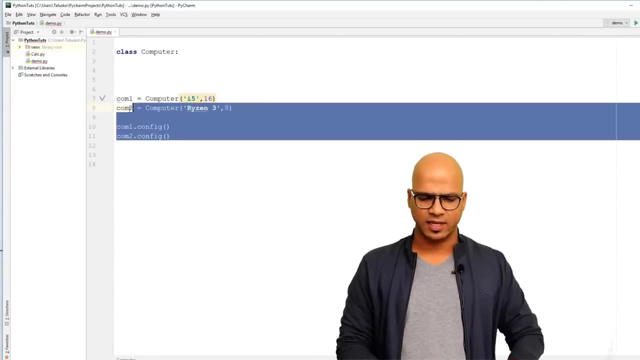 we have talked about init right Now. init is actually a constructor. But why this constructor? We'll see that here And why this is so important. So what we'll do is: let's remove this thing and let's see a computer class again. Let's go back to computer class. So this is a 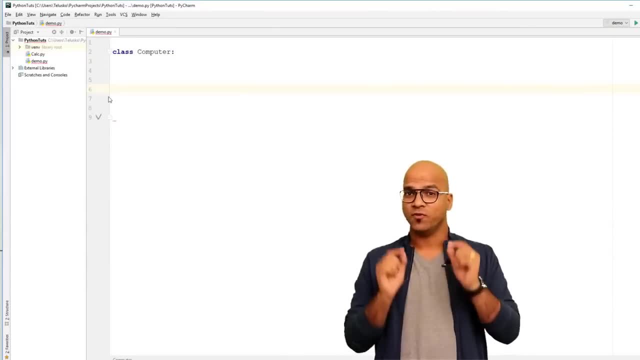 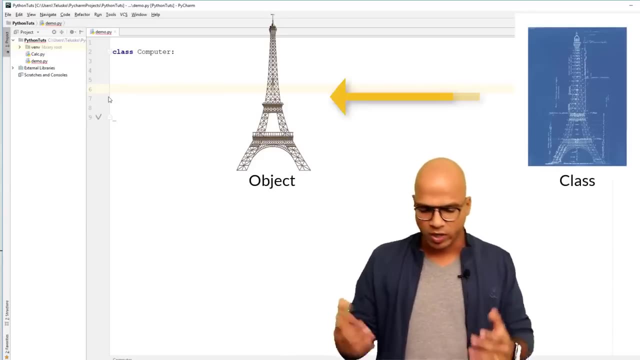 class right, And of course, every class will have an object right. As we mentioned, we have a concept of a design right. So this computer class is a design and then we need to create an object of it. So what I will do is I will say: see, what is the concept of a design right? So 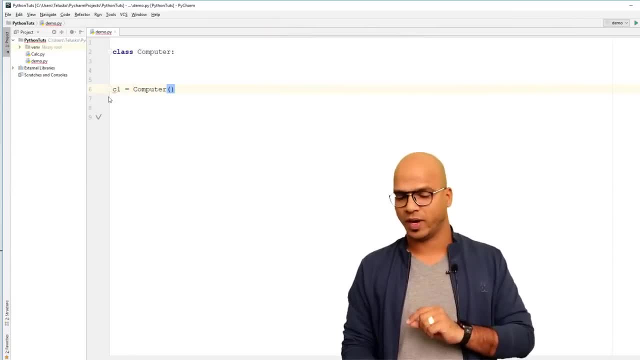 C1 is equal to computer. Now, this computer here is an object, right? I mean this C1 is an object, or you can say C1 is referring to the object. So what happens, you know in your system. 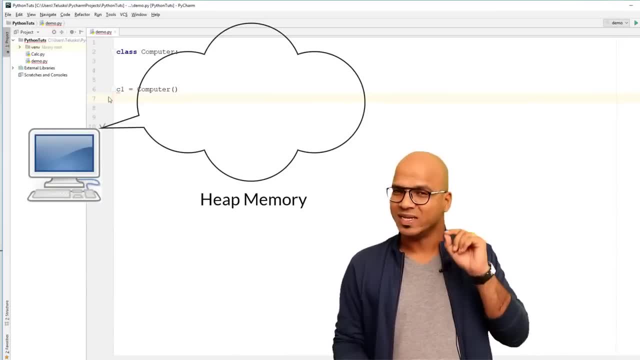 we have a special memory called as heap memory. Now, inside this heap memory, you will get all the objects right. Example: the moment you say you want an object. Now, if you remember, we have talked about integers, string. everything is object in Python right Now, in this scenario, 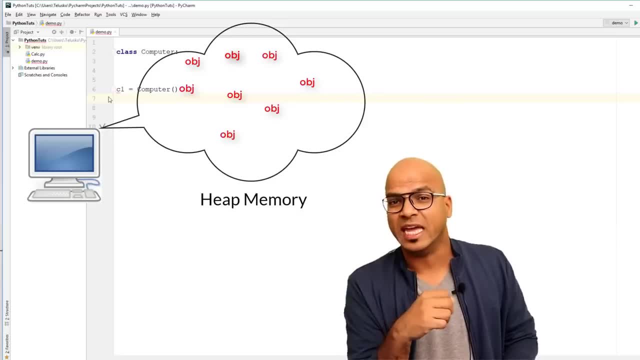 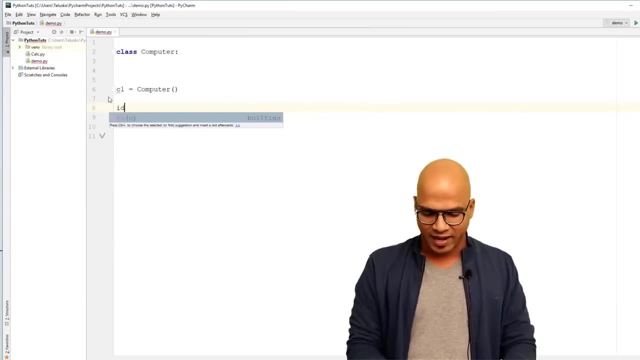 here. this object will take some space in your heap memory. Now, every space will have some address, right? We have talked about ID function, remember? So we can use an ID function here and we can print the value of C1.. So we can print the address. 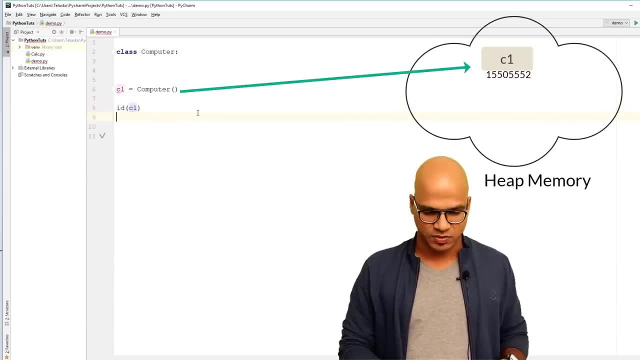 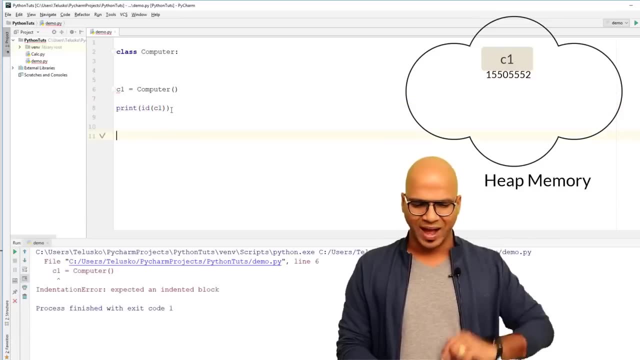 So of course, this object is created somewhere and we need to print the address as well, And the way you can print the address is by saying print. I want to print the address of C1.. Let's do that. Oh, we are getting an error Now. if you remember, we have talked about this stuff, So 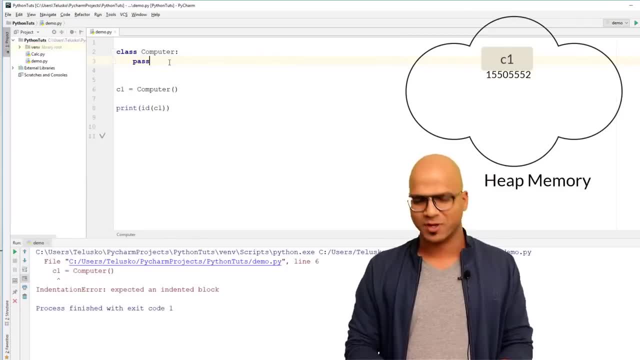 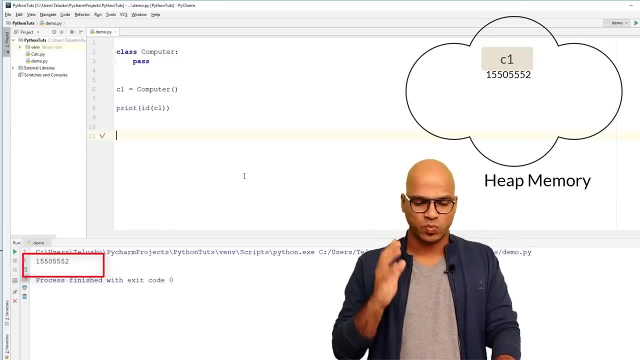 I'm keeping this class empty, right? We cannot do that, So let's write pass, because I'm not mentioning anything in the class here. So let's write pass. Let's run this code now And you can see. we got the output as 155, with the number right. Now. this is an address. 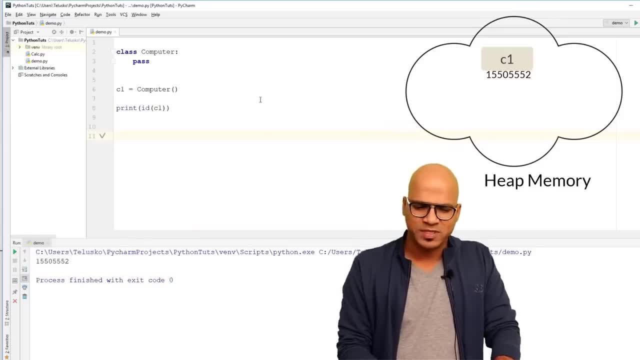 okay, So this is the address of that memory. Now what happens if I create another object? Let's say, if I say C2, equal to computer. now we are creating another object, right? So in total we got two objects. So will it take different space or will it be accommodated in the same? 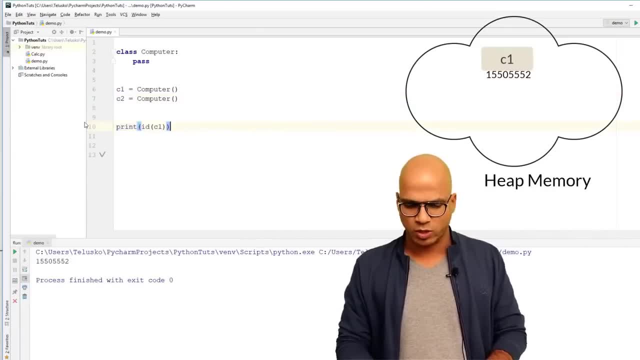 place. Of course, we have talked about this before when we talked about integers allocation. If I run this code, you can see we got different addresses And again, every time you run this code, you will get different address, right? 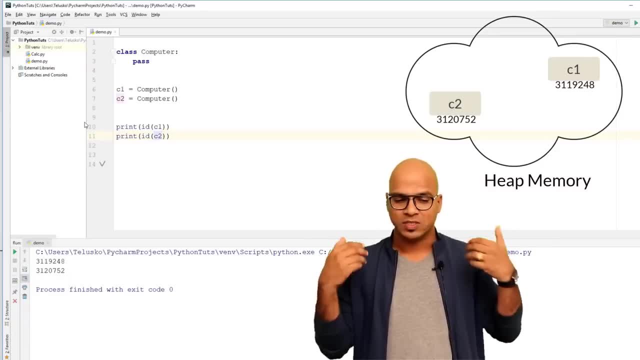 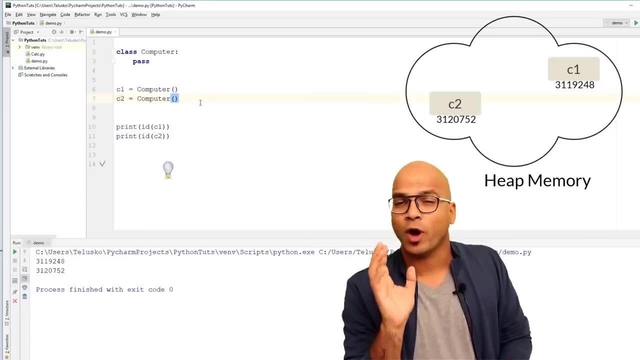 Because every time you run this code, it will create a new object for you. So this time we got two new objects. Now, if I run this again, we will get two different objects, not the same object again. right, Because this is new execution. So point to remember is: every time you create the 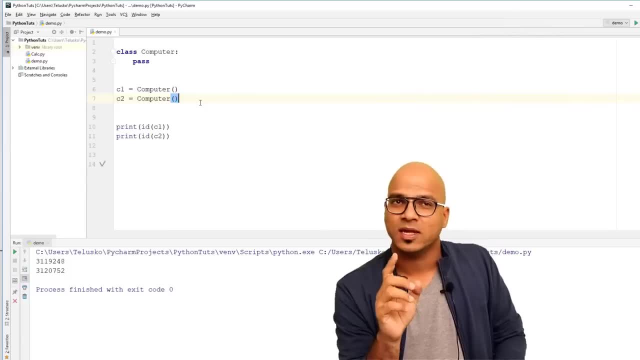 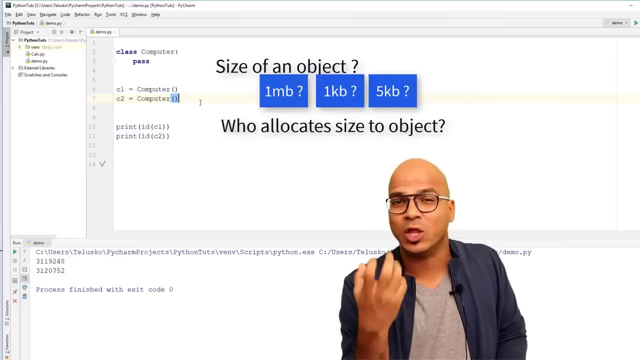 object. it will take two different spaces. Now question arise how much space it will take. Maybe 1 MB, maybe 1 KB, maybe 5 KB. So who will decide and who will allocate the memory? Now the size of the object is depend upon number of variables we have, or the attributes, if you. 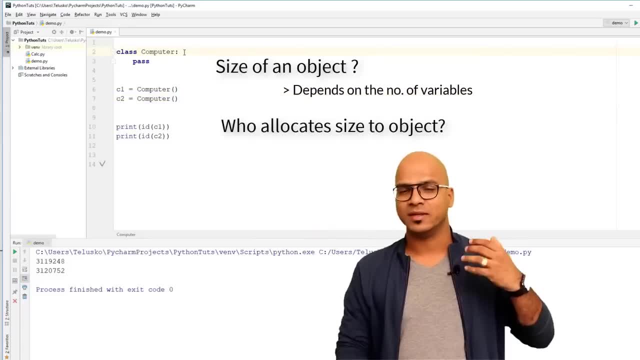 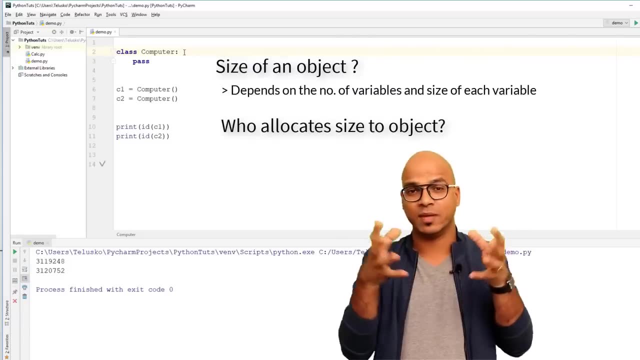 remember, If this class has five variables of different type, it depend upon how much data you pass. it will change the size of it. okay, So the size of the object is depend upon the size of the variables and number of variables. But who is responsible to assign that memory or who is? 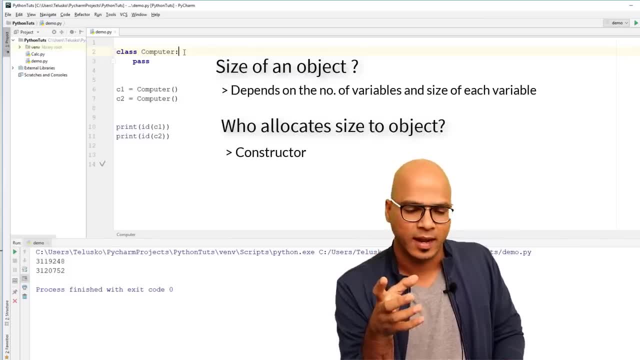 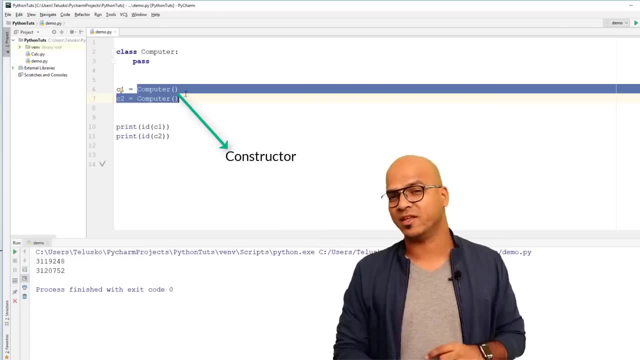 responsible to calculate the memory, And that's your constructor. Now this thing here which is computer brackets, this is your constructor, right? So whenever you write a constructor, it will call you. Of course, you don't have to call it explicitly, it will be called internally. Now, 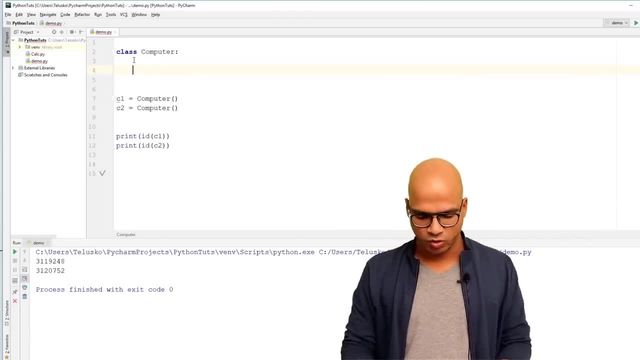 let me define some variables here. How do we create variables? right? So how do we define a variable for the object? Now, in this case, if you want to define a variable, we have one choice which you can define: a function which is init. Again, we have seen that. So this is the init. 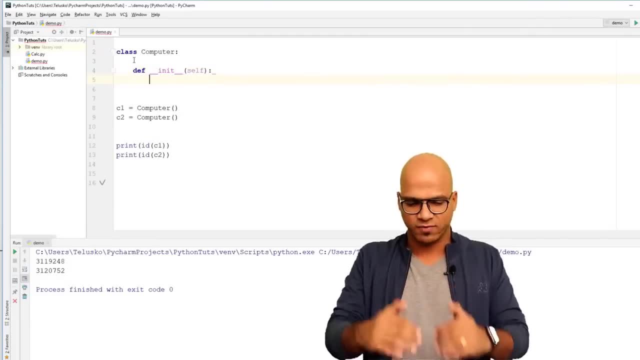 function right Now. it uses self, but as of now, we'll not talk about self. we'll continue here And I will use two variables Again. we have talked about this, but let me just do it once again. 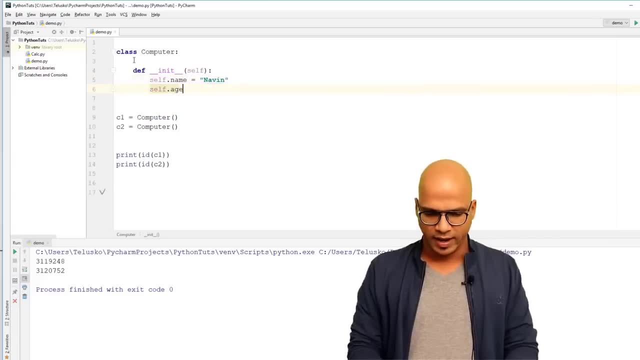 So let's say we have two variables, So we have two variables. So we have two variables and we have two attributes. One is name- I will say name is Naveen- and age, So we'll say age is. 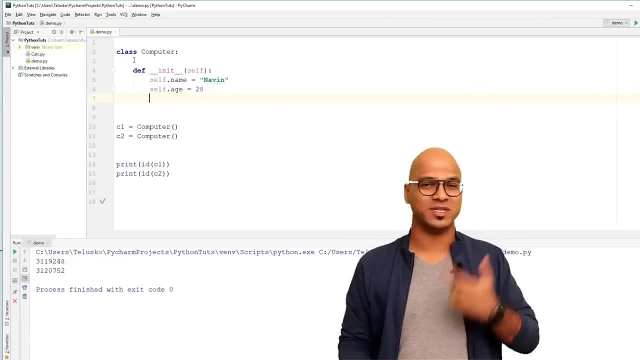 equal to 28.. So we got two things: We got name and we got age. Now both the object will have the same values, right? So you can imagine we have two objects and both the object have the same value. If I want to change it, if I want to change the value of one object, the way you can do that, 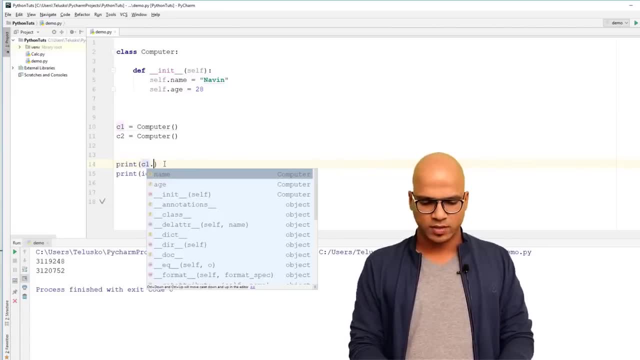 is in fact, instead of printing IDs. I want to change it now because of course, the IDs will name of C1, and I want to print the name of C2 as well. So what will happen? Will it print the? 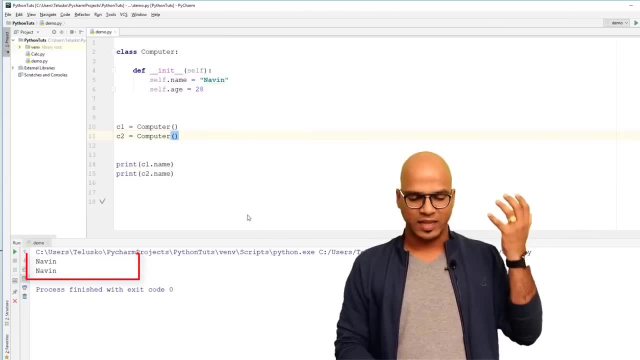 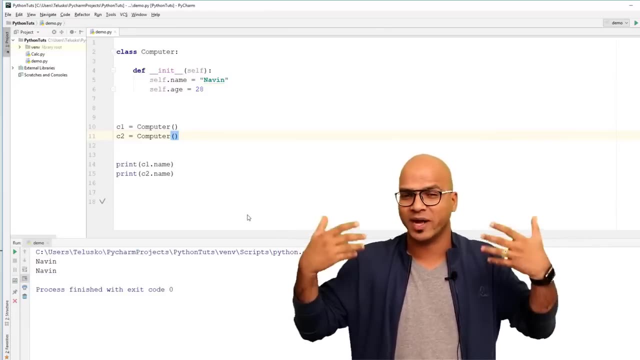 same data or different data? That's a question. So let's run this code and you can see they are printing Naveen. Of course, right, Because the moment you create the object, both will have the same value, because that is what, by default, you're getting If you want to assign your own. 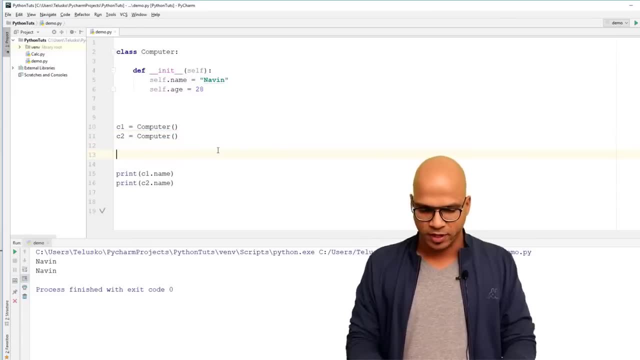 values. you have two choices here. What we can do is, before printing it, we can change the value for C1.. We can say C1.name is equal to Rashi. So we are changing the name right. And now, if I run, this code, you can see that it will print the name of the object. And now, if I run this code, you can see that it will print the name of the object. And now, if I run this code, you can see that. 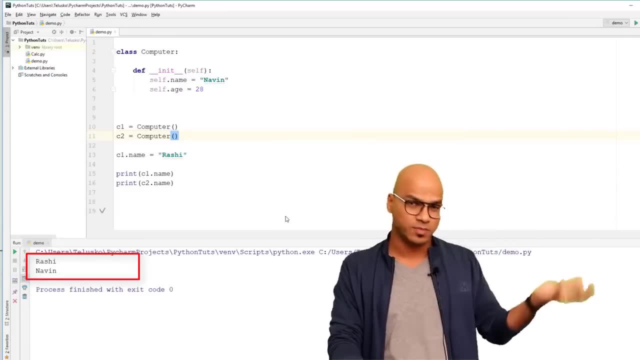 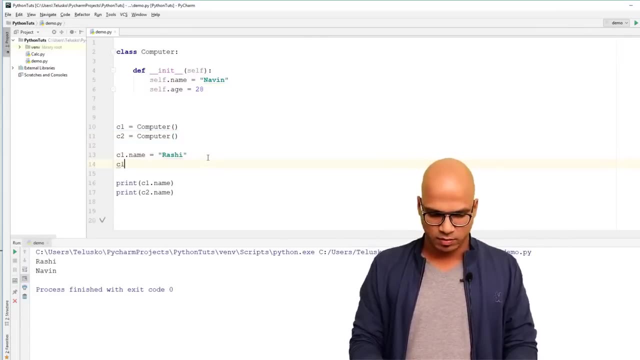 you can see we got Rashi and we got Naveen. So of course C1 is a different object, C2 is a different object and we got different names. So that perfectly makes sense. We can change the age of C1. We can say C1.age is less than 12. We got Rashi with age 12. And of course 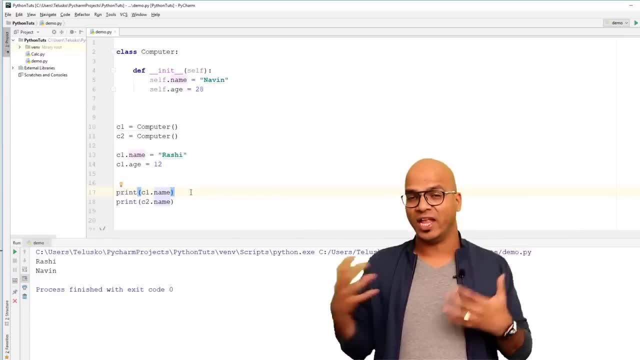 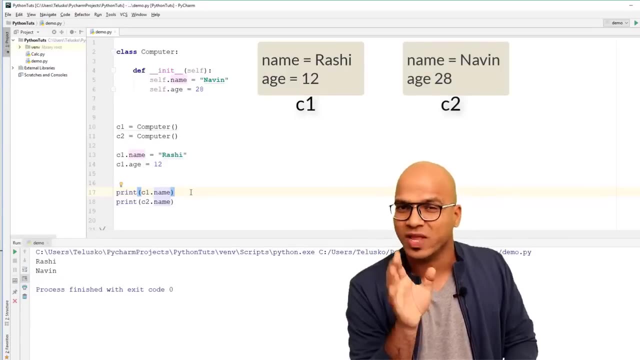 we are not printing age here, but we can do that, So we can change the value of one object from different objects, right, Of course there are two different entities. So remember this: We got two different objects and both the objects will have different variables. 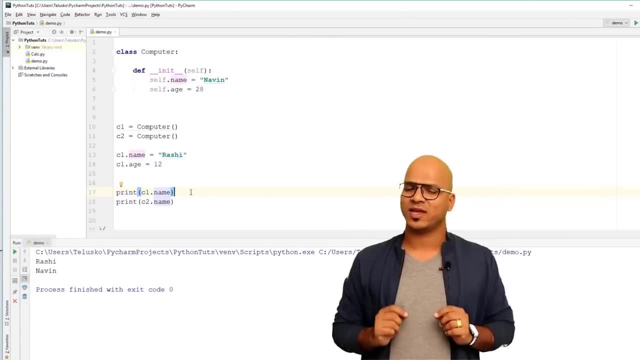 okay, You can assign the values there. you can change it your wish. Now question arise: which one of the objects can you print And what will happen if I print the value of this object? Now question arise: which one of the objects can you print? the value of this object? 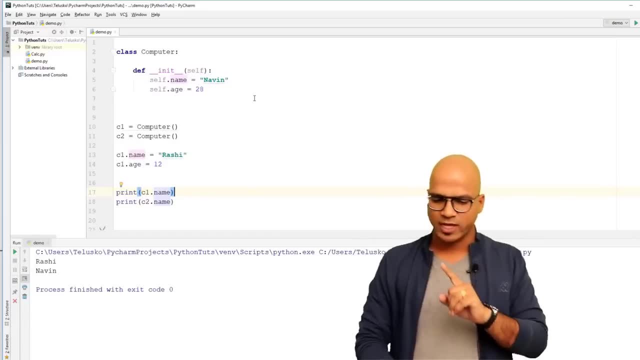 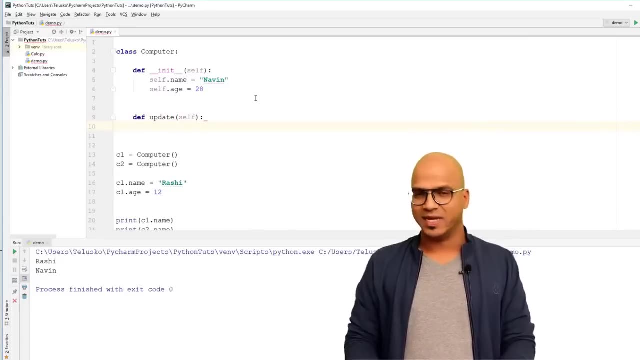 why do we need this self? so what i will do is just to explain that. let me take one more method here. we'll say def, update, okay, so i'm changing the value of something. and the moment i say update, i want to change age. i will assign new age and we'll say: age is necessary, so we are changing. 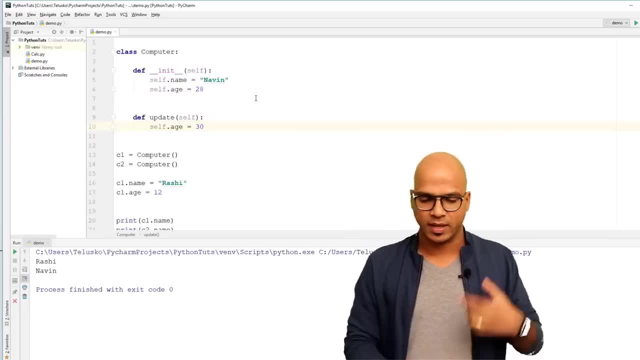 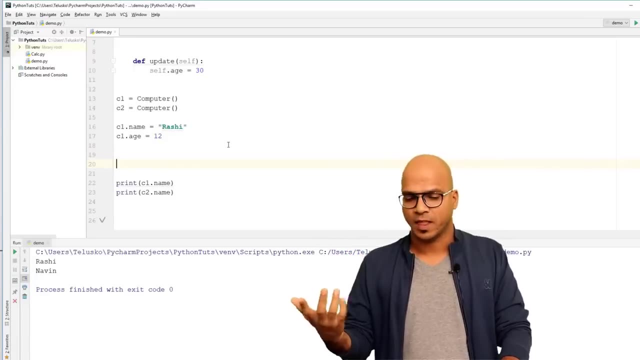 the age now, right. so we got a method which will change the age totally. now i want to call update. now, how do you call update? with the help of class name or with the help of object name? let's try with objects. i will say c1, dot, update. now. see, we have two different objects, right. so what this? 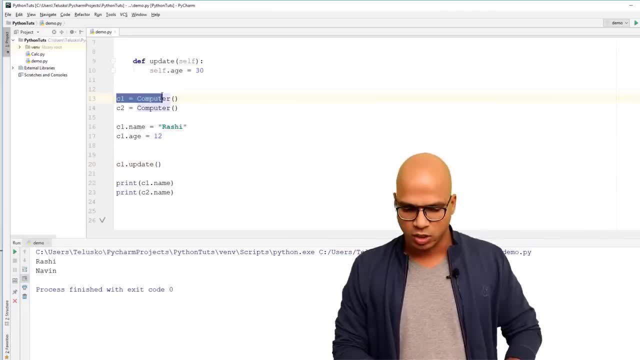 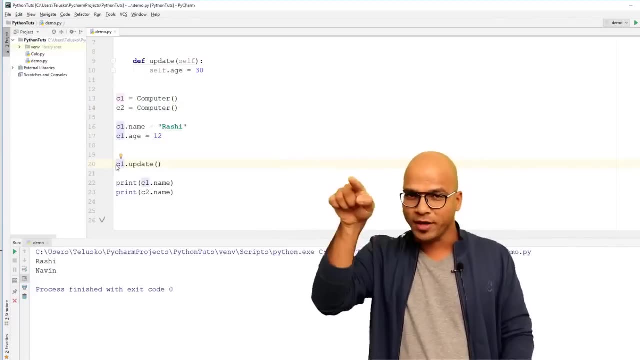 program execution: right, so execution will start from here. uh, you got the object. you got the object, you are changing the names and everything is fine. the moment you say c1, dot, update, your pointer, which is your focus, will move towards this update function of update method. so it is executing it. 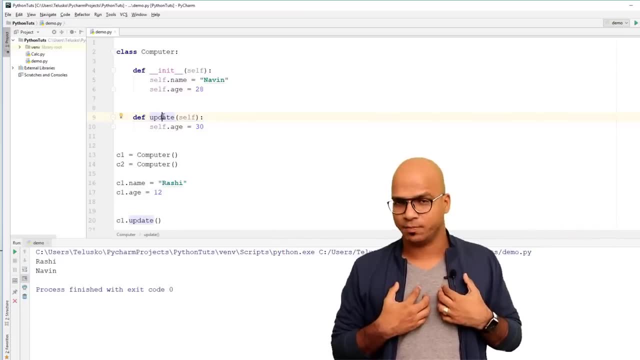 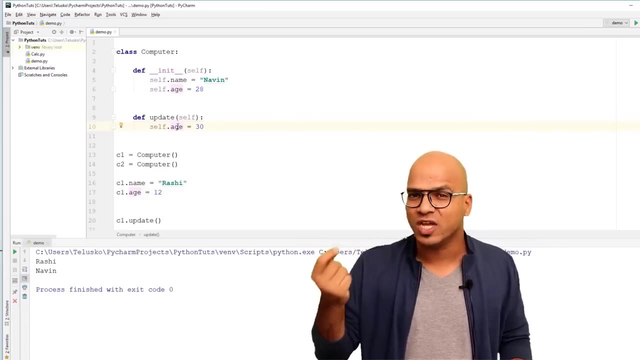 right. update will say: okay, i'm getting called, i belong to a class computer, my job is to do something, my job is to change the value of age. but hold on, we got two objects which value you want to change? right, because we are calling update and we are not. 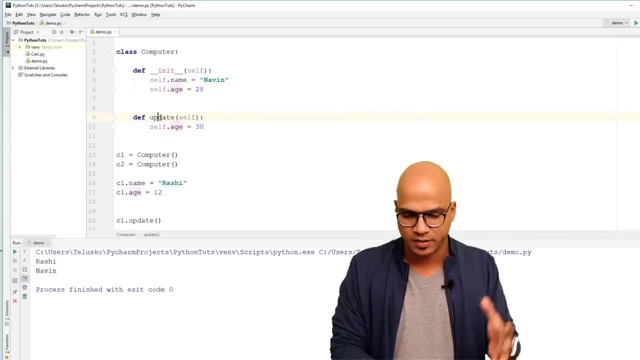 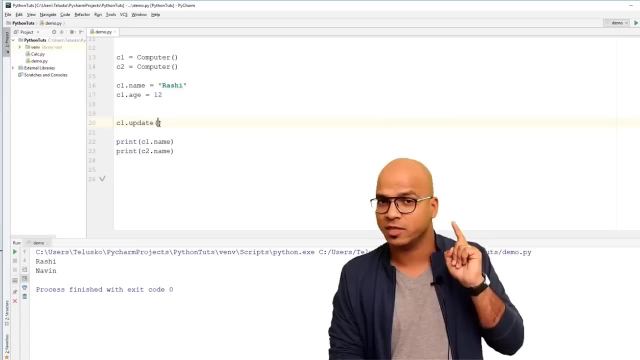 mentioning which object i'm talking about. because when you call this update, we have not mentioned is it c1 or c2. we have mentioned that by calling it. so we are saying c1, dot, update, but we are not passing anything in the bracket. so when you are calling it, when you are calling update, how your 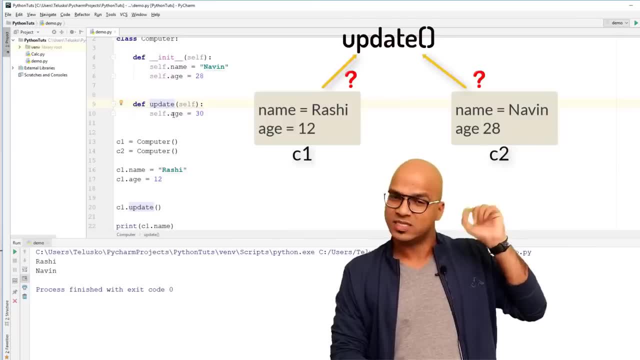 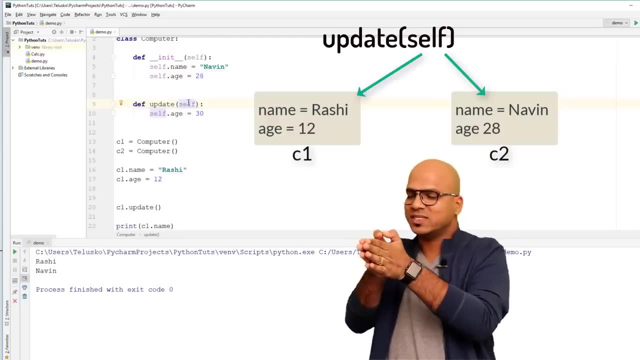 pointer will know which object i'm talking about. is it the c1 age or is it the c2 age? and that's where you need to use self. so this self is a pointer, or you can say self is directing to c1 or c2. so we have two objects. this self will direct either on. 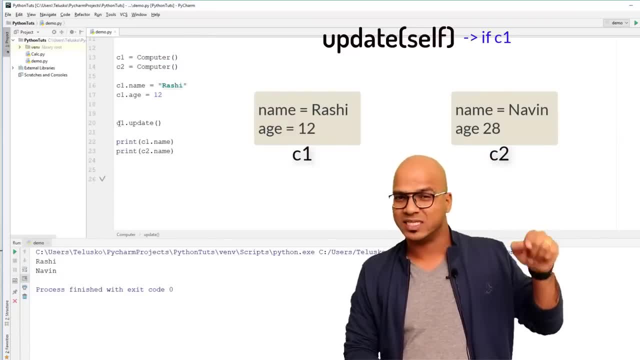 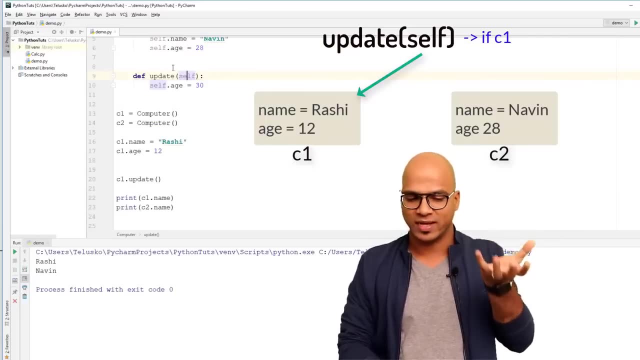 c1 or c2 based on what you're calling. so if you're saying c1, dot update, then in the bracket it is passing c1, so self will be assigned to c1, okay. so that's the importance of that self. it is very important because it is referring to the object. if you have 10 objects and if you want to refer, 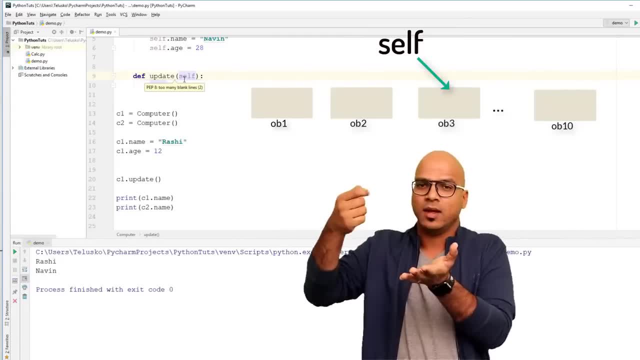 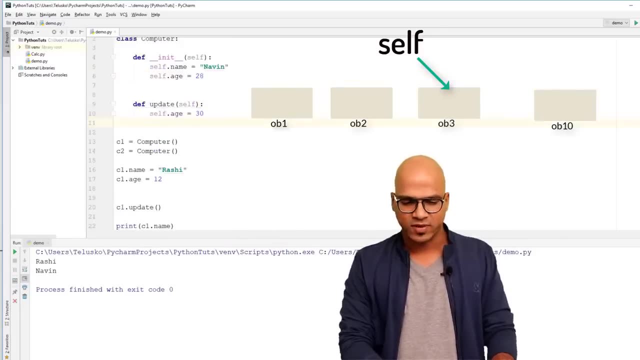 to one object, you can use self. so it is the current instance. you can say, even if you have 10 objects at one point you're working with the one object that is self. i hope that makes sense. so that is self right. so we have talked about constructor and self here. 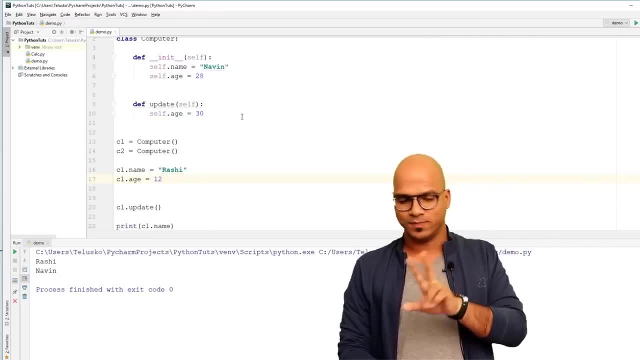 let me show you one more thing. what if i want to compare two objects here? okay, so i want to compare. let's say we have c1, c2 and both have same names. right, so they have same name and they have same age. but let's say i want to compare their age. so i will say if c1 is equal to equal to c2. 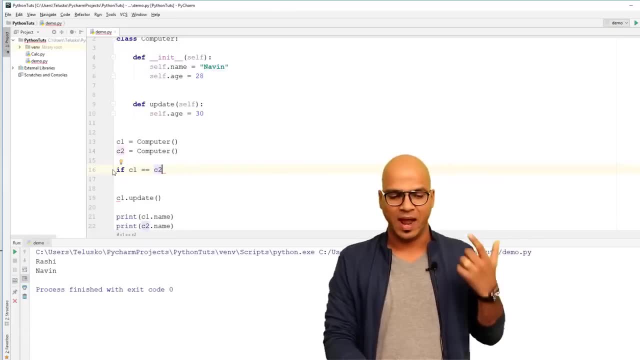 so i want to compare two people based on their age. if their age is same, i want to print their same. so i will say c1 is equal to equal to c2. print they are the same. so let's do that. i want to check. if both the objects are same, then i will print: they are same. 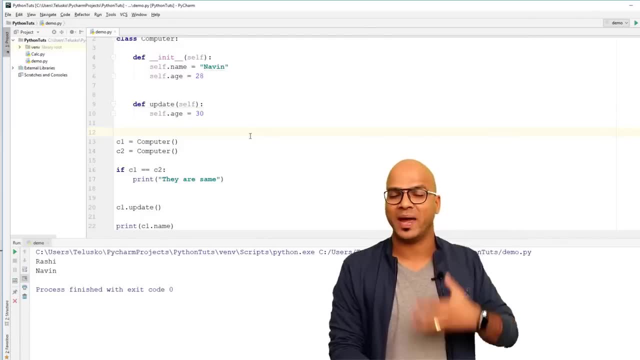 but then i don't want to compare the object address, right, i want to compare their values, i want to compare their age. name doesn't matter if name is different. what is what should be same is age. now, in this case, we cannot simply say c1 equal to c2, because we don't know. 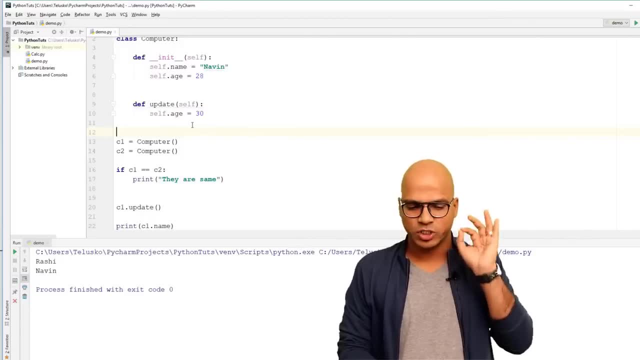 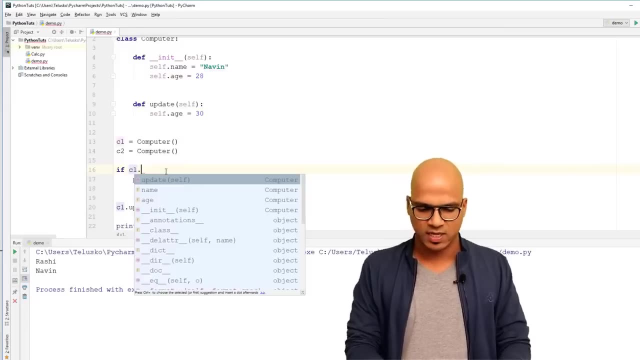 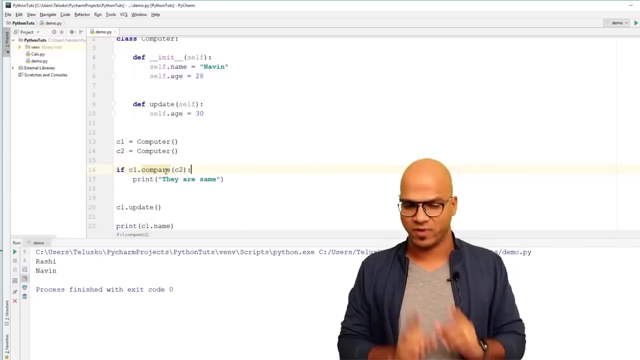 your python don't know how to compare. so in this case what you will do is you will use a separate function to do that. i will say: hey, i want to compare c1 with c2, so i will say c1, compare, and you can pass c2, because we are comparing it right. again, this compare is not a inbuilt function. so if i 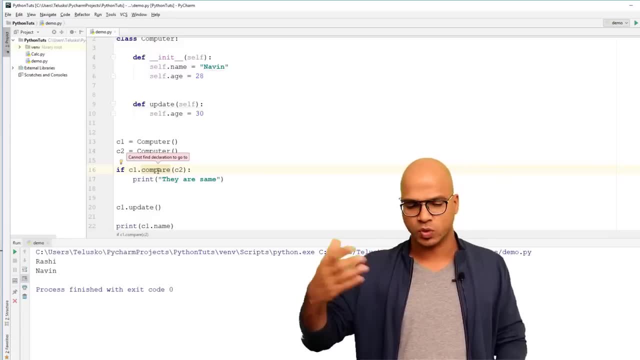 click on this, you can see it says: cannot find declaration to go to something. the thing is, compare is not a inbuilt method we have. so in order to work with compare, you have to define your function, you have to say that compare and in this compare, of course you have to pass. 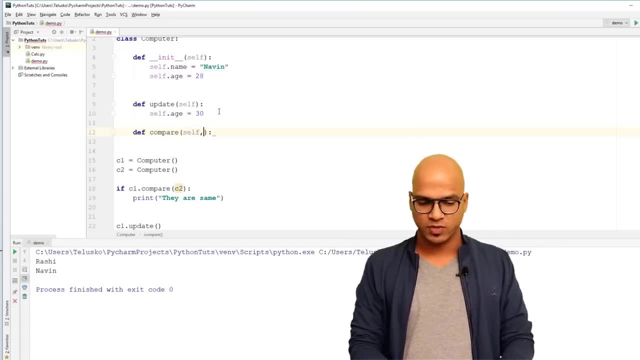 self. and then you have to also pass one more object which is of c2, right? so we are comparing two objects, right? so we have to pass self. so what is self here? so the c1 becomes self and c2 becomes c2. again, you can change in the name, it's your choice, right? 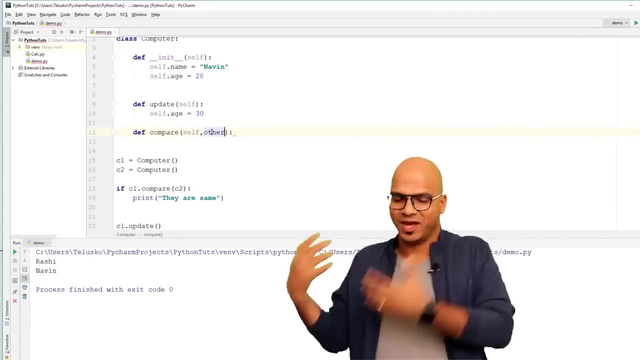 you can say other right, so you are comparing self with other. so c1 becomes self and c2 becomes other. now why c1 becomes self is because c1 is calling it, so c1 is comparing itself with c2. you can reverse it. okay, you can say: c2 dot compare c1. in that case c2 becomes self and c1 becomes other. 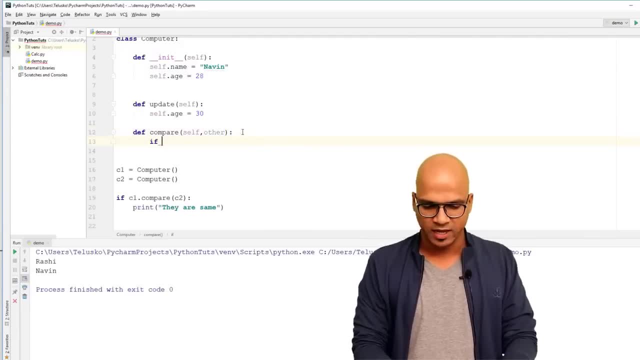 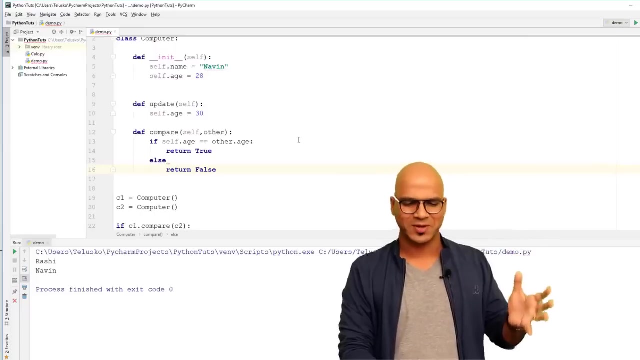 right and now, once you have this self and other, you can compare. if self dot a is equal to equal to other dot h, you will return true, else return false. in fact you could have done that in one line, but just to make it look good, i'm doing this and now you can compare it. 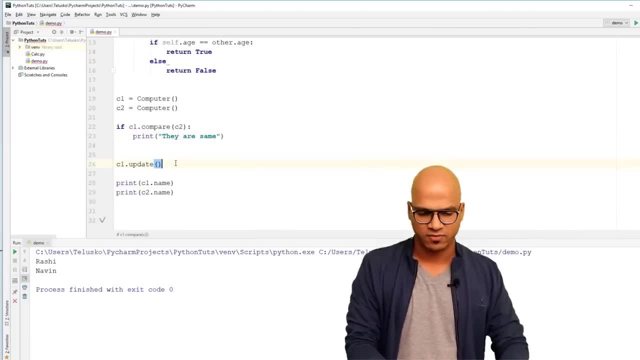 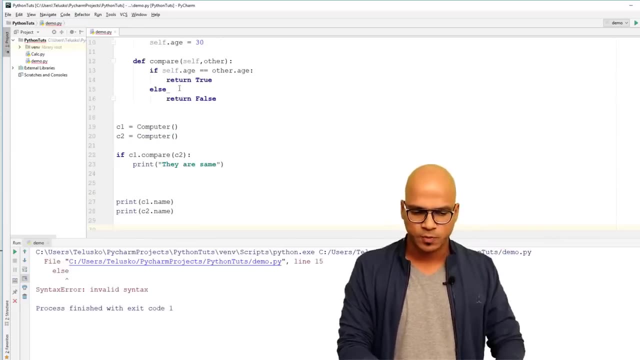 right, so they don't have same age because, uh, we are changing it after update. let's remove the update part here. they'll say they have the same age, right, let's run this demo and you can see. oh, we got an error, we forgot to put a colon there. my bad, let's run this code and so you can see it. 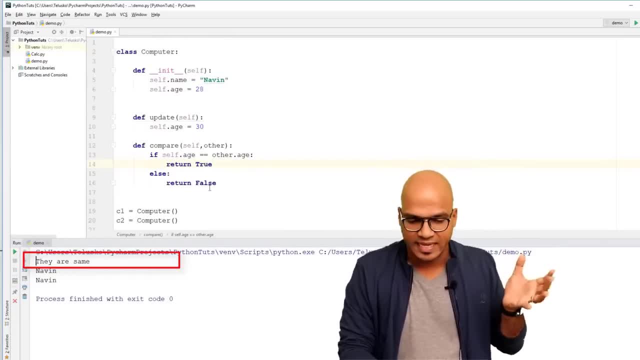 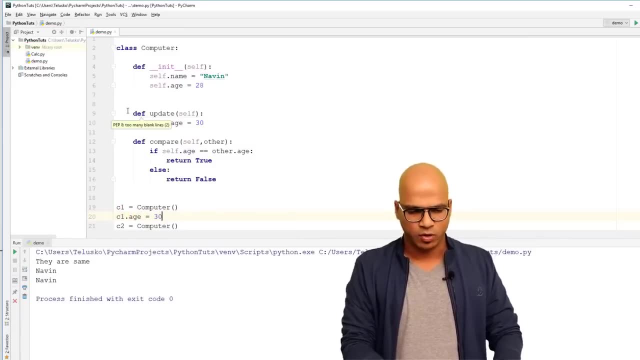 printing. they are same, so they are same right now. what if they have different age? so what i will do is once once, once i got c1, i will change this age of c1. i will say: age of c1 is 30. anyway, we are not. 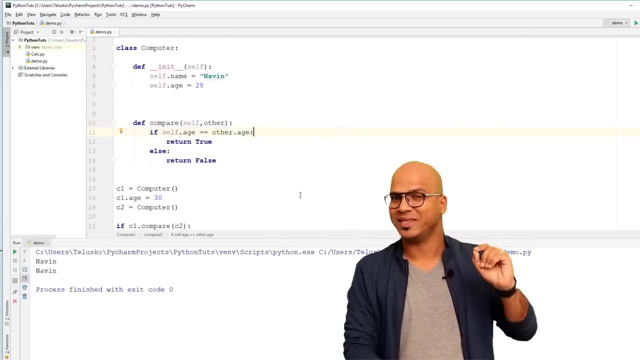 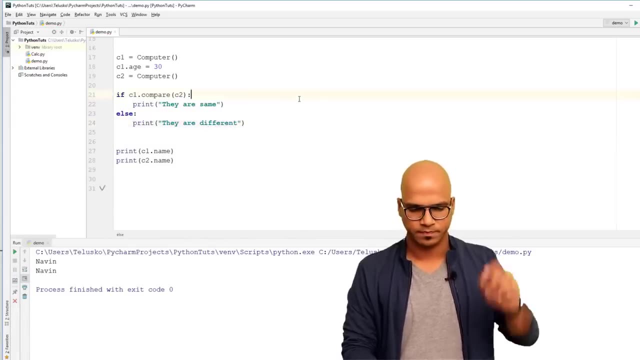 using update here and we can say: run demo and you can see it is not printing. they are same. we should print the else part as well, so that we'll see: is it different? let's print they are different and let's run this code. okay, so that we got they are different. now, since their age is different. 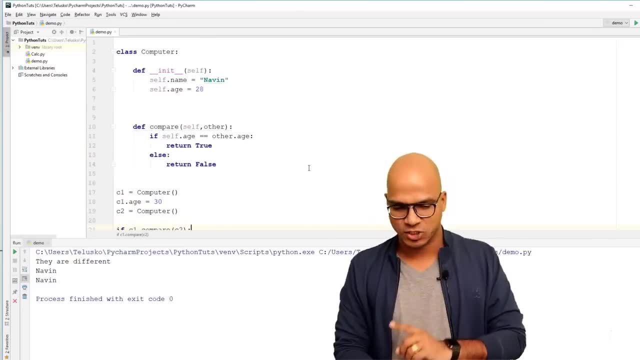 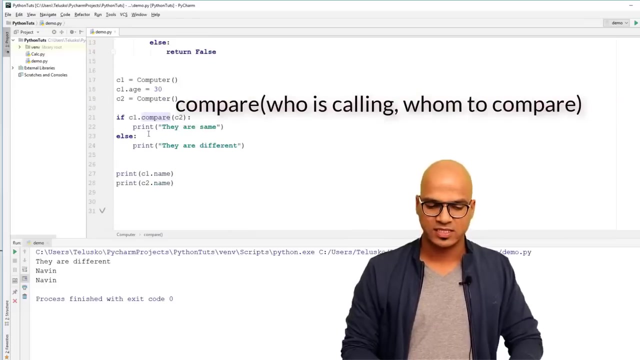 we are getting that different. see, names are same, what is different is age. so we can compare two objects by defining our own function, which is compared in this case, or method in this case. but remember, this thing, compact, takes two parameters: the first one who is calling it, and second one whom to compare right. so here, in this case, we are saying c1, dot, compare. 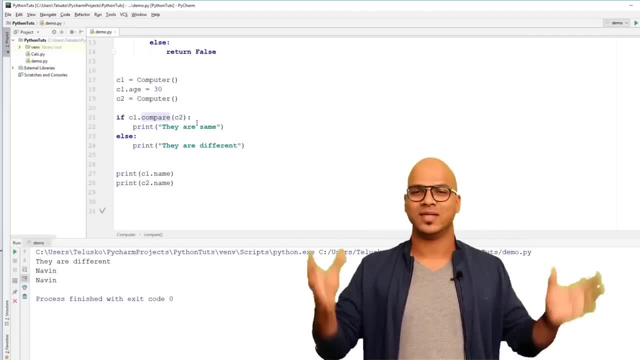 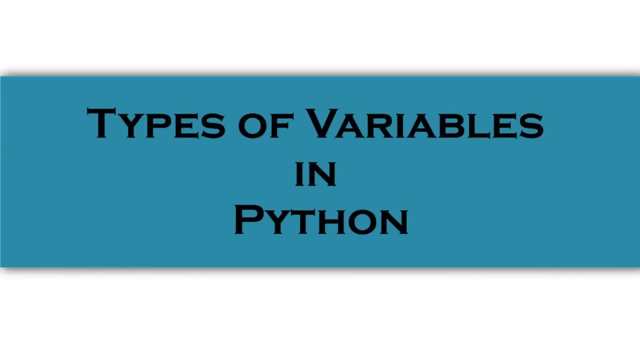 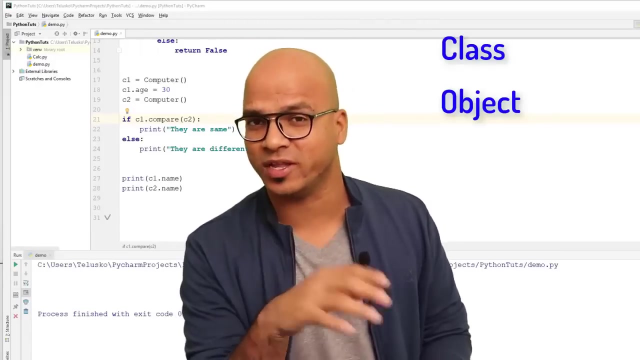 with c2, so c1 becomes self, c2 becomes other. this is very important. i know it is a bit confusing at the start, but the moment you start working on it it becomes very easy. now we know how to work with this, so let's just start with this. we have a class and object right, and we have also seen how can you. 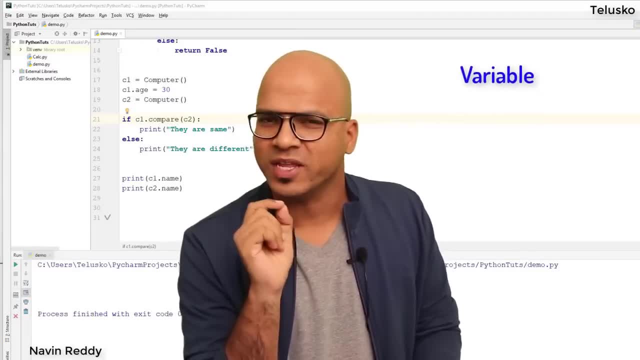 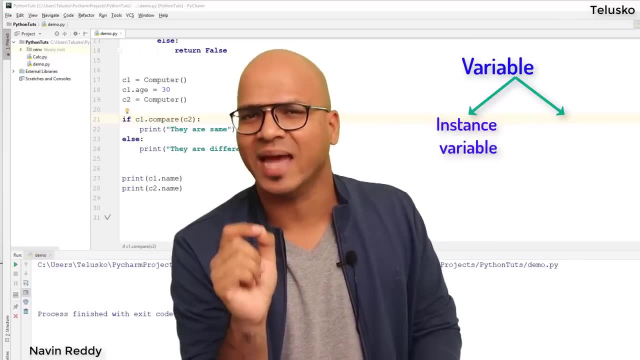 create a variable inside an object. of course, right, every object should know something. but when it comes to variable in oops, we have two different types of variable. the first one is a instance variable and the second one is a class variable, or you can call them as static variables. what is? 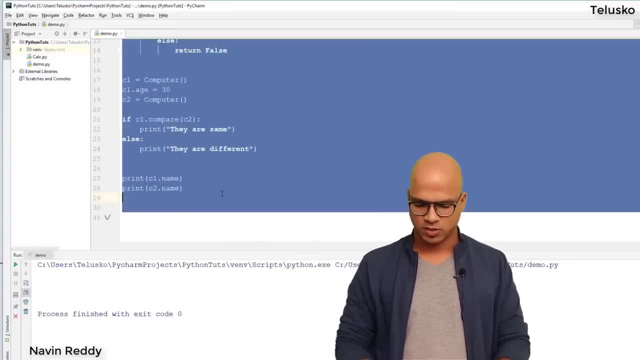 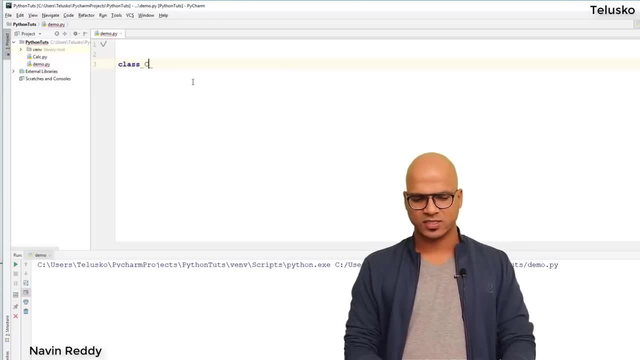 the difference between them. now think about this: let me just remove this code, okay, whatever we have done till now. so let me just clean this up, okay, so we'll start from a plain slate. so here with another very example. let's take a class call us card. okay, we all love cars, right? so let's say: 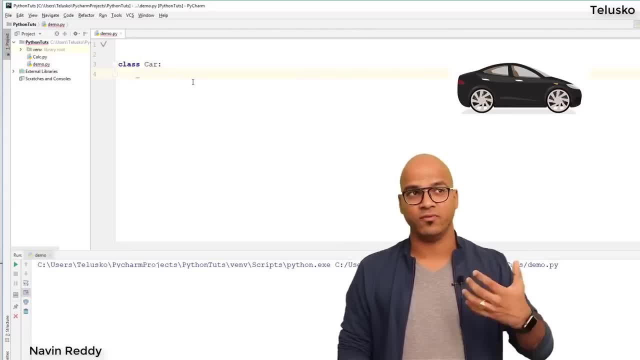 we have a class card and of course, every card will have different variables, right? of course you can mention the company name, you can mention the type of engineer working with and the mileage, what it gives you. so we have different variables, okay. so what i will do is, if i want to use those, 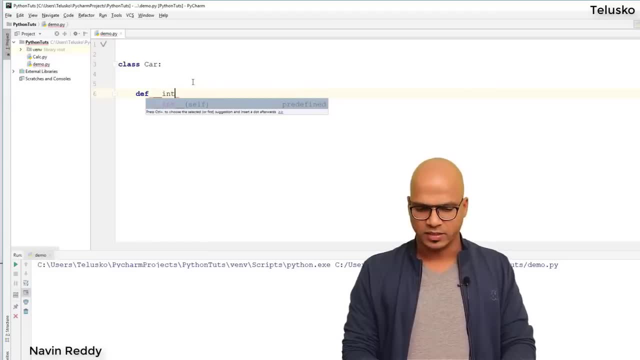 variables. here we need to use a function which is init, so you will say init function and in this you can define those variables right. i can say self dot mileage and i will say mileage is, let's say, 10, and then i will say the company. so company would be, let's say b m w, any random company doesn't. 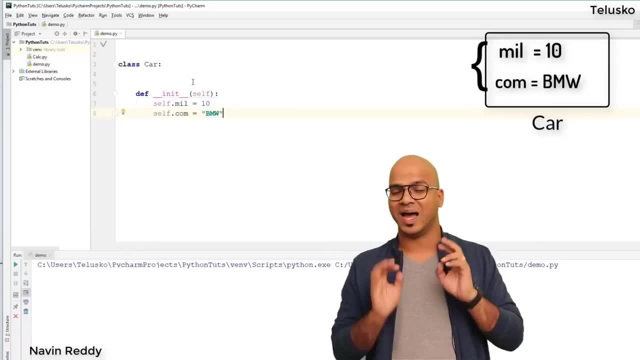 matter. so we have these two values right now. these two variables are called as instance variables. so when you talk about mileage and com, these are instance. now why is our instance? is because as your car changes, as the object changes, this value also change. by default, the value is 10 and 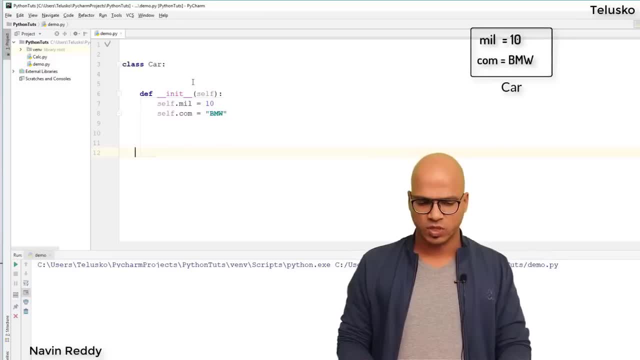 b and w, but you can change it right. example: we have done that before. just to give you a glimpse, i will say: the first one is c1 and this is car. that's my first object. i will go to c2, which is again a car. that is, we got c1, c2. now we got two different objects. 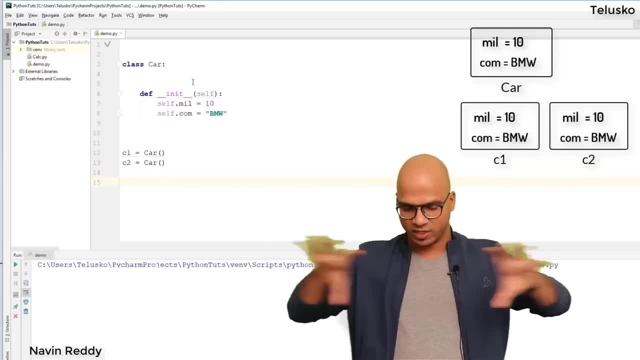 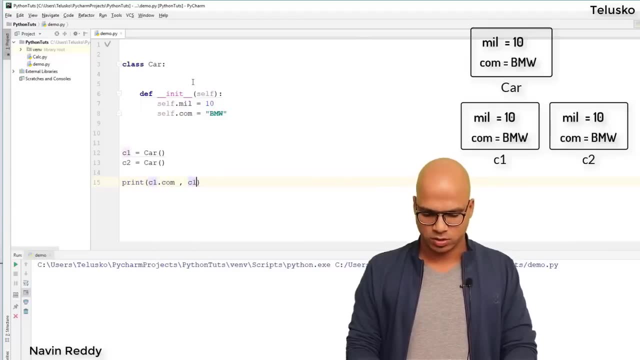 and both the objects will have different variables, right, different area for the variables. and now if i print the value, so i will say c dot com. and i also want to print c1 dot mileage. so i want to print both for the, both the variables. so you can see we got c1 com, c1 mileage. 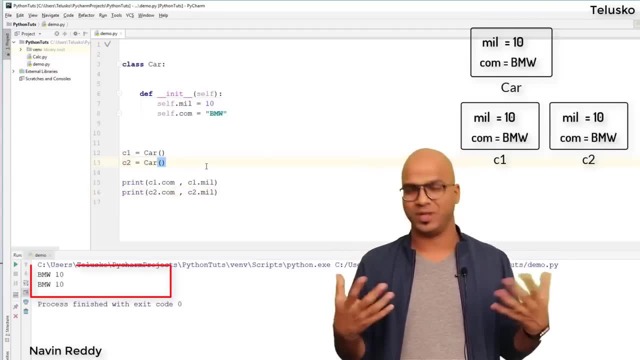 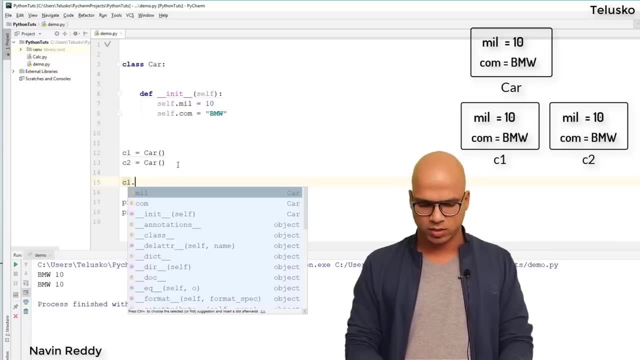 c2, com, c2 mileage, that's perfect. and now, if i run this code, of course it will print same values because they are same. but can we change it? yes, we can. so i will say: if i change for c1, so let's say c1, dot mileage. so let's say c1 mileage changes from 10 to, let's say, 8, this is what happens, you. 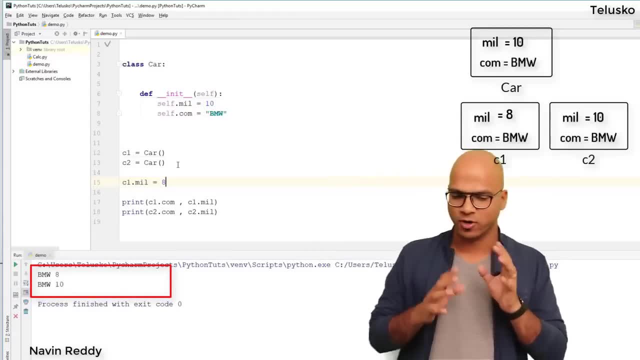 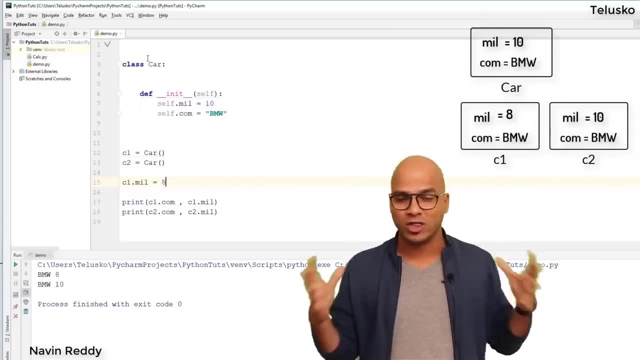 know with some cars. and let's run this code. you can see the value is changing. now. so of course, both the objects are different and they will have different values. but what if i want to create a variable which is common for all the objects? of course, these variables, which are instance variable, 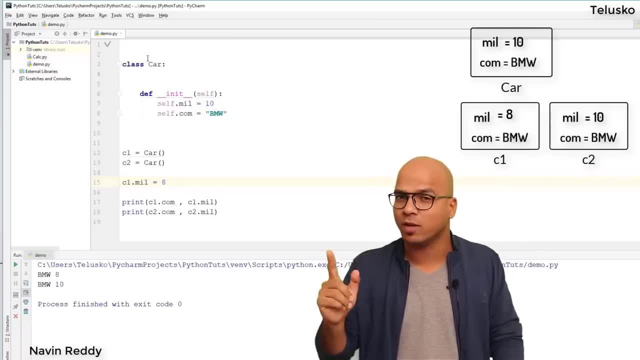 they are different for different objects. right, if you change one object, it will not affect other objects. what if you want to have a variable which will change? it will affect all other objects. example: the number of wheels in a car is four right. by default is four right. but what if in 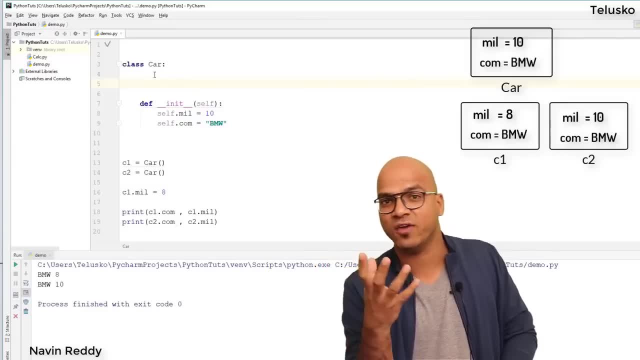 future. we got a new concept and they're saying: hey, now, this time we will have five tires or five wheels. i don't know why we have five years, but let's imagine in this case, what you will do is you will define a variable outside in it. okay, because if you create or if you define the 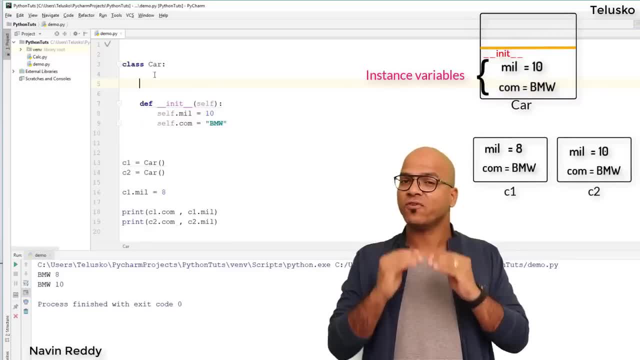 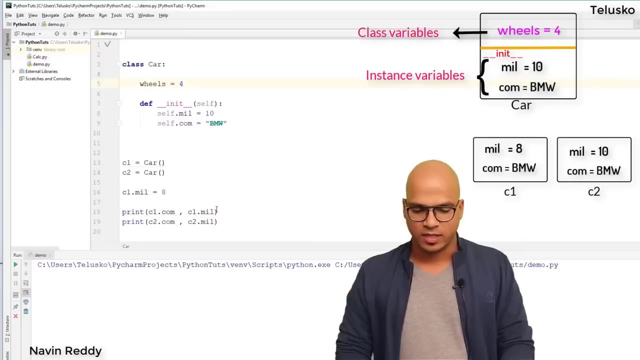 variable inside in it, it becomes an instance variable. if you define a variable outside in it and inside the class, of course, it becomes a class variable. let's say we'll say wheels. so let's say wheels are by default four of course will be four right. and if i print the wheels as well? now how do you print wheels? the way you can print is very 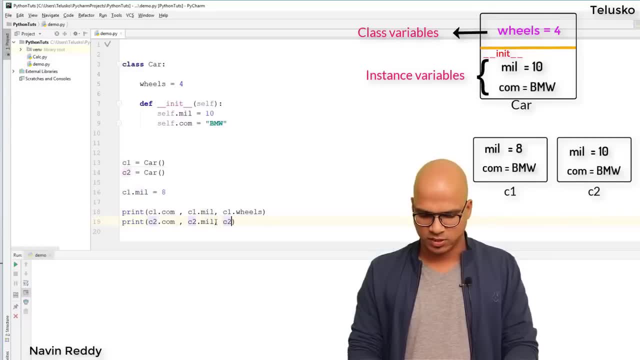 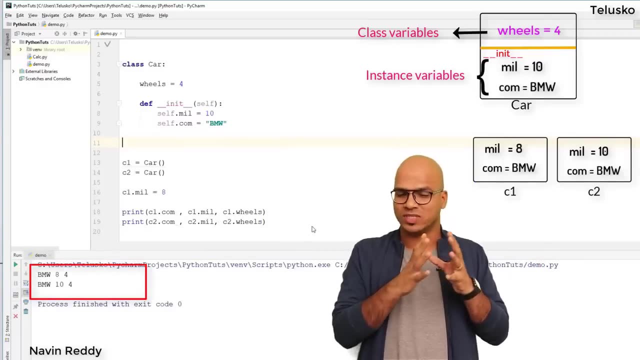 simple. you can say c1 dot wheels and here as well as say c2 dot wheels. and let's run this code now and you can see we got the output. we got four and four. so if you want to access wheels, you can use say c1 dot wheels and c2 dot wheels. see, instead of using the object name, we can also use class name. 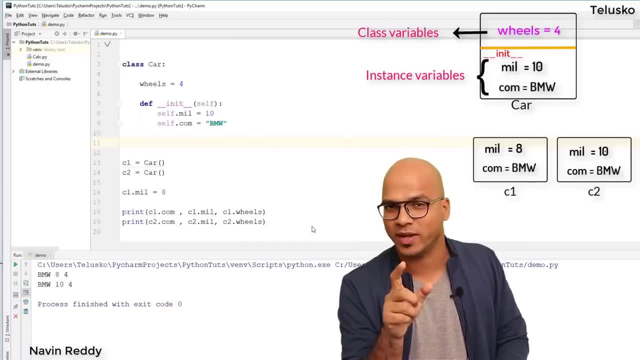 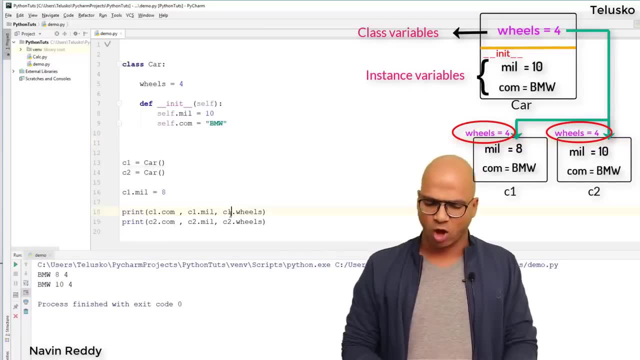 because, see, if you talk about mill and com, it is specific to the object, right, but that's not the case with wheels. wheels is common to all the objects, so every object can share the same value of it. so we can use object name or we can use class name, both works, so you're getting value. 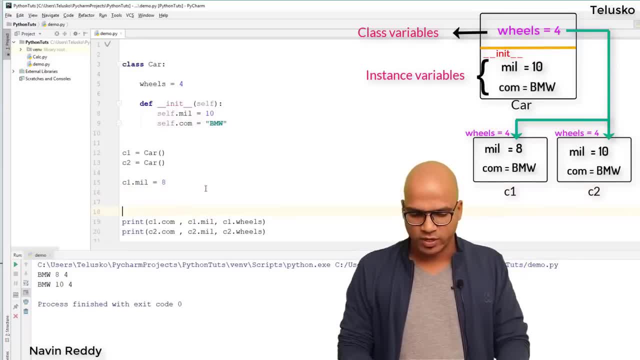 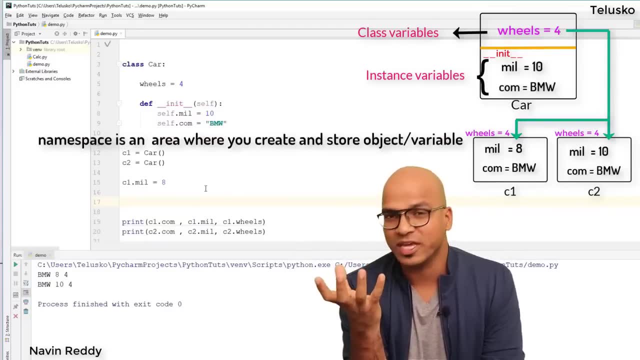 4: right, what if you want to change the value of it? if you want to change the value, you can come here and you can change the value. see what happens. you know in your memory you have different namespace. now, what is namespace? the place where you create an object or the variables. that was namespace. 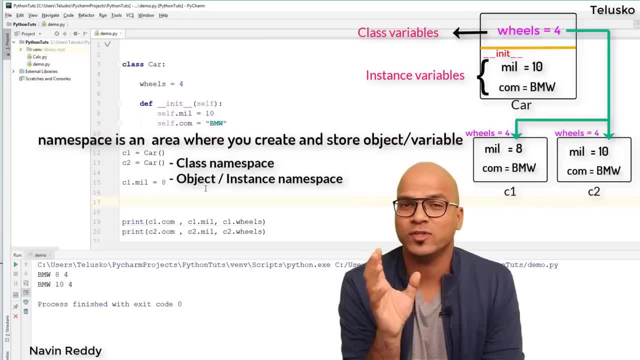 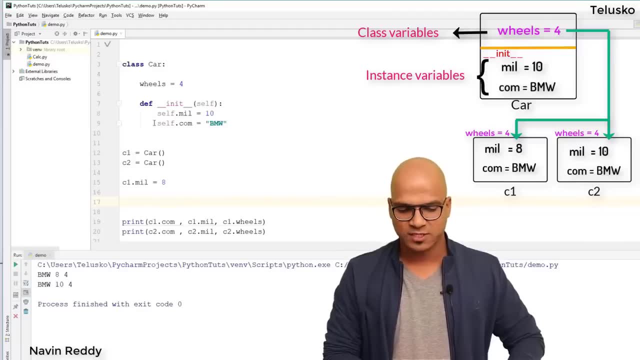 so we have two type of namespace. one is class namespace, where you will store all the class, where you will create all the instance variable. so these variables, which is mill and com, they are instance right, so they will belong to instance namespace. this wheel belongs to class namespace. 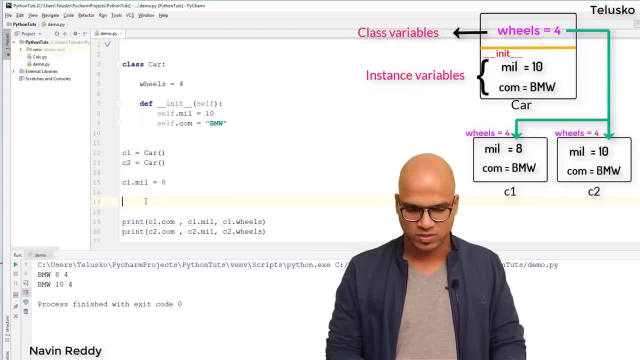 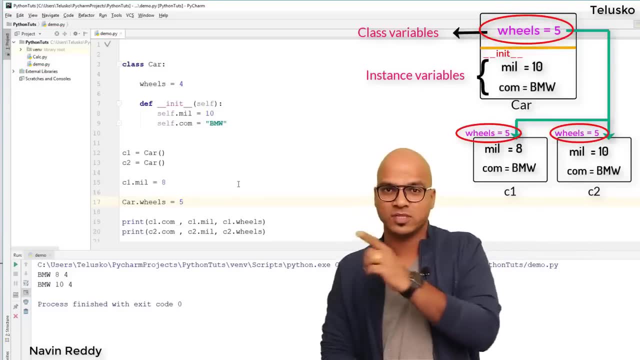 right. so if you want to work with wheels, if you want to modify it, you have to use a class name. you have to say car dot wheels and you can assign the value to five. now, the moment you change the value for wheels, it will affect all the objects. right, because they are shared. so this wheel is 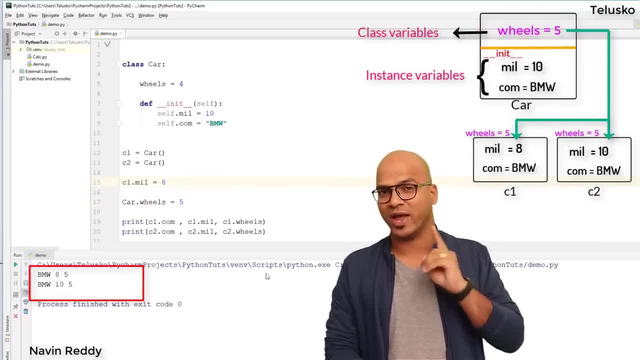 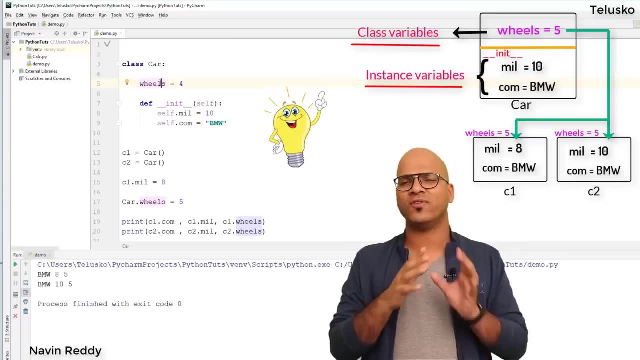 shared between all the objects. and now on this code you can see the output is five and five. so that's your class variable. so the point to remember is we have two different variables. we have instance variables and class variables, or in fact class variables also called as static. 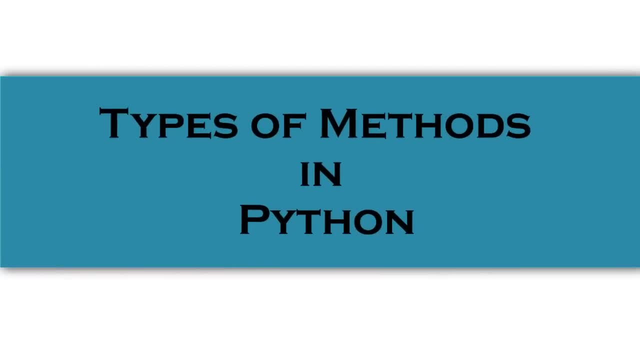 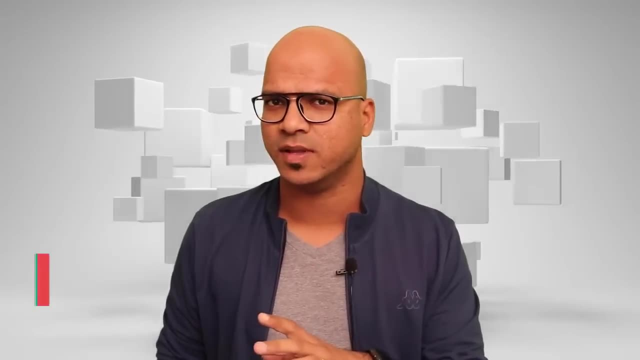 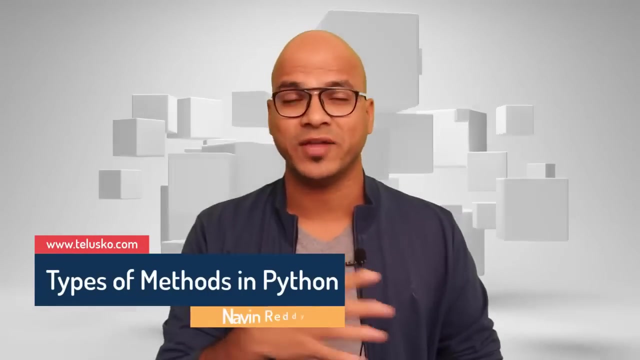 variables. now, till this point, we have talked about different types of variables. right, we have seen instance variable and a class variable. we can call them as static variables. right now, in this video, we'll talk about methods and different types of methods. now, we have seen that right. when we talk about 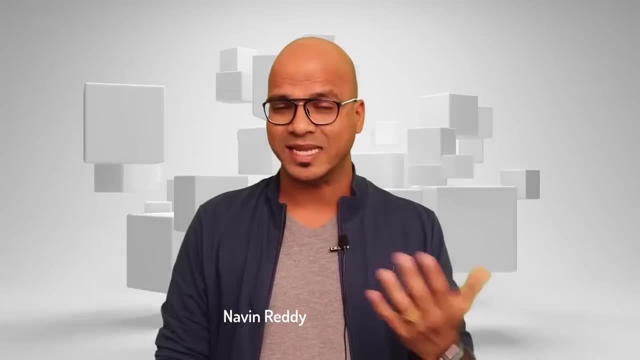 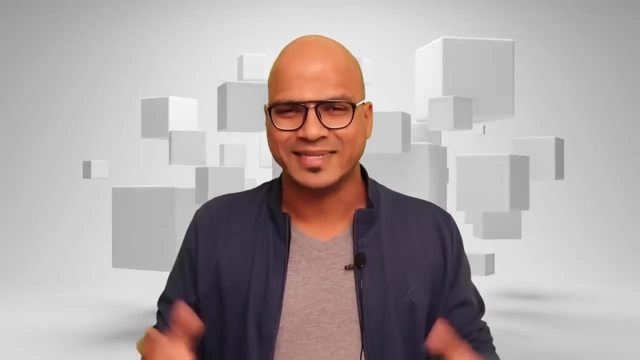 objects. object will have two things right. the first one it will have is variables and second one is methods. now, variable to store data and methods for the behavior, right? so if you want to perform some operation, that's where methods comes into picture. as human as well, we know something and we do something right. so those are your. 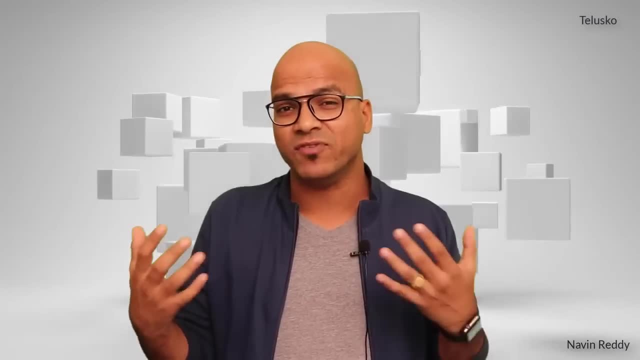 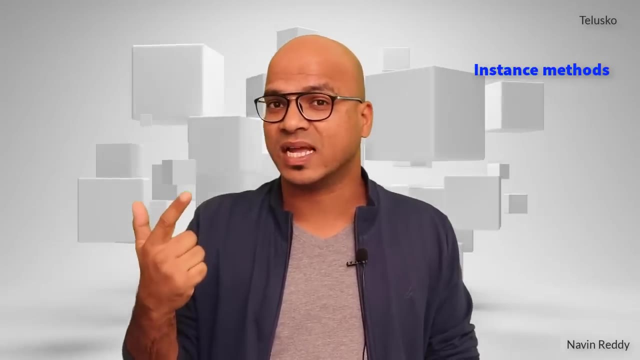 variables and methods. right now, here, when you talk about methods, we have different types of methods. now we basically we have three types of methods. the first one is instance method. the second one we have is class method, and then we have static method. oh, hold on. when you talk about variables, 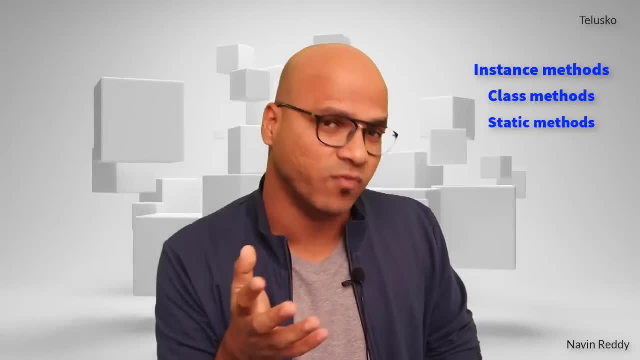 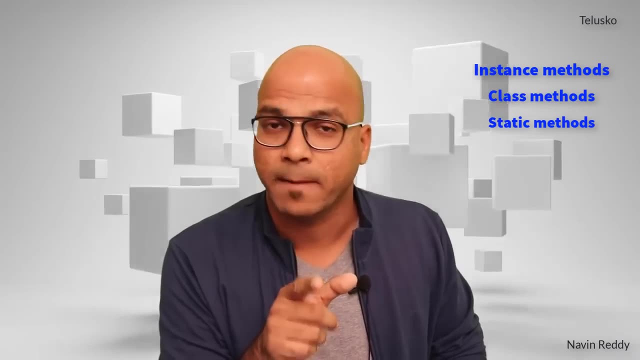 we only have two. right, because class and static behave the same way in variables. but hold on, in variables we have class variables and stability variables, which are same. that's not the case with methods. okay, so class methods and study methods are different in methods. okay, so let's. 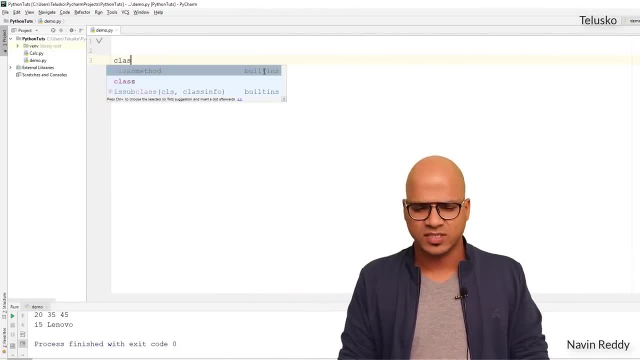 get started. so understand this concept. we'll take an example. so let's take a class here and we'll in this class as student. so in this student class, we'll be having multiple variables. right now, of course, when you talk about student, we have names, we have row number and then we have 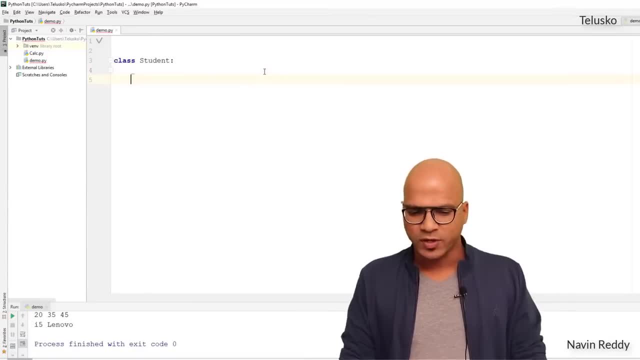 marks. at this point let me only focus on marks. okay, so what i will do is let me create a function which is your init function, because i want to declare some variables. so it says self dot. now i want to go for three variables here. one is marks one and marks one i want to pass this value from. 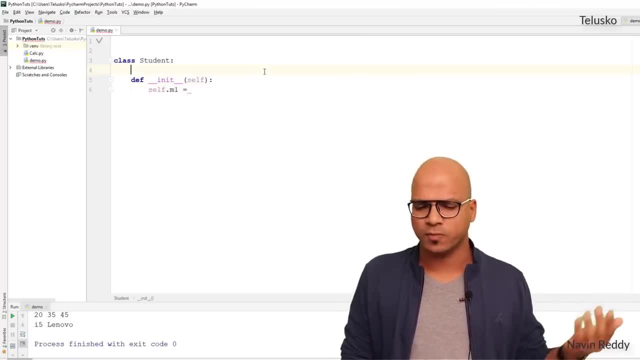 the user. okay, of course you can define your own values here, but i want to pass the value when i create the object, and the way you do that is by saying self comma. you will pass m1, m2, m3. i want to pass three variables and m1 value will be assigned to the object by saying self dot m1. 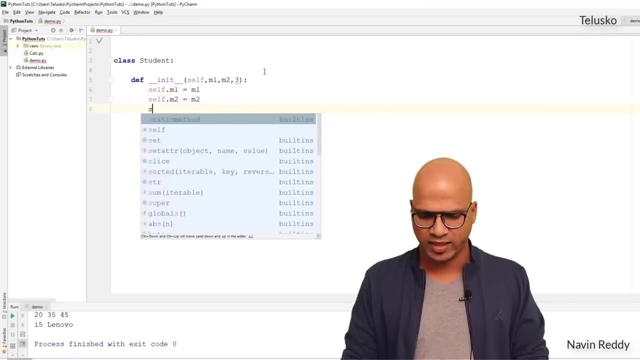 equal to m1, i will go to same thing for m2. i will say m2 and the same thing for m3, right? so we got m1, m2 and m3. now we got three variables. i want to create certain objects here. okay, let's create. 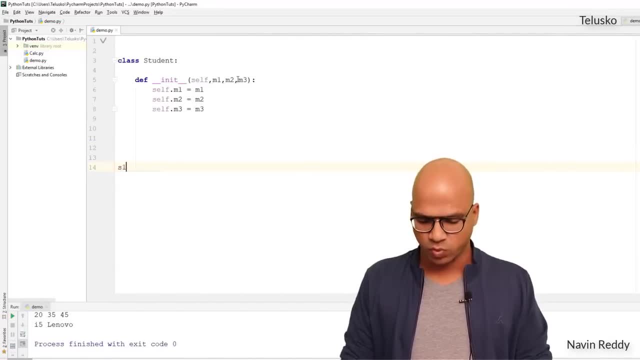 objects for this i will go back here. so let's create the object here. i will say s1 is equal to and as usual, we can create multiple objects, but time it will go for s1 equal to, i will say student, that's my first object, and if you get one more object we'll say s2, equal to student. so we 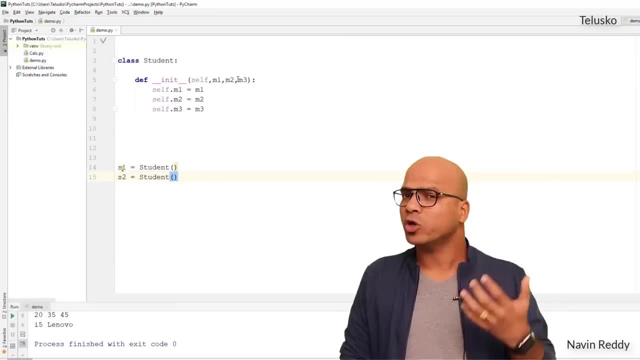 basically, we got two objects here. one is s1 and s2. i also want to pass a value to it, right, because we are not passing it. so let me pass any value, a random value. i'm not actually saying what i'm typing here, but then we got three values there and here as well. i will go for any random value that doesn't make. 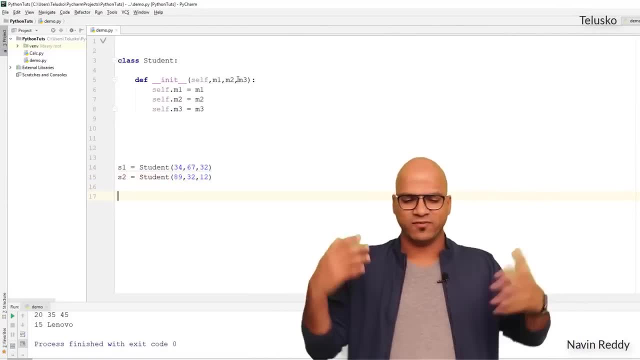 any sense to see that. so we got these values right. so first one got 34, 67 and 32, seconds student got 87, 32 and 12.. now what i do is, of course, this variable c of m1, m2 and m3. those are: 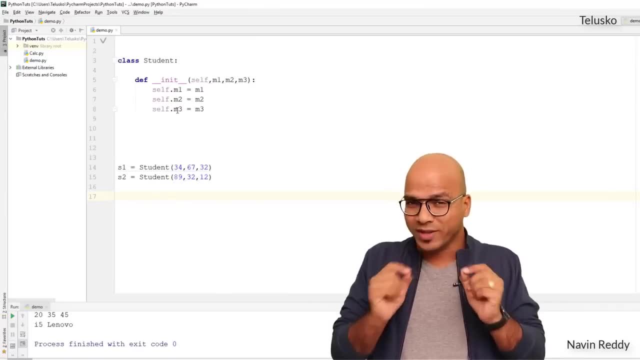 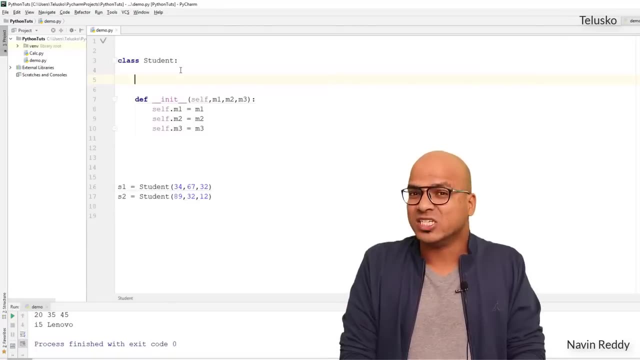 instance, variables. right, we have talked about that. we, at this point, we have not created any methods. let me just do that. in fact, before going for methods, let me also create a variable, a static variable this time, and the way you create a static or a class variable just by defining or declaring. 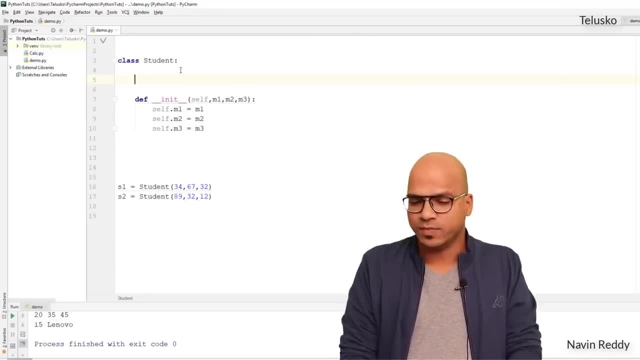 constructors, right. so here i will say: i have a variable and we'll name this variable as school because, of course, right a student belongs to a school, right or a college. at this point, all the students belongs to the same school, which is the disco. imagine if we have the disco university. we'll 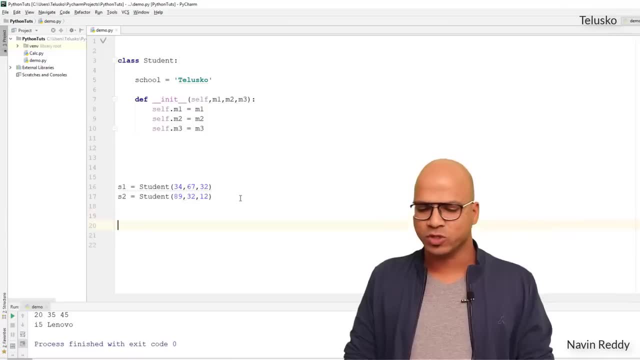 be having a school, so we got the school name as well. right, so you can print those values by simply saying: in fact, you can print those values here as well. you can say x1.m1 and x2.m1. we can do that. what i am concerned about here is: i want to know the average of marks. okay, so i've got these three. 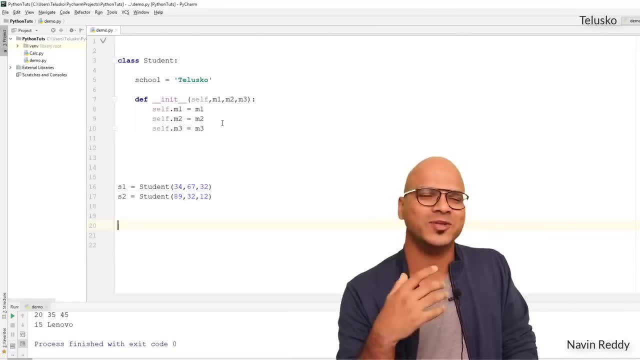 variables right. i want to perform some operations and then i want to know the average of the marks. how do you find the average right so you can? the logic of average you can define by yourself. you know everyone have their own way of doing it. i will be doing a very simple calculation, so let 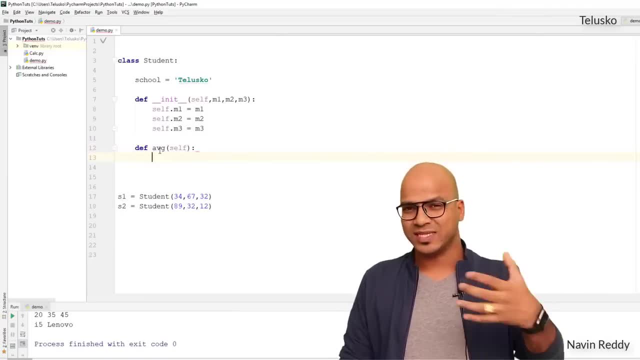 me create a method called as def method, called average. so when i say object dot average, it will give me average marks. okay, so i want to return the average marks. and the way you do that? by saying return. you want to return the value and here you will simply say m1, or not just m1. you have to say 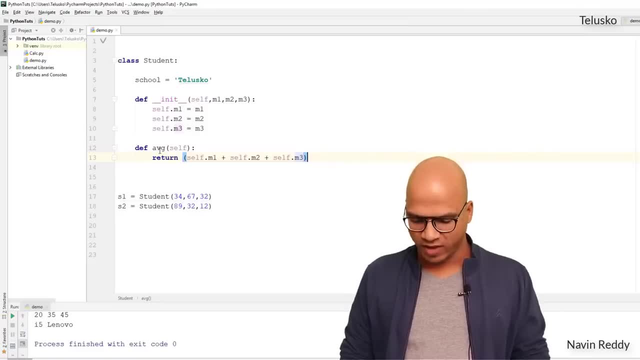 self dot m1 plus self dot m3. so we have to divide this number by three. that's how you find the average right and we know the stuff right. that's how you find it average of multiple numbers. so we got the average and we are returning the value. okay, so now this: 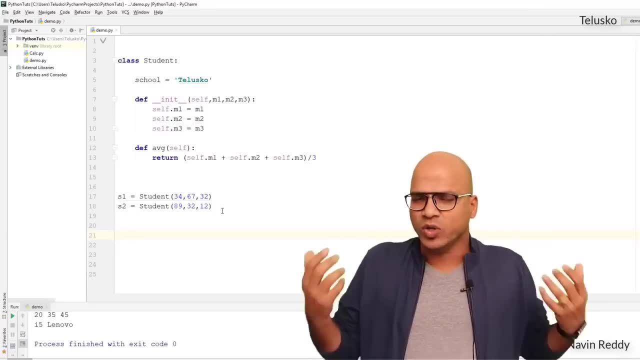 if you focus on this average, this is a instance method. how do you know that's an instance method? because we are passing self. now, when you say self, it means it belongs to a particular object. right, of course, we are defining that in a class, but it works with the object and that's why you're. 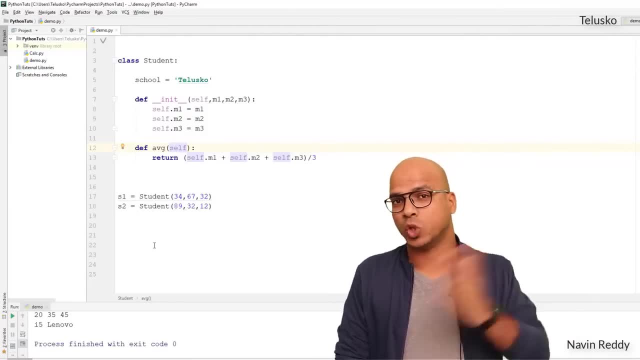 passing self. so if you want to call average, you have to say s1 dot average, or you have to say s2 dot average, because we are passing self. we cannot simply say student dot average, because we are not using object there. but in this case we have to say s1. 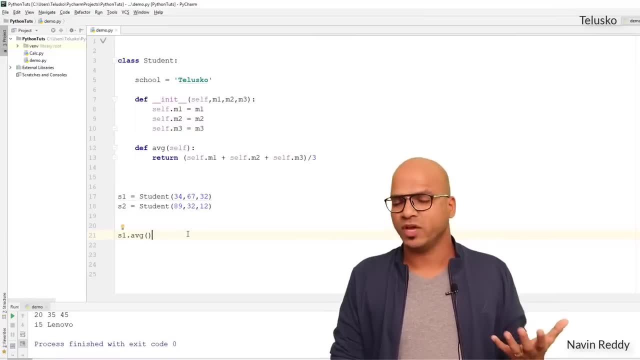 avg. that's how you do it. so i have to say s1 dot avg. it will give you the value, so i will print the value here. i would say: print the average here. so let's run this code and you can see it works. we got the average of first student. you can do the same thing for second string. you can stop saying. 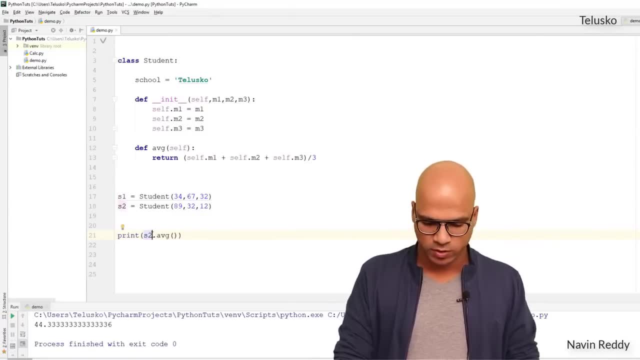 s1 dot average. you can say s2 dot average and if you run this code or you can see we got the average for second string as well and they almost same, i don't know why. okay, so after changing value we got different average, you know. so this was just a coincidence. you know, i've given some values and 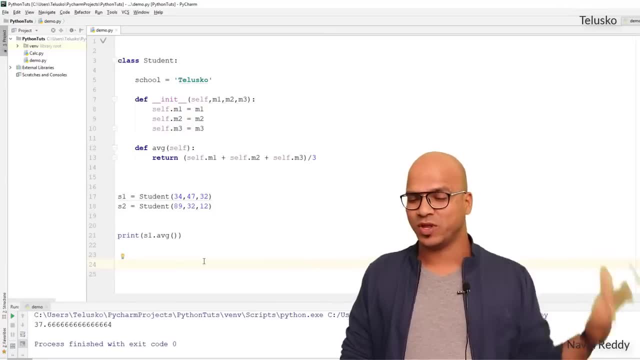 then they were giving the same average right. so yeah, so you got different average for s1 and the average for s2 dot. so that works. now what we're going to do. so this method here, this average, is a instance method, because it works with the object. now, in instance itself, we have two different types. 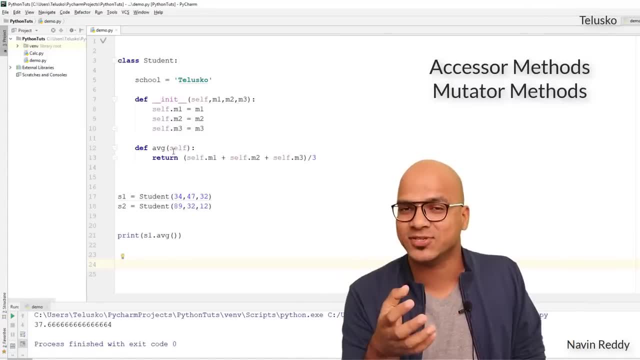 okay, the first type of instance which we use is called as accessors and the second type we use is mutator. so we have accessors and mutators. now, what is accessories? so, if you are only fetching the value, see, ultimately, when you talk about these methods, they are only responsible to work with. 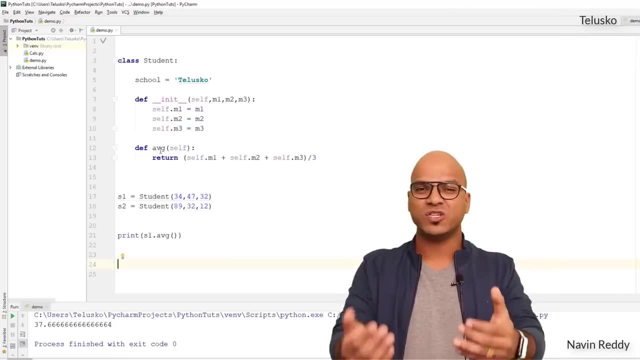 variables, right, which is your instance variables. so if you want to just fetch the value of the instance variable, we will be using accessor. this is what we are going to use: accessor and there accesses. if you want to modify the value, you will use mutators. so the way you do that example, if you 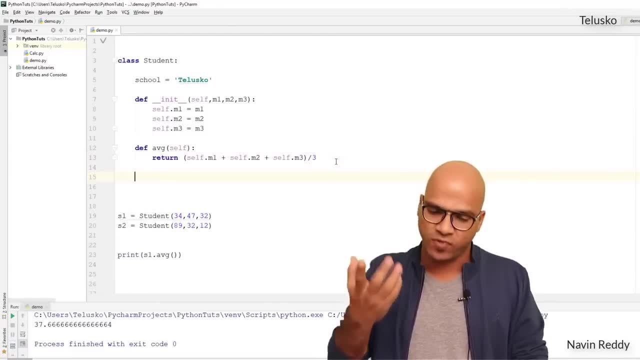 want to fetch the value of m1. so if you want to know the value for m1, you can fetch directly. you can say print s1.m1. you will get the value. like this, or instead of using the variables, we should actually use methods. so what we'll do here is we'll say def and we'll define the function as. 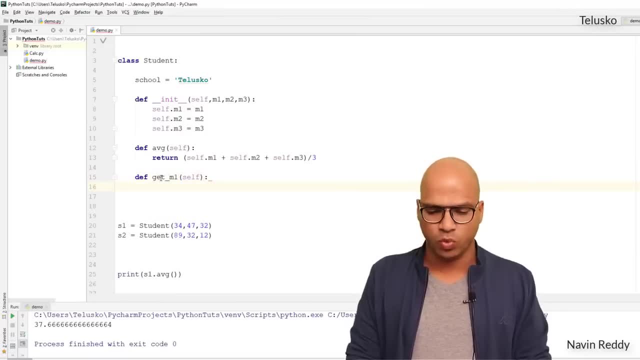 get m1. so we'll say get m1 and which m1 you want. so you will say return, i want to return the value for selfm1. this is how you do it. so if you want the value for m1, you will say get m1 and you've. 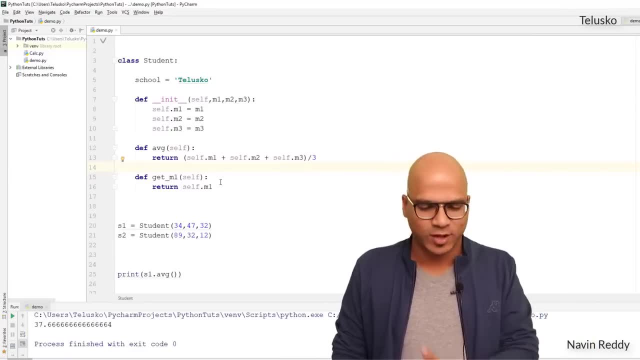 got the value. normally it's not compulsory to have that get keyword there. you can also say m1, that's fine. but when you write a code conventionally you simply specify get there. so whenever you say get methods or in fact to set the value, we use set methods. example, if you want to set the value for 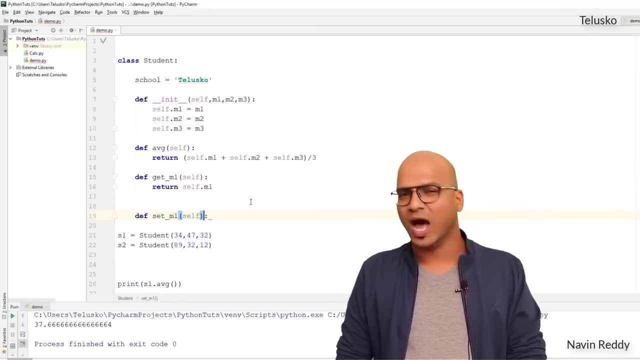 m1, you will say set m1. of course we are passing that from a constructor, so we can say set m1. and you can pass some values here. i would pass a value, f, i would say a value, and this value will be assigned to the value of m1. so if you want to set the value for m1, you will say set m1 and you will. 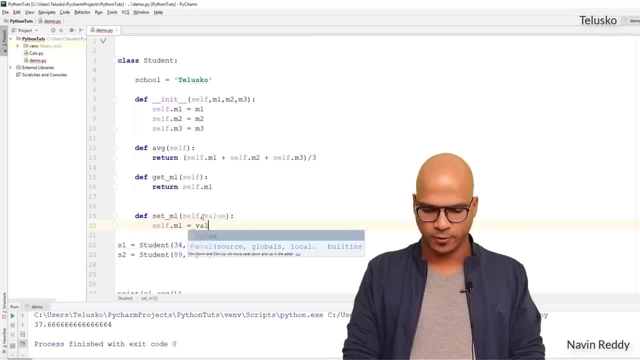 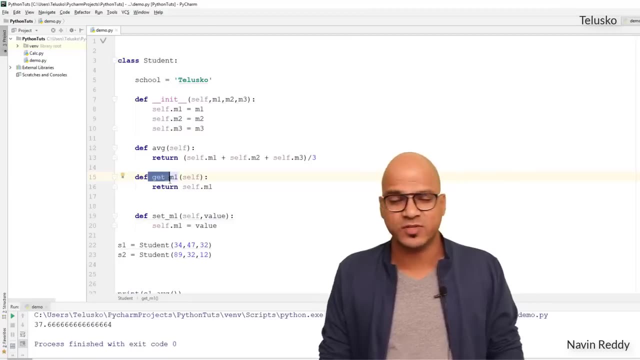 assign to m1. so we'll say selfm1 is equal to value, so you can use constructor to pass the value or we can use setters, right? so we have get methods and we have set methods. now for different variables. we'll be having different get and set methods, right? so if you have three variables, you 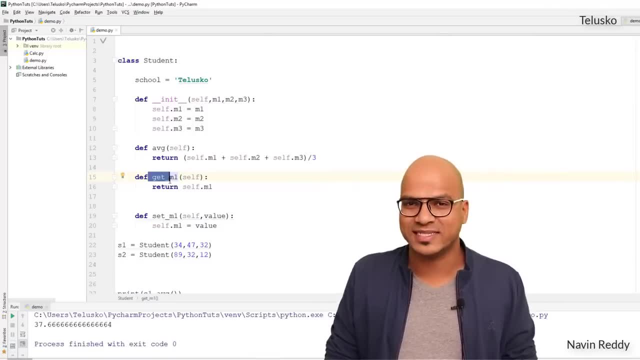 might be using three get methods and three set methods, and that's why they're called as getters and setters. right, so getters get the value, setters set the value. getters only fetch the value. it will not change the value. that's why we say accesses setters. they change the value and that's why we 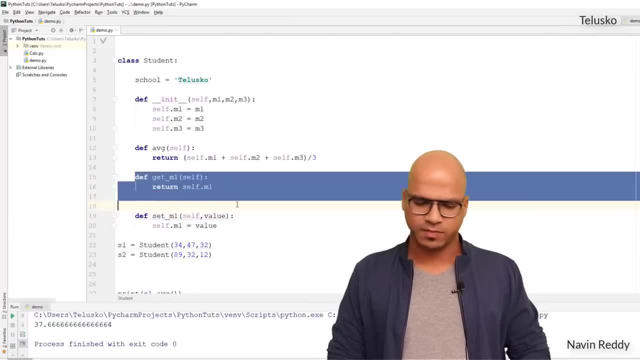 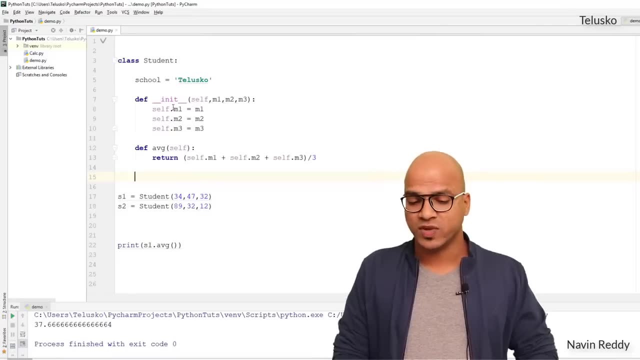 say mutators. so this makes sense. whether or not you can do that, you can do that, you can do that, you can call these methods right, but this works. now, once you talked about instance, the second type we have is a class method. now why we use class method? see if you talk about these variables: m1. 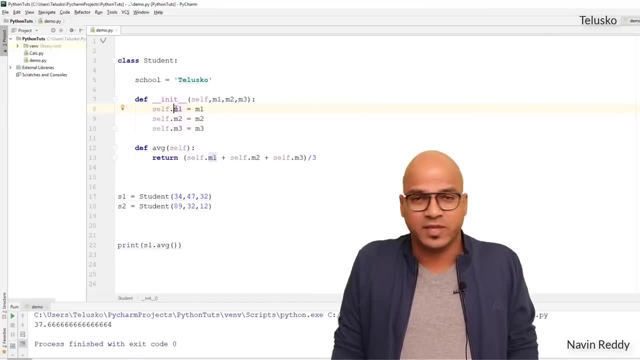 m2, m3. those are your instance variable. right? an instance variable can be used with instance methods. what about this one? this is school right now. school is basically your class variable, and if you want to work with class variable, you need to use a class method. and the way you do that? 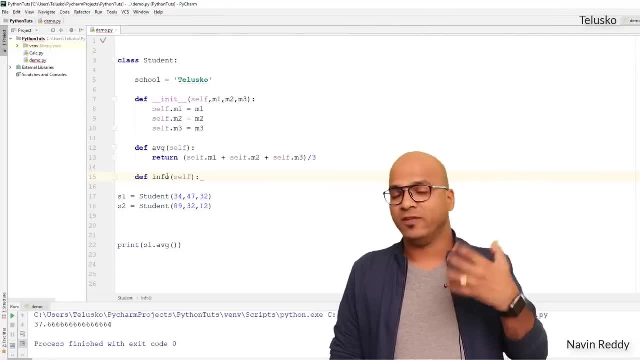 let's say i want to know the info of a student, so i will say dev info, info will print the name of the school. okay? so let's say, if you are studying for teresco, you will be. it will print teresco and of course, all the students belong to same school, right, if you? 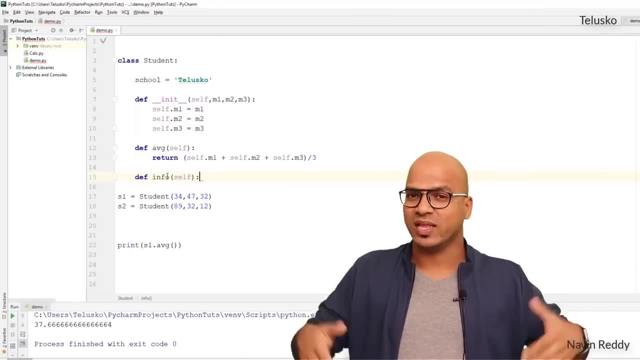 change school name for one student, it will affect all the student. example: this channel name earlier was lavin skills, right, and we have changed it to teresco. so if the name changes for one subscriber, it will affect all the subscribers, right, and that's what is happening here. so if i want to, 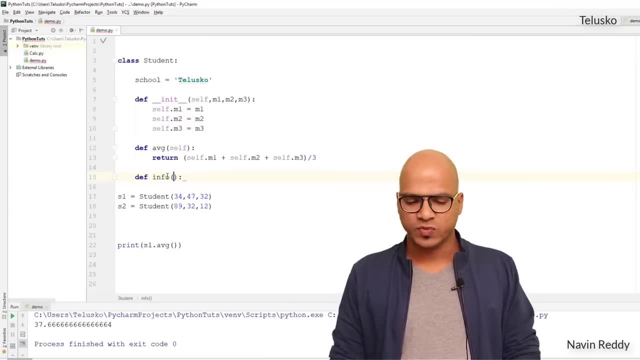 print info and that to a school name. i don't want marks here, of course. we don't want to work with self, we want to work with class, right? so if you are working with instance, you will use a self keyword. if you are working with a class variables, you have to use class. 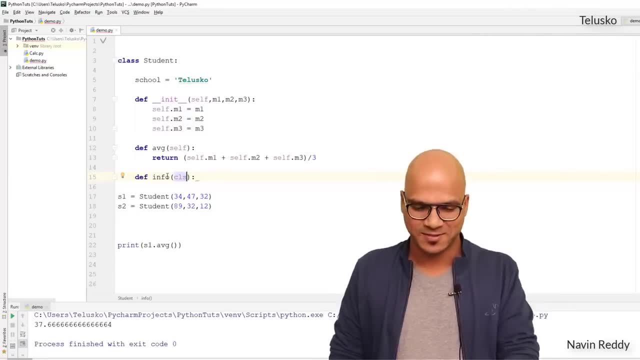 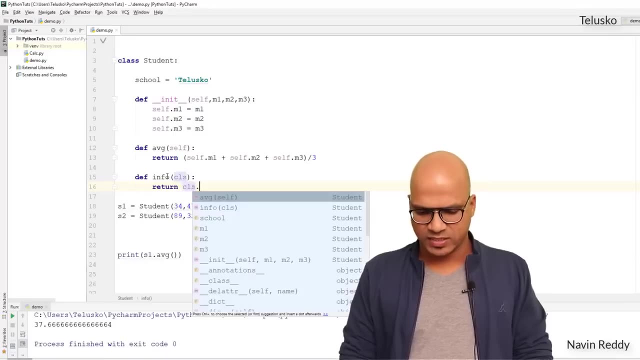 c l s. okay, it should be cls, it should not be something else. now, once you got that, you can simply print the value. so you can say print, or you can return the value- your choice- or you can say: return cls, dot school. that's how you do it. so you have to say clsschool. so whenever you want to, 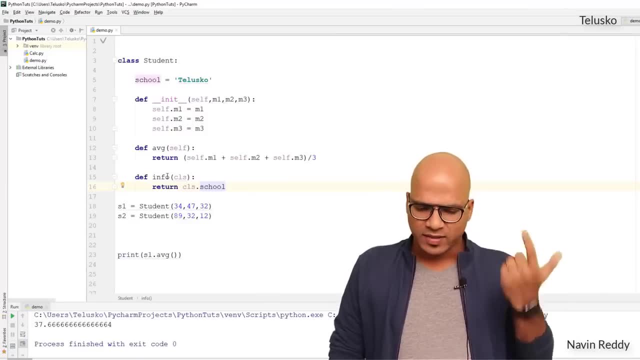 work with class variable. you have to say clsschool- okay, but then how do you call info? it's very simple. you will say print s1 dot info. we can do that, but there's only one problem. info should work with all the objects, right? it's not specific to one object. so instead of 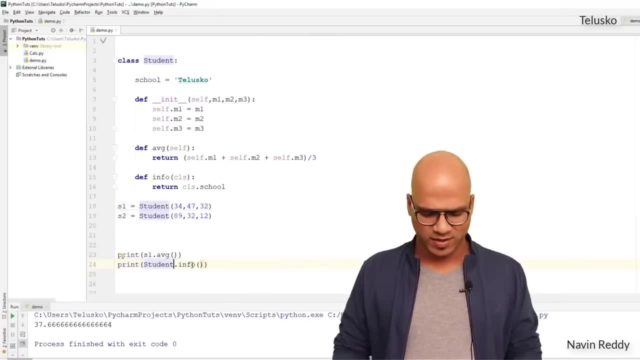 using s1. we can use a student dot info. now this should work. let's try. i will say run. oh, we got an error. it says info missing one required potential argument, which is a position argument, which is cls. oh, we have to pass cls. that's weird. i don't want to pass cls, right, in fact, we are not even doing. 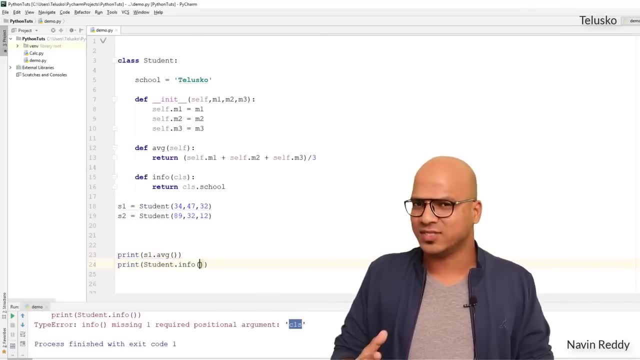 that for average. we are not passing s1 here. also, i don't want to pass thing normally. what happens? you know, if you want to create a class method, we need to use a special symbol or special way of doing that, and we can use something called decorator. 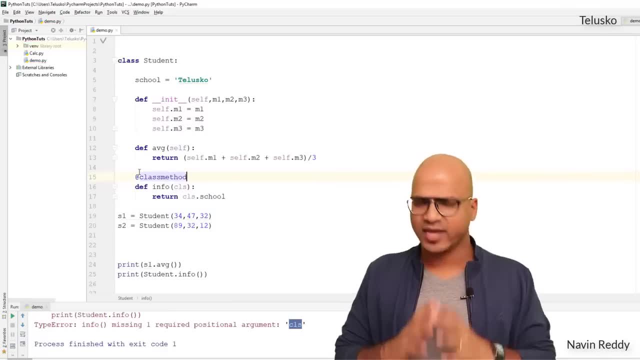 so we have to say at the rate, and you have to mention this as a class method again. we'll talk about decorators later in detail, but time being, we got a class method decorator. so if you want to use info as a class method, you have to say at class method. okay, that's how you define it, so let's run. 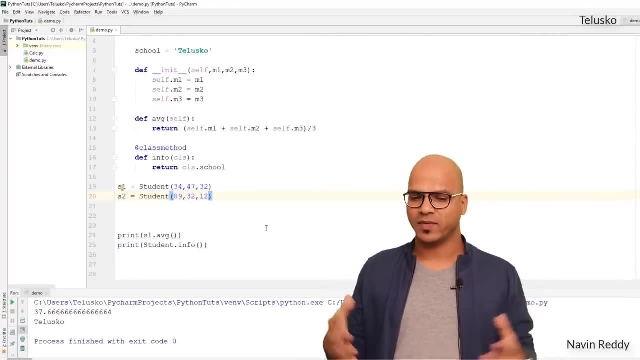 this code now and it works. you can see that we got the disco there. quite simple, right. so now we know about instance method, because it works with instance variables. now we know about class method, because it works with class variables. how about static methods, say? think about this, let's. 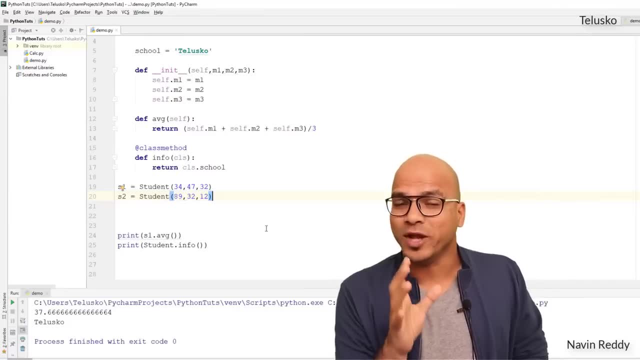 say, if you want any method, okay, it doesn't matter what method we want here. if you want a method which has nothing to do with instance variable, which has nothing to do with the class variables, we want to do something extra, okay. so something different which is not. 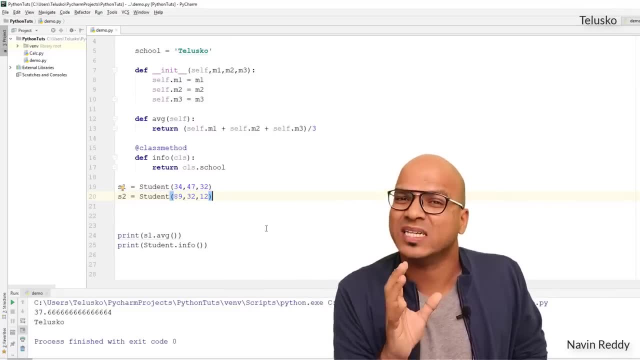 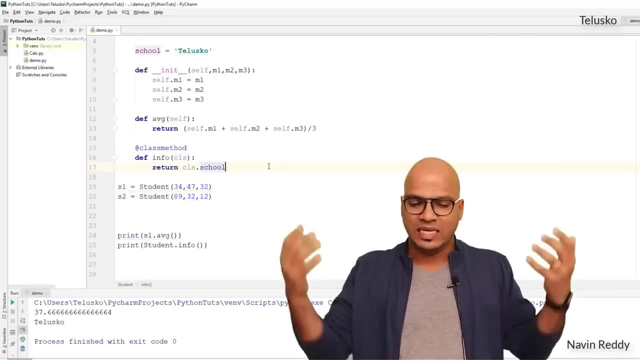 concerned with the variables. at that time you will be using a static method because we are not concerned about instance variable, we are not concerned about class variables. example: let's say i want to print the info about this class- okay, not about student, but the class. so i will say def. 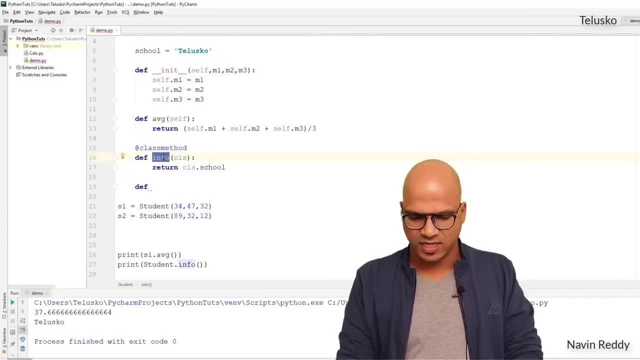 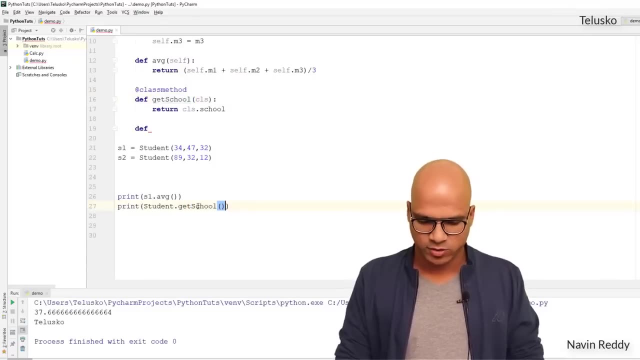 about. you know. in fact, instead of saying info for class, i would say get school name. that will make more sense. so i'm changing the name from info to get school for class method. okay, not for this. and let me also change from here. so we'll say get school here. i will define a function and 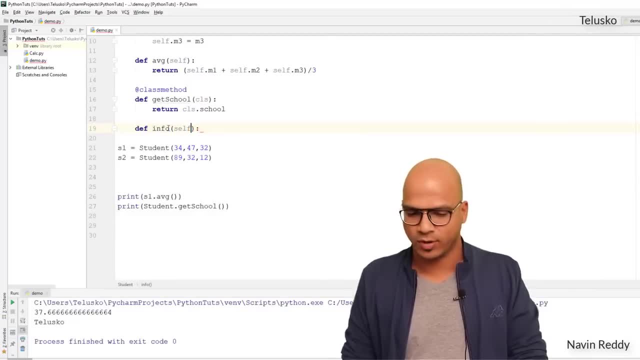 the function name would be info, because when i say info, i want to know the class name. okay, so this is not related to the object, this is not related to class, so i will keep it blank. okay, so if you don't want to relate this to a class, keep it blank. if you don't want to relate this to a object, keep it. 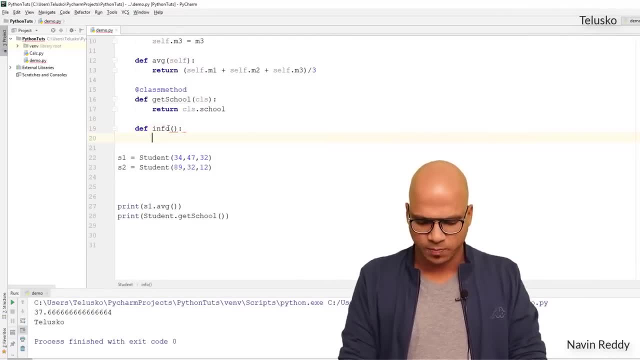 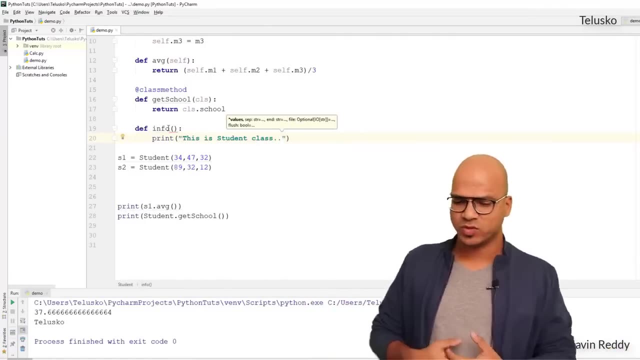 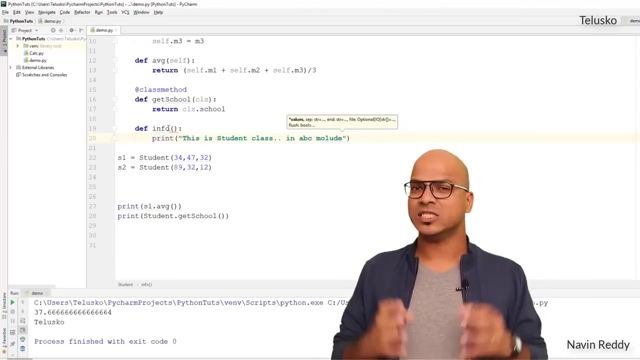 blank, no self, no class. okay, static method and this will return. this will print, in fact, not return. this is student class. you can do that right? so we are printing: this is student class and n abc module. that's it. you can print whatever you want. as i mentioned, important is this method is nothing to. 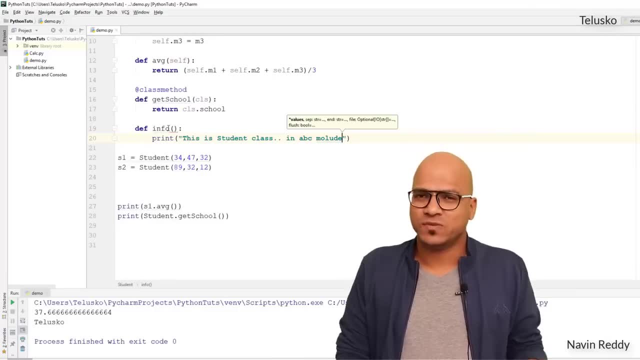 do with the class variables and the instance variable now where it will be useful. so let's say, if you want to perform any operation which has something to do with the other object, other class objects, we can use static methods here. or if you want to perform some operation like finding: 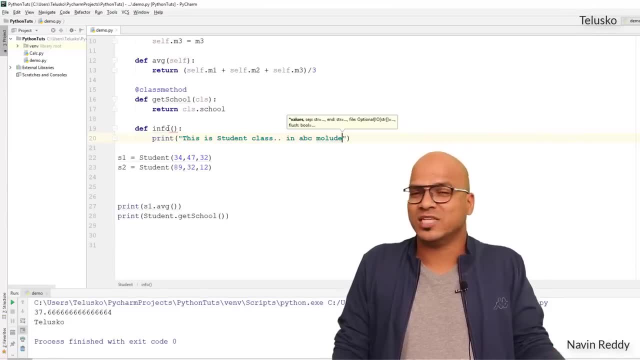 a factorial of a number. right, because the factorial has nothing to do with the class variables or instance variable. maybe you're passing a value, you just want to know what's the factor of the number. you can use static methods there. now, since we are using a static method, we need to use a special decorator here as well. so we have to say: any guess we will. 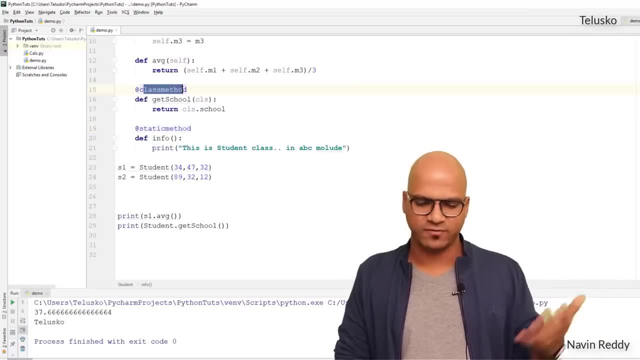 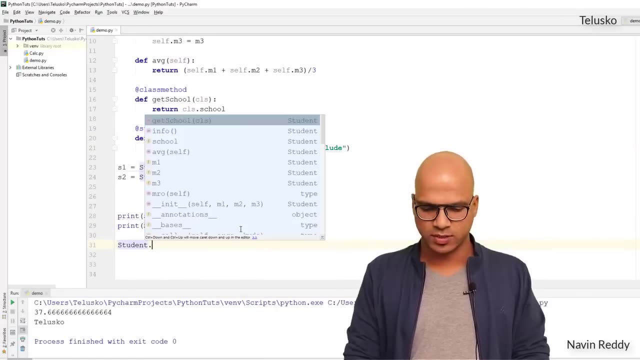 be using static method. so for class method you have to say class method and for static method you have to use static method. okay, and then you can call it so you can say so. you have to use a class name, so you will say studentinfo. right, so this is static, so you don't have to pass anything. 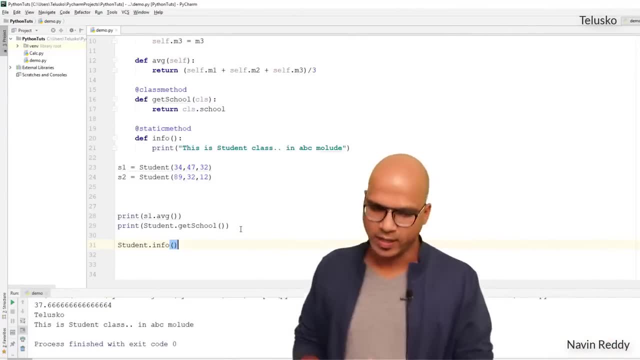 not even class and not even object. let's run this code and it works okay. so basically, we have different types of methods. we have instance method, which works with instance variable. class method works with class variable and static works with nothing. it has, if you want to do something extra with your class, nothing to do with class variables. 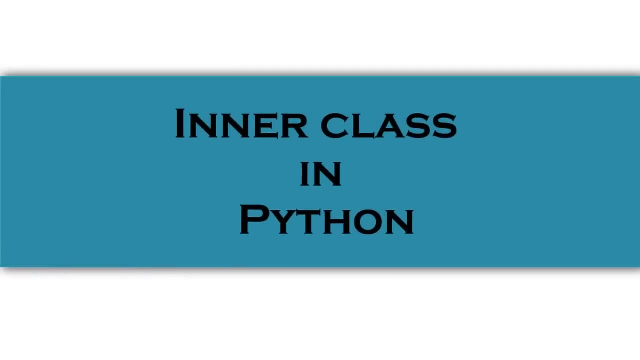 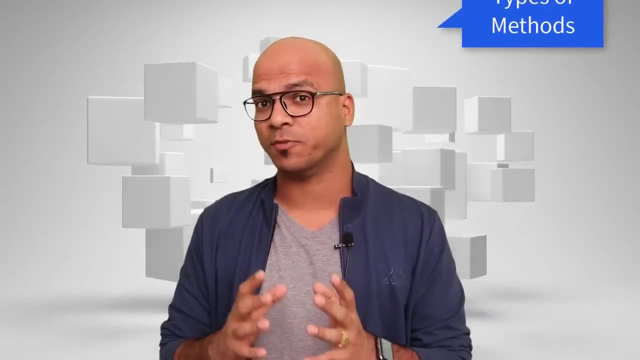 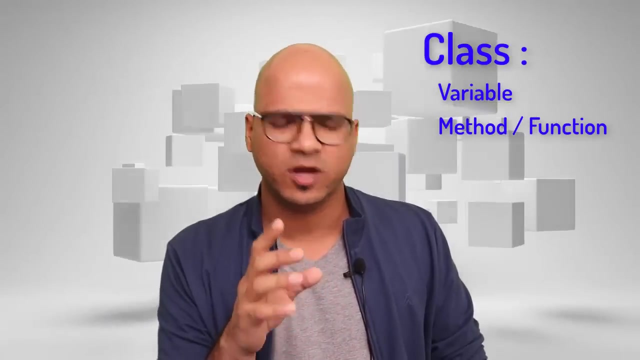 or instance variables go with static. now, till this point, we have talked about different types of variables and we have talked about different types of methods. right, so we can write variable and methods inside a class. right, so a class will have variables and methods. the question is, can we? 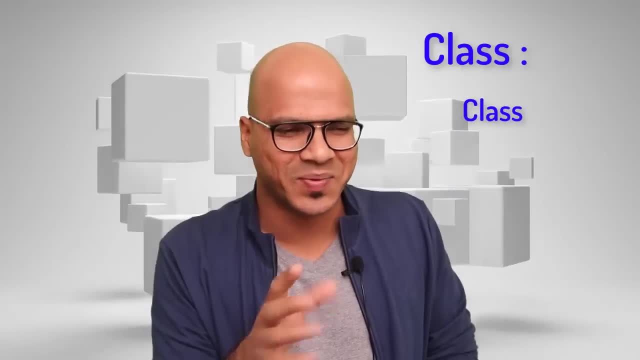 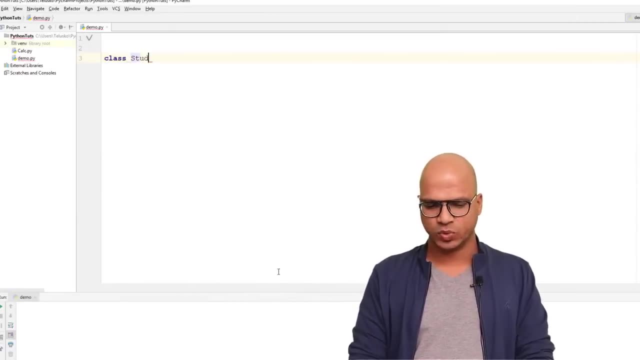 have a class inside a class. that sounds weird, right? why would anyone would have a class inside a class, so let's try to understand that. so let's say i have a class here and this class name is student, as usual, with the way we have done earlier. 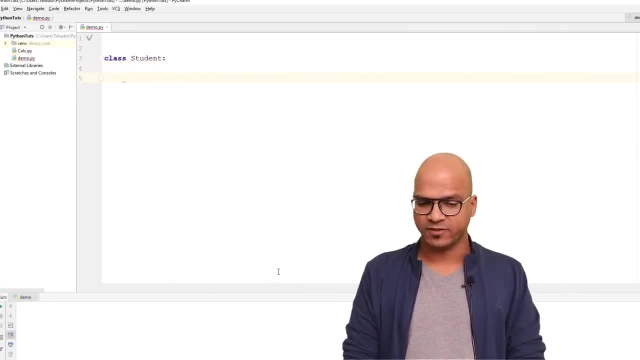 and when we talk about student, we have different types of variables. right, let me define that function first and the variables which i want here is self. first, i want a name. of course, in the last example we have taken marks, but here let's take something different. i would take a name of a. 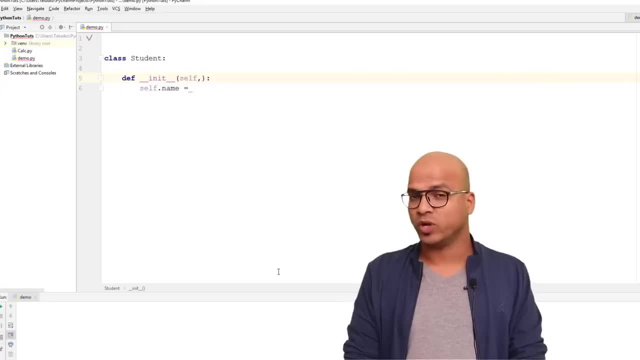 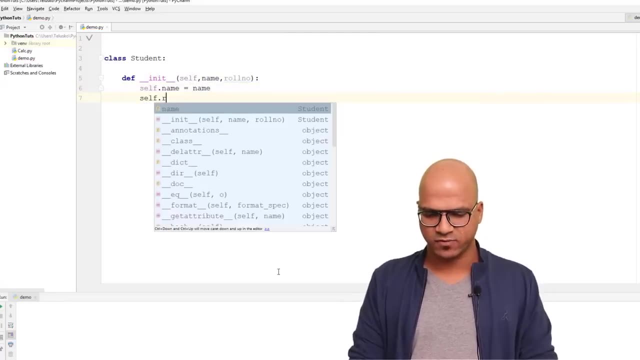 person and that will be coming from a user, of course, or from when you create object. we'll say name. the second thing i want is roll number, and i want these two details and then i will assign name here and i will say self dot roll number. now we have used to it, right, so i would say: 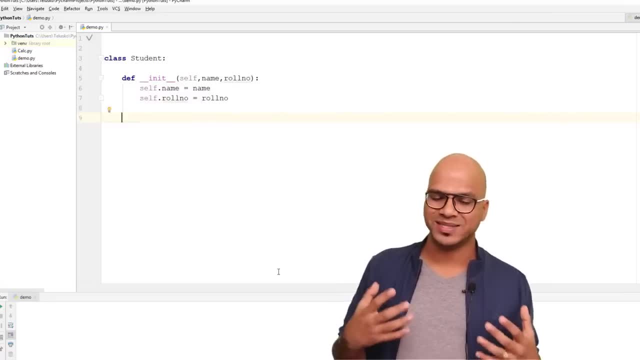 roll number right now, once we got these two variables, and what i want is i want to print them. the way you print these values is by defining some functions, right, of course you can do that directly. example, if i create object here, so let's say the object is s1 and i will say student and 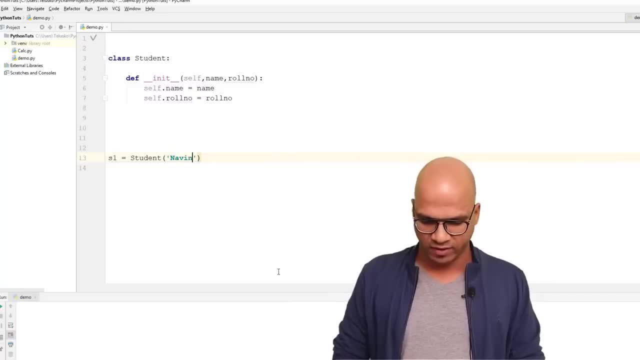 when you create this object, you have to pass values as well. right, the first one i want to have is navin and roll number is letter 2. the second object is s1 and i will say student, and when you create this object, you have to pass values as well. 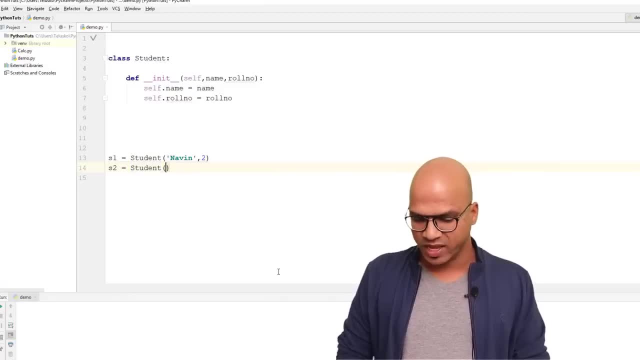 we want here is s2, and we'll say student, in which we'll be having two things. of course, I would say: this is Jenny and the roll number is, let's say, three. so I have Naveen and we have Jenny here. we got two and three, okay, so let's say I. 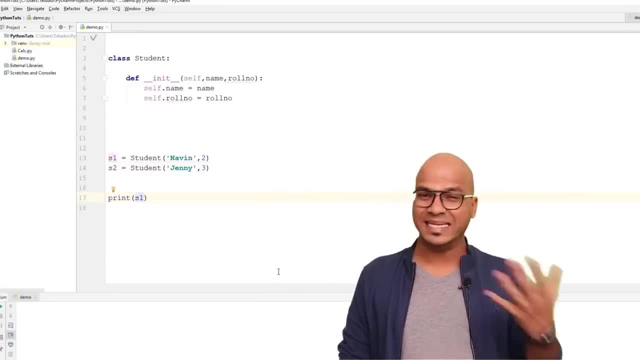 want to print. I want to print s1. so I want to print all the details about s1. okay, I want to print the name and roll number. so the way you do that is by saying s1 dot name and we can say s1 dot roll number. so this is how you can print. 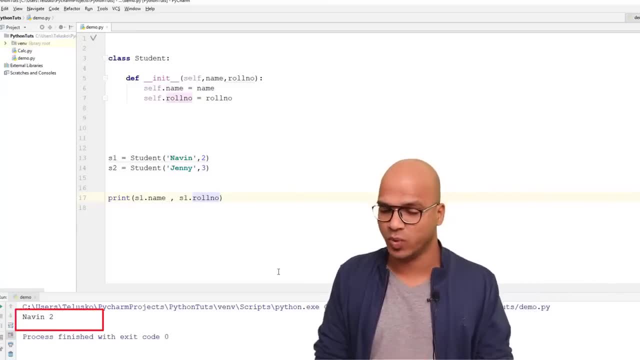 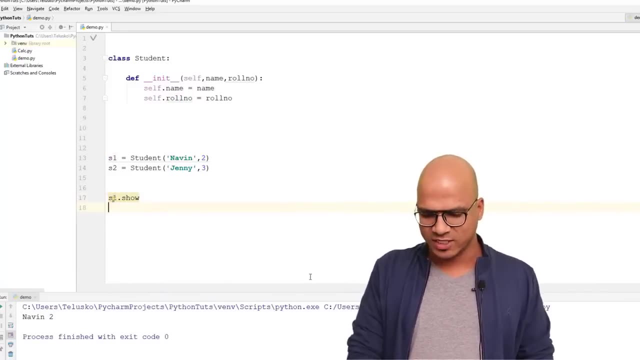 the values right. let me run this code and you can say it works. we got it there. details about s1. now what I want to do is: I don't want to see. this doesn't look good, right. what you should be saying is you should say: s1 dot show. so when I say: 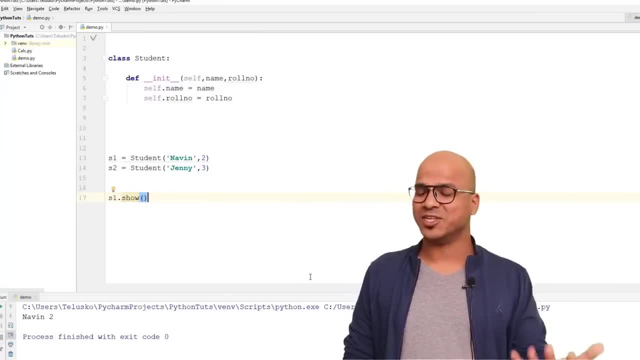 s1 dot show, it should print all the details about s1. maybe it has roll number, name or different variables, right? so of course we need to define that function or method here. so we'll say dev show. so this will print self dot name and will print self dot roll number. so we are printing this two data, right, it should. 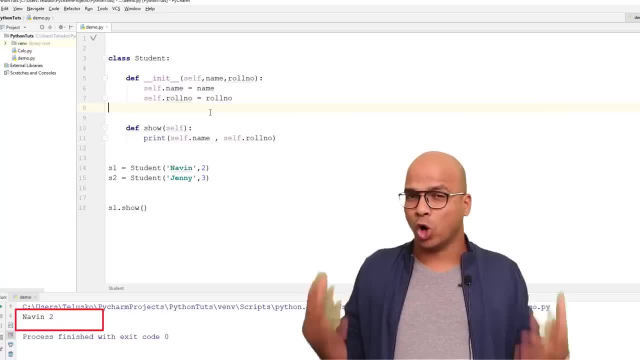 work. let's run this code and you can see. we got the same data. now let's say: student also has a laptop, of course. right when you say you are doing IT. in fact we have done that right. so you are a student of the Cisco. you will be using a laptop to run your code or desktop. 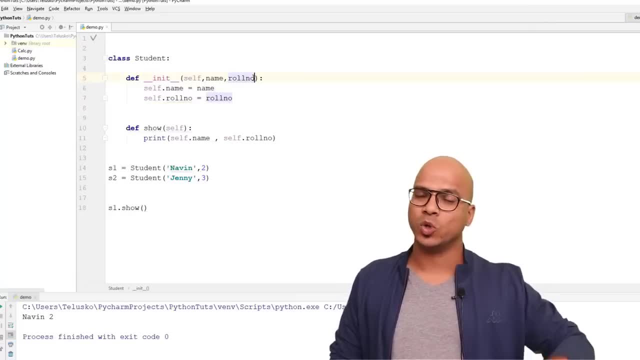 doesn't matter. and let's say we want laptop here. so of course I want to know which laptop we are using. so I want to know your config. now, in that case, I will also ask a user: hey, tell me which laptop you're using. the problem is we talk. 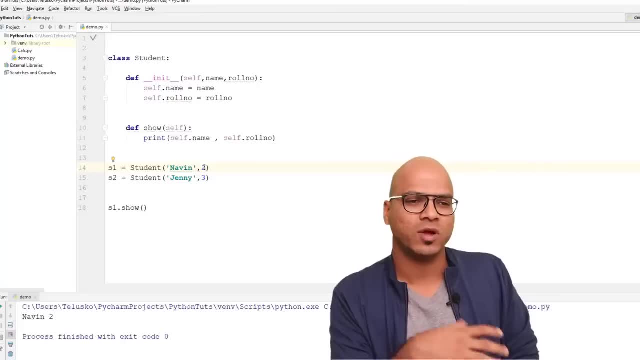 about laptop, that different things, important, right, it's not just about brand. you will not simply say, hey, I have HP laptop, I have a Lenovo laptop. you will also mention the configuration, maybe CPU and run. that's very important. maybe you have an i5 CPU with, let's say, hdb ram is enough. so I want to know your 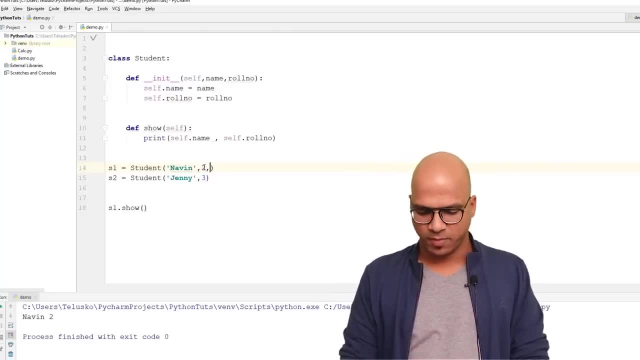 config. so what you will do will you pass three variables like the, you will pass a brand, HP, and then you will also pass the CPU which you are using, let's say i5, or you will also pass, let's say, ram of a GB. yes, you can do that. okay, so I have to. 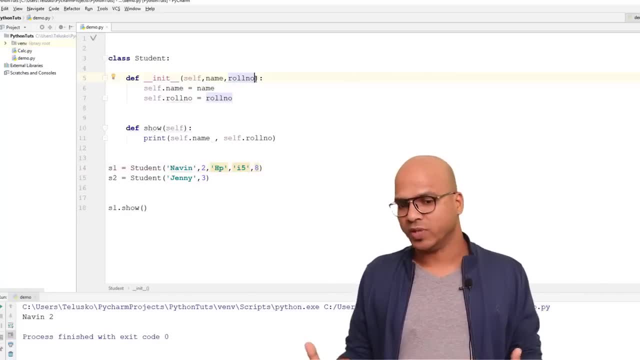 accept this. variables here. I have to accept that here. right, and we can do that. the other option which we have is: we different, okay, so the other option which we can do here is we can create a class. okay, we can create a separate class as laptop or instead of creating a computer, we can create a class and we 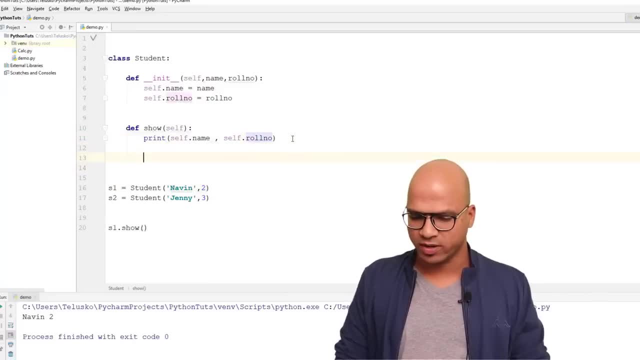 can create a laptop or, instead of creating a computer, now we can create a class outside the student, we can also create laptop inside student. so a laptop will be only used by student and in this case, so i will say a class and also laptop. so we are creating a laptop. 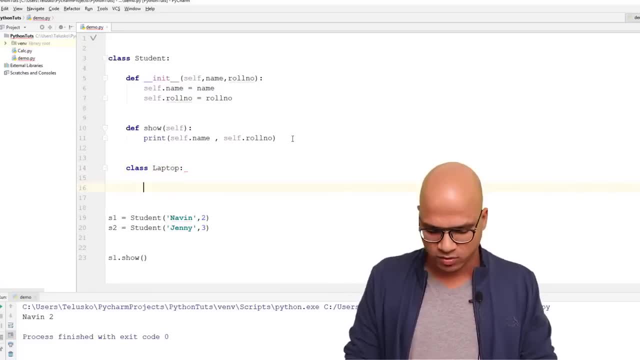 class inside a student, so that we can get that group okay. so we have to also say def here and we have to say in it: right? and then let's create variables. so the first variable we need here is brand, and let's say the brand is hp. that's the first thing we need. second thing we need is the. 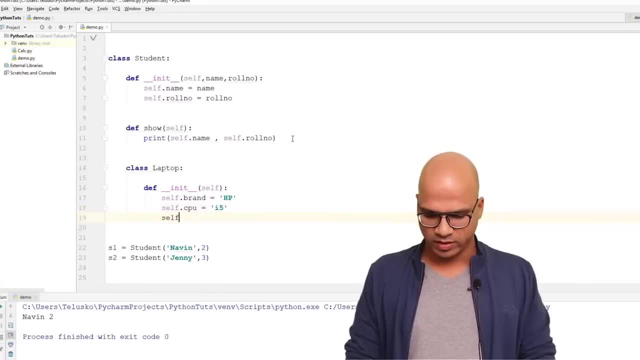 cpu which you are working with. i would say cpu is i5 and the third one is ram, let's say gb ram. so we got these three things right now. we got these three variables and where to create the object of it. so we can create the object here itself, so we can create the object inside the init, and 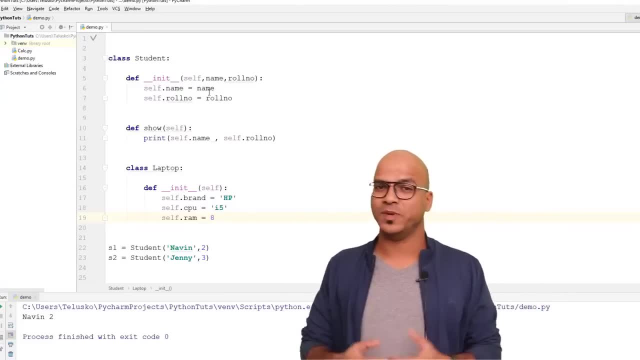 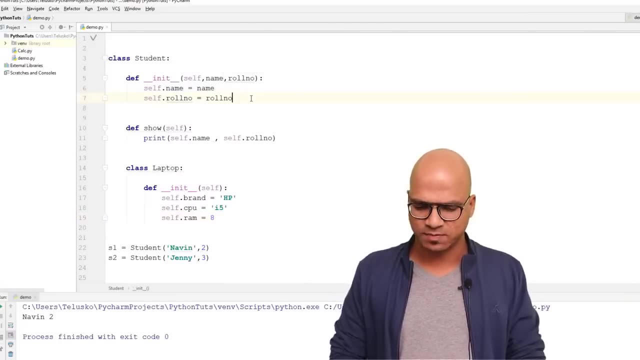 normally that's what we do. so if you want to create object of laptop, we should be creating that object inside the outer class. okay, so the object of laptop will be the inside the student class. the way you do that is very simple. here you will say: self dot lap. you can create any variable. 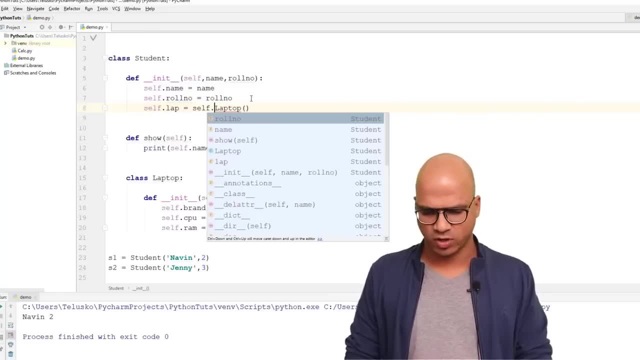 you want and you will say self dot lap. you can create any variable you want and you will say: say laptop, or we are getting error so we have to say selflaptop. okay, this works. so you can see, in the constructor itself you can define a variable. so in the outer class you can define a variable. 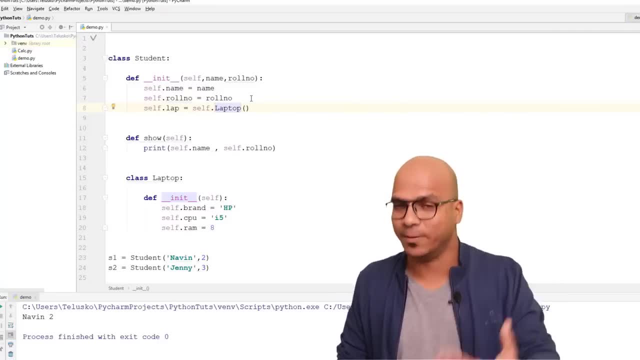 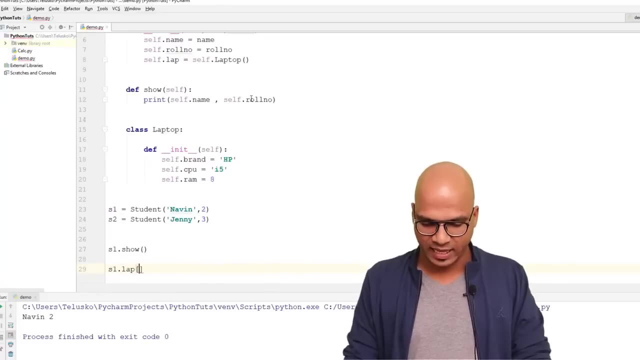 lab and you can define the object. so if you really want to use a laptop, you have to say the student object: dot, lap, example. outside. if i want to use it, i will say s1 dot, lap, dot, whatever brand you want to fetch. so you cannot simply say labbrand, you have to say s1.labbrand, because 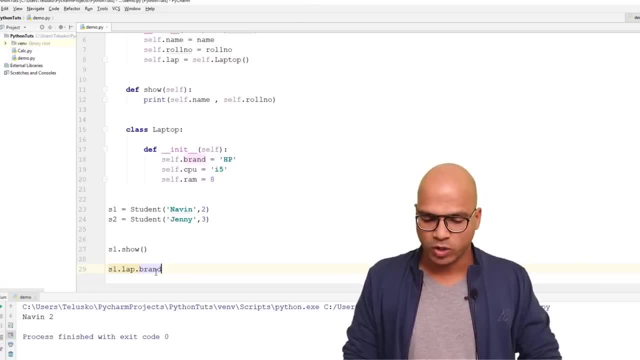 the lab object is inside the student class. this is one way. what if you want to create another object of it? let's say i don't want lab i want. so you can simply say lap1 is equal to s1.lab. you can get another object for s2. you can say lap2 is equal to s2.lab, because 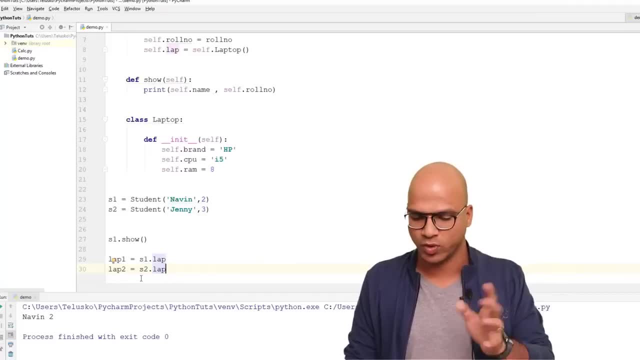 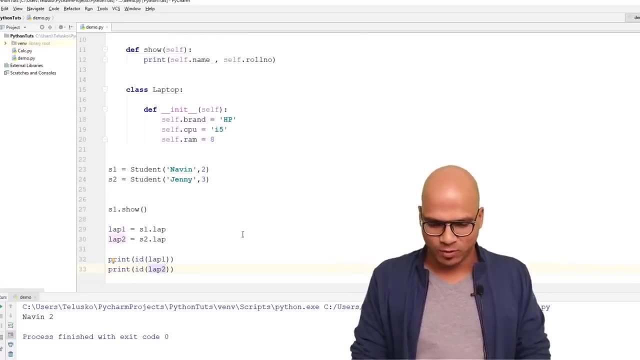 for every object you will get different laptop object. okay, trust me, this is how it works. in fact, you can also check that we got two different laptop object here. we will print lap1 and let's print laptop, so let's print the ids of lap1, lap2. we got two different objects here, so this works. 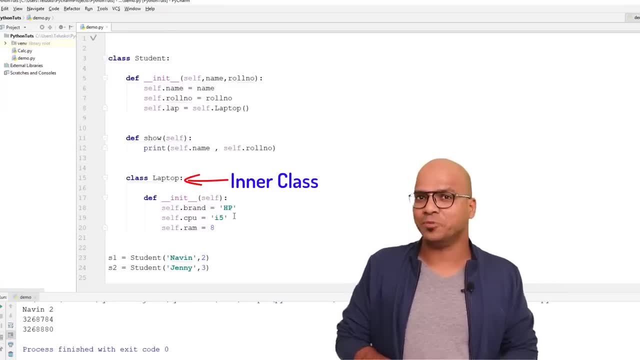 okay, this is where you create inner class. okay, so we have a laptop as an inner class of a student, right? uh, you could have done the outer class as well. i mean, you could have to do different classes, that even that works. but sometime, when you know that this class will be used only for student, 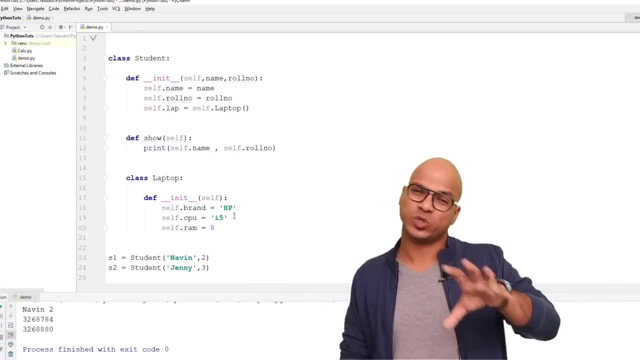 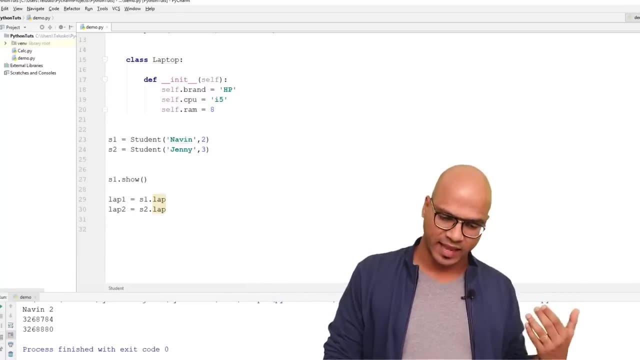 nothing else, then you don't have to create a separate file for that. you can do that in student class itself. now can i directly create the object outside? let's say, i don't want to get object of laptop inside the student class. can we do it outside directly? let's try. so i will say that. 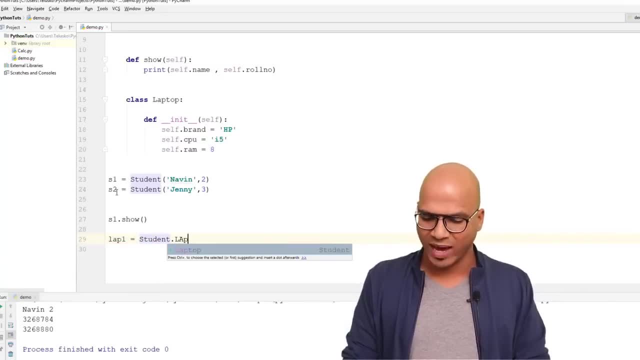 one is equal to, i will say, student dot laptop. now, why shouldn't here? because you cannot simply class, so we have to always say: student dot laptop constructor. you cannot simply create laptop directly, okay. so this is one thing you have to remember. you can create the object of. 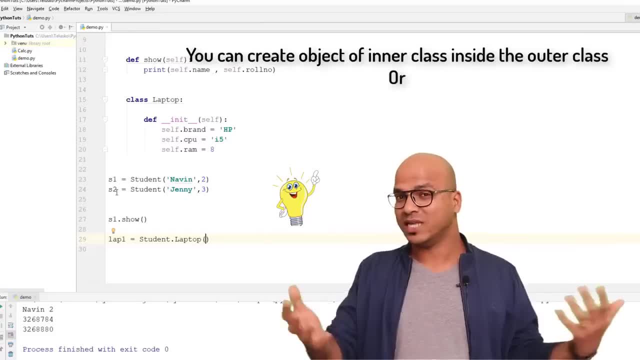 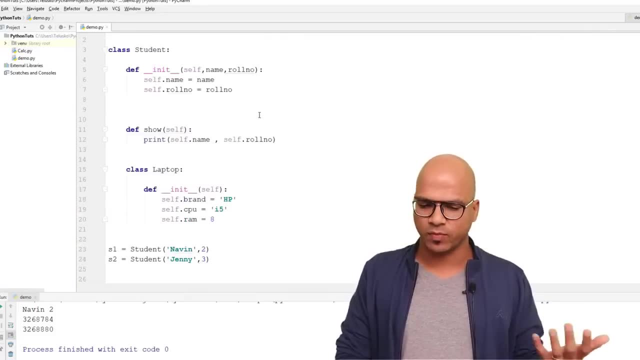 inner class inside outer class, or you can do that outside the outer class provided you are using the outer class name. so you have to say studentlaptop. okay, this works, in fact, just to enhance the example. what i will also do is we can create a show method for a laptop as well, so we can say: 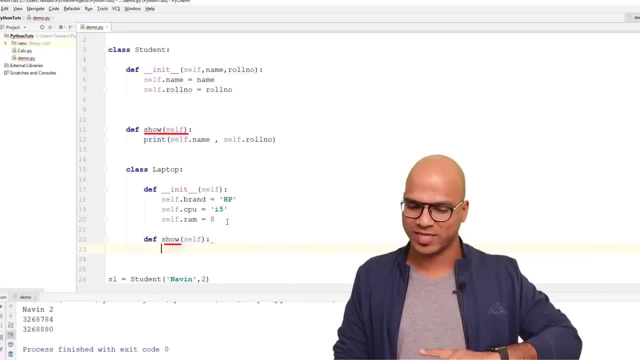 show for laptop and you can see we have two show methods. one is student and one is laptop. okay, so show method inside laptop also we have show, but these are two different show methods. the show method of student will print the data about a student and the show method of laptop will print. 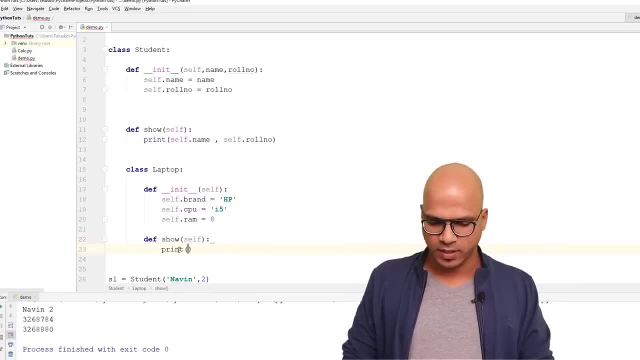 the show method of student. i know that makes that's weird, so let's do that. so i will say: print self dot brand, self dot cpu and self dot ram. okay, so we are printing this data. so this show is different from this show. let me now print laptop here. let me on this code and you can. 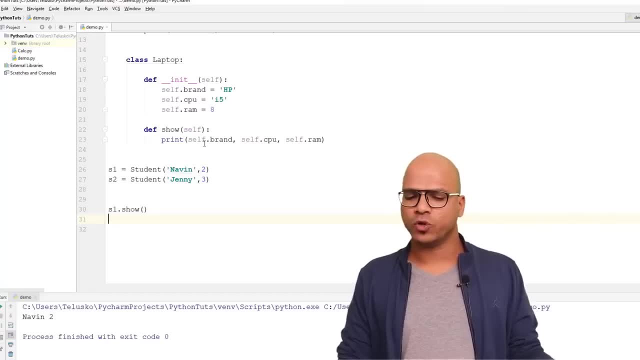 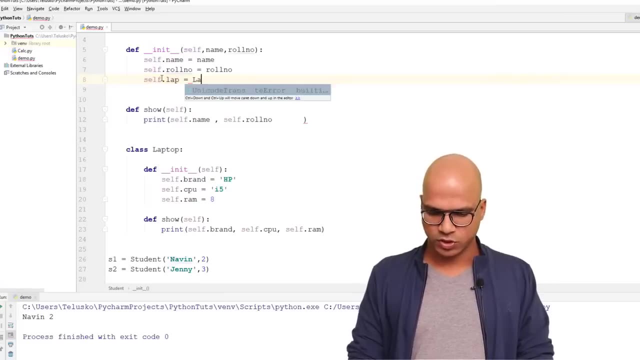 see it prints only the name and the roll number. i also want to print the laptop. you need the object right. we have removed that statement because if you want to access laptop, you have to say self. dot lab is equal to laptop, but you have to say self. so this is important and 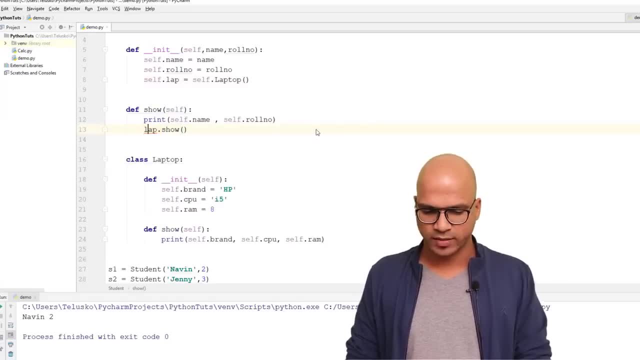 after printing this, we'll call laptop show, because we also want to do that, so we will say self dot laptop show. okay, so we are printing data about a student and laptop as well, so this should work. let's run this code and it worked. you can see we got data about a student and a laptop as well. 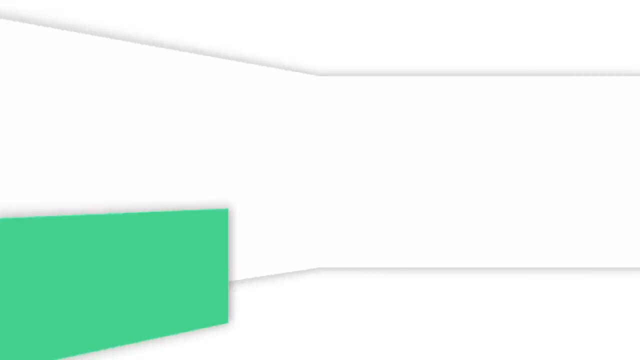 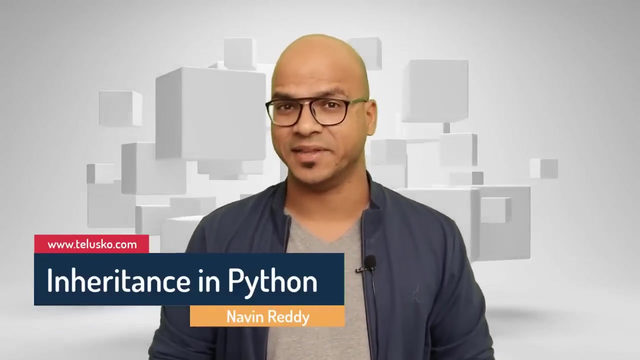 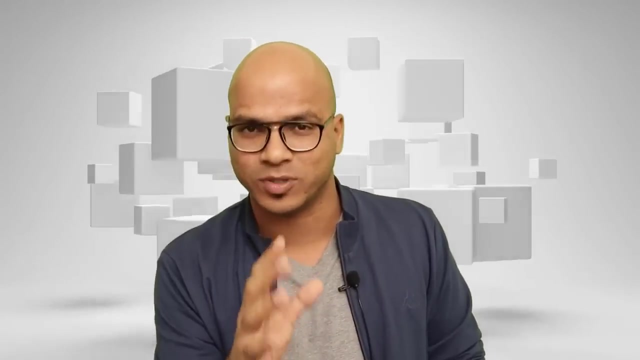 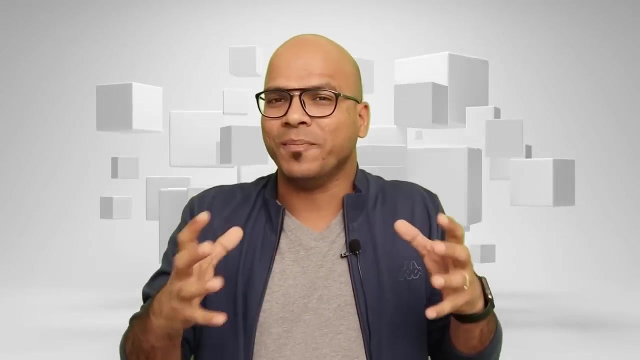 so this is how you create the class inside a class. now, in this video, we'll talk about inheritance. now we talk about a concept of oops, you know, which is object oriented programming. we have so many concepts to talk about, and one of them is inheritance. now, in real life, what we have is we have this parent and child relationship, right. so whatever, 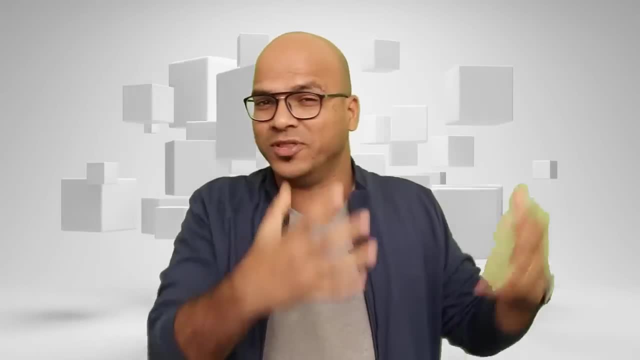 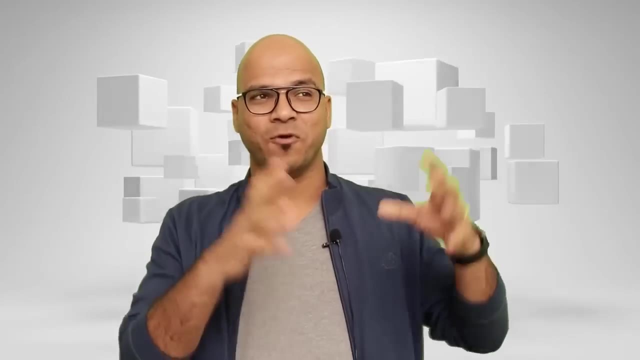 belongs to your parents belongs to you. example: if my father or mother has a phone, it's my phone, right? by default, my phone would be my phone, but my father's phone would be my phone, right? that's how it works. so if your parents house, it's your parents house. it's your parents house, it's your. 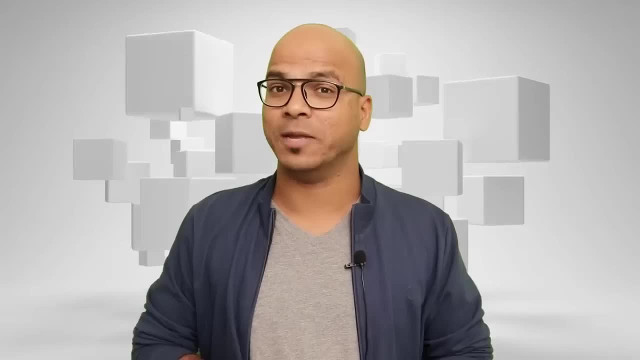 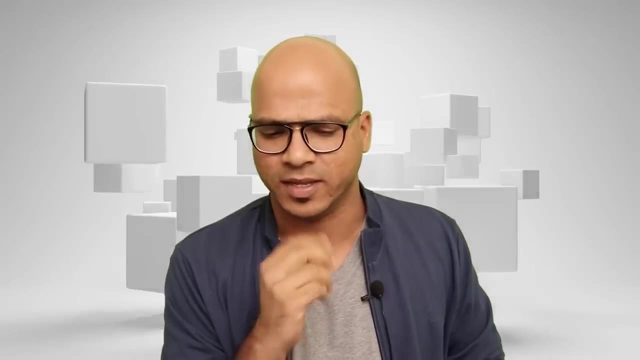 house. that's what we say: inheritance right, the same concept you can implement in programming as well. in fact, all the languages which follows oops concept, they do implement inheritance right, and the way you do that is with the help of classes. class inherit a class. let's try that. what i'm 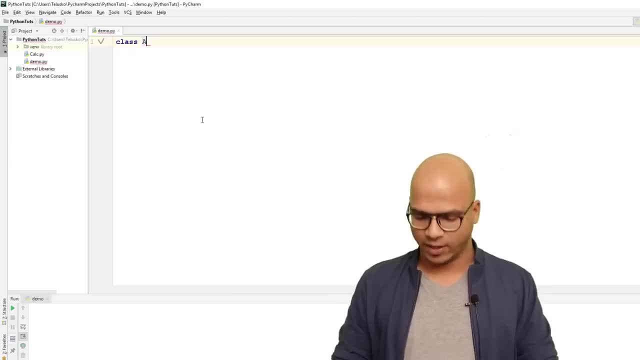 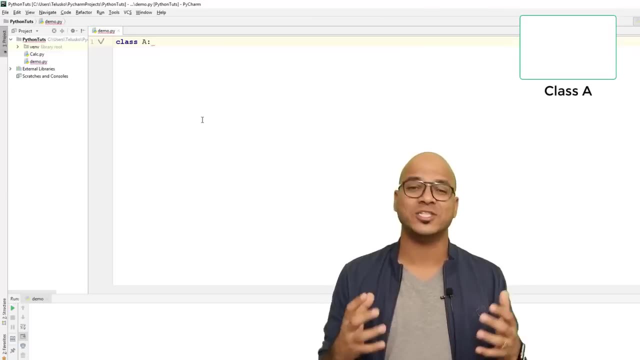 talking about is, let's say, if you have a class and class is a, okay again, it should be a logical name. so you can go with employee class, you can go with student class, you can go with laptop class, whatever class you love. but, time being, just for the example, we are going for class a. 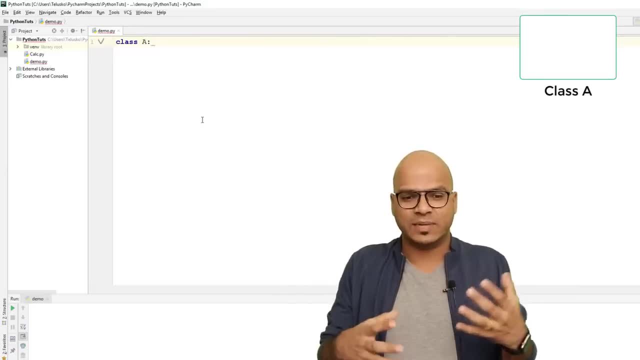 and class b or class c. in future we'll try to implement some other examples using different names and with proper example, but at this point, just to keep it simple, let's go for class a. now, if we talk about this class a, this class a will have multiple features. right? maybe we can define. 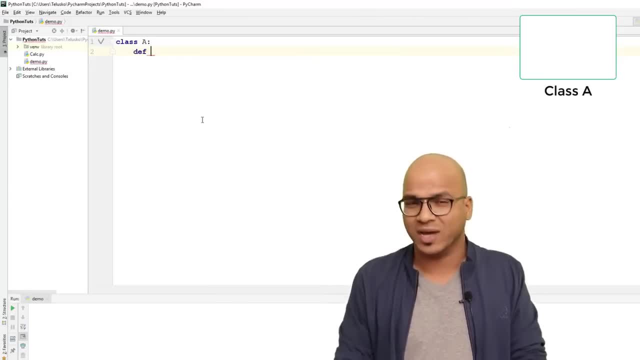 two methods here. so we'll say definition that the first method which i want to go for is, let's say, feature one. okay, so let's say we got this function, which is feature one, and this function does provide you something. okay, so time when we are printing, feature 1 working, that's it, nothing much. 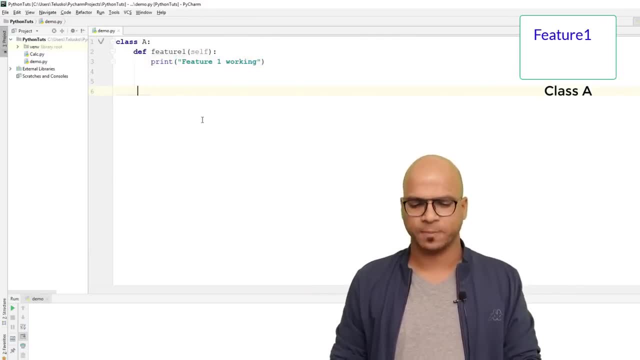 of course it can be a complex code, but make it simple. let's keep it that, and then we can have another feature here. let me just copy paste this code. so i will say copy and paste, and this would be my feature two. so we got feature one and feature two, and this will point. feature two is: 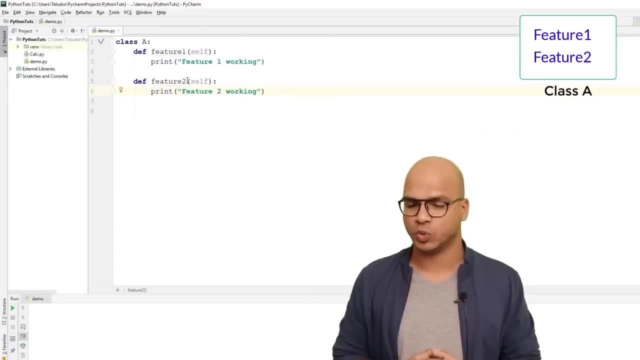 working. so this class a has two features. we got feature one, feature two right, and the way you can access them is with the help of object right, and the way you create an object is very simple. you simply say a1 is equal to a. that's how you create the object right, where a is your constructor again. 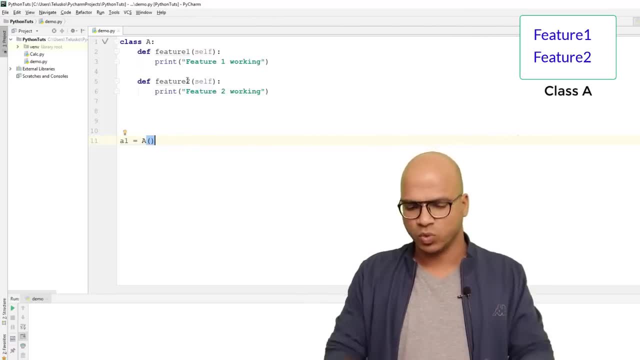 you can find that init method here, but not needed at this point. so this will work and using this a1 you can call feature one, you can call feature two. right, so you can say a1 dot feature one and a1 dot feature two, and this will work. let me just run this code and you can see we got feature. 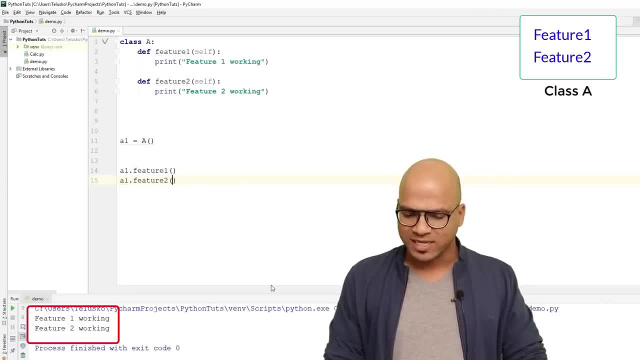 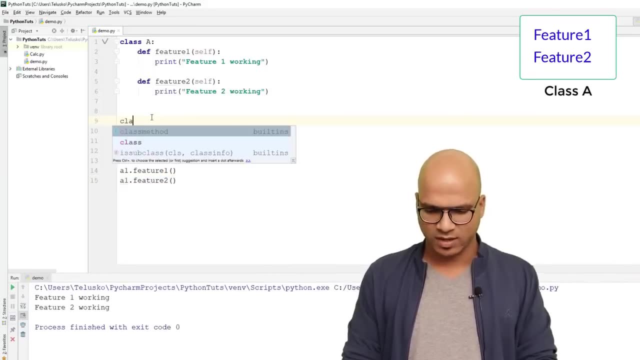 one working feature, two working. so this code is working. now what i'm excited about is: let's say, we have one more class, let's talk about class b. so let me just create a class b here itself. so here i will say class b, and class b will also have two features. i will name this as feature. 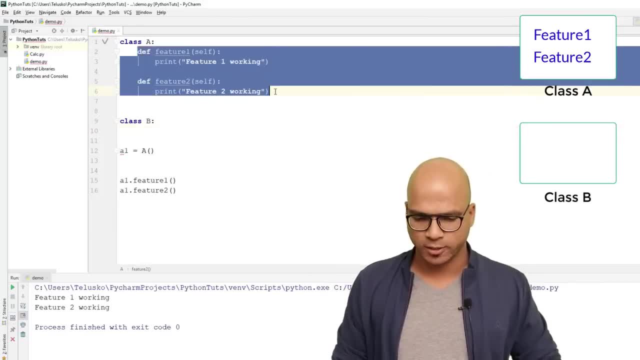 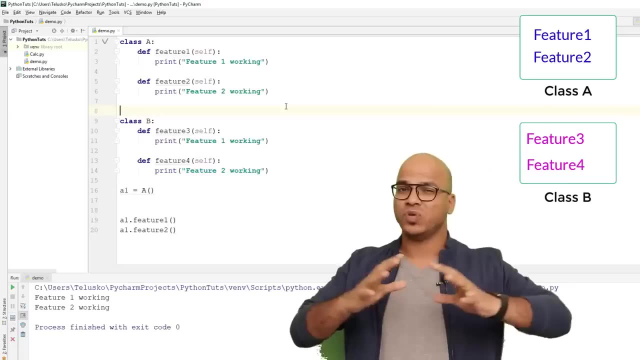 three and feature four. instead of typing them, let me just copy paste the code here and we'll name this as feature three and feature four, right? see normally what happens, you know, when you work on a project. of course we have a very big team, right? so example: if one person is defining a class, okay, in 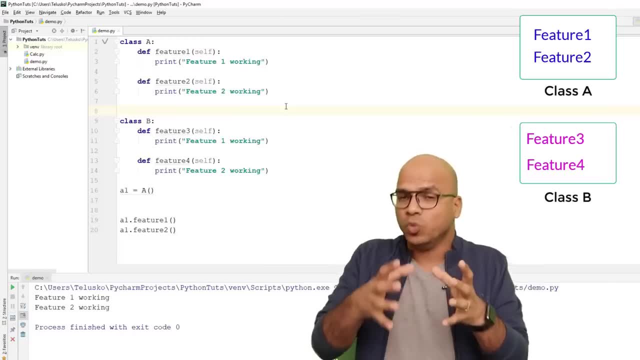 that class. we provide you four features or four methods. maybe you want to define some other class in which you need some extra features and you also want the existing features. you don't have to redefine it right, you can use it, and the way you do that is simply saying example in this class b, 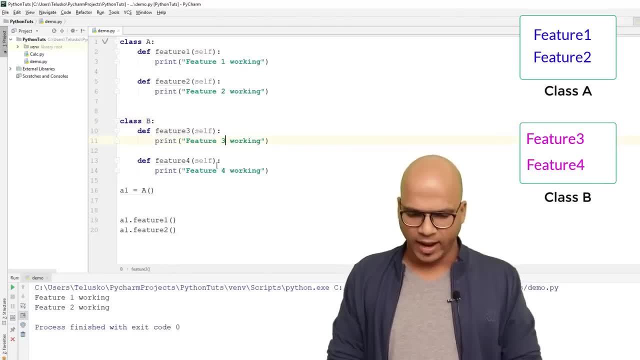 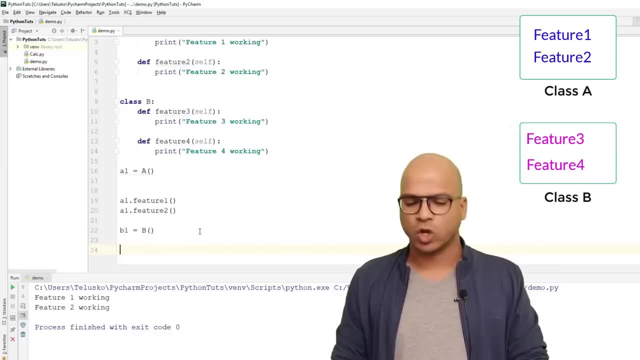 we got two features right. we got feature three, which we got feature four and, of course, if i create the object of b1, so b1 is equal to b, and the functions which you can call using b1, so if i say b1, dot, you can see we got only two options. we got feature three and feature four, of course. 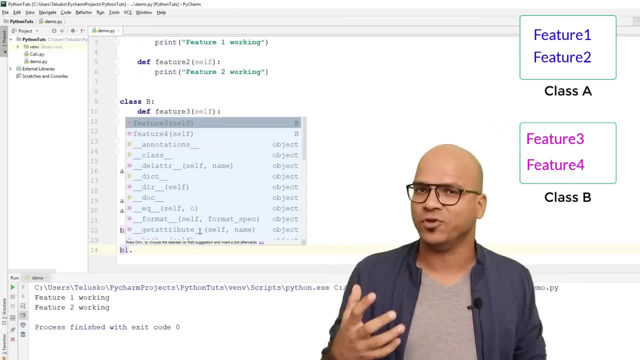 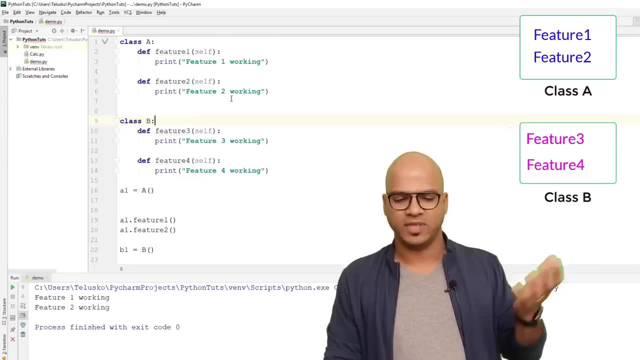 right, because in b class we have only two features. what if you want to get the features of a as well? and that's where inheritance comes into picture. so we can say, hey, this b is a child class of a, and the moment you say child class, it will import all the features. so what i will say is this: b is a. 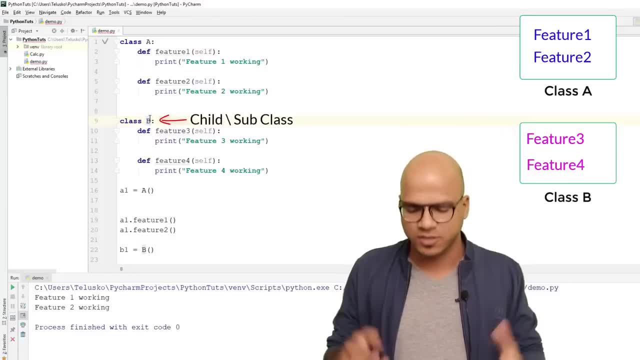 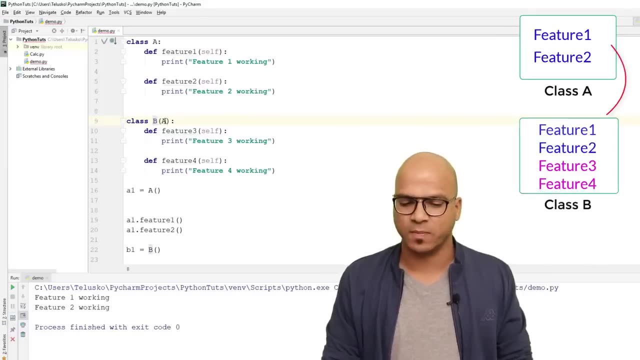 child class or you can say subclass. we have different terminology we can use here and we can simply say: in the bracket you can say a. so this class b is inheriting all the features from a and we got it right. just writing that one thing you know. just bracket a, we are saying b is inheriting. 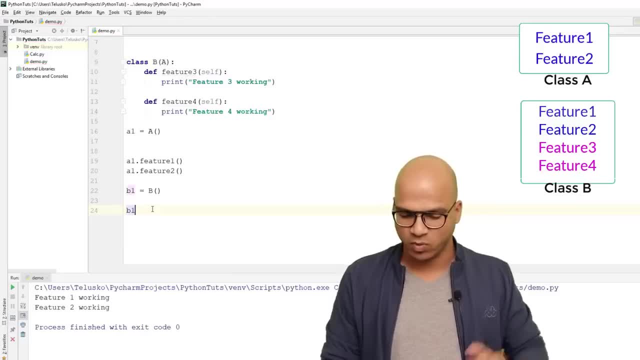 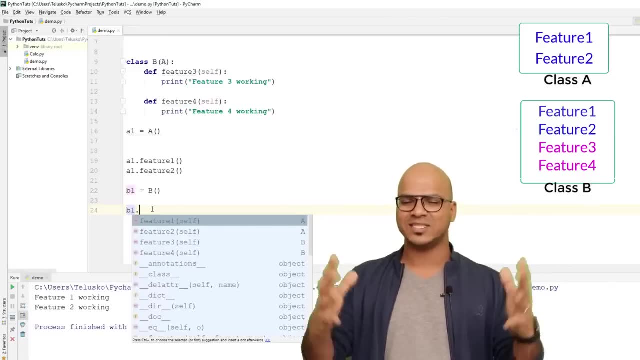 the features from a, which means with the object of b, which is b1, in this case, the moment i say b1.c and b2.c, and b3.c and b4.c, and that's the importance of inheritance, which simply means if you already have a class which provides you some feature, and in future, if you want to create, 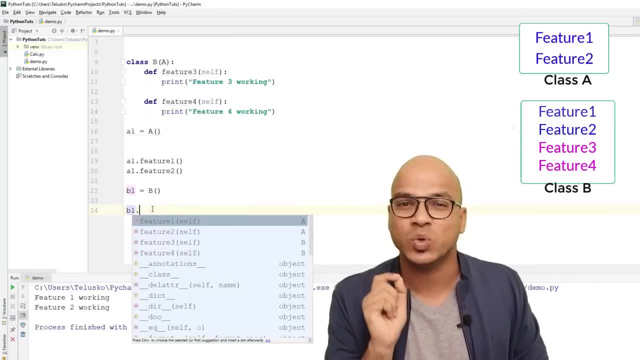 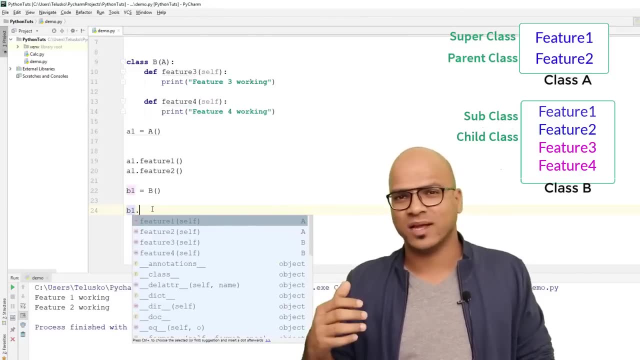 your own classes in which you want to use those features. you just need to inherit them, right? so we can use some terminologies here. we can say superclass, subclass, or we can say parent class or a child class, so time will refer them as superclass and subclass. so super is a class. 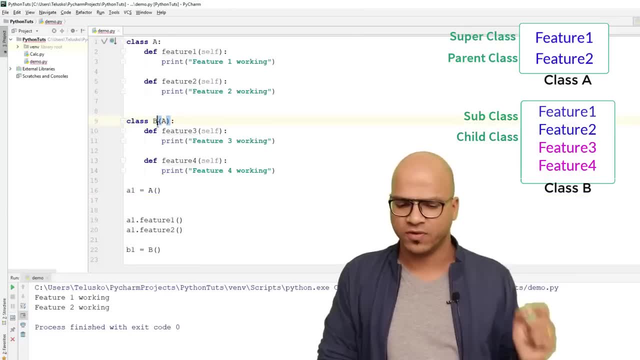 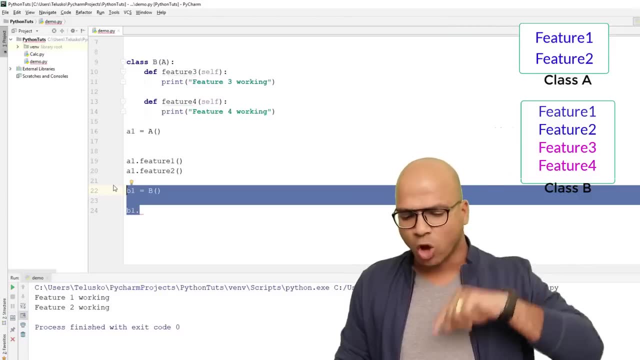 which is a, and a class which inherits the class. we will call them as subclass. so b is subclass and a is superclass. so that's the concept about inheritance. now this is also called as a single level inheritance. we have some other types as well. we also have a multi-level. 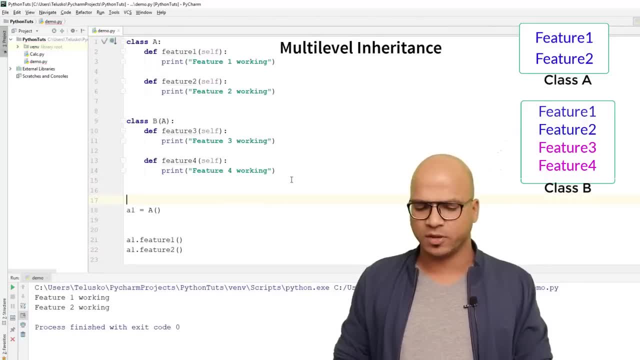 inheritance. now what it means. example: let's say: if i have another class here, let me create one more class here, and this class is, let's say, c, so we'll call this class c, or this class c inherits b. now what will happen is: whatever you do in this class, let's say time bin, i will define only one. 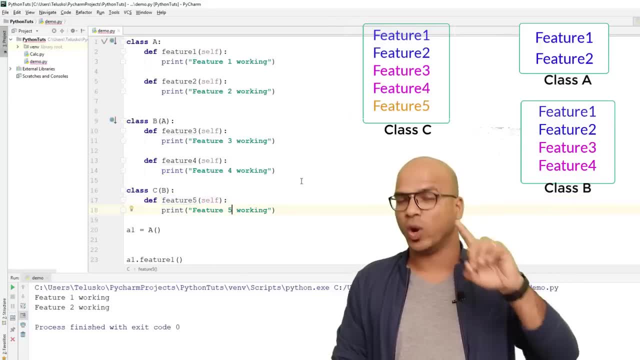 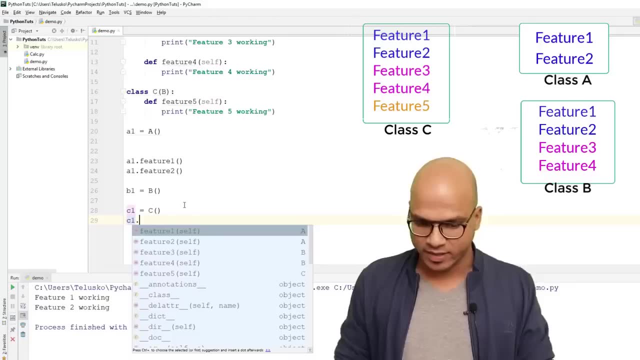 so this is feature five working right. so we got c class, which has only one feature. but the moment you create a object for c1, so i will say c1 is equal to c. the moment i say c1 dot. see the methods you can use. so we can use feature one. now. feature one, feature two are coming from a right, but c is 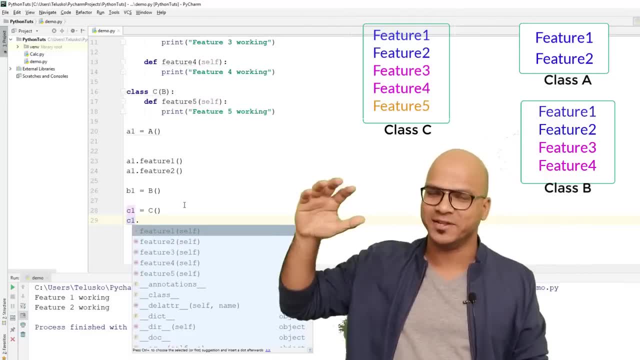 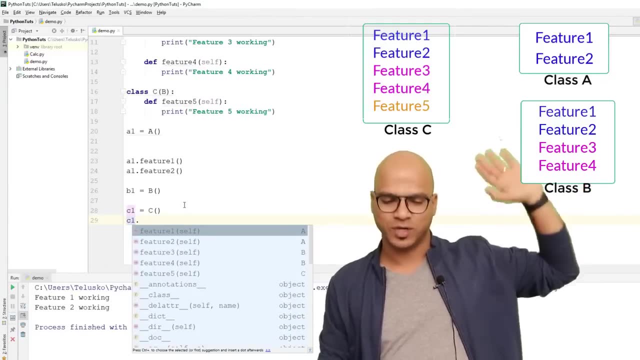 only extending b. so that's relationship: we have grandparent, we have parent, and then we have child, right? so a child can access all the features from parent, grandparent, great grandparent, right? so that's how it works. okay, this is working right. so we got single, where you have one superclass. 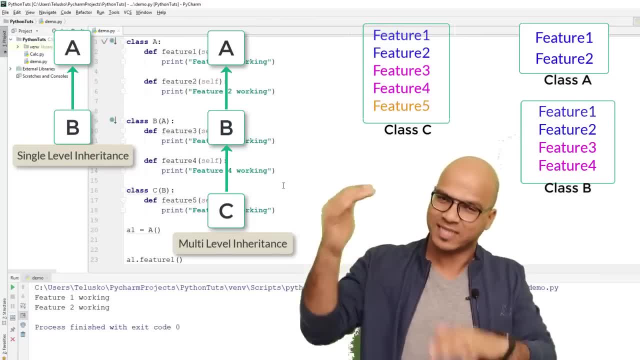 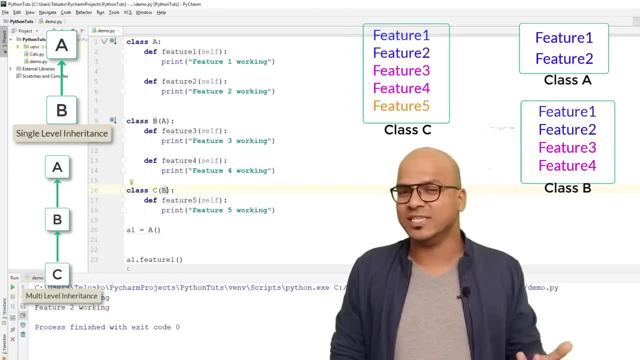 one subclass, then we have multi-level. when you have superclass subclass and then i get surplus of that superclass, okay, this is working. what if you go for multiple? what is multiple here? let's say the c is not only taking from a and b, we got some other class as well, just for time being. what? 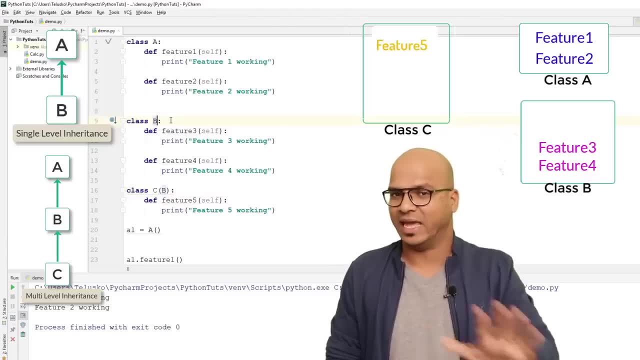 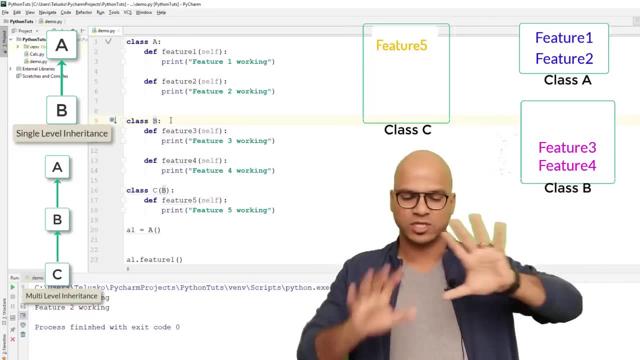 i will do is i will say b is not inheriting a. okay, so a and b, they are two different classes, nothing, they are not related to each other. a provides two features. b provide two features. okay, so there's no relationship between a and b. there are two different classes. c says i want to access. 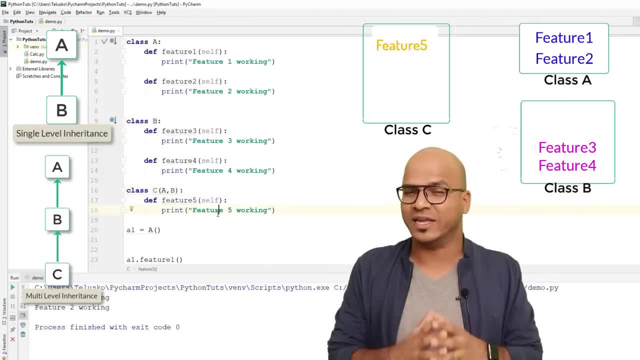 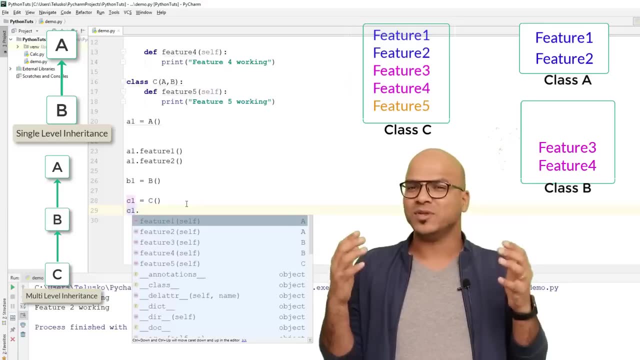 features from both, from a and b. so in this case, so c will inherit from a and b, both, so you will say a comma b, so c will copy from both, or c will inherit from both, so we will say c1. the moment you say c1, you can see you can access all the features. that's not the case with b1. now b1 can only access. 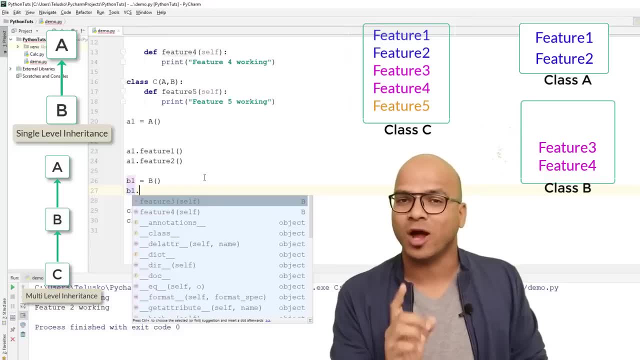 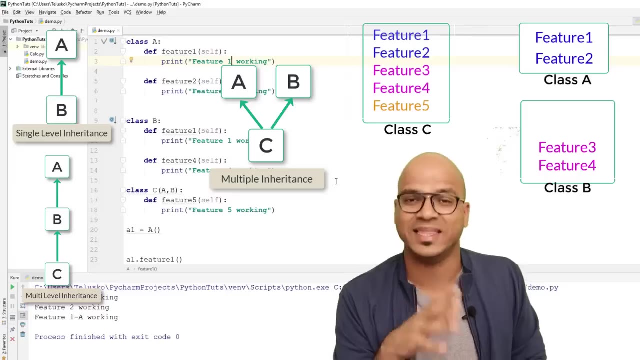 two features: feature three and feature four- because b is not inheriting a. okay point, remember. so we got a, we got b and then we got c. c is inheriting both the classes a and b. so this is how we have done with single, we have done with multi-level and then we have multiple. so this: 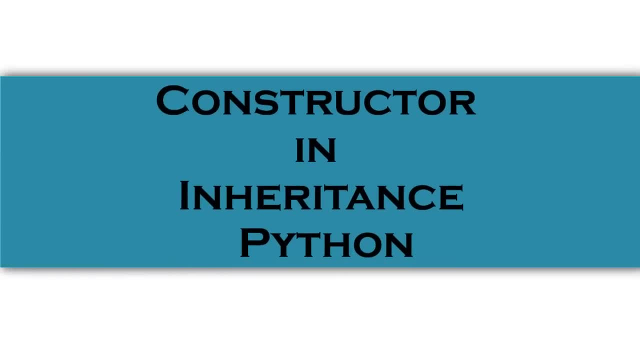 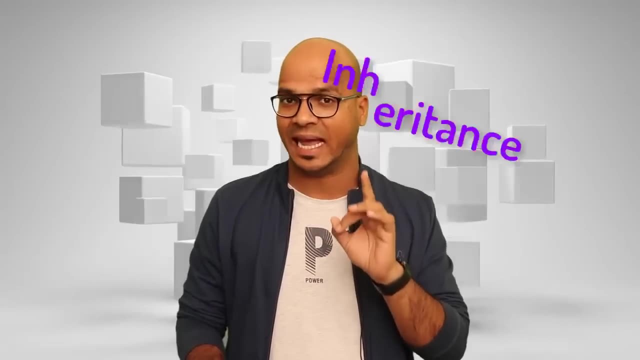 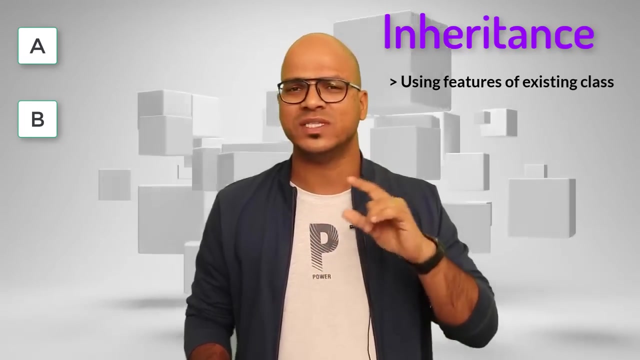 is how we can work with inheritance. now to this point. we have talked about oops concept right, in which we have seen inheritance. right now, what is inheritance? if you already have some classes and if you want to use the existing features, you will simply say class b, which will take the 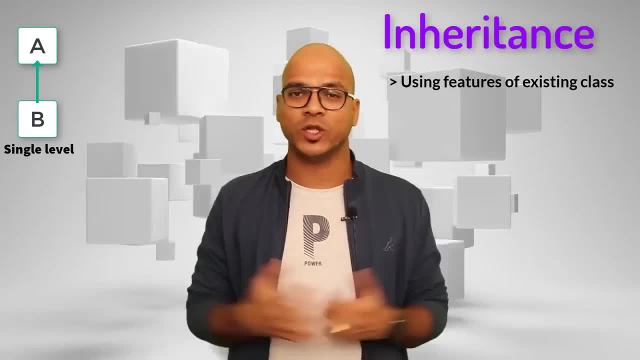 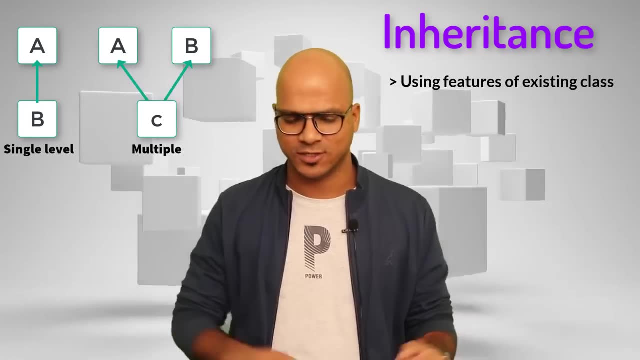 features from a. right, so class b inherits a. or you can go with a concept of multiple inheritance, where one class will extend from two different classes or more than two classes, right? so in this case we have class a, class b and then we have class c, which 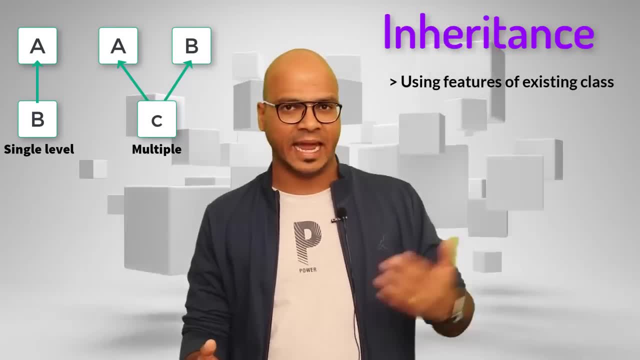 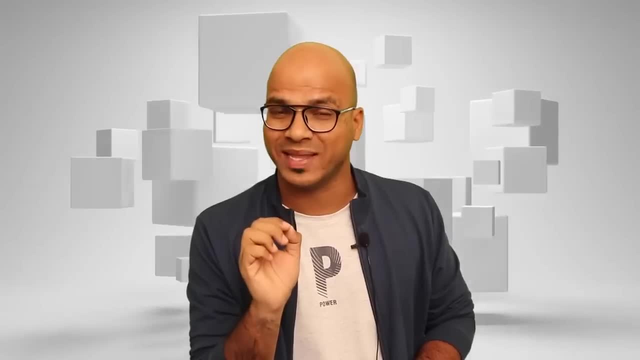 is print which has a feature five, but it is also inheriting a and b, so we can say: c has five features, right, so that makes sense. now what we'll do in this video is we'll talk about two topics. the first one is the constructor in inheritance, how it behaves, and we'll also talk about method. 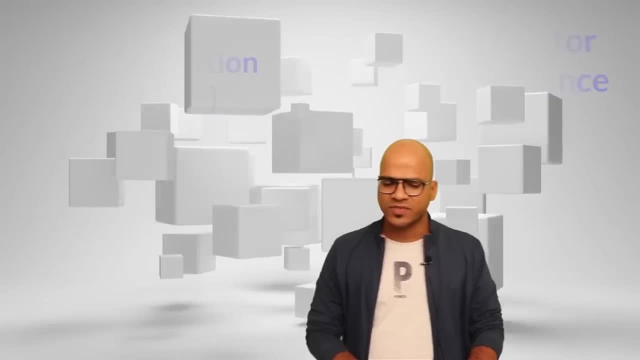 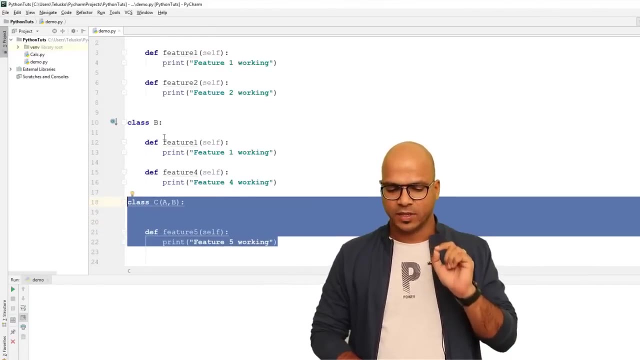 resolution order. or you can say, mr o, so let's start with the constructor time bin, let's ignore c. okay, so let's say we don't have this c, so we'll ignore that part and in fact we'll delete that part from for time bin and let's focus. 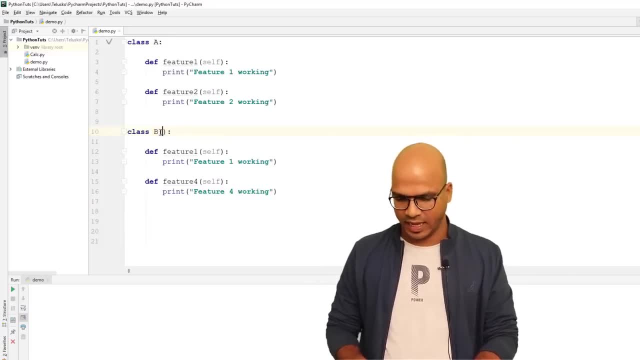 only on a and b, where b is inheriting a. okay, so in total, in b we have four features. right now what happens is if i create an object of a. so let's say, if i say a, 1 is equal to constructor of a. so this: 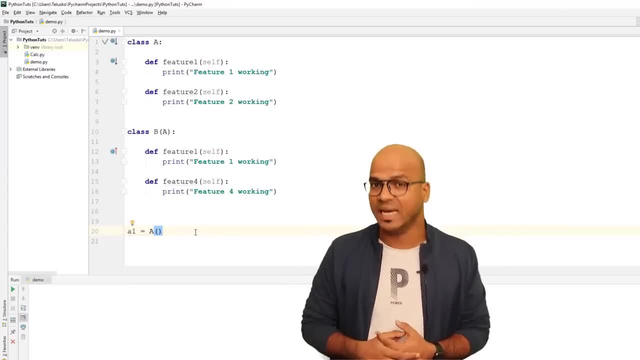 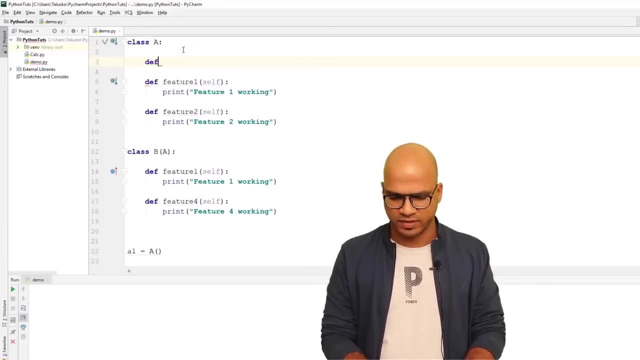 will work right. so when you say a bracket, that's a constructor, it will call a method which is in it, define it. it is there somewhere, right. but let me define my own constructor on init here. so i will say def and we'll define the init method and this init method will print one stuff. so let me say: 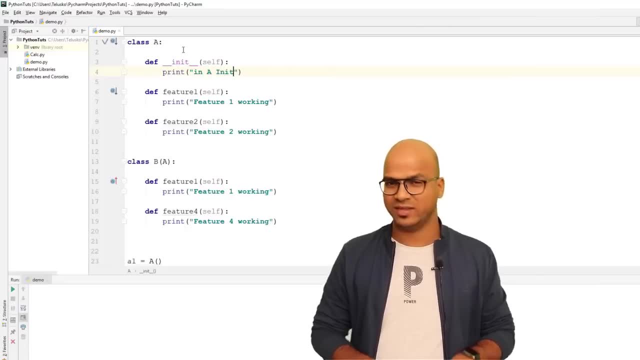 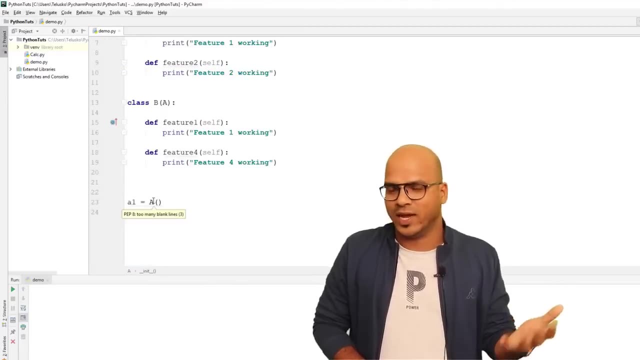 print in a in it, nothing much. we are not doing anything extra here. we are just printing in a in it, that's it now. what do you think what it will print? of course we are creating object of a right, so it will only execute a see with the object of a. you cannot access features of b, okay, 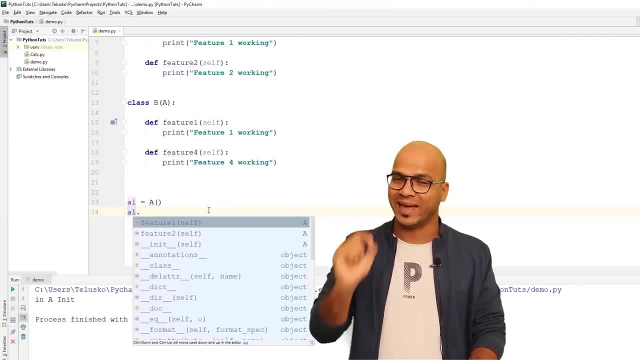 so even if i try, example, if i say a, one dot, you can only access feature one and feature two. but yes, if you have an object of b, you can access all the features- right features- from a and b, because b is a subclass and a is superclass and, as i mentioned, subclass can access all the 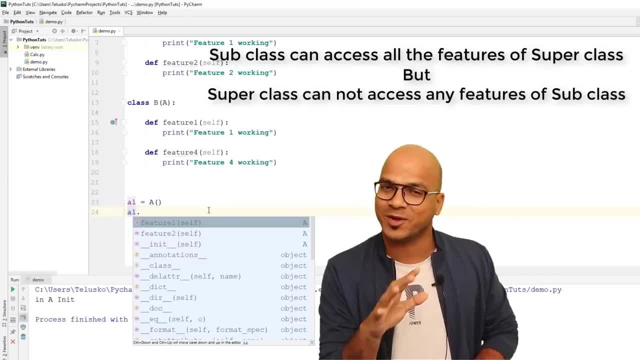 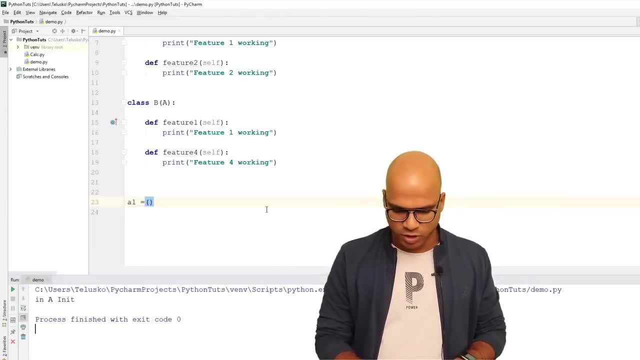 features from superclass. but that's not vice versa, right? a superclass cannot access all the features of subclass, not even one feature of subclass. okay, this is fun. now what if i create object of b? so i'm not getting object of a, here, i'm getting object of b. doesn't matter what is a1 or b1. 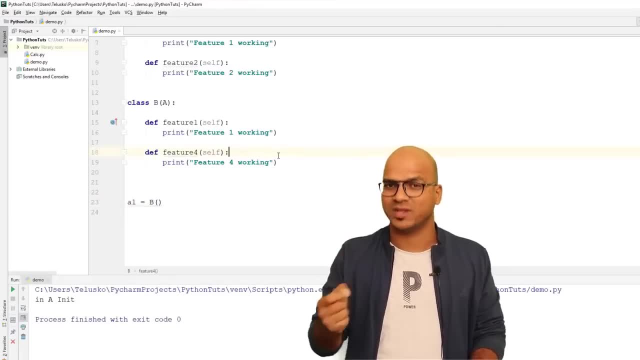 important is: if i create an object b, will it call the constructor? that's the question, because we are not getting object of a, we are getting object of b. will it call the constructor of a? that's the question. let me just run this code and it works okay. so even if you have the object of b, it will. 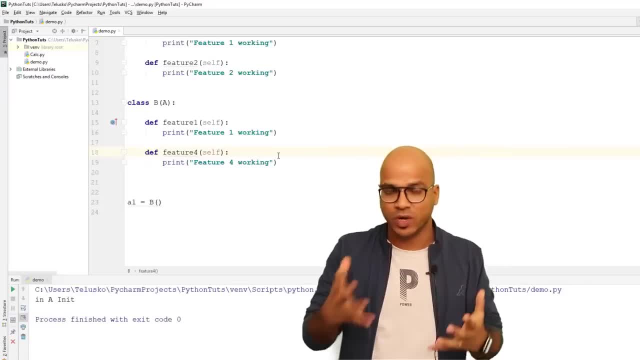 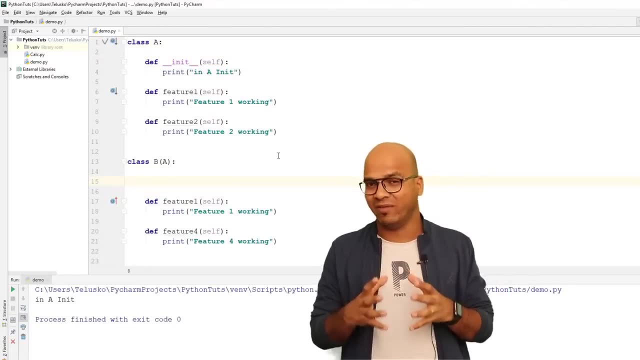 still call the constructor of a right. that's how it works. but what if you have your own constructor? what if you have your own init method? example in bc, in b, we don't have that in it, right, and that's why it's going up. so let me repeat: since we don't have in it inside b, that's why it is going to a. 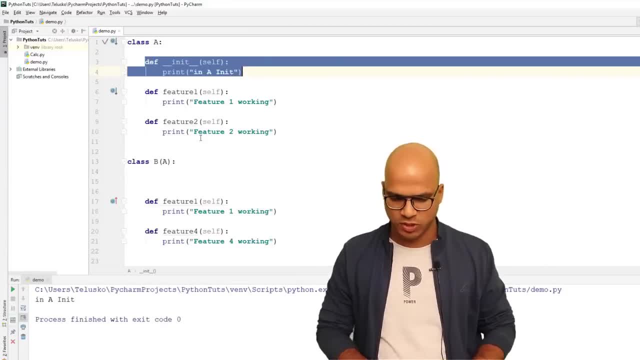 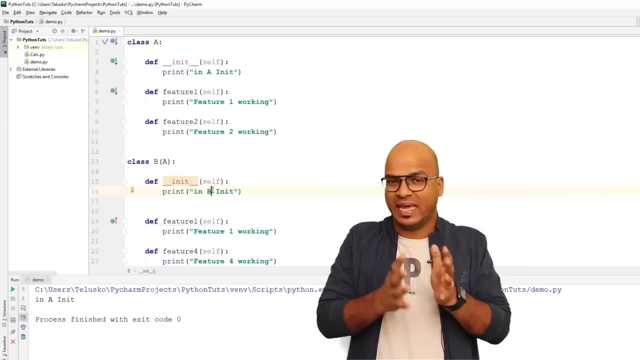 but what if you already have a in it with you? so i will simply copy paste here in b, so both have in it. but then in this i will print in b in it. right? so in a we are printing in a in it and b we are printing in b in it. so this makes: 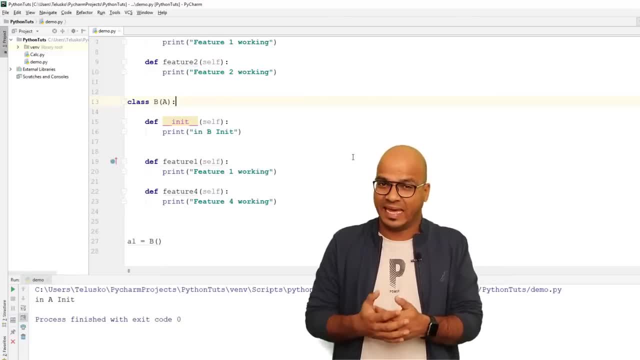 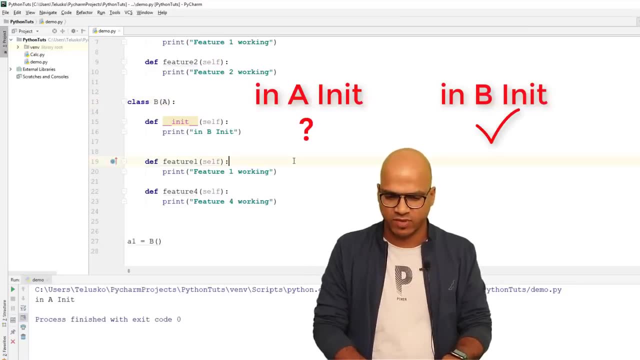 sense. now, what if i run this code? what it will print it? will it print in a in in it or in b in it? of course, right, if you are getting object of b, it should only call the init of b, right? and let's see if that works. and let me run this code. and we are right. so when you run the code you can see we. 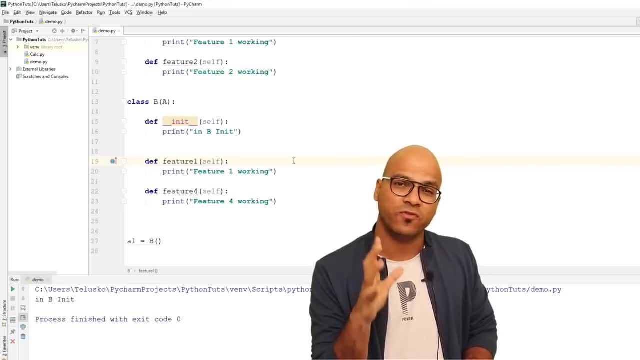 can see that the in it of b is going to be the in it of a right. so that means if you create an object of b, first it will try to find the init of b. if it is not there, then it will go for a. okay, that's the point you have to remember. but what if you also want to call the init of a is? 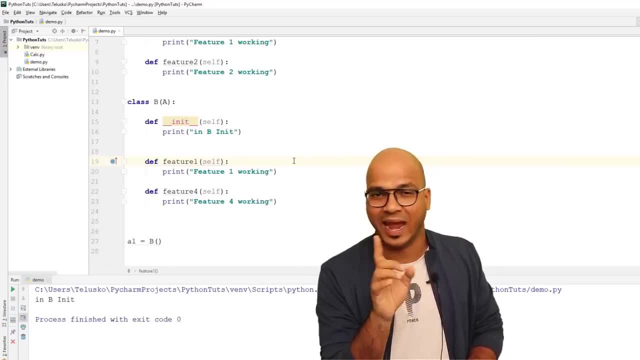 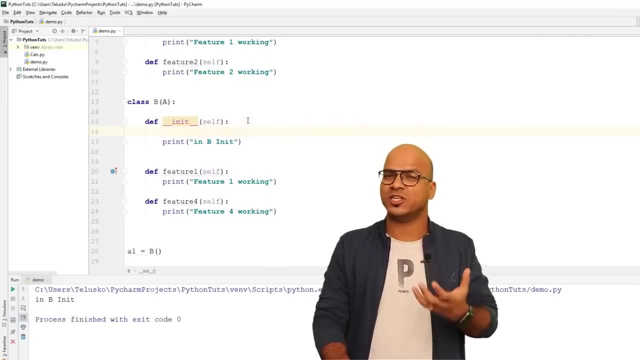 it possible? i mean, if i create object of b, can i call the init of both the classes, i mean a and b. see, by default it will call only b, right? what if i want to call a as well? and that's where we have a. so with the help of super, so you can say super and it's submitter, basically. so you will say: 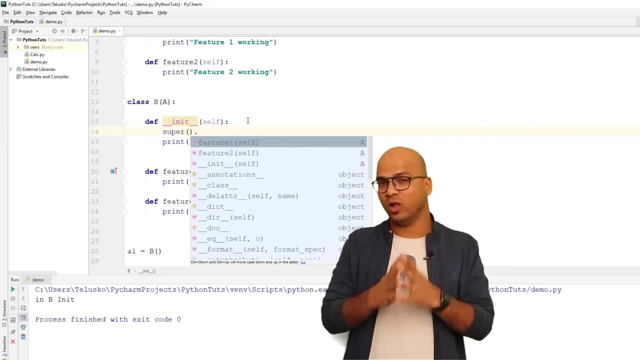 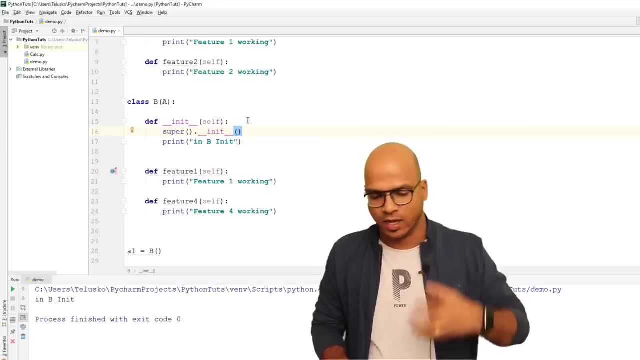 super dot. the moment you say super, you can access all the features of the parent class. so it gives a super dot in it. so what we are doing is we are trying to call a init method of class a. so the moment you say super, you are representing the superclass okay, which in this case it is a. so 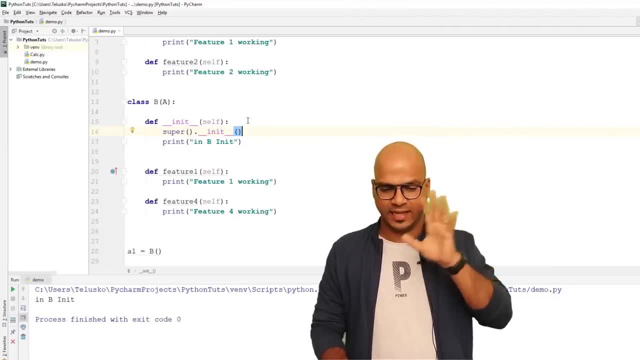 we are trying to call the initial method of class a. that's important. and now let's run this code and you can see we got both the output- we got in a- and the height of the project and we are trying to say the order of the class. the only union which represents the class a is called the init method. 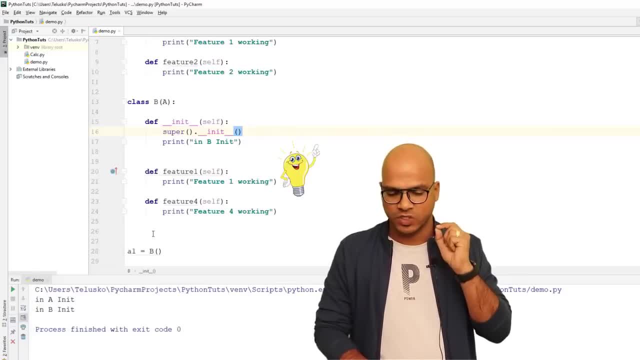 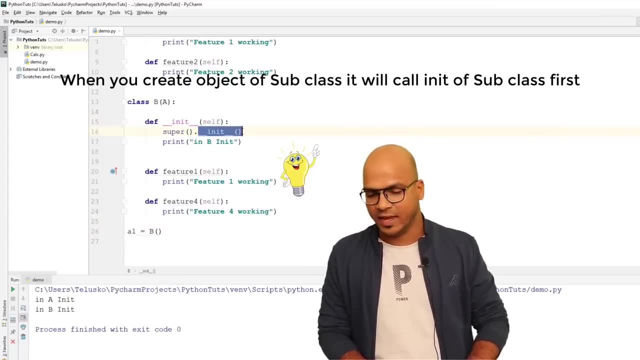 and we got in B int. So point to remember is when you create object of B, it will call the init of B first and then from the init of B you're trying to call the init of A, So it will jump up, it will. 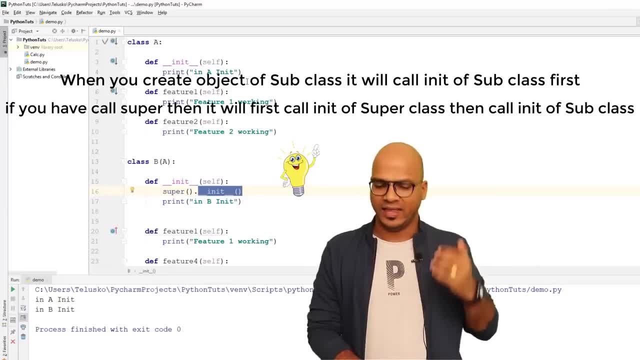 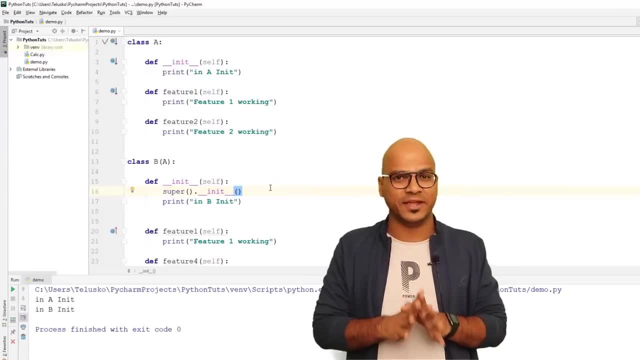 execute the init of A first, which will print in A init, and then it will come back to print in B init. Okay, that's why we got the output. So this makes sense. So we can work with constructor in inheritance. right Now let me add a twist here. So what I will do is I will remove this super from. 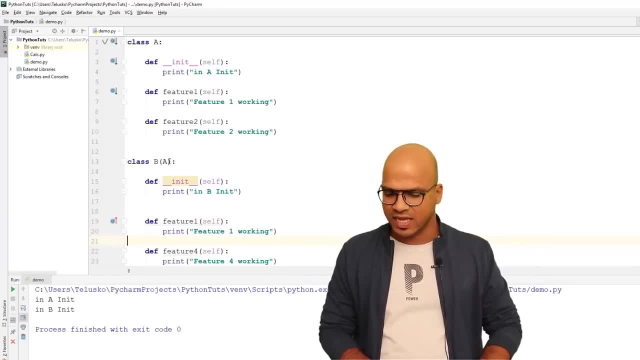 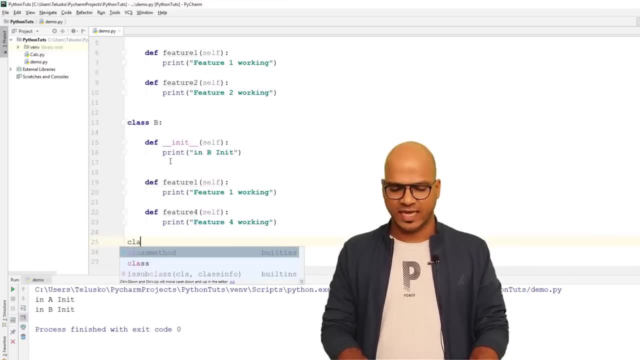 here, Let's clean it, and I will not even say that this is B. So class A and class B, two different things. okay, They're not linked with each other. But then we have class C, As we have done earlier. 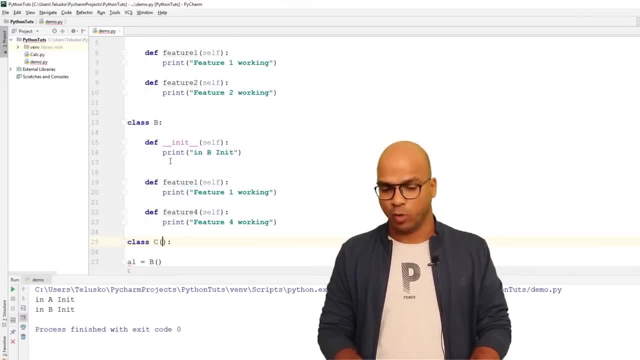 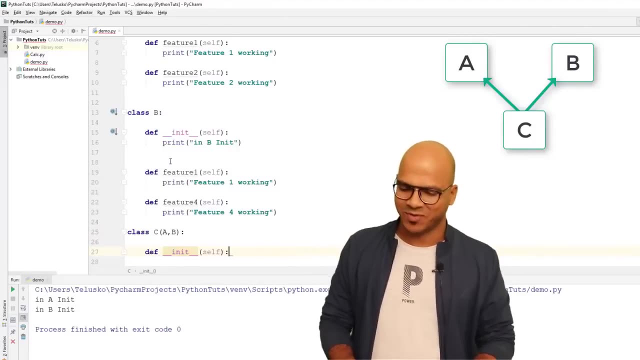 we'll say class C, and class C will inherit both the classes A and B. okay, And now, if I say def and init, you know right what we're trying to do here. First of all, we'll print in C init. 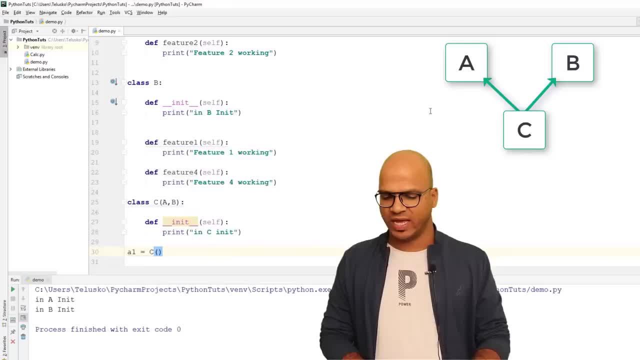 okay, And then I will create object of C. So there's no object of A and B. I'm trying to object of C. Now, what do you think? Will it call the init of C, or A or B? Of course, right. When you say the object is of C, it will call the init of C. only. Let's run this. 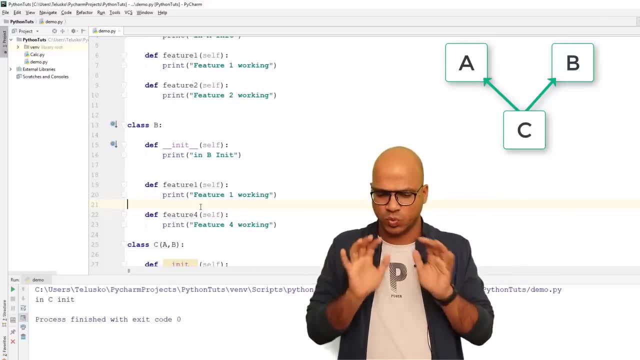 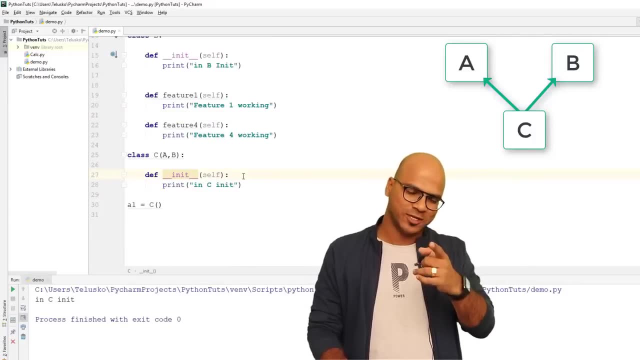 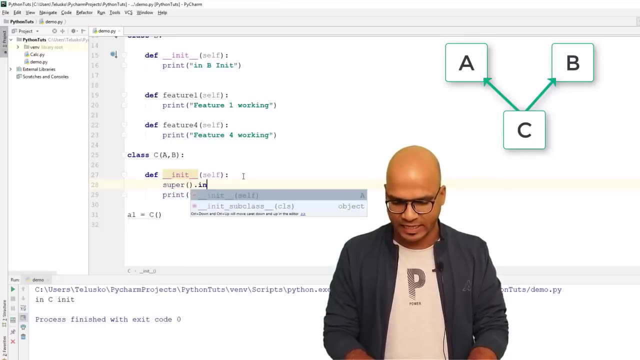 code. And that's right. We got the output as in C init. So this works perfectly. But what if you want to call the init method of a superclass? But there's a twist here. Now C has two superclasses. one is A and B. The moment you say super dot init. 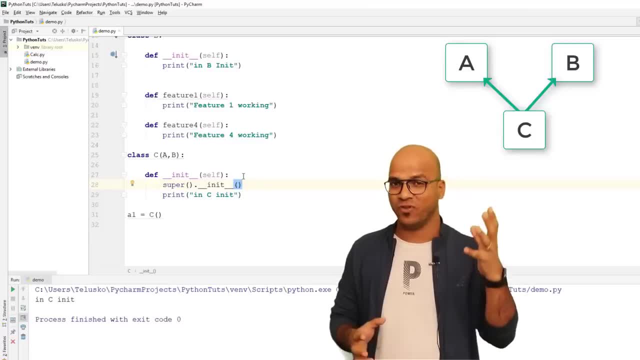 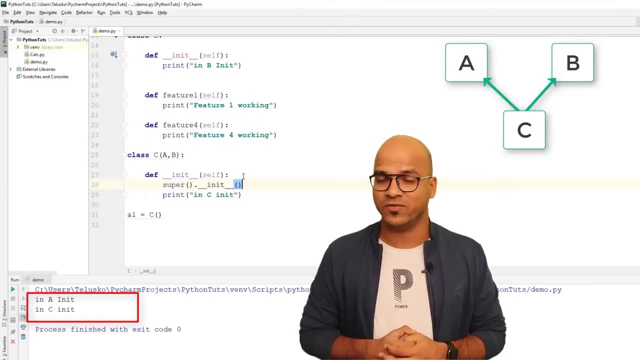 now, what do you think Which init it will call? Will it call the init of A or B? That's a question. Let's run this and let's see what happens. The moment you run this code, you can see it says in A init. That means we are unfair here. We are biased towards A. We are not taking B here. 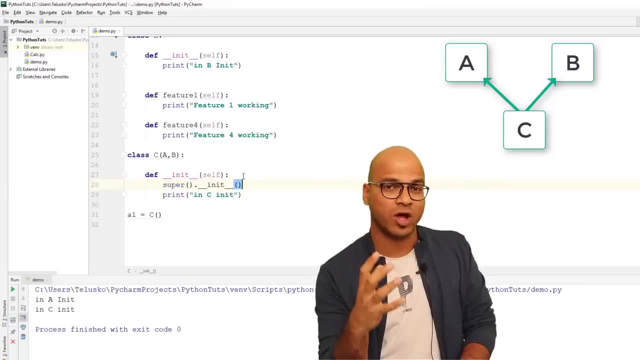 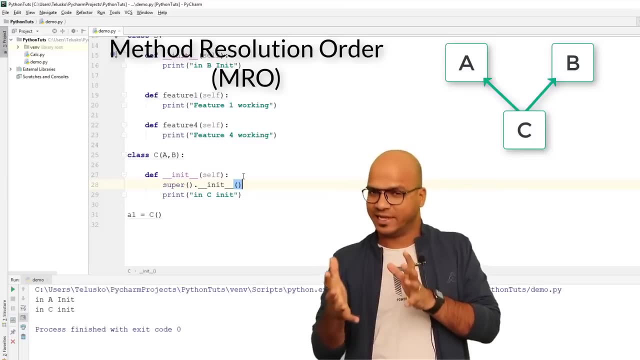 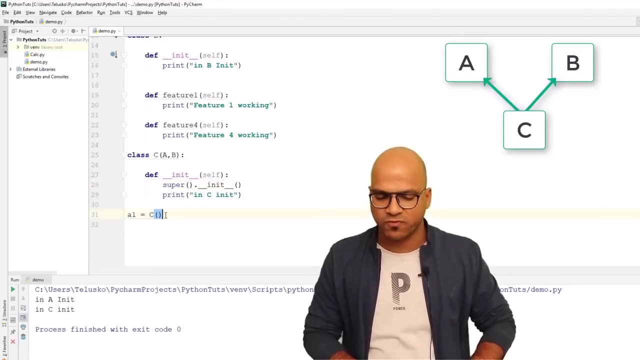 right, This is completely wrong. But the thing is we have a concept of MRO, which is method resolution order. So what happens is, whenever you have this multiple inheritance, it will always execute the init of C, So first. so the moment you say init, it will try to find the init of. 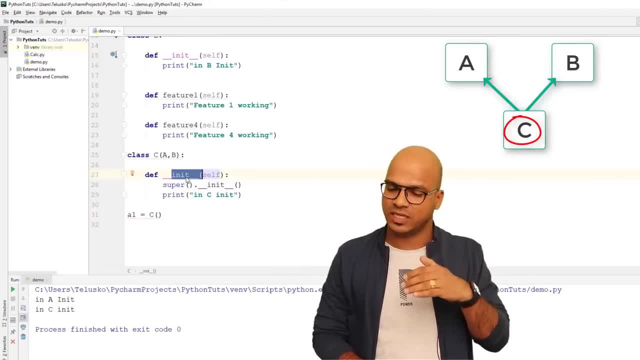 itself. So since we have init here, it will execute the init of C Then the moment you say: super dot, init. now we have two classes, right, A and B, And on the left-hand side we have A and on the right-hand side we have B. So it will prefer left one first. So it goes from left to 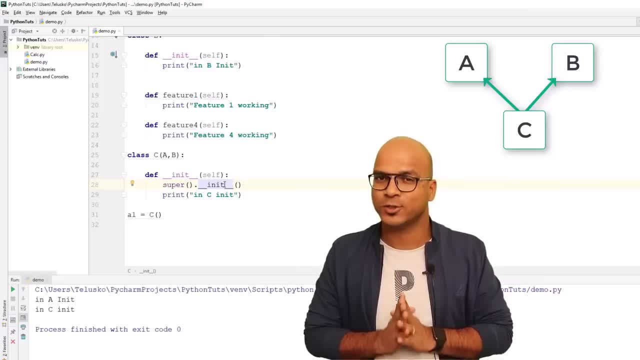 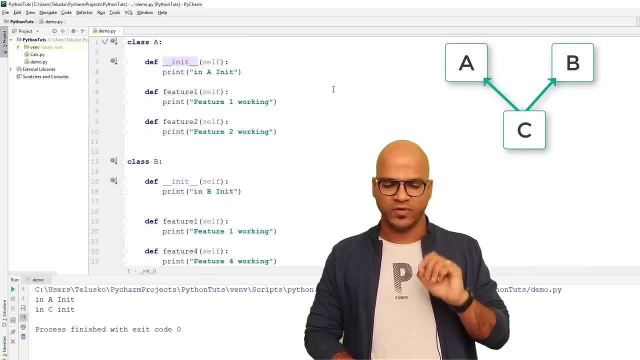 right, And that's something you have to remember. It's always from left to right, okay, And that's why we got in A init. The same thing can be done for methods Example. let's say we have two methods which are the same. So in this case you can see we have feature one in A and 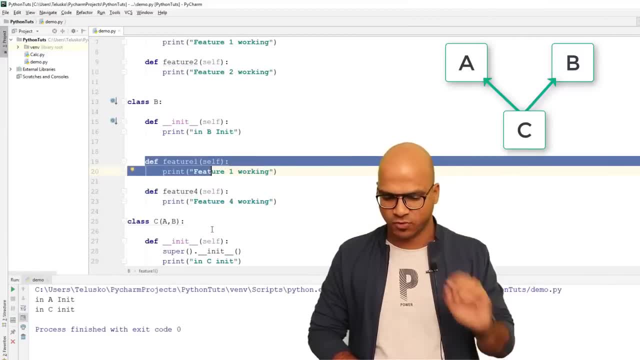 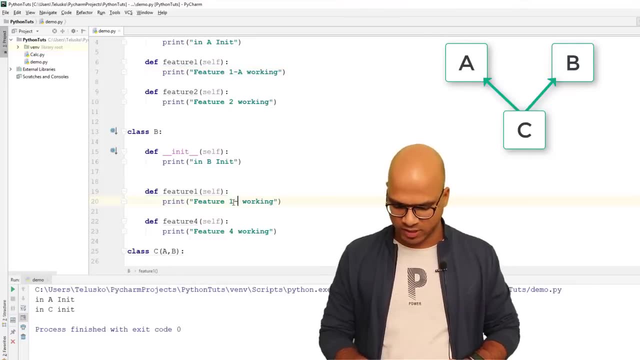 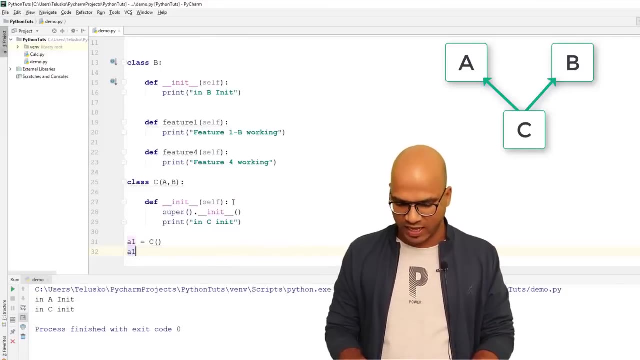 feature one in B. Both are the same methods with the same name of course, And in this I will print some different message. Here I will print feature one A and here I will say feature one B. That means the feature one is in A and feature one is in B. And now, if I try to call so, I will say: 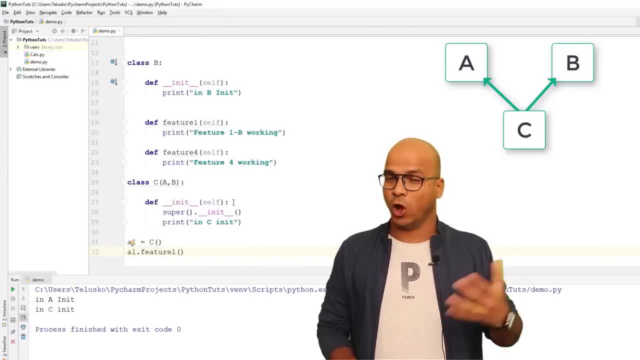 A1 dot feature one. will it call from A or B? That's a question and we know the answer. right, It will always call from A, Because it goes from left to right and you can see the output. So this is something you have to. 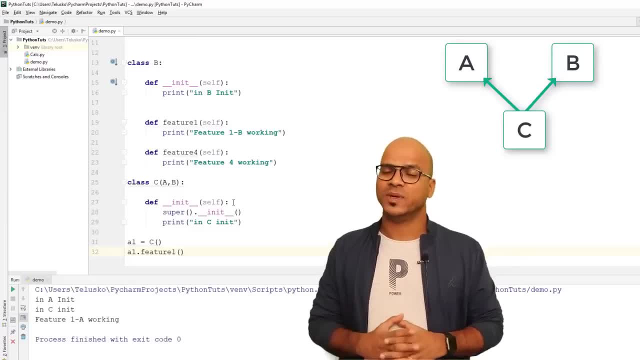 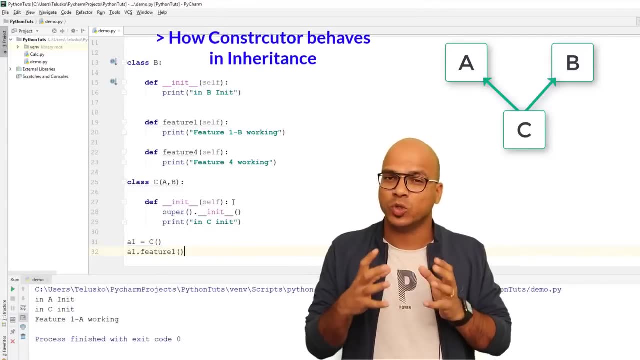 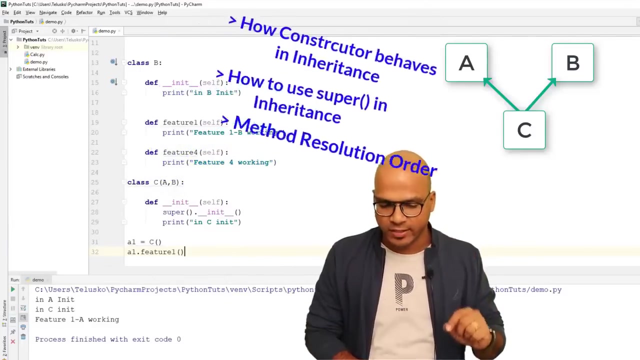 remember, which is the concept of method resolution order. So basically, in this video we have talked about three things. The first one is how constructor behaves in inheritance. The second one is how to use that super method, And the third one is MRO, which is method resolution order. Now, in fact, 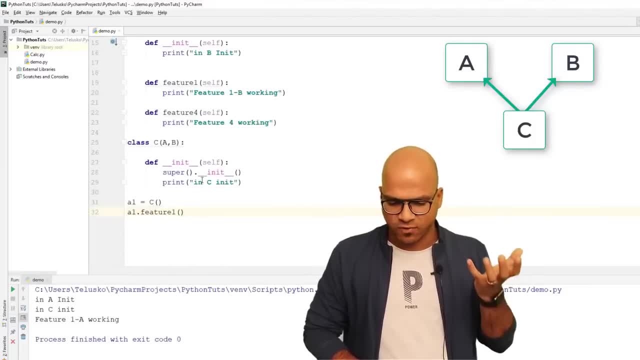 with the help of super method, can we call a function? Let's see that. So let's say from. we have a function here which is def, and I will say feature Fee. that's it. And in this I'm trying to call the method of superclass. right, So we can say super. 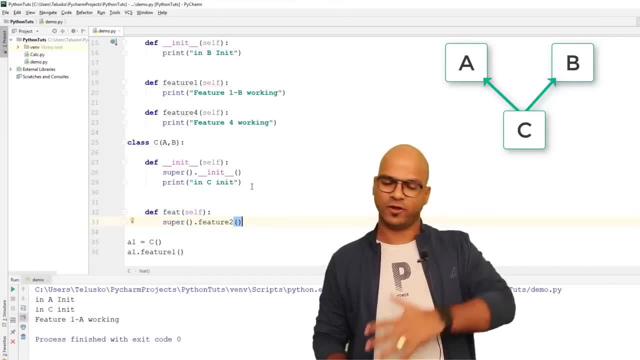 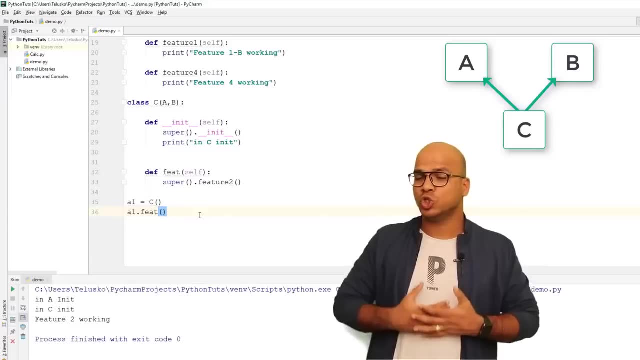 dot and we can use that thing. okay. So you can say: super dot, feature two, And let's see if it's working. Let me call feature. It should call the feature two. So yes, it works, So you can also use. 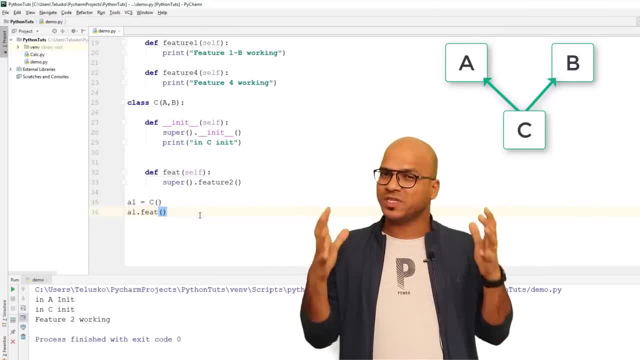 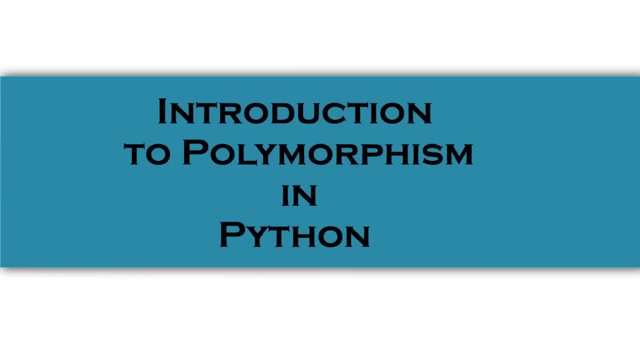 super method to call other methods as well, not just in it. So to represent this super class, we use super method. okay, Now we have started talking about the super method, So let's say we have a function here. Now we have talked about objects, right. Then we move towards class, And then we have discussed. 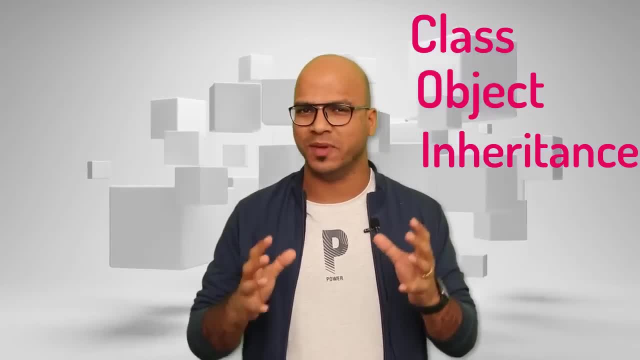 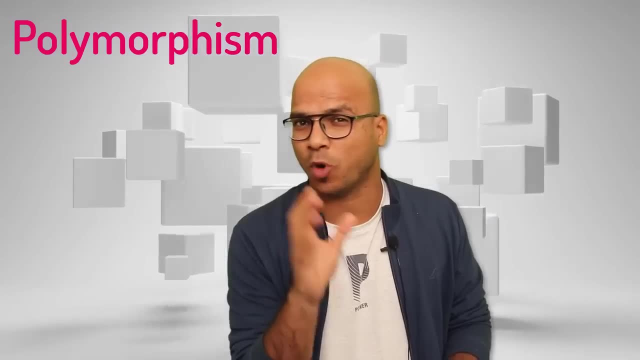 about inheritance. Now it's time to focus on one of the major concept in OAPS, which is polymorphism. Oh, that's a weird word. right Now, when you talk about polymorphism, let's break down this word: poly and morphism. So poly means many, right, And when you say morph, it means forms. So that means: 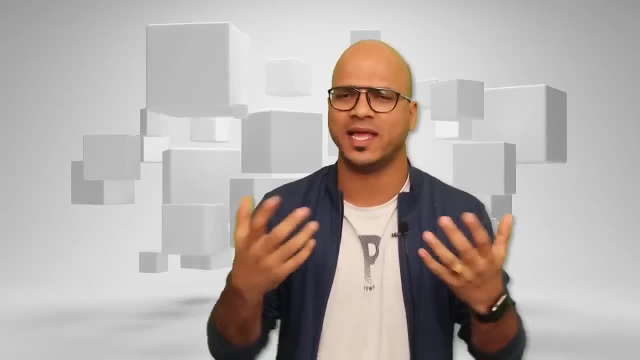 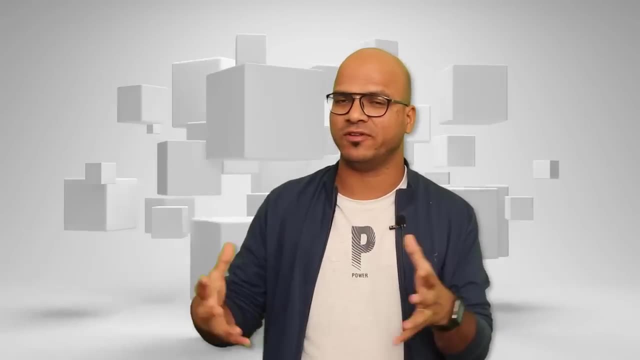 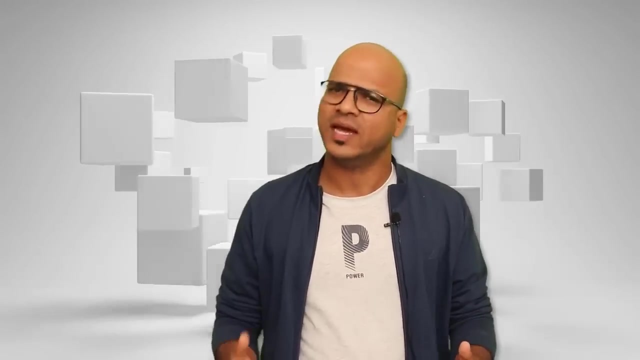 one thing can take multiple forms. Example like: as human, you know we have different forms. As the situation changes, we change ourselves, right Example: we behave differently. different location at office, We behave differently. when we are with our friends, we behave differently, So we are polymorphic. In the same way, when you talk, 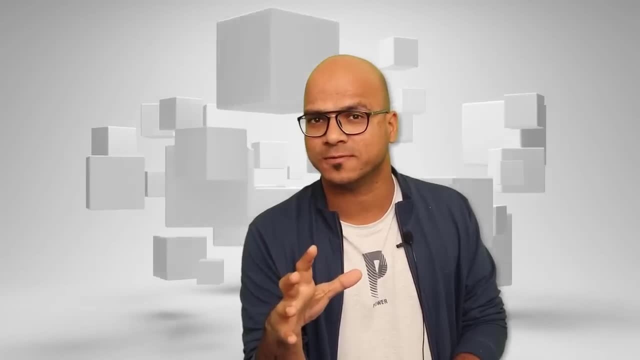 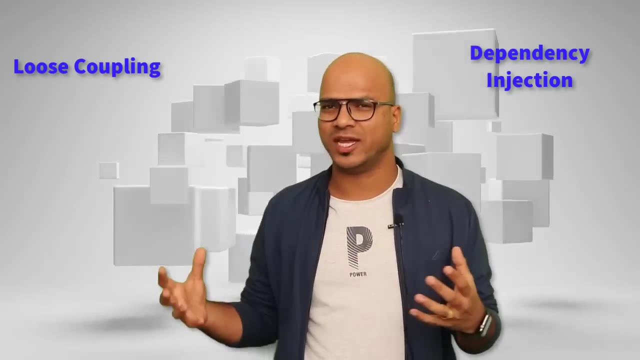 about object-oriented. objects will have multiple forms, So this concept is very important when you talk about software development. So we use this concept a lot when it comes to loose coupling, dependency injection. We also have a concept of interfaces, which we'll see later. 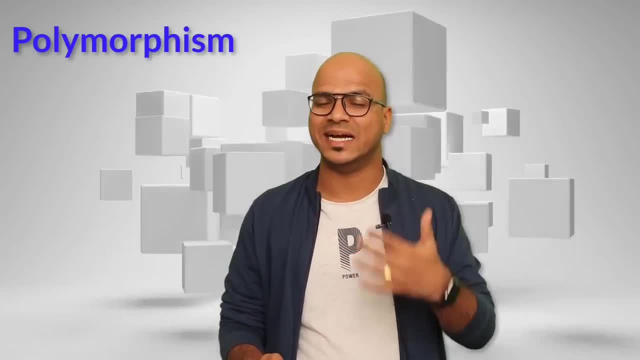 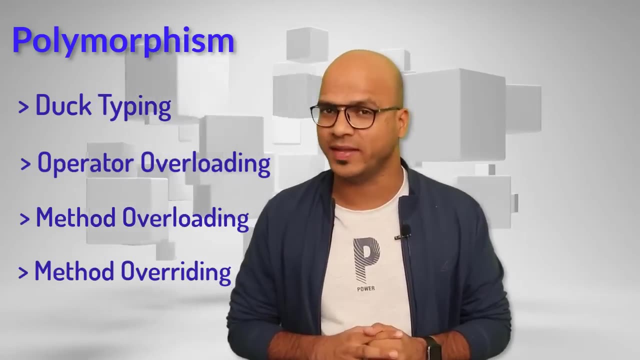 There are four ways of implementing polymorphism. The first one is duck typing in Python. The second is operator overloading, Then we have method overloading and method overriding. In the next few videos we're going to talk about all these topics, okay, And one of the interesting one is: 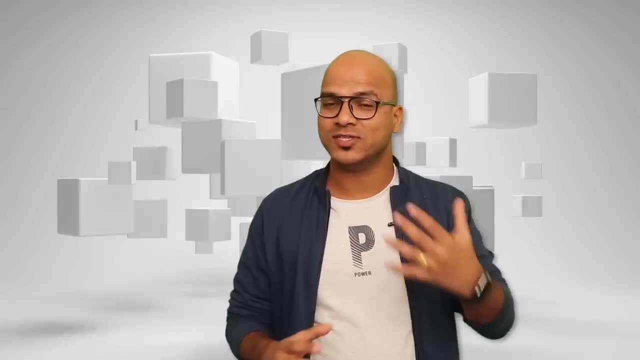 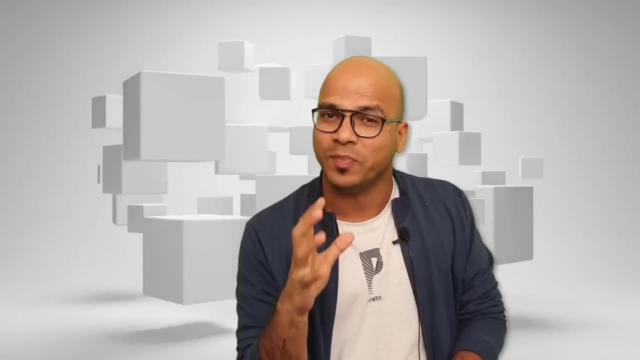 duck typing, especially if you're coming from different background, let's say if you have already seen Java or C++ or C Sharp. this is a bit different for you, because in Java or in C Sharp, we have to mention the type of the variable which you work with. right, We have to mention the type. 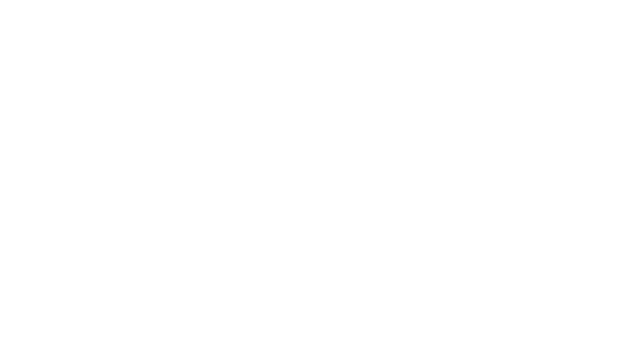 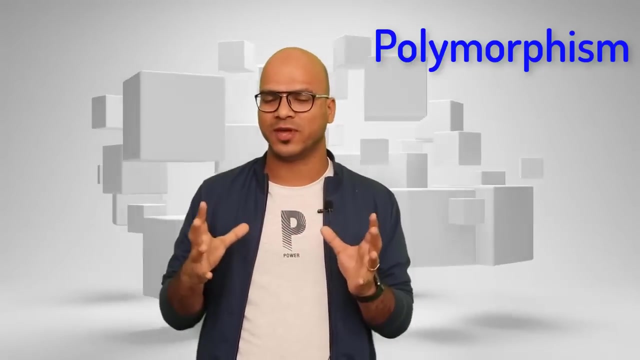 of object you work with. But Python, we have something different, right? In the last video, we have talked about polymorphism, right? Which simply means you have one thing which will behave in a different way, Or you can say one thing and multiple forms. 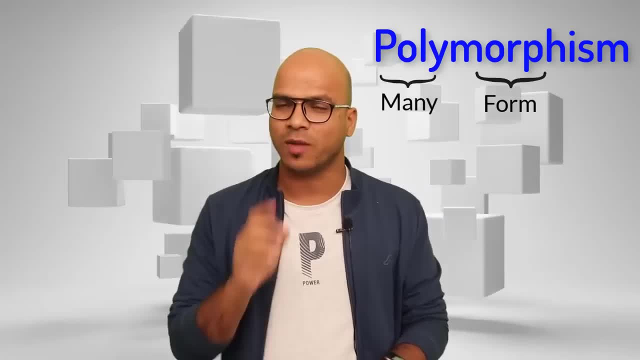 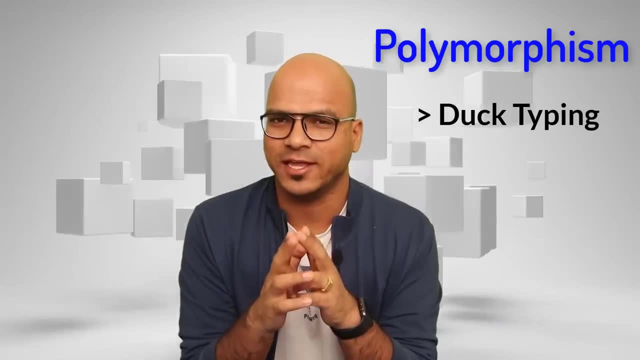 right, There is many forms. Now, in this video, we'll talk about the first way of doing that, and that is your duck typing. I know that's a weird word, right, Duck typing. We have this famous line, which is: if there's a bird which is walking like a duck, which is quacking like a duck, 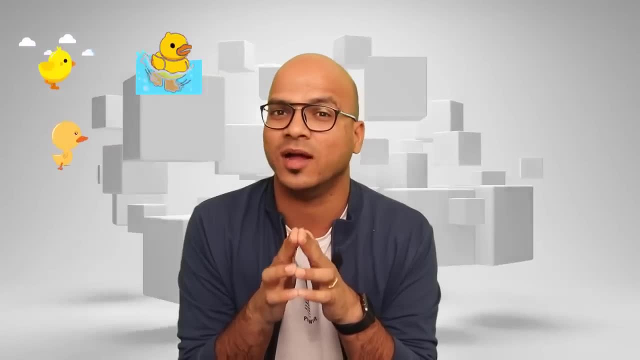 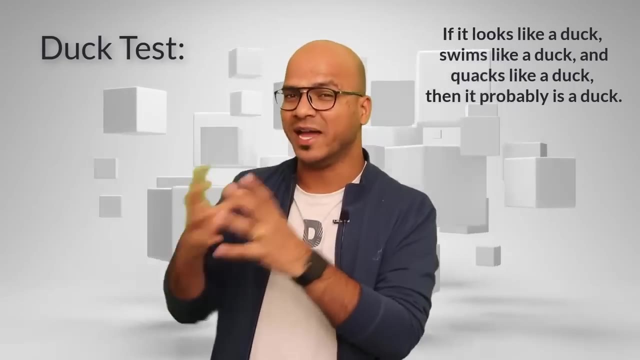 and which is swimming like a duck. that bird is a duck right, Which simply means it doesn't matter if it's a duck or not. What matters is the behavior of that bird. if it is matching with duck, that's a duck right. Now. how do you? 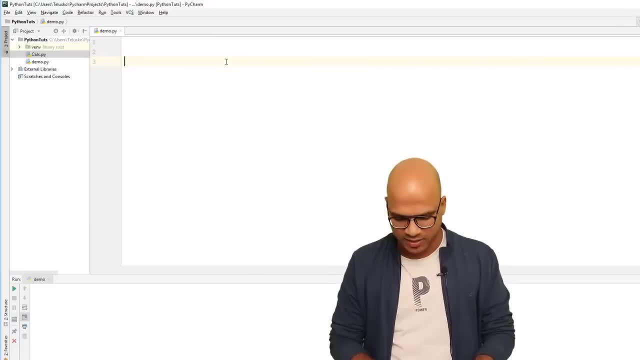 implement that in programming. So what we will do here is: let's take an example. Let's say, if I have x equal to 5.. Now, when you talk about the type, now in Python we have a concept of dynamic. 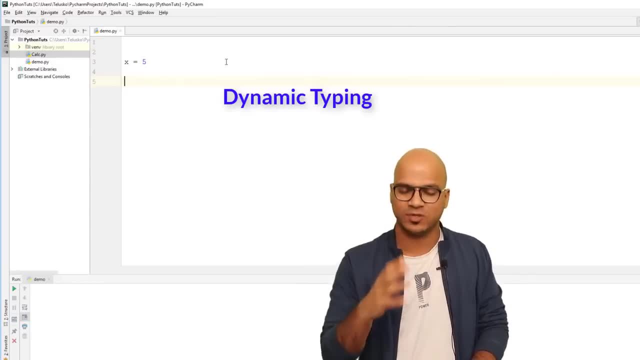 typing, which simply means the type you can mention later. Example: when you say x equal to 5, the type which we are representing now is integer. But what if you say x equal to 5?, Let's say Naveen? are we changing the type of x here? See, that's not the case. What is happening? 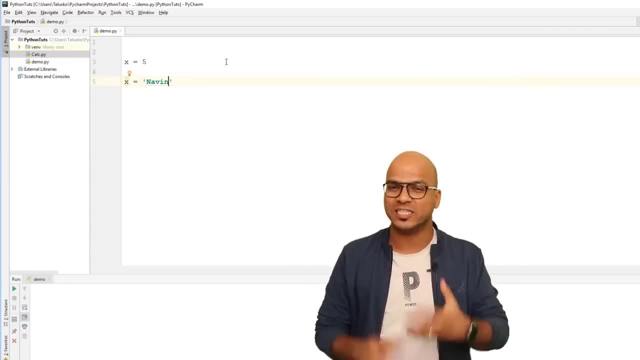 here is: when you say 5,, in your memory you got a space which is of type integer. When you say Naveen, in your memory you got a space which is of type string. The x is just a name to it. 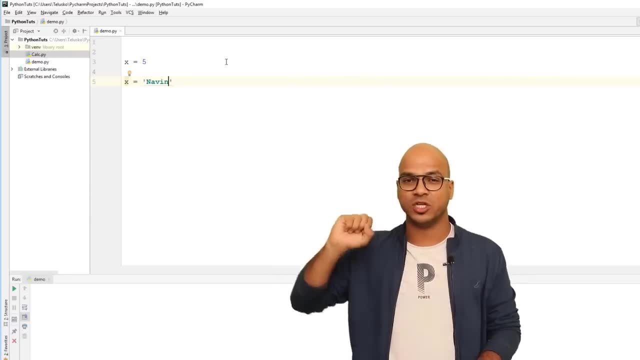 okay. So when you say x equal to 5, there is an object of type integer, you are just naming it as x Later. when you say you got Naveen, you got some space in your memory and you are representing. 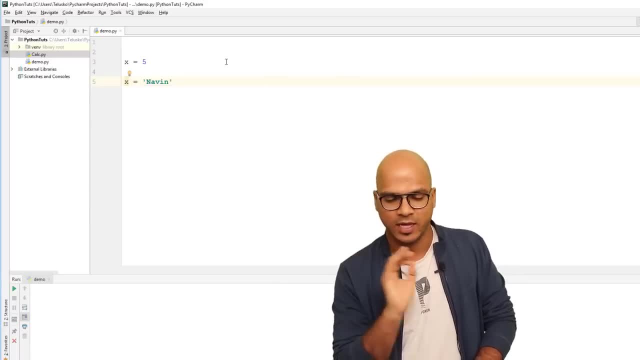 that with x. X is just a space. So when you say x equal to 5, you are just naming it as x, A name to it. okay, So we don't have specific type to x The moment you say type of x. 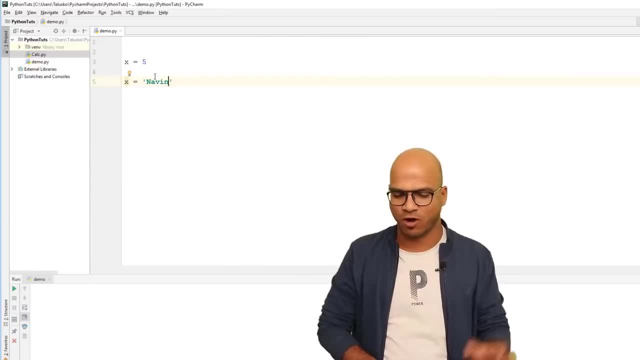 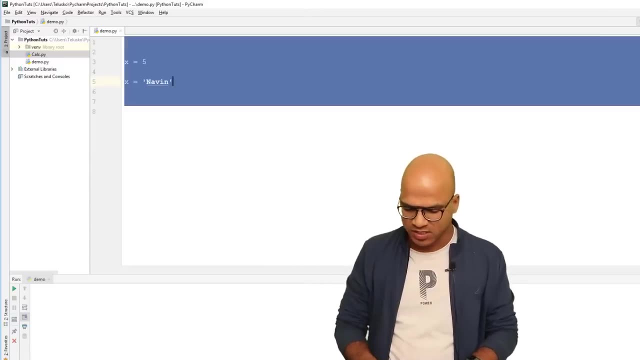 you are actually getting the type of 5.. When you say the type of x, you are getting the type of Naveen, right. So that's one thing you have to remember. The moment you give a variable name, that's just a name to a memory. Now, to understand duck typing, what we'll do is we'll take another. 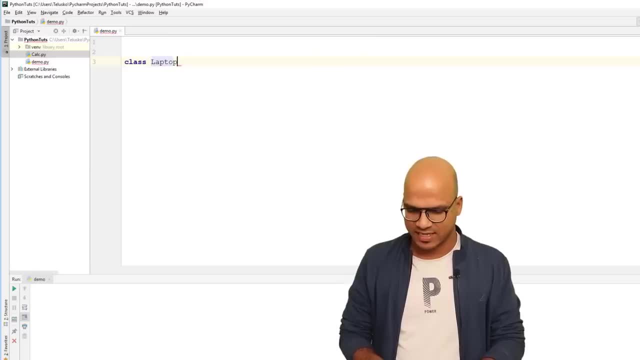 example, To explain this, what we'll do is I will create a class and we'll name this class as laptop, And this laptop class will have a method which is, let's say, code. So, in this code, what I will do is I want to execute my code. right? So, as a programmer, what we do is we 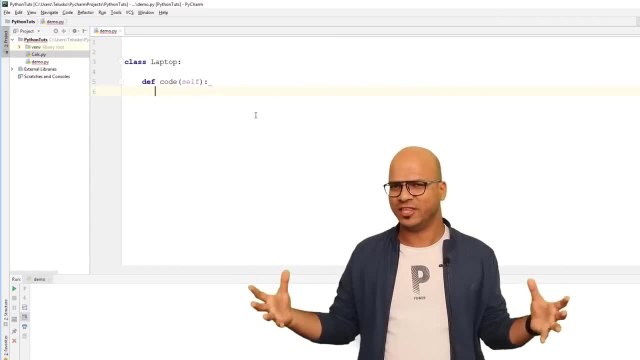 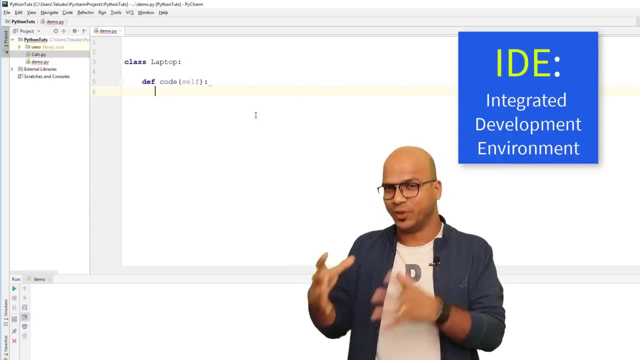 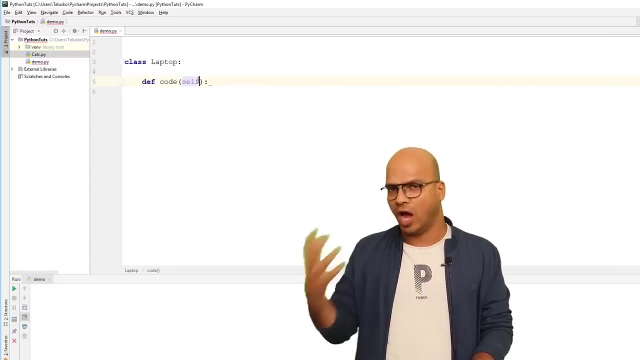 write code. right, We write code and we compile it, we run it and we get the output at the end. But then to do that we also need an IDE which is Integrated Development Environment, And in this case, if you want to write a code, you need to pass an IDE. So we are expecting in the 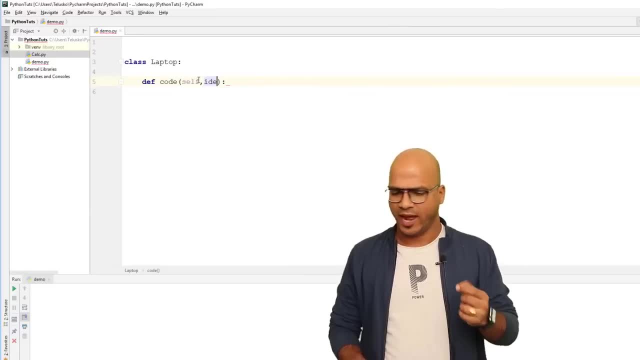 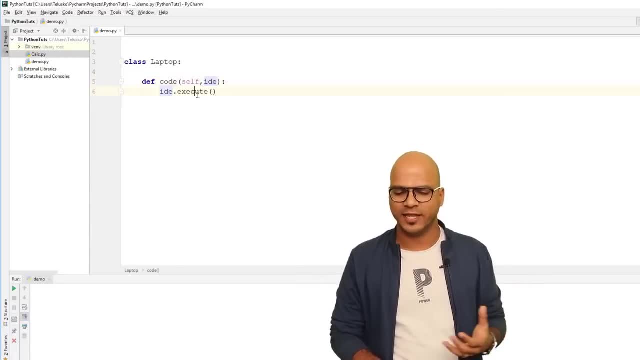 float. Is it a type of string? Now, of course, right. when you say execute, that means there's something which is not there in the existing classes which you have. That means the type of IDE is something very unique. It is something which is user is defining right, That means if 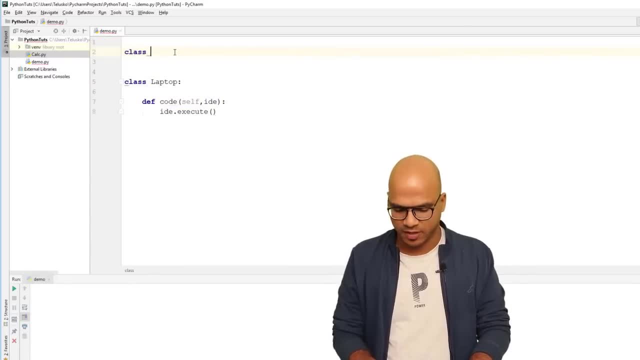 you want to create this object IDE, you need to create your own class. Let me get a class here and I will call this class as PyCharm. Now, for different languages we use different IDEs. In fact, for one language, we have multiple options. right Example when you work on Java. 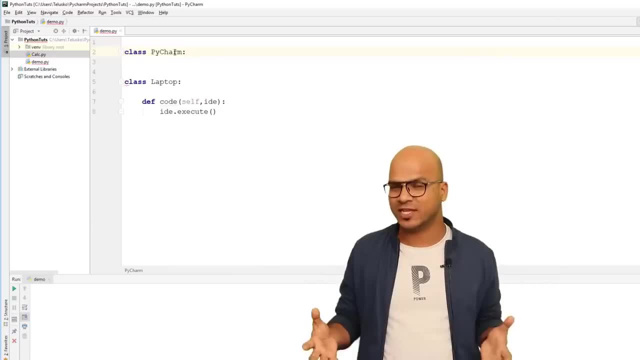 maybe you will be using NetBeans, Eclipse, IntelliJ For Python as well. we have different IDEs. We are using PyCharm here because it works well. Now, when you say PyCharm, of course it will have a method right. So let me define a method which is def execute. 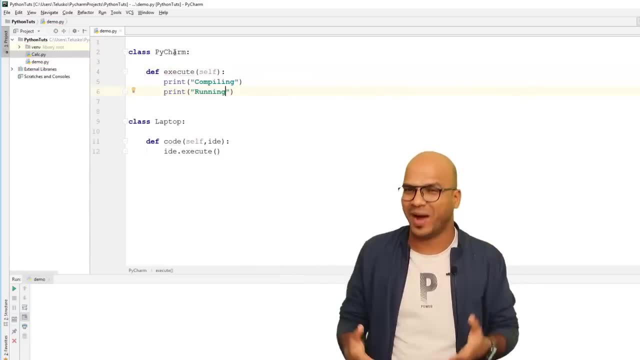 So you can see we have these two statements. The moment you say execute, it will say compiling and running. That's what you do, right? Your code gets compiled and your code gets run. Now will this work? Of course not, because we are not calling anything. So when you run this code, 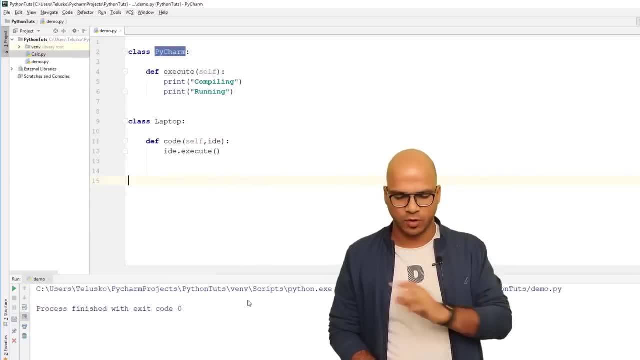 you will not get any output. Let me just try it out. I will right click and say run demo. You can see there's no output because we are not calling methods. Let me call code. The way you call code is by creating the object of laptop first, because you cannot call code. 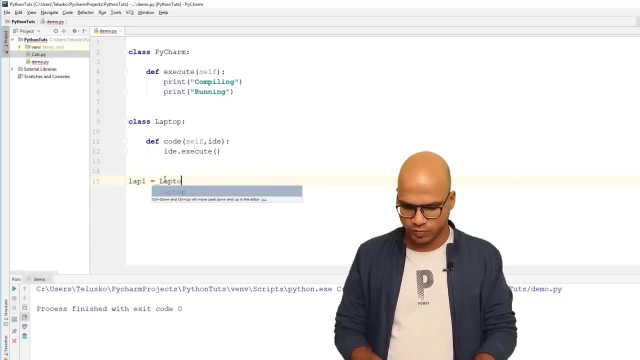 without laptop. So I will say: lap1 is equal to laptop and with the help of lap1, now you can call code. So you can say lap1.code. but there's one problem here, which is: inside a code, you have to pass an argument which is of IDE. Oh, that's a question. now, How do you pass an IDE here? So 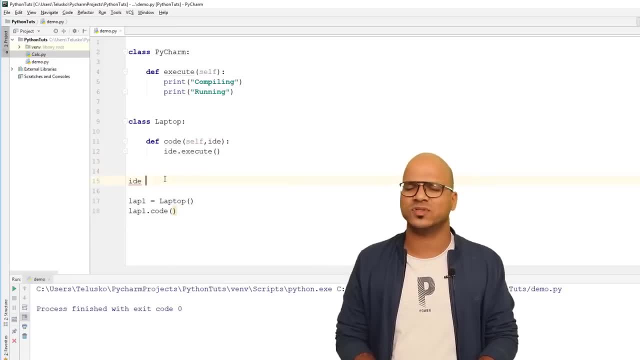 what I will do is first you need to create an object of IDE. You will say IDE. Of course, you can have different names here, but let me go with IDE. So IDE equal to this will be of type PyCharm. So the type of IDE we are working with is PyCharm, right, Which is user-defined, of course. 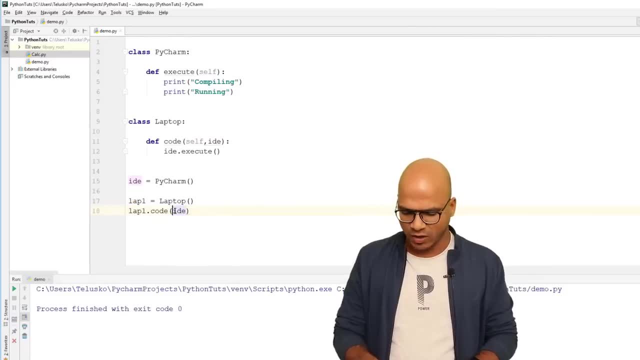 and then when you are calling code you have to pass IDE and now it should work. You can see from this code you got compiling and running. So the type of IDE here is PyCharm. but is it fixed? Can we change the type of IDE later Maybe? let's say we have one more IDE, Let's say in future. 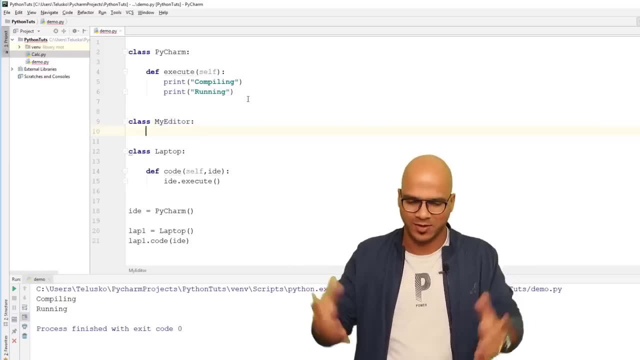 I'm creating my own editor, okay, which is way better than PyCharm, Maybe, and in that as well we have the same method, Let's say execute, and in that I'm doing some extra stuff, you know. So my IDE also does spell check. Maybe PyCharm does that. My IDE also does. 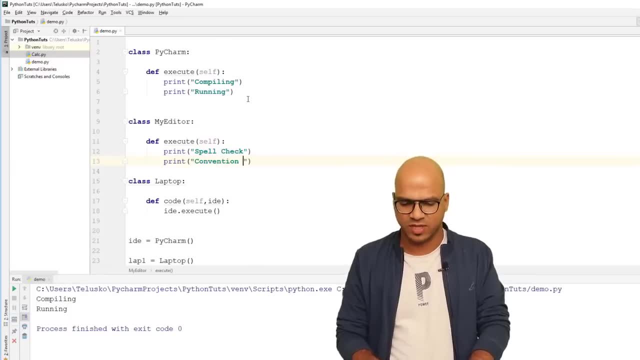 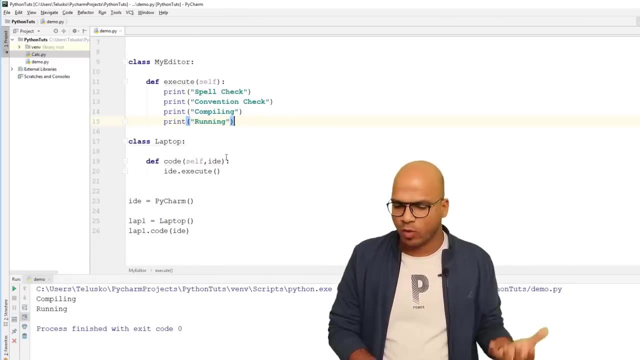 what Convention checks. you know the name of the variable and different stuff. and then it also does compiling and running, right? So my IDE does extra stuff. Now what if I want to change the type of IDE? Is the IDE type fixed to PyCharm? Not exactly, because this is dynamic typing, right, So you can. 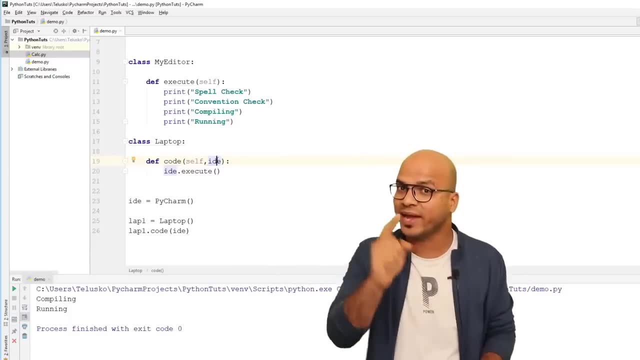 replace this IDE type from PyCharm to editor, provided you have that method which is execute right, It doesn't matter which class object you're passing. What matters is that object should have the execute method right, Because in IDE we are saying execute. So now, even if you change from 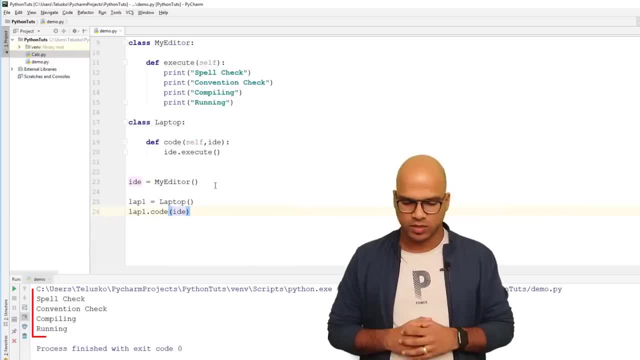 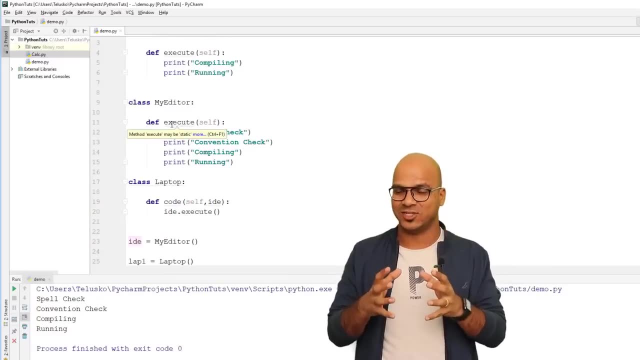 MyCharm to MyEditor, there's no problem, The code will still work right, Provided you have that method. okay. So if you should be having this method, which is execute, and that's the case, If that bird behaves like a duck, it walks like a duck, it quacks like a duck, it swims like a duck. 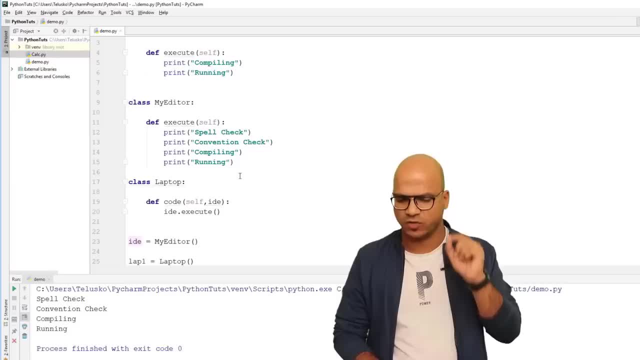 it should be a duck. In the same way, if there is an object which is IDE and it has a method- execute, that's it. We are not concerned about which class object it is What we are concerned about. it should have that method which is execute, and that is called as duck. typing right, I know. 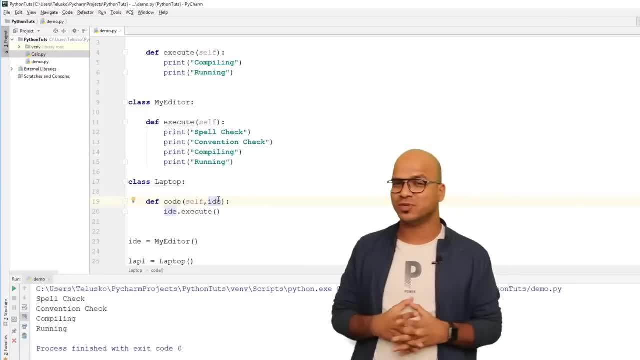 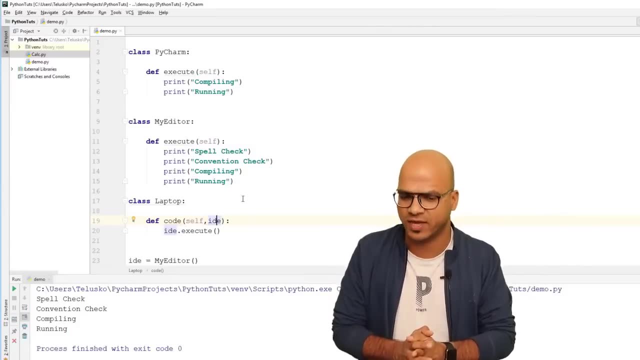 it is amazing. and if you're coming from different background, like Java, So we have a concept of interfaces, right? So that's what we do: We create interface and we have this MyEditor and PyCharm as which will implement that interface. but if you are new to this programming, don't worry, that's. 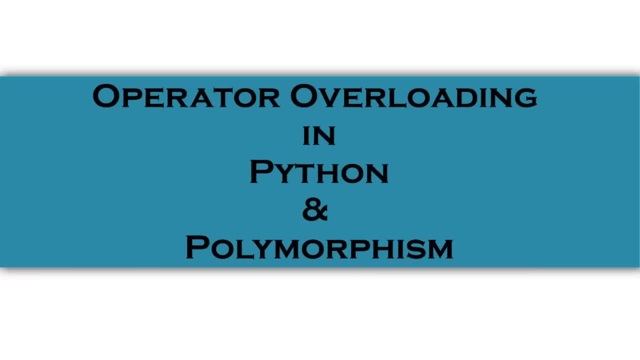 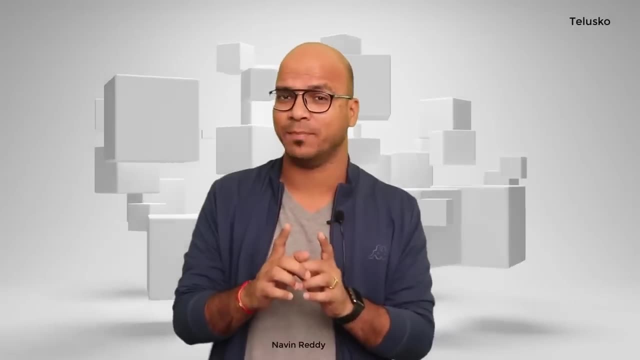 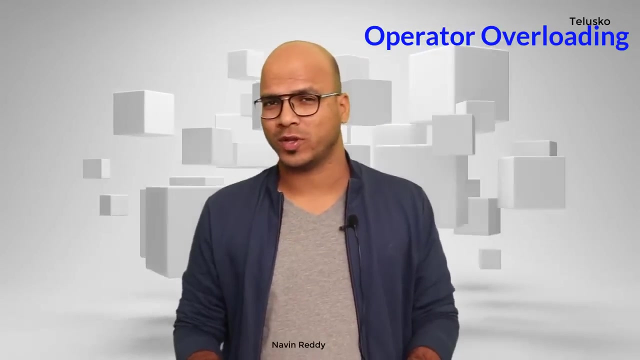 the dao part, right, this is simple. we have started talking about polymorphism, right, and in that we have seen one example of duck typing. now in this video, we'll talk about operator overloading. so what is operator overloading? so we know the concept of operators, right, so we have two operands example. 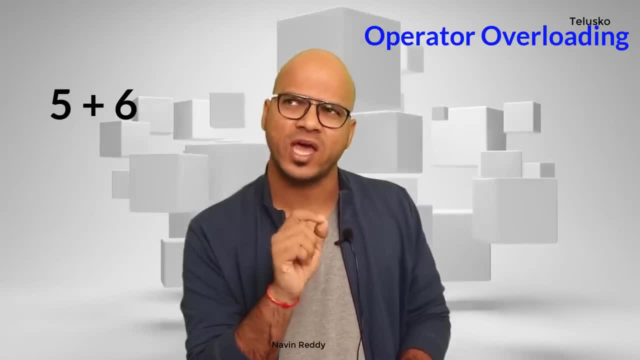 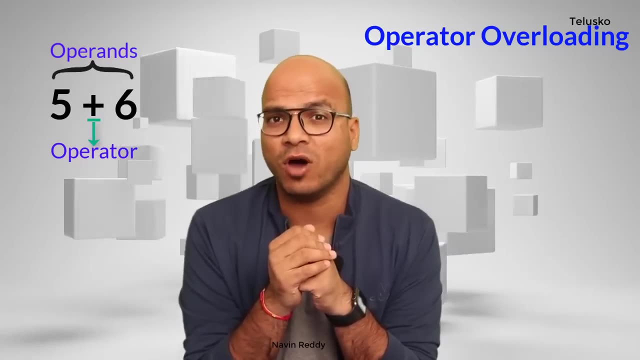 if you want to add two numbers, you can say five plus six, where five and six are your operands and plus is the operator. so we know that right. and then we have a concept of polymorphism. so it simply means you have one thing which has multiple forms right now. if you can think about this, we 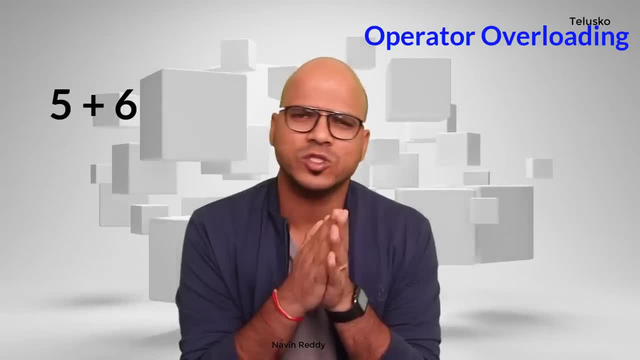 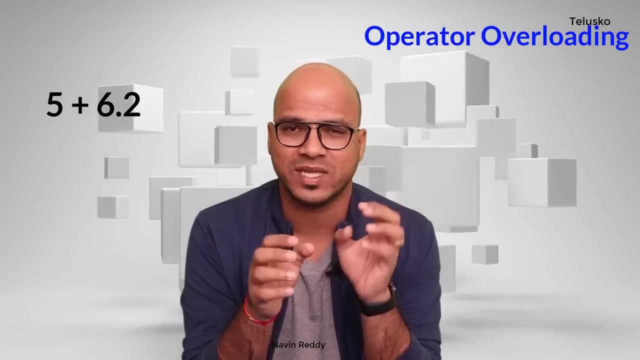 have two integers and then we are trying to add them. we can also add an integer and a float, right. so in different programming language it does support. what about two strings? so if you say you have two strings, let's say: hello plus world. will it work? and the answer is yes, right, so plus. 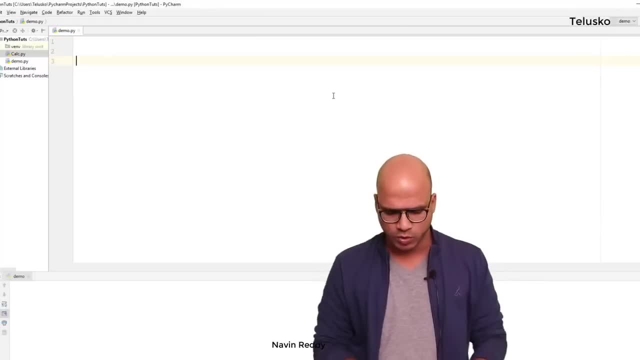 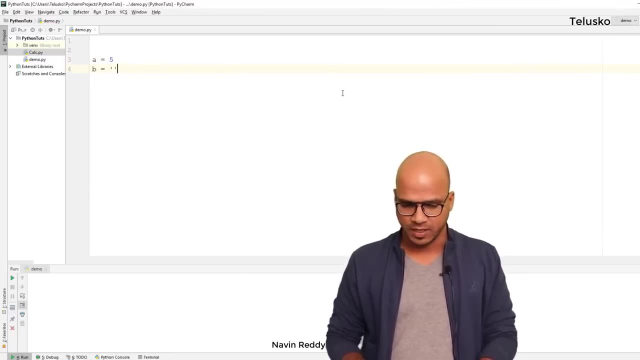 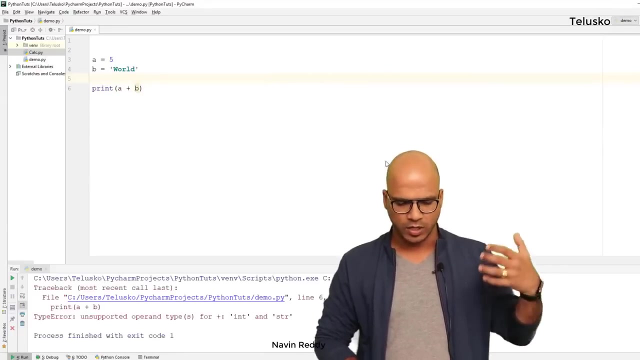 works with the strings as well. but what if you want to say you have a number five, so let's say we got a and a is five right. and then we got b and b is, let's say, world. now can i print by saying a plus b? the moment you try to run this code, you can see we got an error. it says unsupported operating. 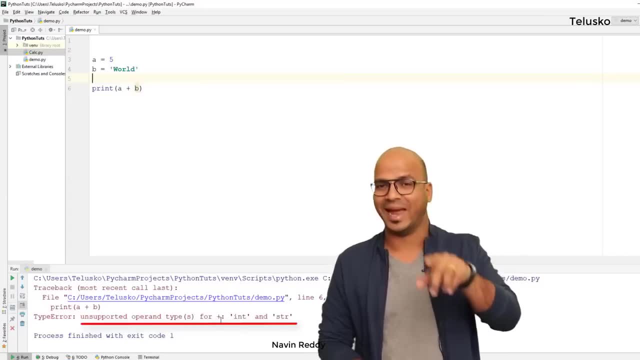 types for plus, so we cannot use int and string for plus, right? so all these things are predefined. all these things, they are called as a string. so let's say, if we want to print a string, let's say a string is called as a synthetic sugar, which simply means it is trying to simplify the code for the user. see, 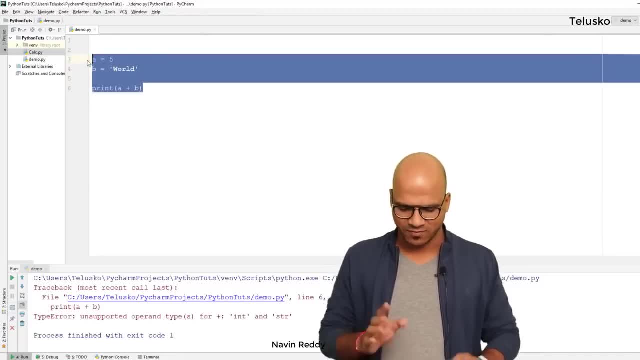 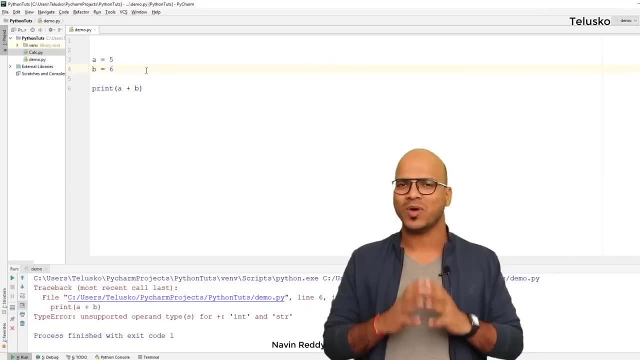 behind the same things are a bit different. imagine this one example: if i say a is five and b is six, now what do you think? what is happening behind the scene? now, trust me, whatever happens in python happens with the help of object right, and here as well. when you talk about a and b, the type of it is. 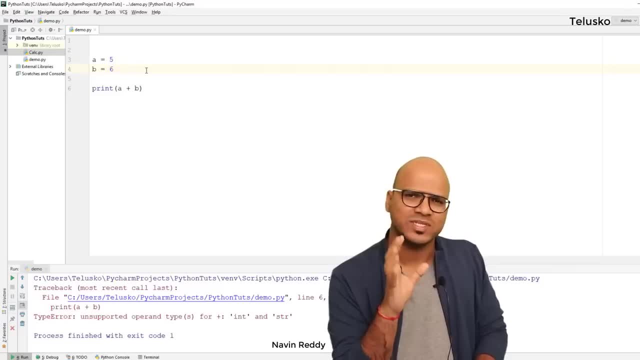 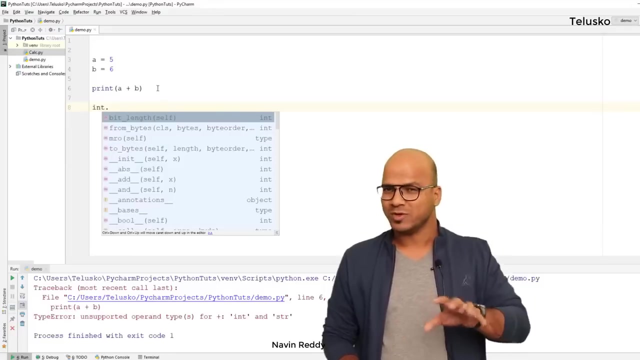 is int right, so int is a class here. and when you say class, of course class will have certain methods right. so behind this scene, what is happening is when you say a plus b, which is of type integer, it is calling something. so behind this scene it is calling int. dot the moment you 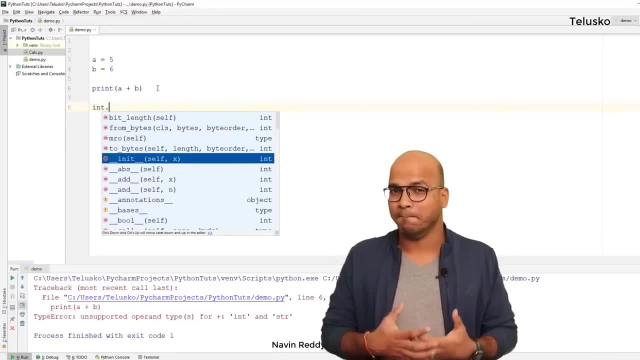 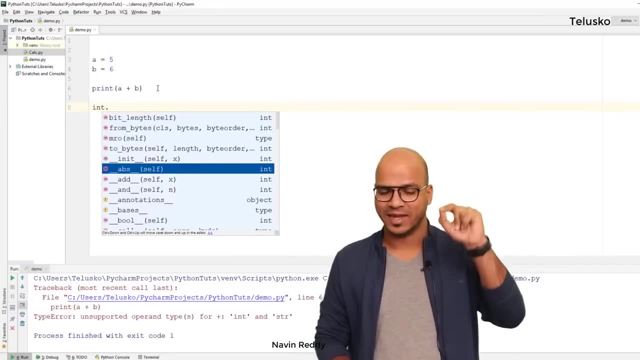 say int, dot, int is a plus right and you can see we have a method called as init, we have a method called as abs and we also have a method called as add, which is very important here. the moment you say int, dot, add, this is taking two parameters. okay, the first one is a comma, b. so what we are doing, 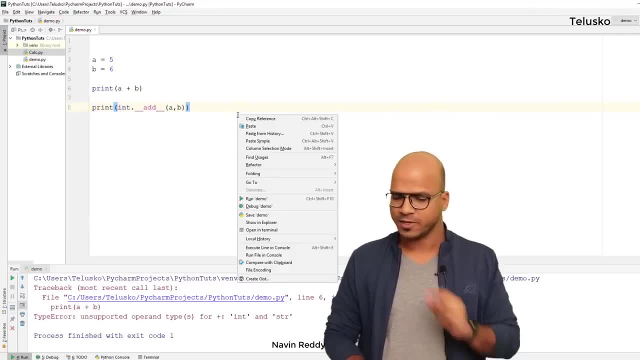 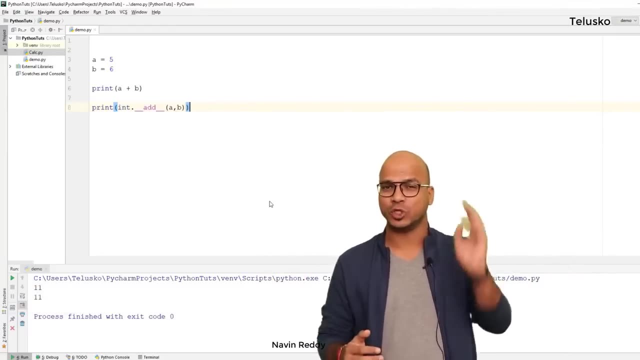 print a plus b. the same thing can be done here. let me run this code here. you can see we got the same output. so both are printing 11. so you can say a plus b, or you can say int dot, add by passing two parameters, a comma, b, and of course the first one looks cool. right, you are simply saying a plus. 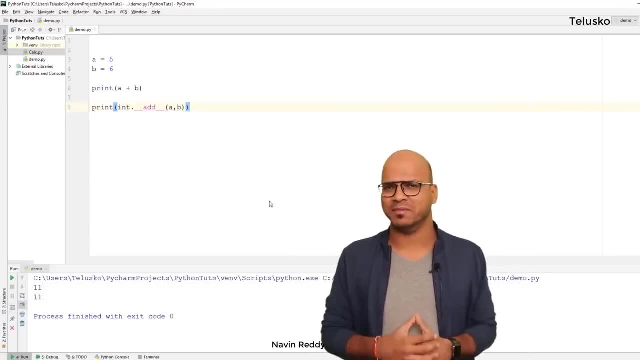 b, because from our childhood we are doing that, we are trying to add numbers using plus operator. but the moment you come to programming, in programming, whatever you want to do, you will be doing that with the help of methods, and add is a method which belongs to the 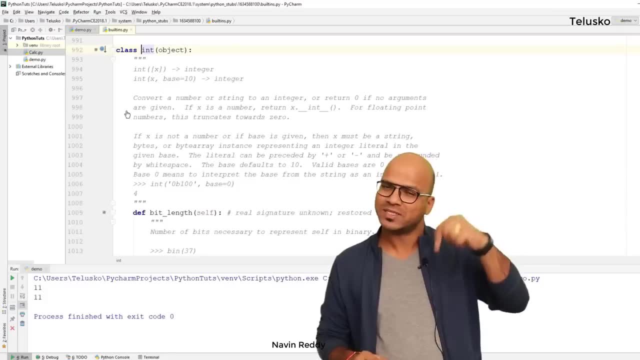 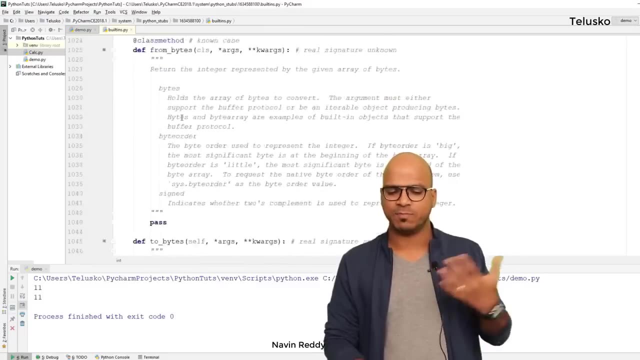 int class. right, if i jump to integer, so you can press on the control button and click on the method which you want to see or the class which you want to see. you can see it's a class and this class has multiple methods. in the same way, the moment you say int dot, you can access a method. 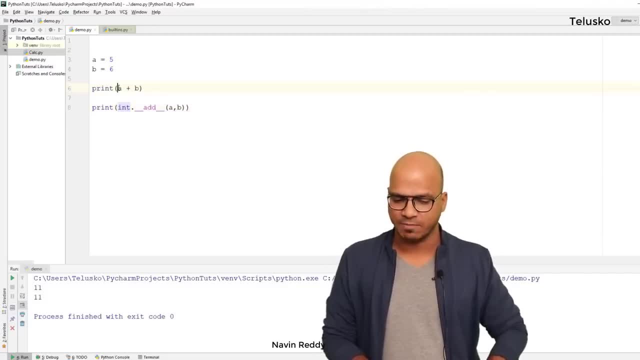 called as add and you're calling a comma b, so even if you say a plus b behind the scene, this is getting called right. so this is one thing you have to remember. okay, so we'll talk about orbit overloading later, but this is something you have to remember. so whenever you add two numbers, 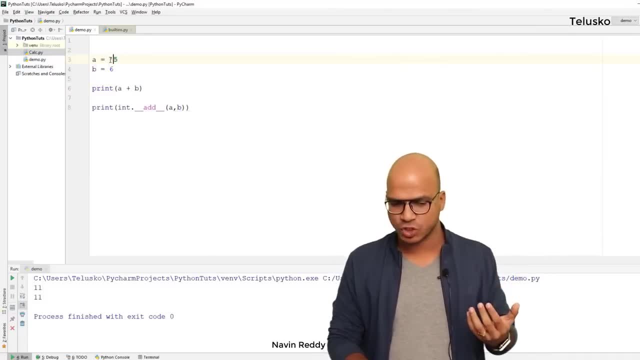 this is what is getting called behind the scene now. if these two things are strings, so if i make it string here now, this is not integers, right, they are strings. so i have to say str dot add. now, when you say str dot add, in fact str also has a add method which takes two parameters. 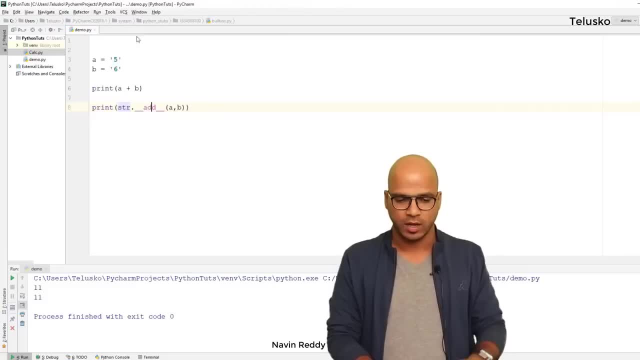 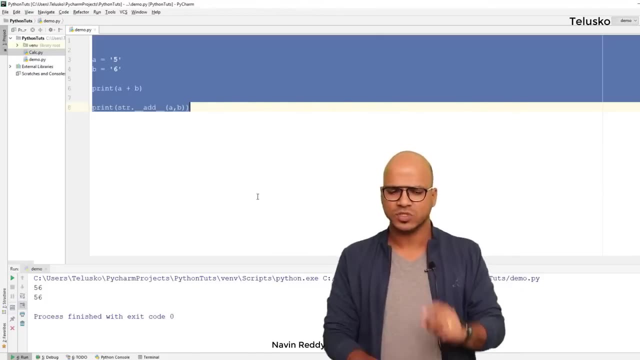 and both should be of the same type, with a string type, and then it will work right. so if i run this code and you can see it is working. so we got five and six as a string, so they got concatenated here, so this works. the moment you change the type of it, it will not work because the inbuilt class, the 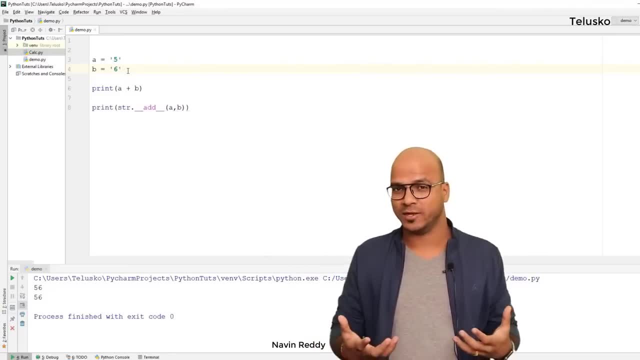 doesn't have two things, which is integer and string together, right. so this thing you have to remember now, once we know: the moment you add a plus operator, it calls the add method. the moment you put a minus operator, it will call a sub method. the moment you use a star symbol, which is: 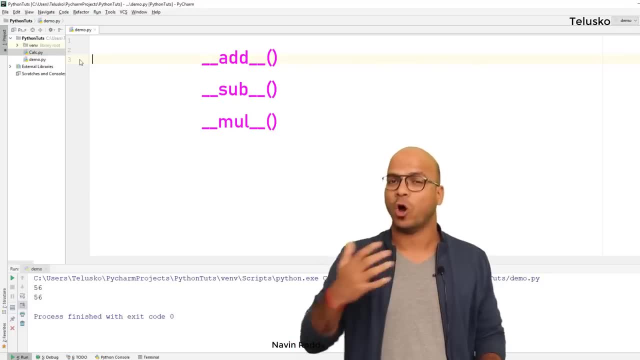 multiplication, it will call mul method. so we have different methods for different operators, right, and normally those things are called as magic methods. but that's what they say, magic methods, right? so all these operators behind the scene, they work as methods. now, to understand the concept of overloading, what i will do is i will say class, and let's say we have a student class and every 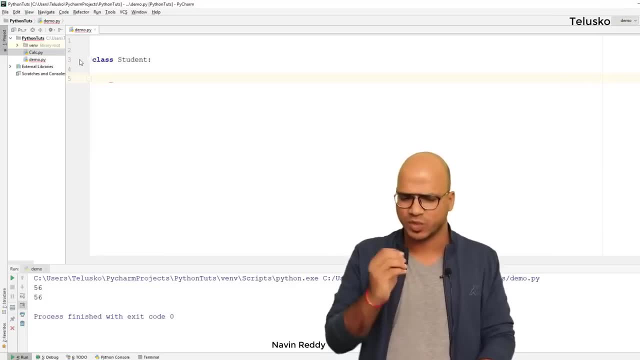 student will have, let's say, two variables, and that will be marks one and marks two, just to keep it simple. uh, so what i will do here is i will say def and init and here i will say self dot m1 is equal to: oh, now we want the value from the user, right? so, or maybe i want to pass the value, so i will pass. 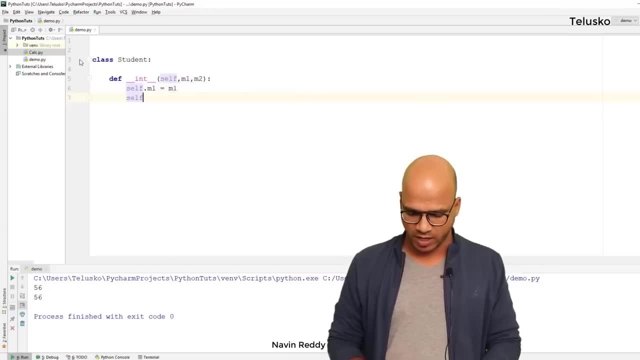 it from here: m1, comma, m2, and let's specify self dot: m2 is equal to m2. so we got these two values. what i want to do is i want to create two objects, okay, two students. object one is, let's say, s1 is. 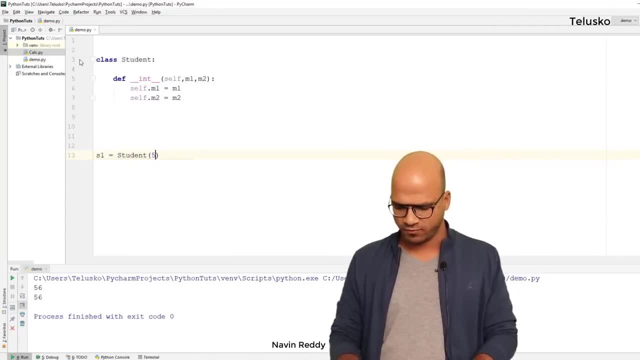 equal to student and this will take two values. i would say, uh, 58 comma 69, that's the value here, and then s2 is equal to student and this student will have, let's say, 60- 65. so we got two marks here, right, we got two student and you shouldn't have two marks. now i want to apply the operator here. 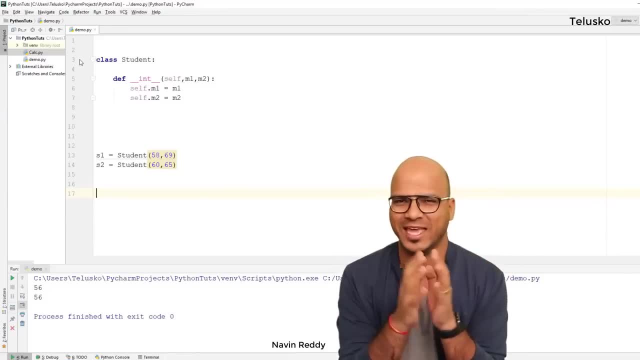 which is plus operator. so i want to add this to student. so the moment i say s1 plus s2, i want a. is it possible to do that? let's try. so i will say s3 is equal to s1 plus s2, because now we know that. 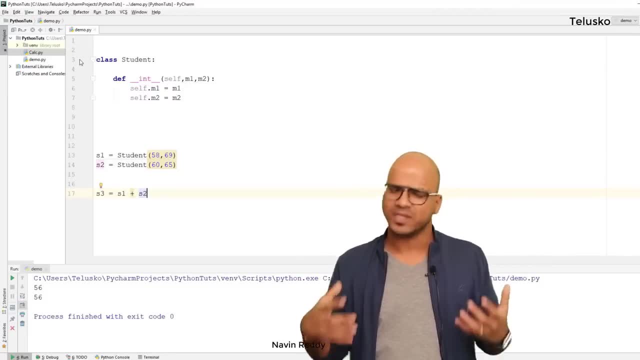 plus operator means it will add two values, but it is possible with the help of integer, it is possible with the help of string. is it possible to use plus operator with student class? that's a question. so let's run this code. let's see what happens. okay, we are not printing the value of s3, but let's run. 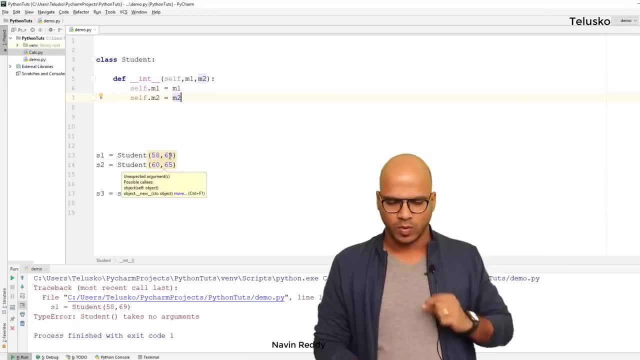 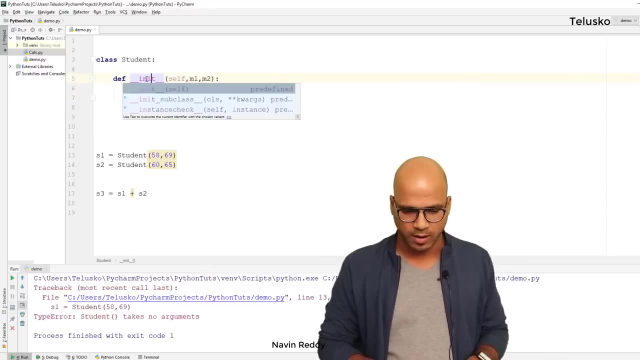 this code. the moment you try to run this code, you will get an error. oh okay, we got different error here. it says: student takes no argument, but it is taking arguments right watch wrong. oh, we have written the wrong method name. my bad, let's run this code once again. so i was. 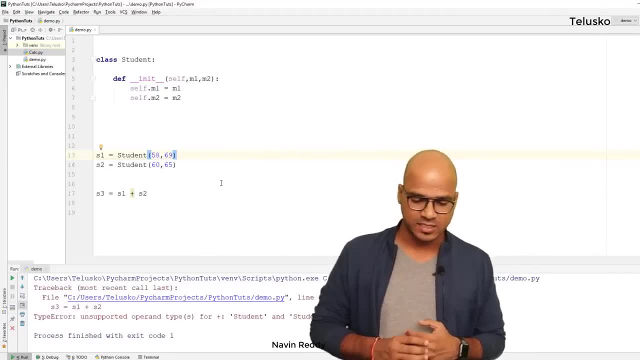 expecting this error, not the first one. and the error is it says unsupported operating type plus. we cannot use plus between student and student because we have not defined it right. if remember behind the scene, even if you use plus with integers, it will be calling a add method. but if you see our class, we don't have that add method right. 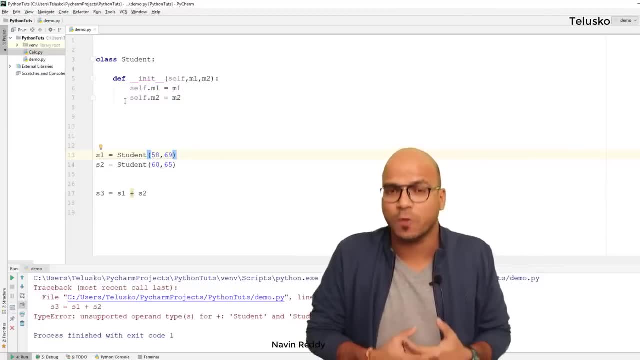 because if you say s1 plus s2, how your compiler, how your python, will know what to do and that's where you have to define it. yeah, that's we have to say: hey, the moment anyone says plus of a student, you need to call this method call as add. okay, so you can overload the operator and you can change. 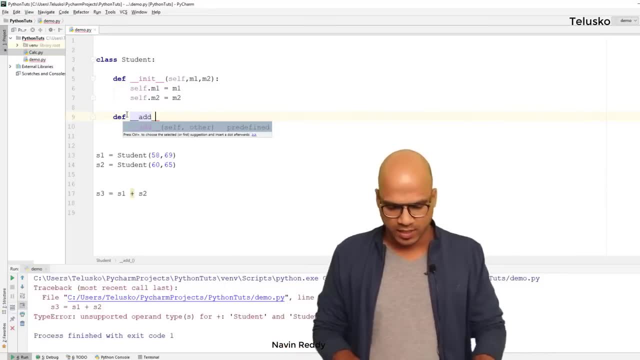 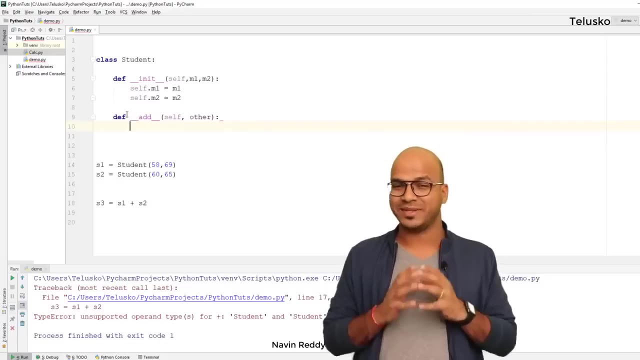 definition for it. you can define anything you want, right? so i can say add, and this ad will take two parameters. the first one is self, comma, other, and you can see if it takes two parameters, self and other. okay, guess what is happening? so, behind the scene, this code is getting converted into. it is. 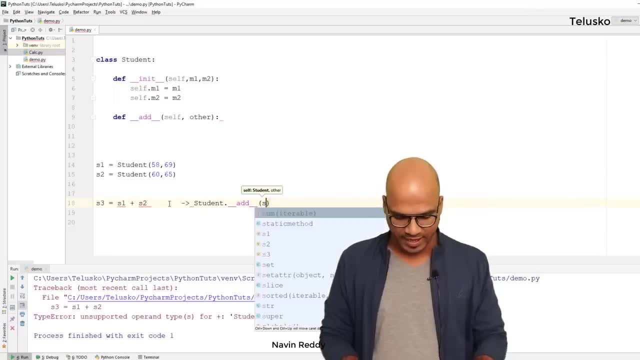 going to be self. dot add, which takes two parameters: s1, comma, s2. so what is self and what is other here? so the first parameter is self and s2 is the other parameter. you can change the variable name. that's fine. okay, you can say: this is o and it should work. it's a variable name, right? so this is what is. 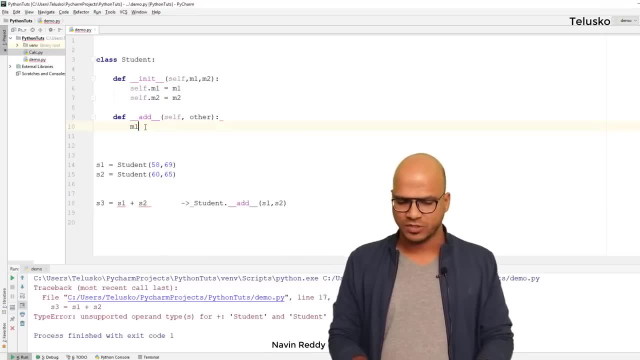 getting called behind the scene, right. so here, what i will do is i will say: let's take two variables: m1- m1 is equal to self dot m1 and m2 is equal to self dot m2. so we got two variables right. oh, not just self m1 plus. it is other dot m1 plus other dot m2. so this is how you. 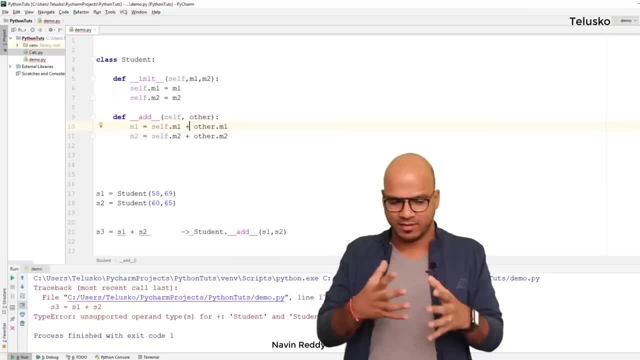 add values, right? so self m1 and other m1 and then m2 will have the addition of self m2 and other m2. so this works. and once you've got these two values, what you'll be doing is you'll be getting a new student object. we'll call the s3. you can have any name, doesn't matter. so s3 is equal to student by. 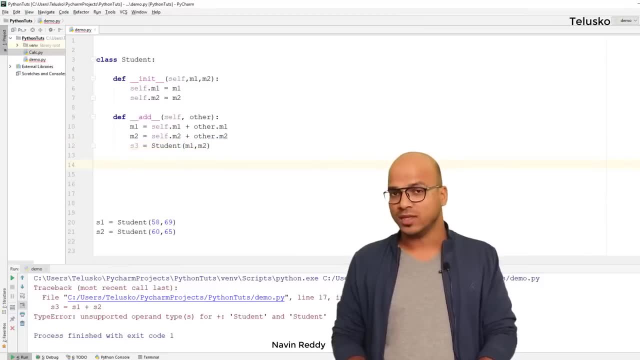 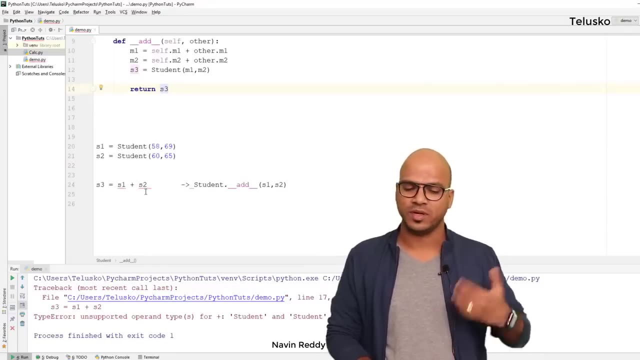 passing these two values, m1, comma, m2, and now, once you've got this student, you will return s3. here is what you're expecting. so the moment you say s1 plus s2, it will return the value, it will return a new object of student and it will assign that to s3. okay, so this is what will happen now if i print. 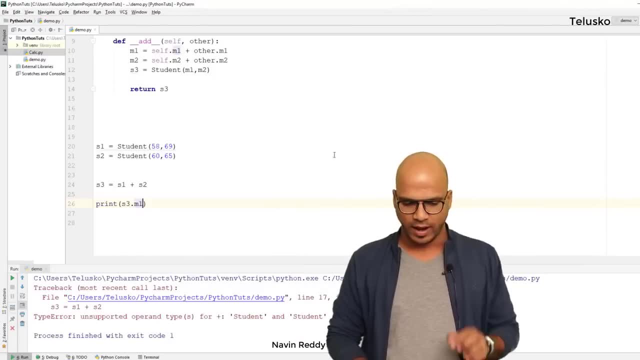 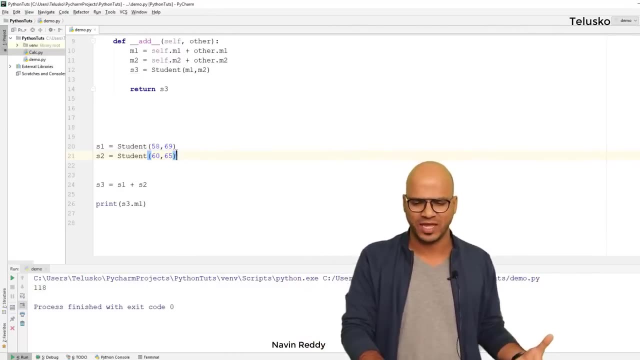 the value for s3. so i will let me print s3.m1 and the moment you run, this code run and you can see it works. we've got 118, is it right? of course it should be right. so it is 58 plus 60 and that's. 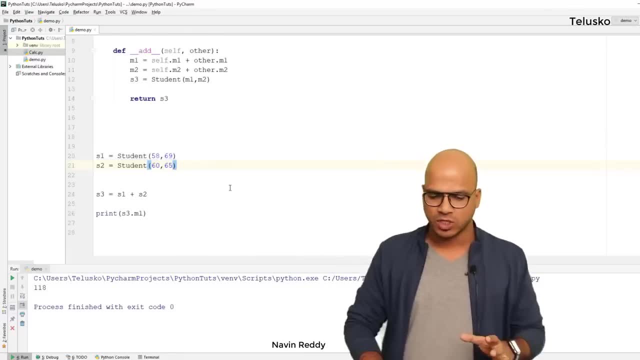 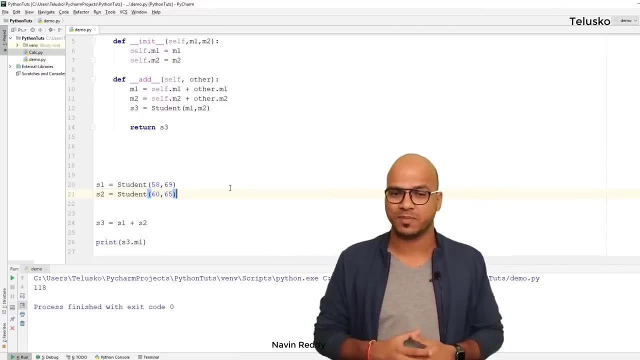 right, we got 118.. this thing is working right, perfect. so if you want to add two students, you need to overload the operator of the student and you need to load the operator of the student and you need to load the operator of plus, because integer knows what is plus, string knows what is. 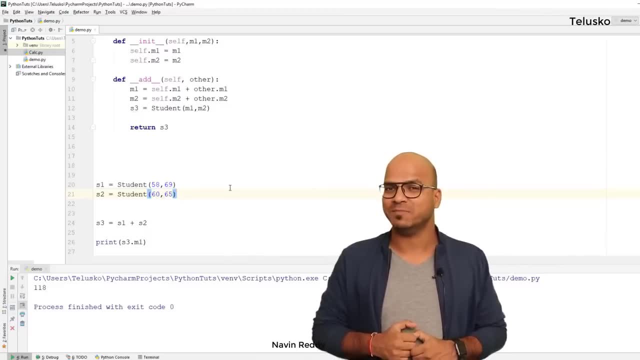 plus your student class don't know what is that plus means. so plus means called the add method. but we don't have an add method here, so we have to define our own method. the same thing can be done with subtraction, which is minus. the same thing can be done with multiplication. so i would 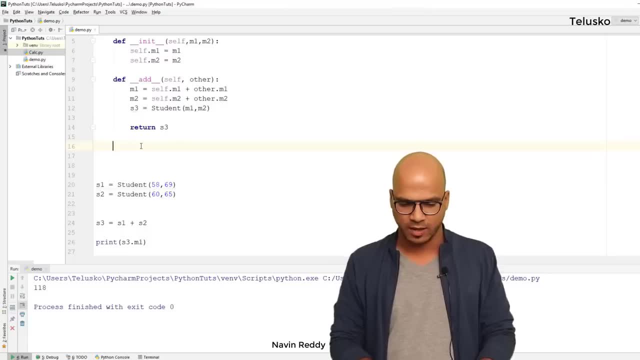 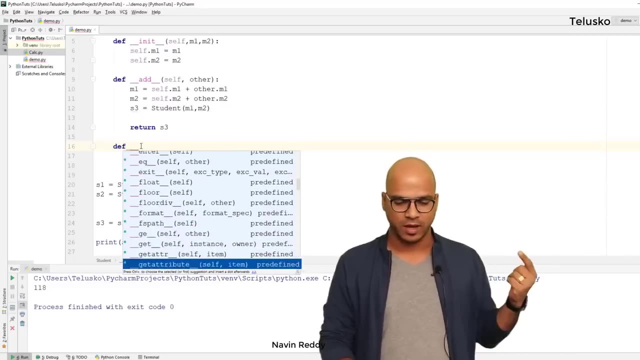 recommend you to explore more on this, you know. so the moment you say def, underscore, underscore, you can see we have so many methods. we also have greater than we also have equal to symbol. we can compare two objects. uh, we can say the different methods available here. okay so, 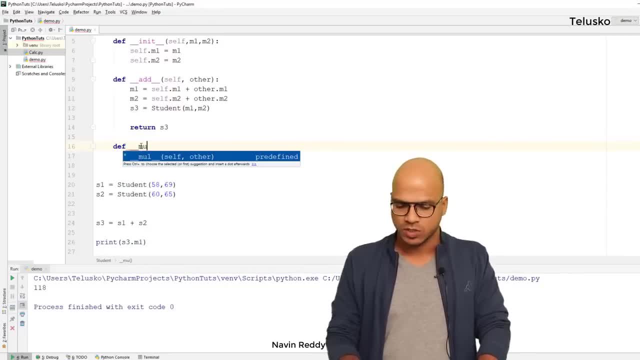 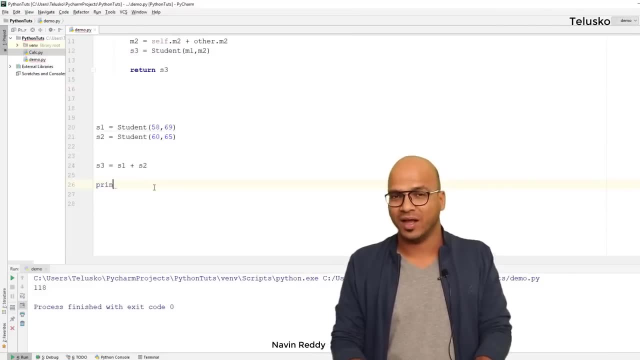 i doubt we also have multiplication somewhere, so you can see we also have mul, so everything is predefined. you can just use them, in fact, for this example. i will take one more. i want to compare if two objects are getting not equal to example. if i say: if s1 is greater than s2, this is the horrible. 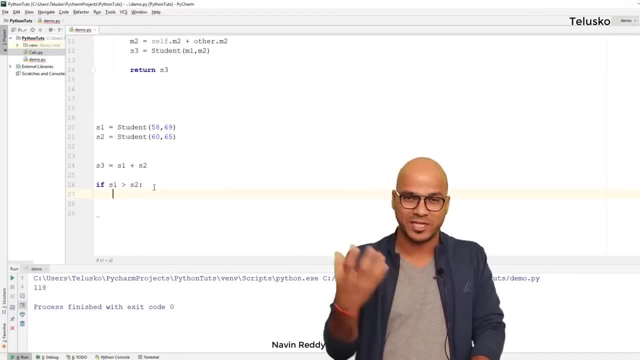 way of comparing students, because marks is not a criteria where you can compare students. but just for the example, i will say s1 win. so whoever has maximum marks, i will say they win. i will say else print, s2 wins. so what we're trying to do here is whoever has maximum marks they will win. but when you say 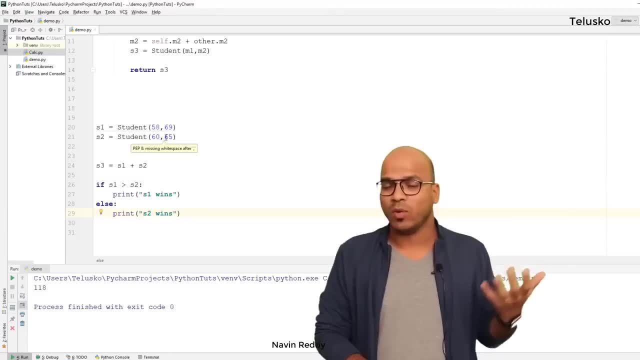 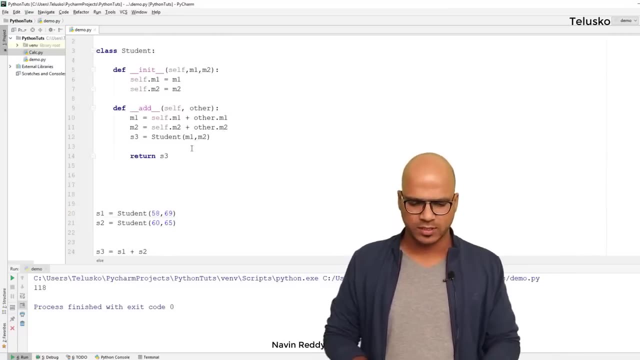 maximum marks. how will you check it? because we are not defining it right. maybe i want to check only first marks, which is m1, or maybe i want to check m2, or maybe the addition of both. you can try it out. so what i will do here is: this will work. of course not, because the moment you try to run this. 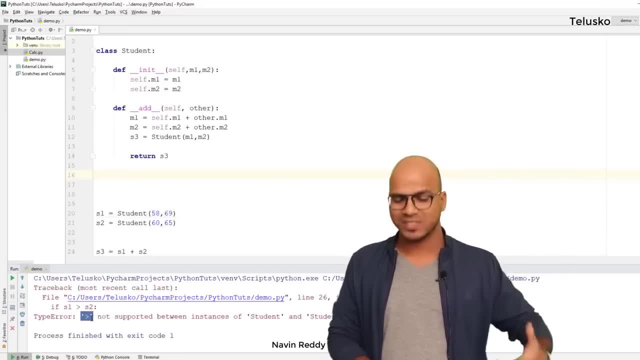 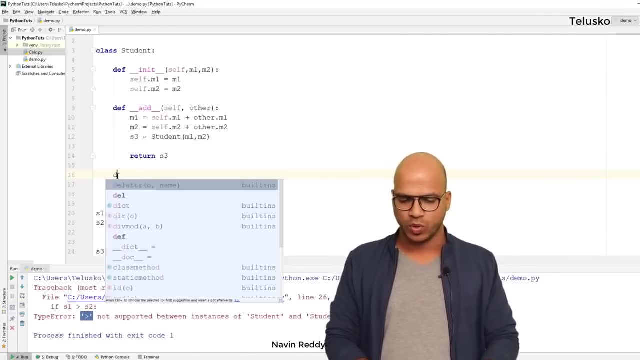 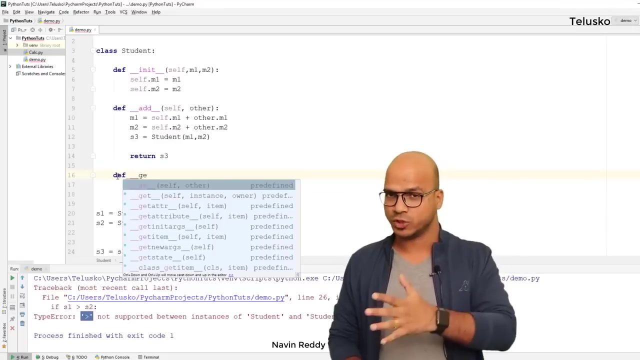 code. it will give you an error by saying the greater than symbol not supported between two instances of student. it is supported for integers because it is predefined, so here as well, if you want to check the greater than symbol, you can use the method. of method which is gt. gt is greater. 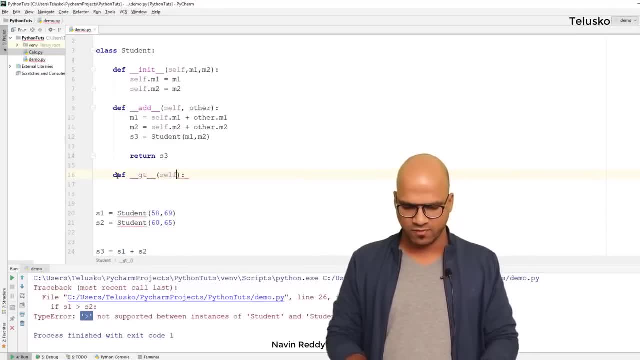 than g, e is greater than equal to. so you want to check only greater than. and then here you will be, using self and other as usual. because behind this thing that is what is happening. it is saying student dot, gt and it's passing two variables, s1, s2. so s1 goes to self, s2 goes to other. and now 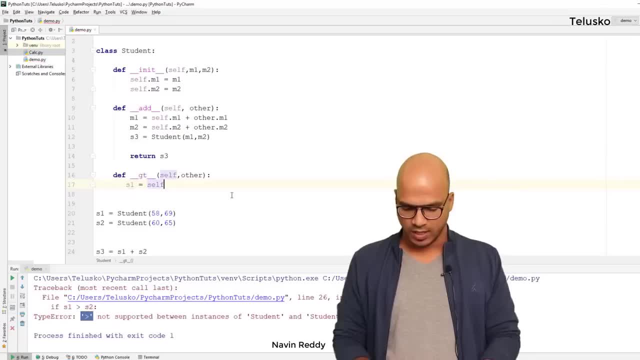 how do i compare? so we'll say s1 doesn't matter, is it s1 or something? so we'll say s1 is equal to self dot m1 plus self 2, and we'll say s2 is equal to other dot m1 plus other dot m2. so we are adding their marks. 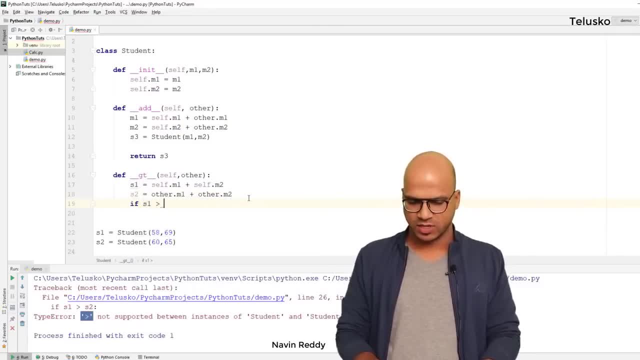 basically, you can compare if s1 is greater than s2. now this time, s1, s2. they're not objects, okay, they are simple variables of integer. okay, if i'm getting confused with this, let me just make it r. that should make sense. so let's compare r1 and r2. now those are just marks, right? if r1 is greater. 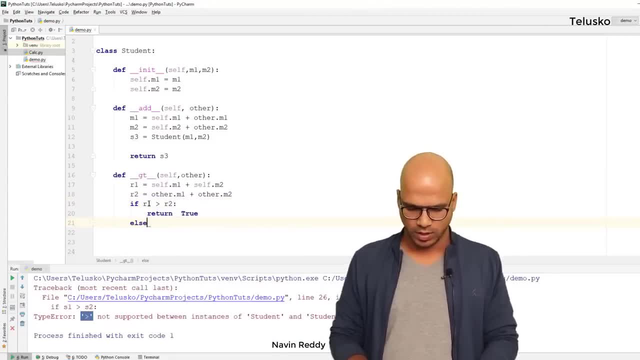 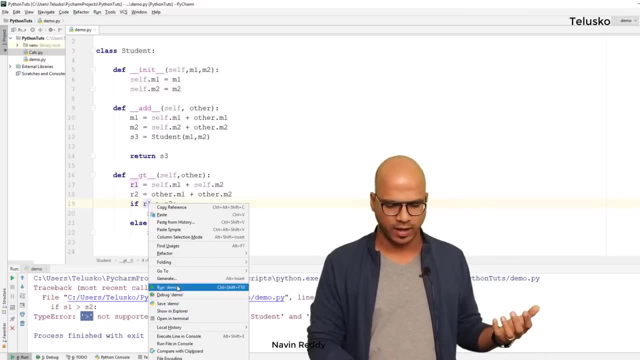 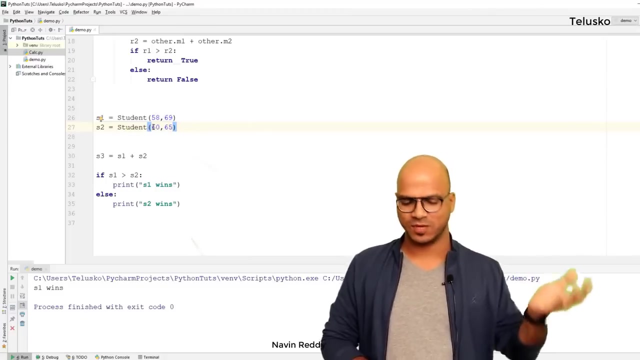 than r2, we will say return true, else return false. simple. now, if you run this code, we are comparing it right. let's compare and let's run. and it worked. you can see s1 wins right because s1 values are higher. so 58 plus 69 is higher than 60 plus 65. 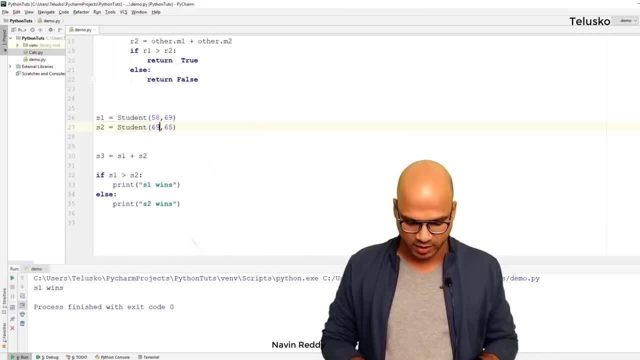 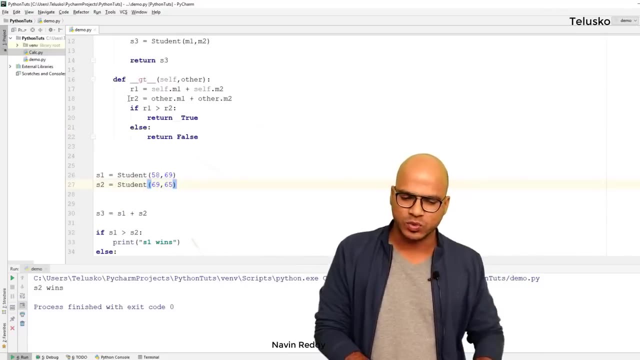 but what if i change the value for s2? let's say this: 69, and you can see, of course, now s2 is bigger. so let's run this code and you can see it says s2 wins. so that's right. so what we are doing is we? 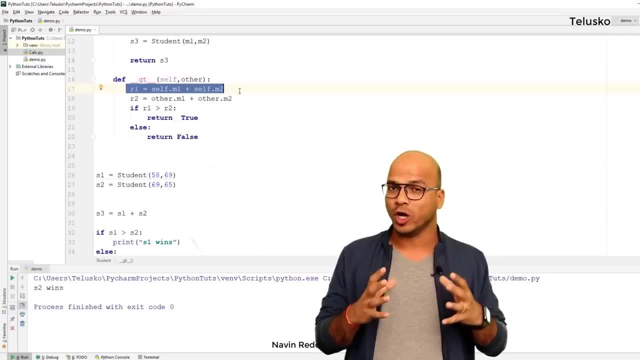 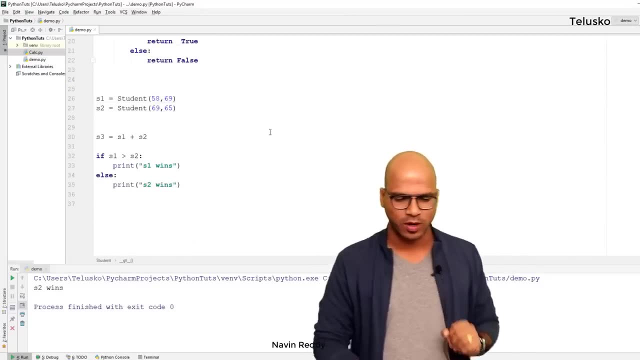 are adding those values and then we are comparing it. so if you want to perform any operation on the object, which i usually find, you have to define all these methods. okay, there's one more: what if you have a variable? let's say a is equal to nine, the moment you say, print a and you can see it will. 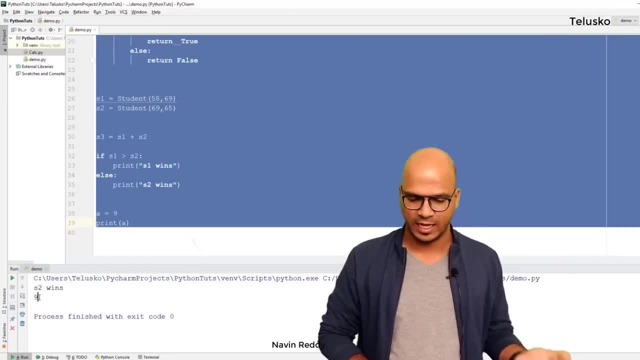 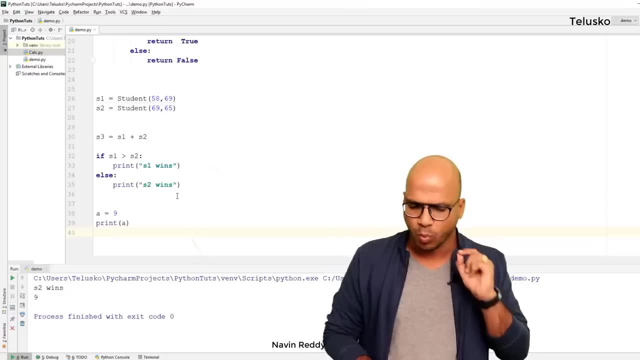 print the value of a. there's nothing wrong with that. you can see it is printing the value of a. now is it printing the address of it? that's not the case, right? it's not printing the address of a. it is printing the value of a. but what happens the moment you try to print s1? it? 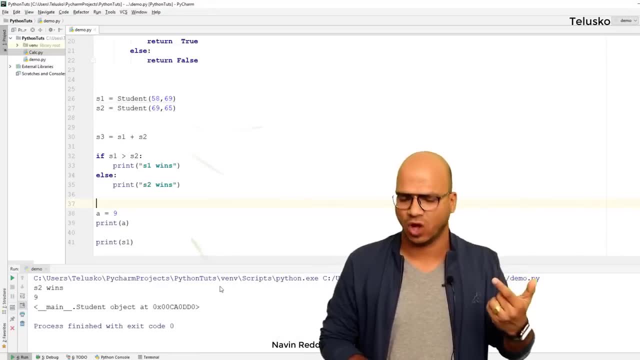 will not print the values of s1. it will try to print the address of s1. okay, so you can see that is it's a student object at the address. at this position. hey, we don't want address, right, we want values. what is happening? so when you try to print the object, it doesn't matter, is it integer or your? 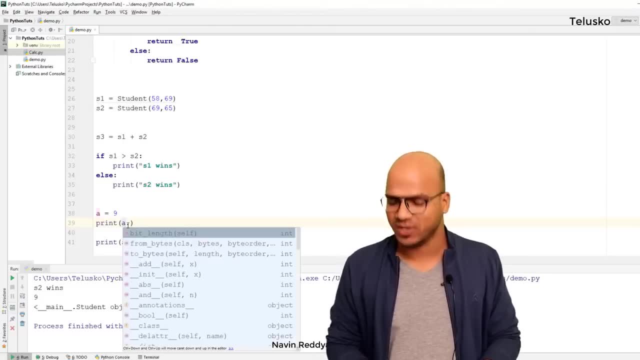 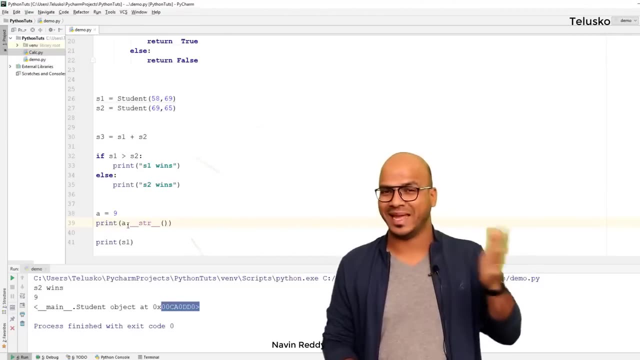 class behind the scene. it is calling a method called as str. it is happening behind the scene. okay, even if you don't call it, it is happening behind the scene. so moment you say print a, it will try to call a dot str, and that's why you're getting that output right. you're getting 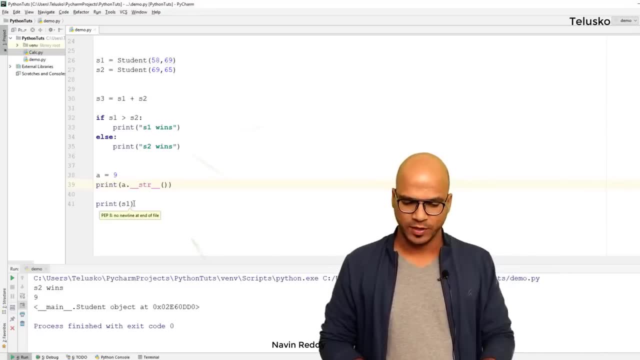 nine, because it is calling str. in the same way, the moment you say s1, even this is calling str. right. and now if you run this code, you can see it is still giving the same output. that means it is calling str. what is this str? so if i click on 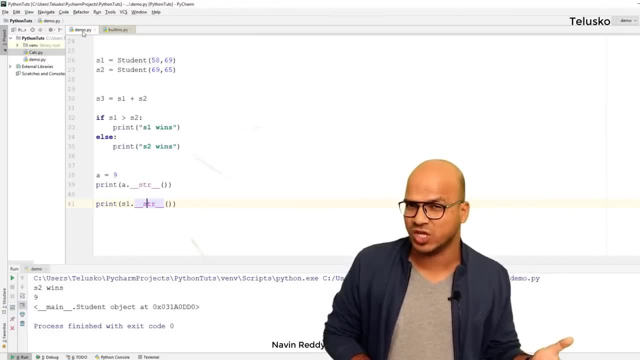 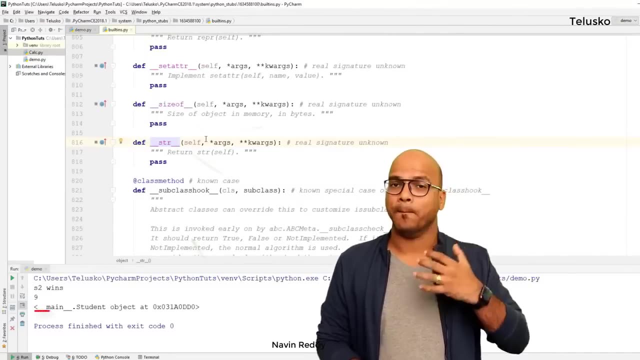 this you can see, it is in built in. so even if you don't define str, function or method in your own class, it is getting defined somewhere. and that definition what is printing? it is printing the module name, it is printing the name of the class and it is printing the object address. we don't 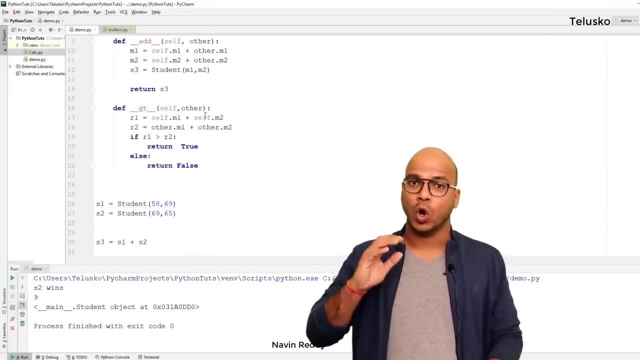 want that. we want values. right, that means we need to override this method. so what i will do is i will say def and the method name is str, so you have to define this by yourself. so we want to return the value of m1 and m2, right? 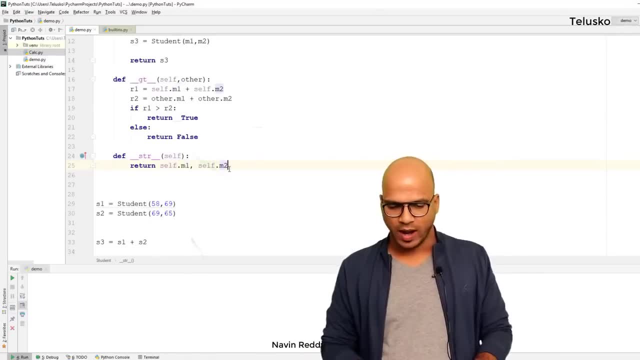 so you will say selfm1, comma, selfm2, and now if i run this code, it will return a tuple. of course, let's run this code and you got it. can you see that we got 58 and 69? so now, if you want to print, 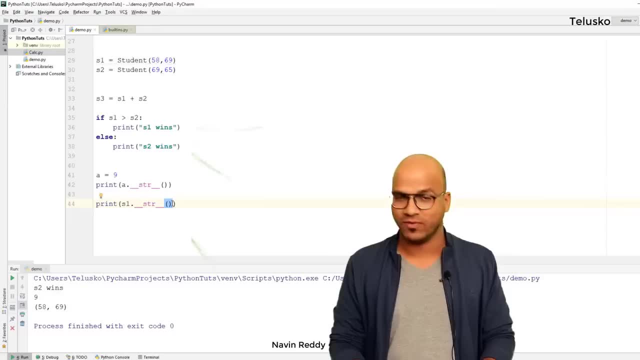 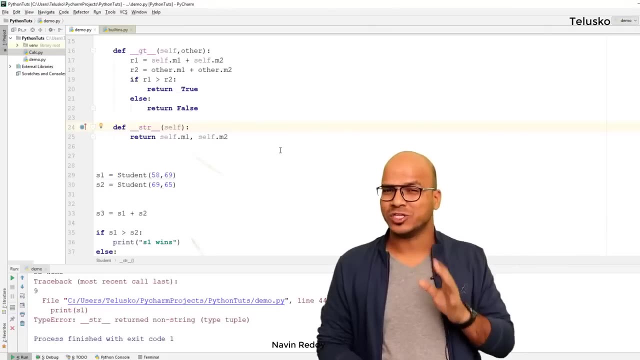 the object. it will not print the address. it will print the values, right, because we are overriding the value of m1 and m2. so if you remove str, if you run this code, you got then error. so it is returning a non-string value. we have to return a string value. how do we do that? because by default, 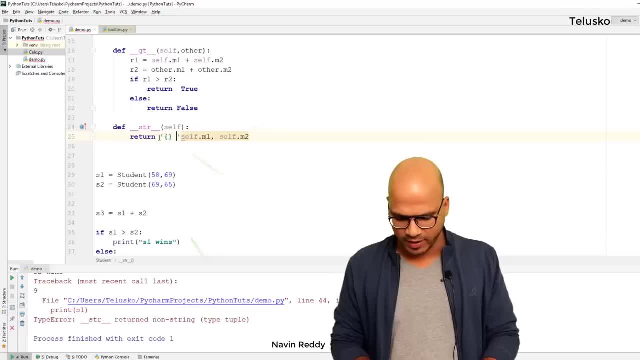 when you say print, you want to print a string, right. so what you will do is you will use a format here so you can say: curly brackets, curly brackets. you're printing two stuff- dot format, and inside this format you can pass this to value. so what will happen is those curly packets will be. 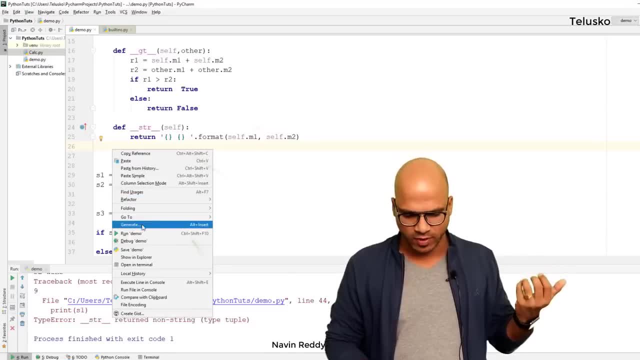 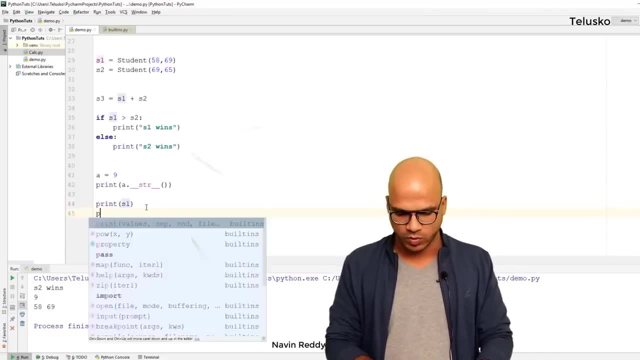 replaced by these values. so you are returning a string now and we have seen that before. right, so let's run this code. and it worked. you can see you got 58 and 69. Even if you say print S1, it does work. You can also print S2 if you want. 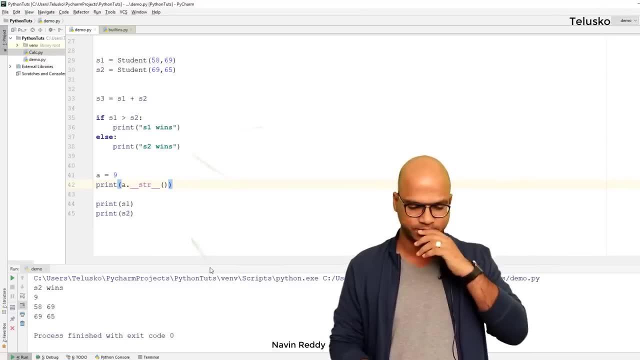 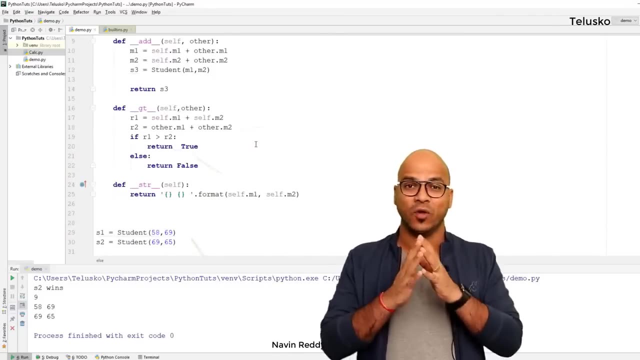 And let's run this code and you can see we got 69 and 65. So that's perfect. So this is how you work with operator overloading, okay, So point to remember is when you perform any operator like addition, subtraction, deletion. 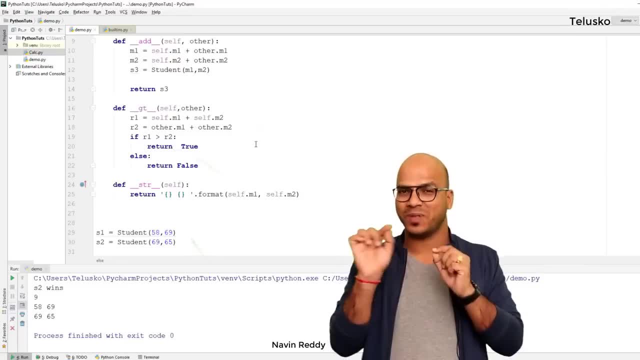 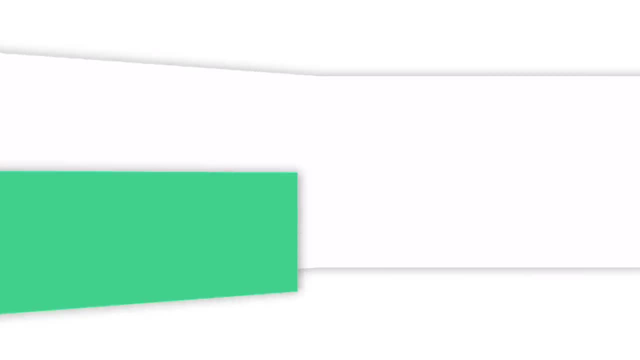 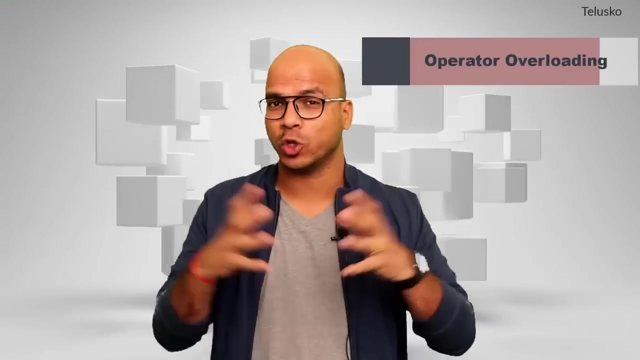 behind the scene we are calling methods okay. So for plus we use add method, for minus we use sub method and for star we use mult method. In fact, we have list of methods there. In the last video we have talked about operator overloading right. 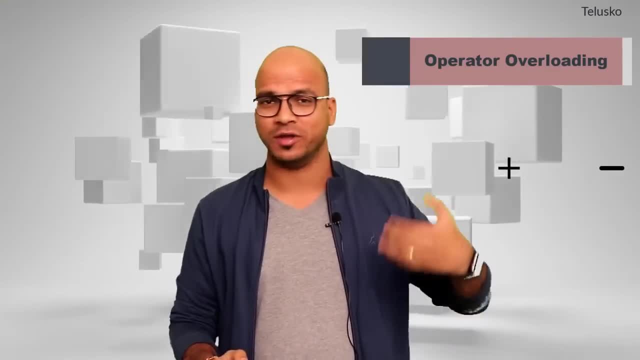 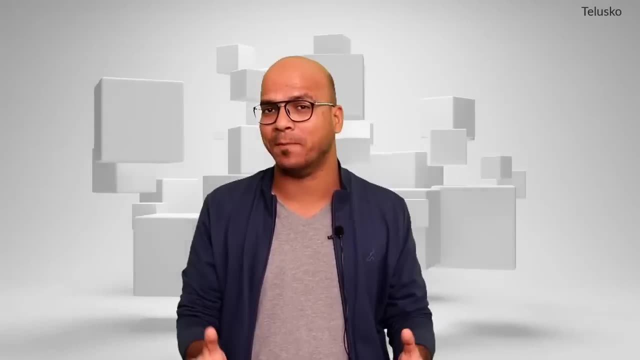 Which simply means you have an operator like plus, minus, or division or multiplication. So the operator will remain same, but the operands will change, right, The type of parameters we are passing, it will change. Example: when you say plus, we are calling the add method, right? 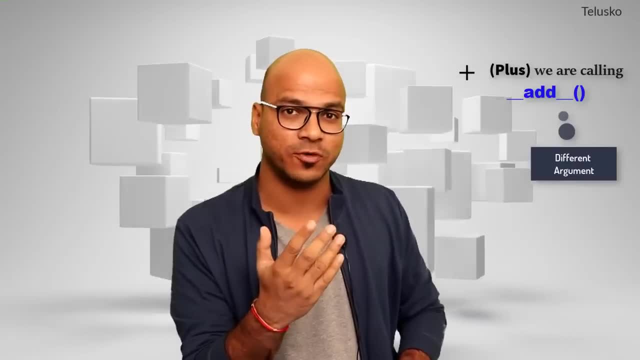 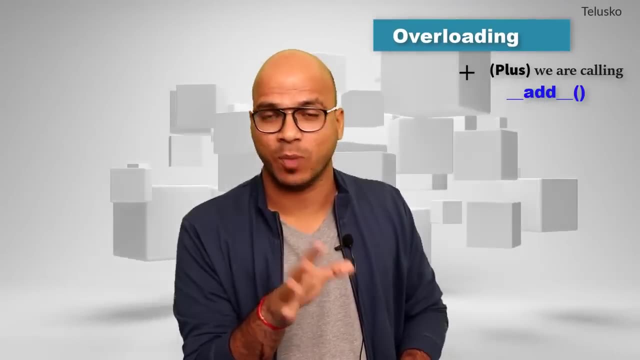 And add method takes different types of parameters or different types of arguments. So that is overloading. So it simply means You have the same method name but the arguments are different, or maybe the number of arguments or the type of arguments are different. 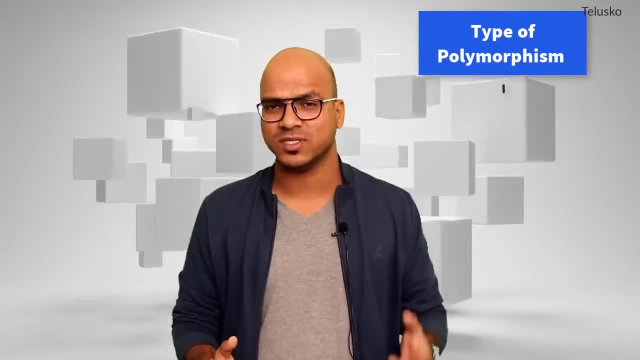 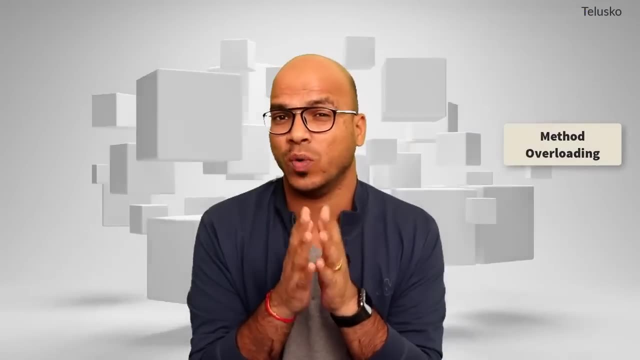 In the same way, we have two more types in polymorphism. One is method overloading and method overriding. So what it means, Let's start with the first one, which is method overloading. Now, languages like Java, C, sharp or any other oops language, they have this concept of method. 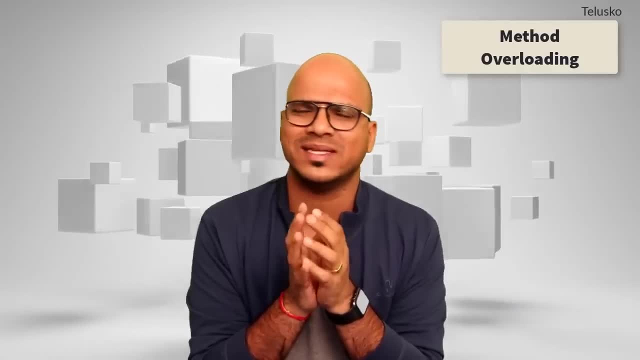 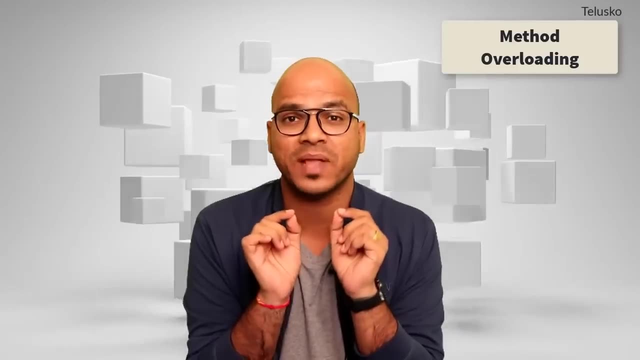 overloading, which is not there in Python, but what exactly it is. So it simply means We have a class and in that class, if we have, let's say, two methods with the same name but different parameters or arguments, which is called as method overloading. example, let's: 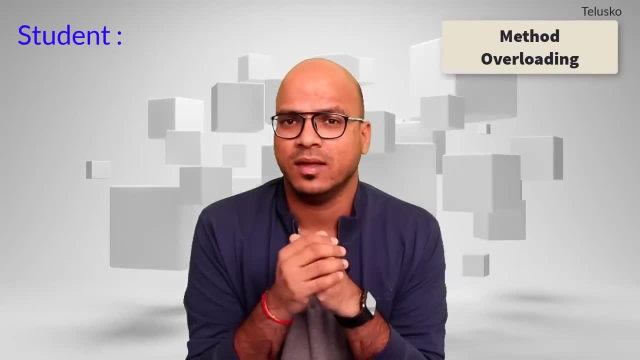 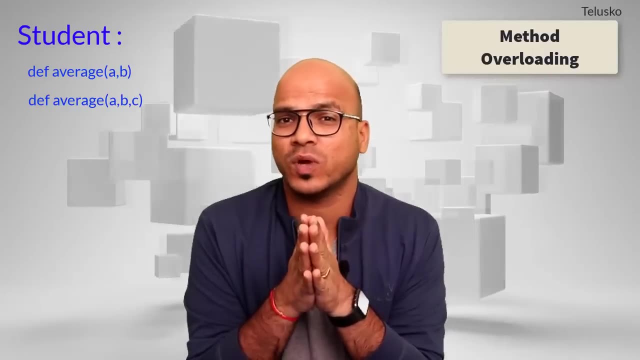 say, if you have student class and in student class, if you have two methods, let's say average. So we have two methods with the same name. average One takes two parameters, One takes three parameters. This is called as method overloading. 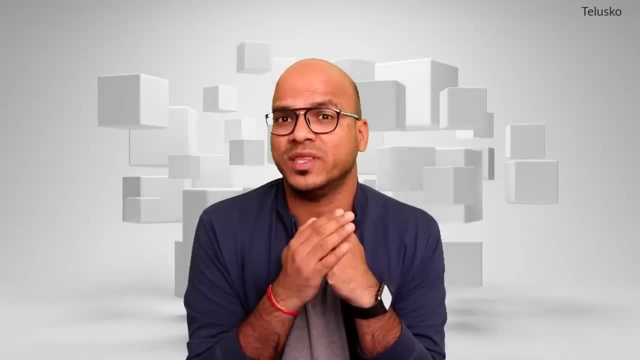 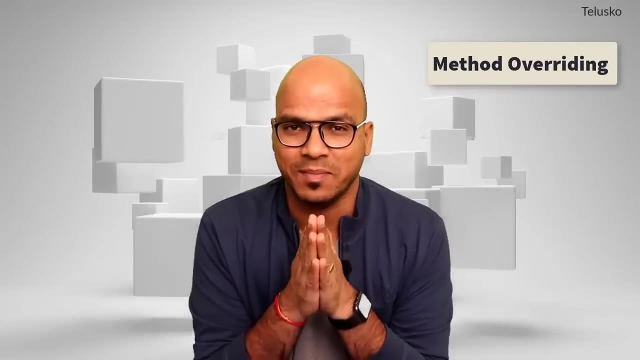 But in Python we don't have this concept, so we cannot create two methods with the same name. The next one is method overriding, which simply means you have two methods. Okay, Two methods with the same name and same number of parameters or arguments. 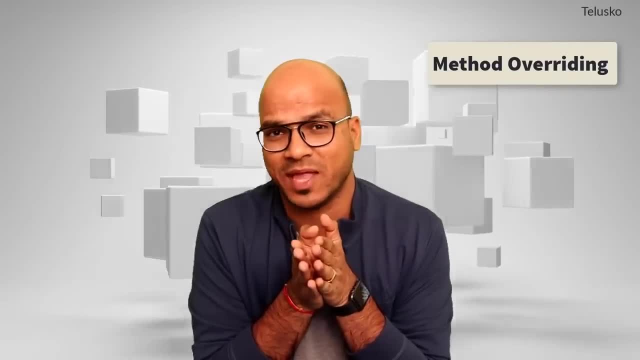 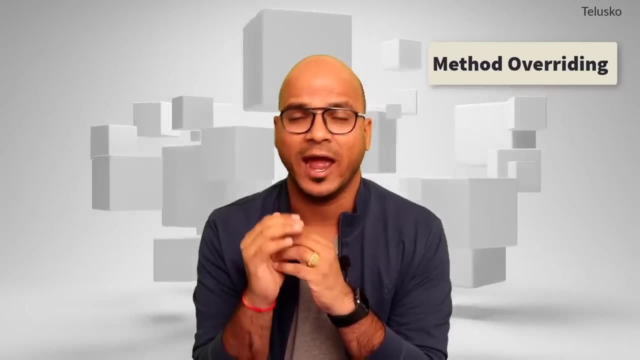 Okay, So that means, can we create two methods with the same name, in same parameter, in the same class? Of course not, Not in the same class. But let's say, if you have a concept of inheritance, we have class A and class B and both the class. 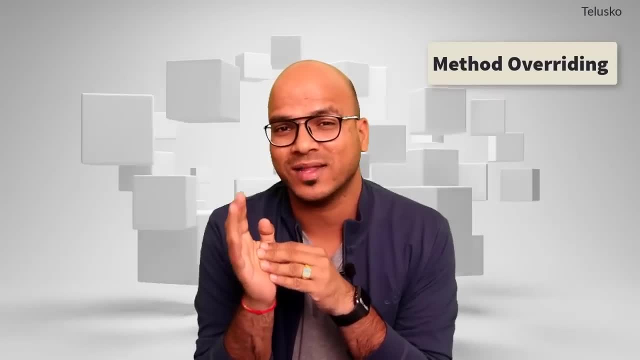 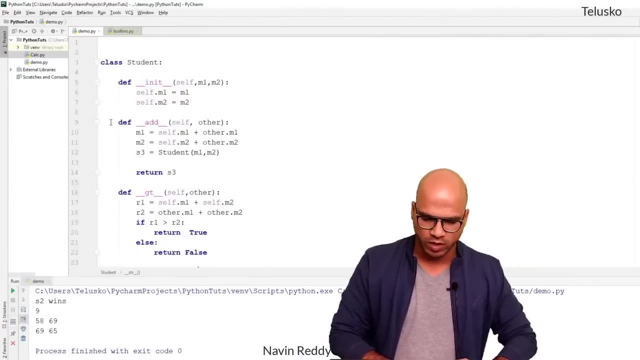 have the same method with the same name, same parameter. This is called as overriding. Again, we'll see the impact of that. Let's start with the method overloading first. So if you want to achieve method overloading, what I will do is I will just remove this. 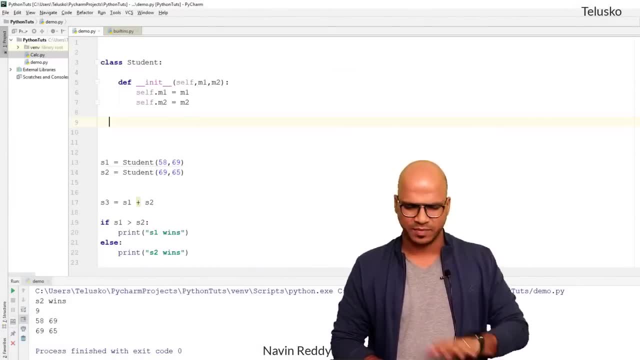 methods from here, Just to keep it simple, Right? So we got an init method and it is working perfectly. Let's remove all the extra stuff from here. We just want to create one object, not even two. I want to add two numbers. 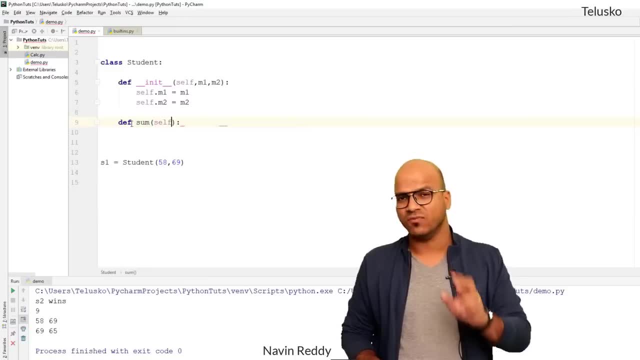 So I have to create a method. let's say sum, and this sum will take two arguments. We'll say A and B, So I want to add two values. That's it, Nothing complex. I want to add two numbers. Now, if you want to add two numbers, what I will do is I will say: S is equal to A plus. 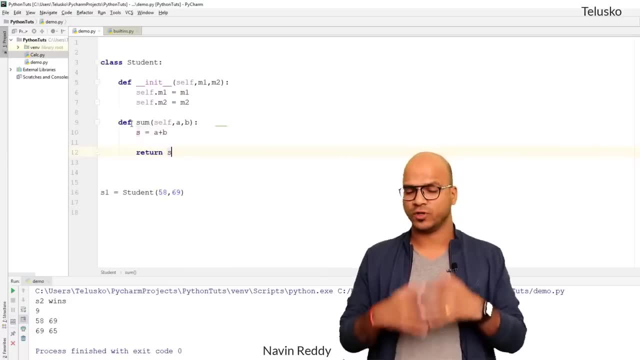 B, And at the end we'll return S. That's what we want to do here. We would just want to return the value of S. Okay, And if you want to work with that, you will say S one. In fact, you will print the value. 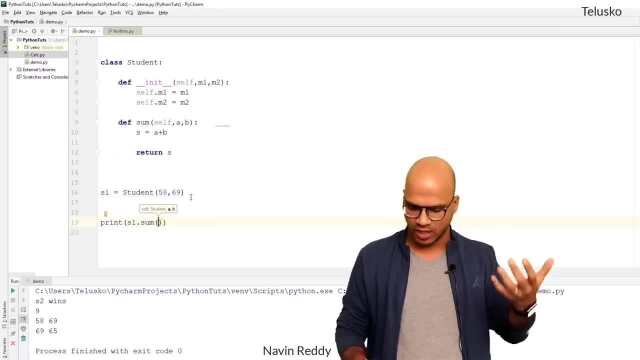 You will say S, one dot sum, And you want to add two numbers here. I will say five and nine and let's see if it is working. Let's run this code and it works. You can see we got 14.. So yes, we can create a method inside a class which takes two parameters, and we can pass. 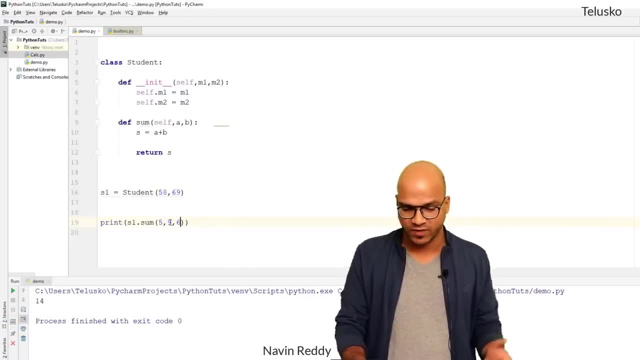 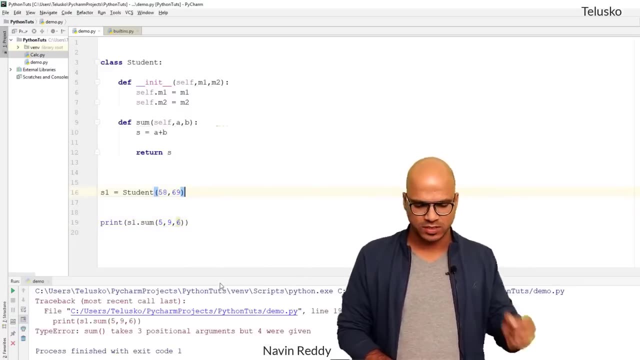 two parameters. It works. What if? if you want to pass three values, they want to pass five, nine and six. Now, this is not possible, right? The moment you run this code, You will get two parameters. You will get an error because you are passing three parameters or you're passing three arguments. 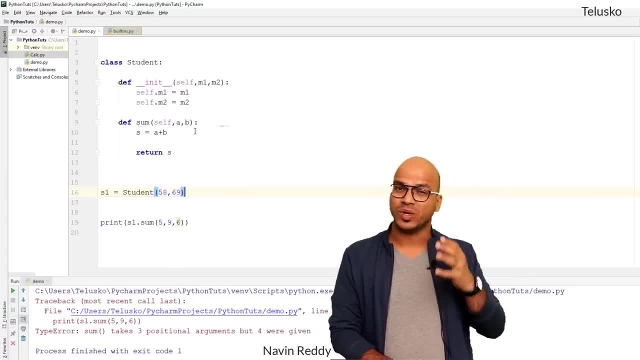 and you're accepting only two. So this will not work. That means you need to create another method, called a sum, which will take three arguments. That's what we do in other languages, But here will not do that. Here, what you can do is you can also use third variable. 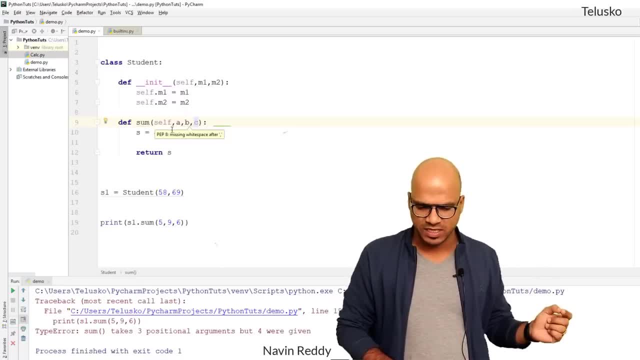 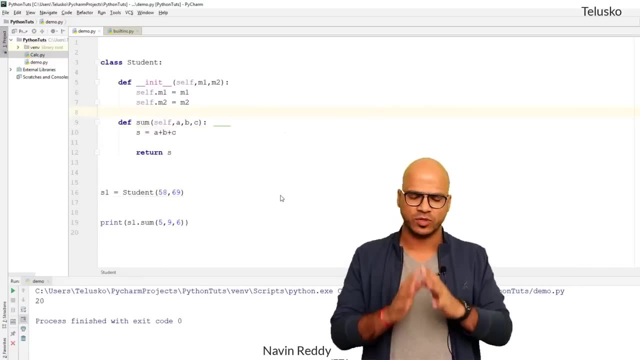 You will say C. you got A, B and C and you will simply say A plus B plus C, right, So this will work. So if I run this code and you can see, you got 20 and this is why you will get 20.. 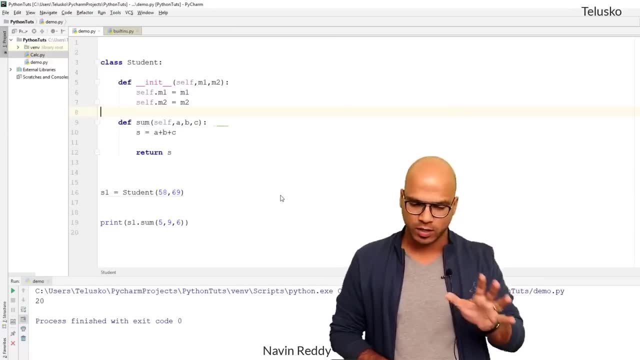 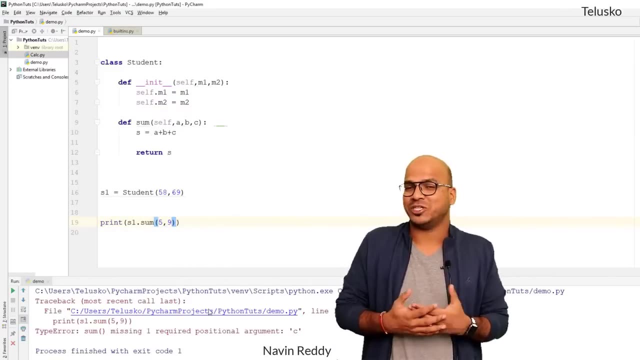 So we are passing three arguments and we are accepting three arguments. it will work. But what if I'm not passing third argument? I'm passing only two arguments And now the problem starts right, Because you are expected to pass the third argument as well. 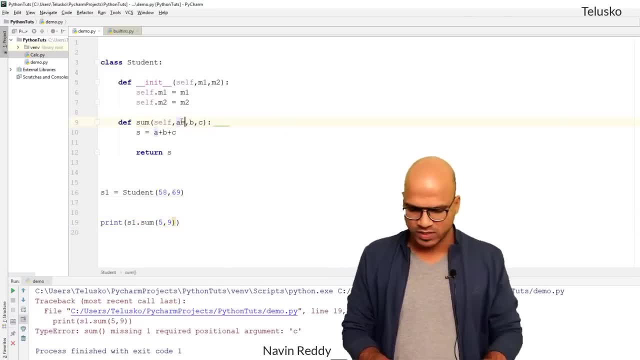 How do we solve this? To solve this thing, we can use a concept where you will say: A is equal to none. So this is one option. The other option: we can use the variable length arguments. If you remember, we have done that before the star and variable name. 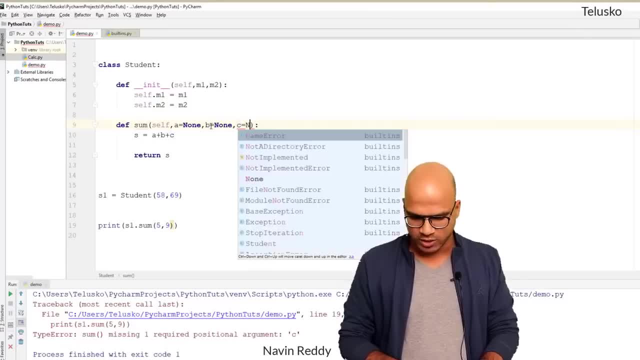 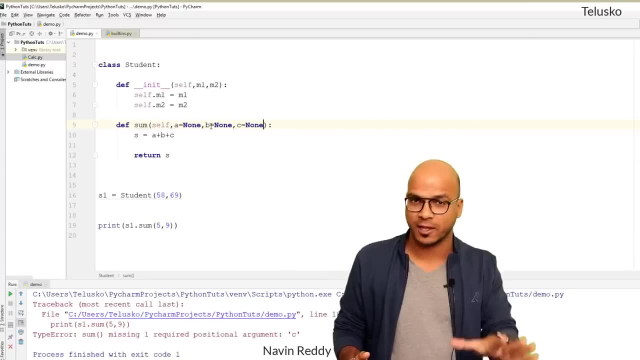 But this is another option. You can say: all the values are by default none, Which means, even if you don't pass the value, this is default arguments, right? So even if you don't pass the value, the default value will be none. 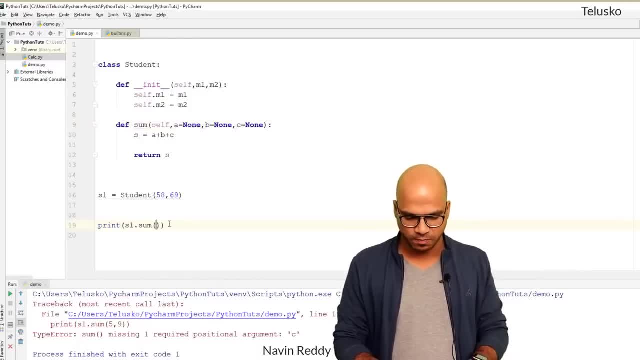 So that means, even if you don't pass any value- example, even if you don't pass five and nine, it will work. All the values will become none. I want to pass some values. I will say five comma nine. I'm passing two values, right. 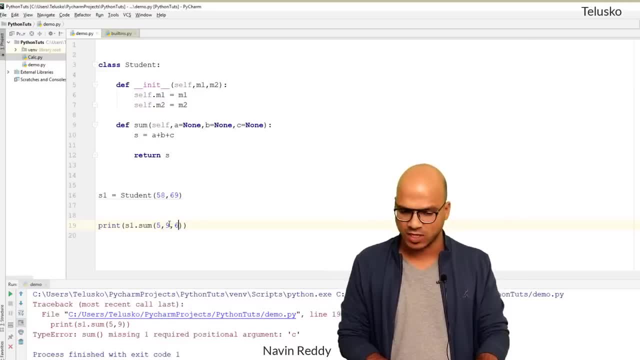 Let's start with third one. Let's say I want to pass three values: five comma nine, comma six. All these values will be assigned to A, B and C respectively. right? So if I will go to A, nine will go to C. 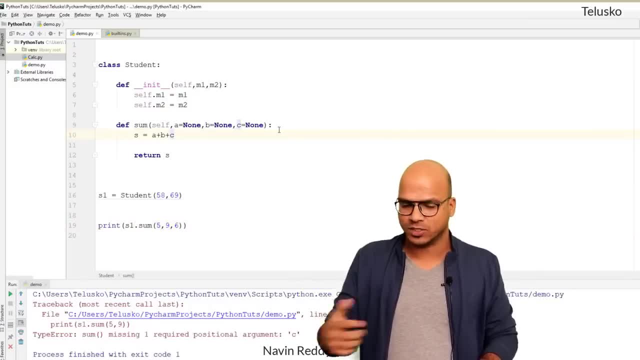 Nine will go to B and six will go to C, So these values will be replaced by none. So none will be replaced by these values, right? So now, once I know this, so we can simply add it. But what if you're passing two? 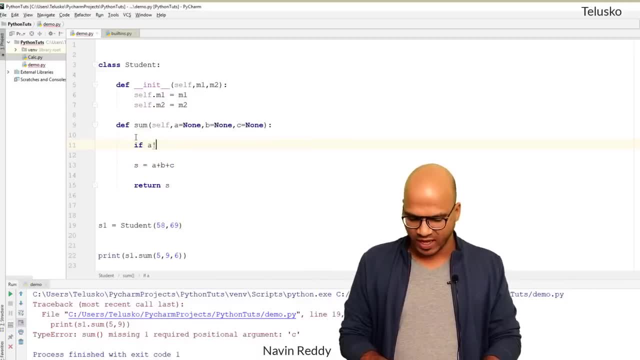 So in this case you will check. So before adding, you will check. You will check if A is not equal to none, B is not equal to none and C is not equal to none. So if none of them are none, that simply means you're passing three arguments, right. 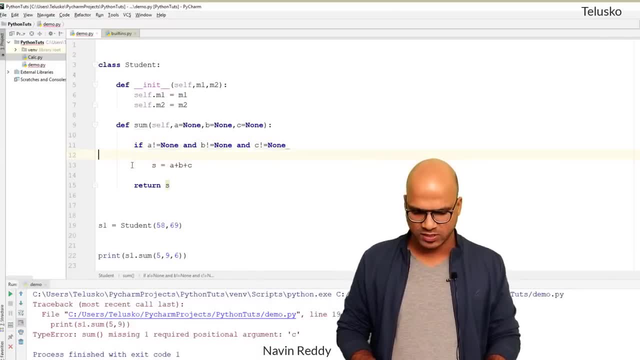 And if you're passing three arguments, this is the calculation we have to go for. You will say S is equal to A plus B plus C, And you want to declare S outside so that you can use it from anywhere. So you will say S is by default zero and you've got this. 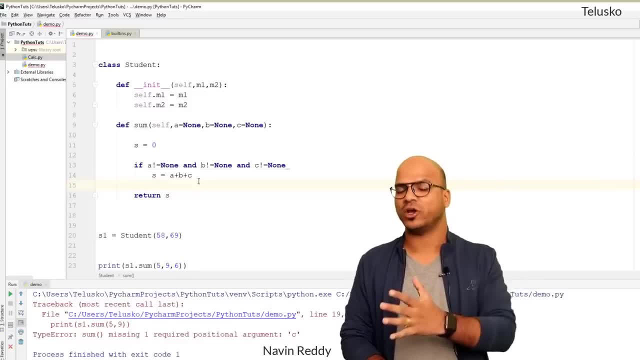 Otherwise, if let's say, if I'm passing two arguments, I'm not passing the third argument, in that case it will go to LF and inside LF I will check. I forgot a colon here, So inside LF I will check if A is not equal to none. 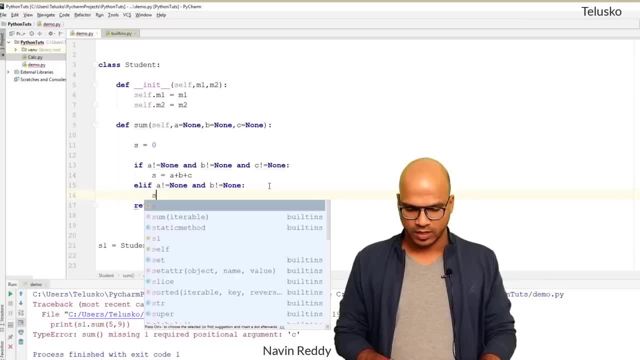 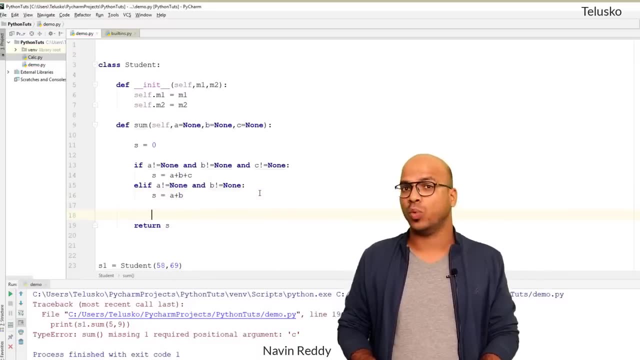 So I'm concerned about A and B If they are not none, in that case I will say: S is equal to A plus B, because we're not concerned about C. right, And we can go for one more condition. What if you pass only one parameter or one argument? 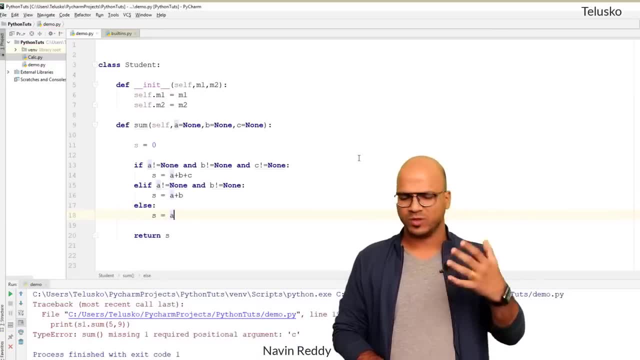 In that case you will say else and you will say S equal to A. So when you say only one parameter, let's say: if I'm not passing nine and six, I'm passing only five, So it will return five, right. 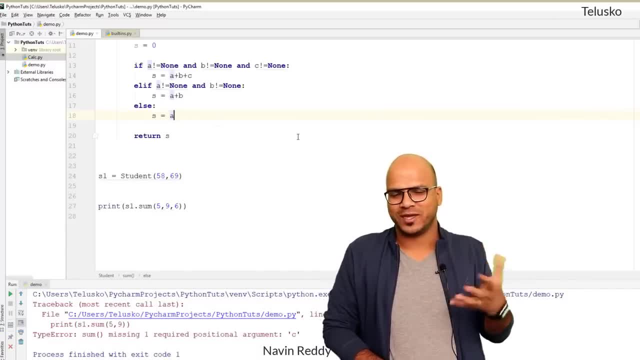 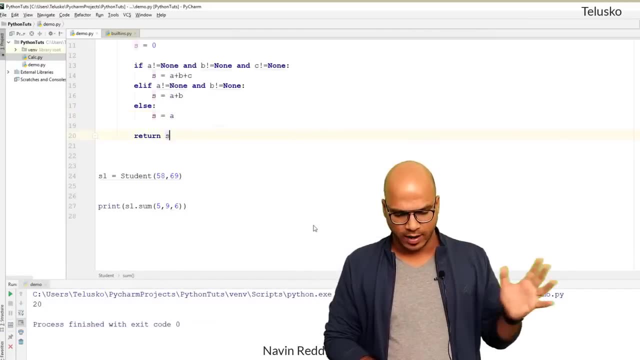 That's what we want, So we can do that. Else part is not required here, but just to make it more effective. we can pass one argument. we can pass two arguments. we can pass three arguments. That's perfect. Let's run this code. 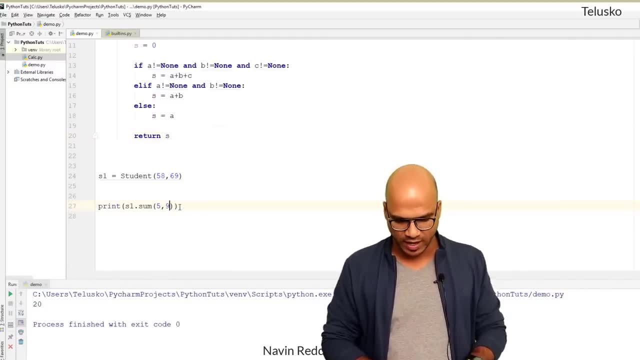 And it worked. You can see we got 20.. Now, if I pass only five and nine, even this will work, Because if you pass only five and nine, it will return five and nine. Okay, If you pass only five and nine, C will get none and it will execute LF and you can. 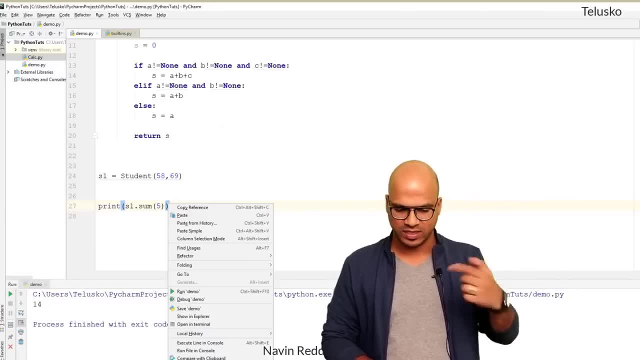 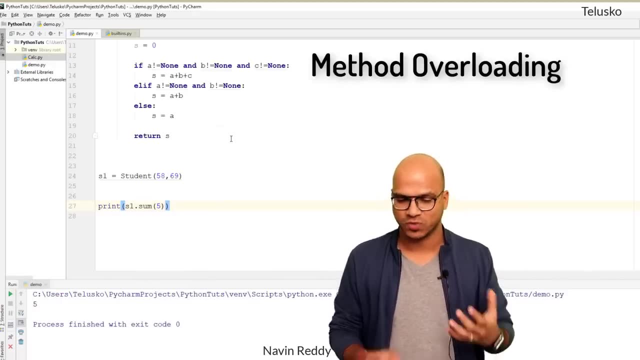 see, we got 14.. Now, if you pass only one value, let's say five in this case, if you run this code, you got five. right, That's how it works. So this is your method: overloading. So we are overloading methods, but then we are not doing directly because it doesn't. 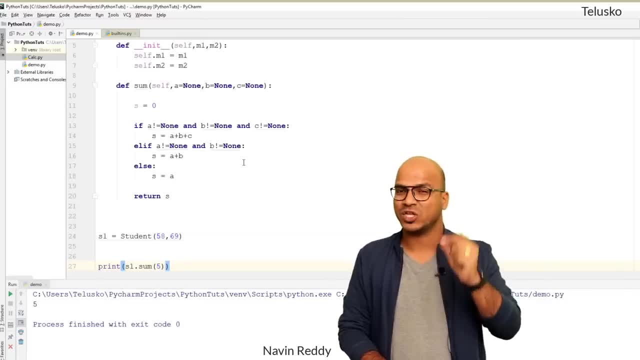 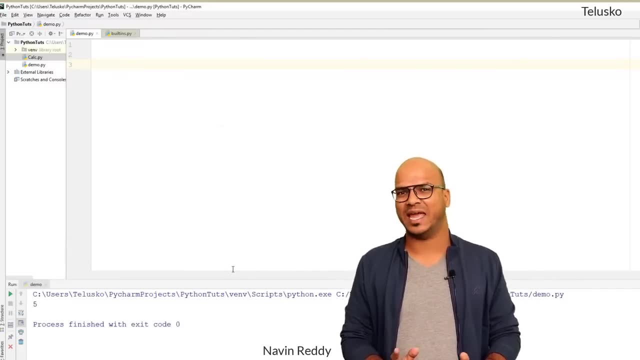 support in Python, so we are doing some trick. The next one is method overriding, So let's go with that. Let me just remove this code And let's once again take a simple example, And this time we'll go for A and B. 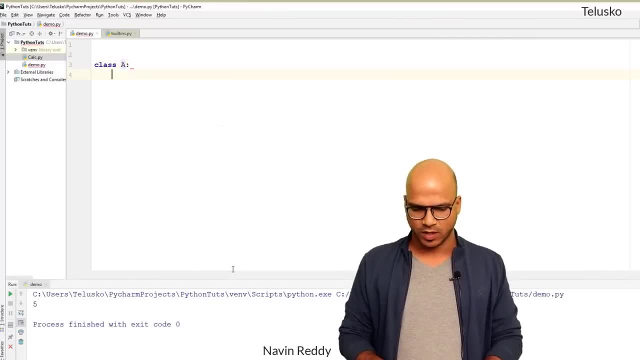 I love these classes. So what I'll do is, let's say we have a class A, okay, And in this class A we have a function. I will say function name is, or the method name is, show, And in this method I will simply print in a show. 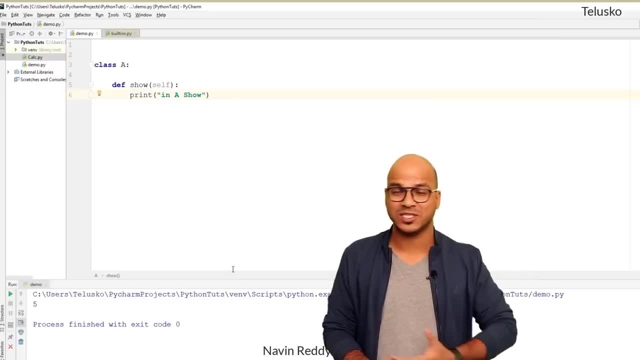 Now, first of all, before going ahead, this concept is method overriding. This is very famous in software industry, you know. So in future videos we'll also talk about this thing. when we talk about interfaces and abstract classes, This concept is used very heavily. okay, 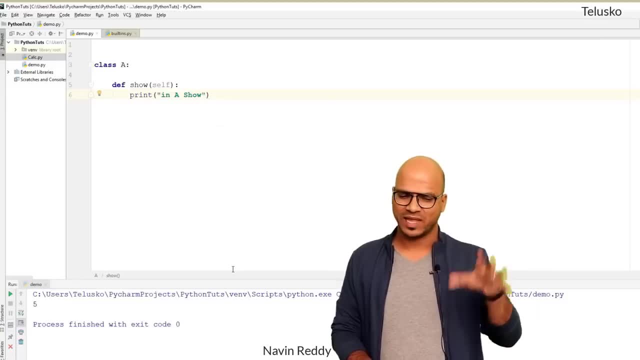 So make sure that you understand this concept properly, Maybe with simple example like A and B, but understanding the concept is important here. We can go with complex example as well. Concept is important. So let's say we got class A, which has a method which is show and we are printing in a show. 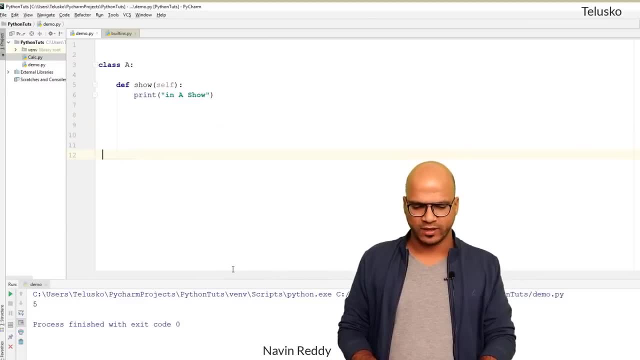 That's it. Nothing fancy Now. if I create an object of A here, so if I go back and if I say A1 is equal to A, so we are creating object of A right And with the help of this we can call show. 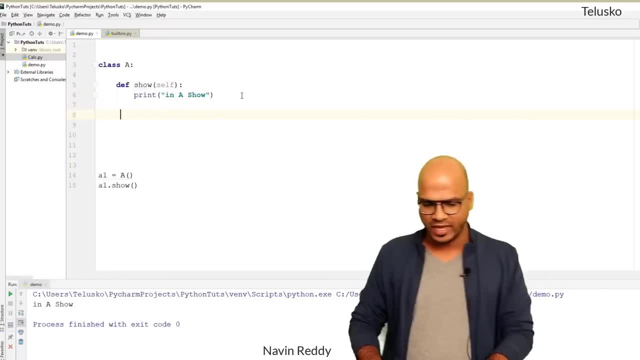 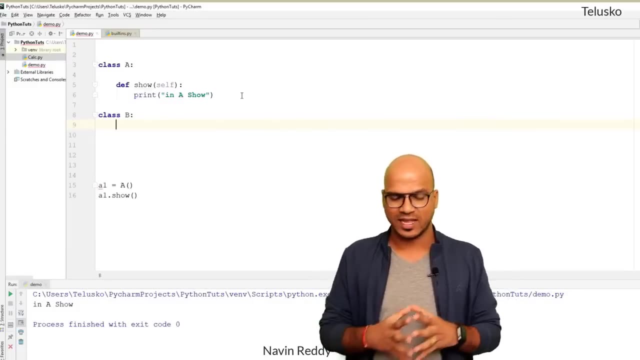 If you know this code, you can see we got in a show That perfectly worked. Now, what if you create another class, Let's say class B? okay, Okay, And now imagine this: class A is a parent and class B is a child. 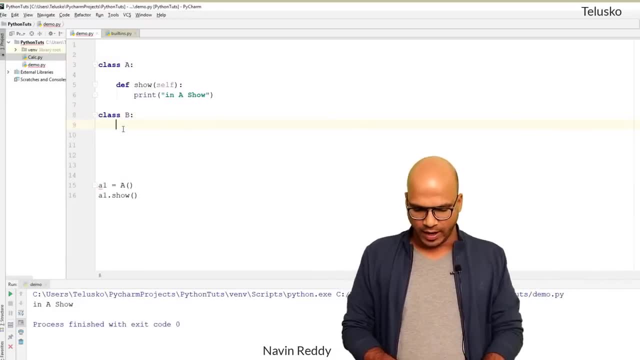 Example: let's say this is my dad and this is me, So we have B here and time mean I'm not writing anything. here. We say: pass, I just want to keep it empty. Okay, So we are keeping it empty. Let me create object of B, not A, but let me get object of B and let's run this code. 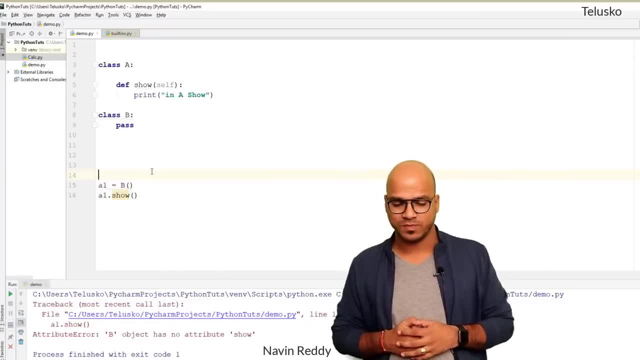 and you can see we got an error. It says B object has no attribute as show. Of course, right In B we don't have anything. At this point you will use a concept of inheritance and you will say, hey, B show. 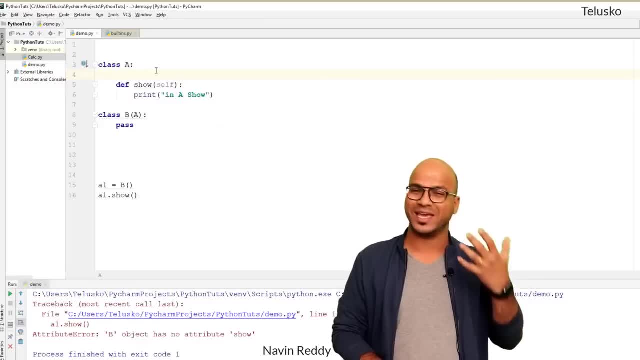 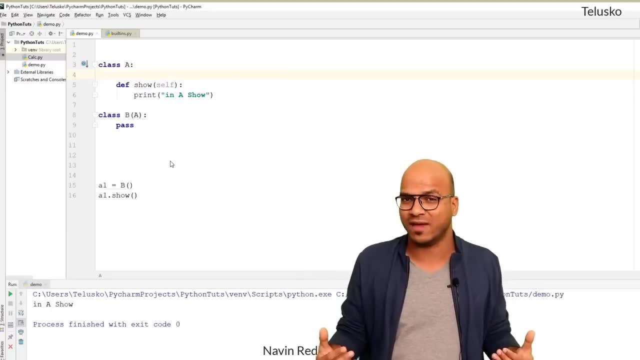 Inherits A. So when you say B inherits A, it means you will get all the features of A to B. And let's run this code and you can see we got in a show because of course in B we don't have show. 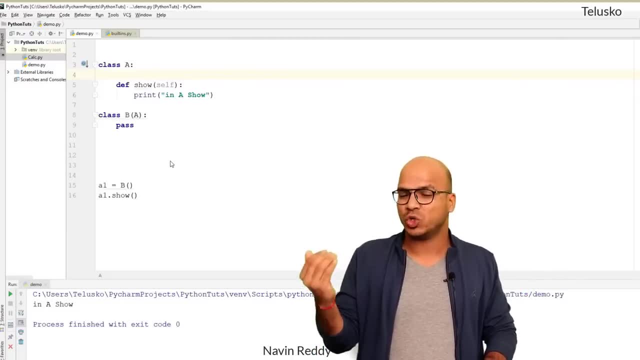 The moment you run this code, it will first search for the method show inside B. Now, since we don't have that, it will go to A to search it, and that's how it works. So, before going ahead, let me tell you one story, a small story. 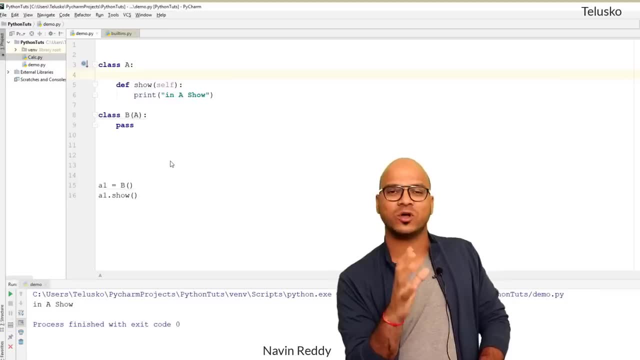 I've used this story in multiple examples when I was teaching Java as well. So the concept is: when I was in my 11th standard, when I've just joined my college, I was not having any phone. okay, So a lot of people they used to ask me which phone you have. 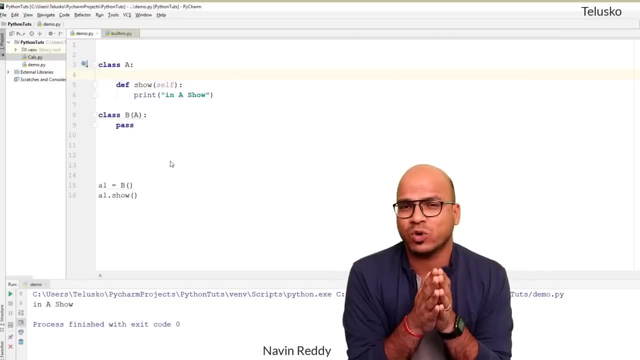 So I used to say: I don't have any phone, okay, Because I was not having a phone. But then this question got repeated multiple times. then I realized, okay, I have to say something Now. at that point my father was having a phone, which is Nokia 1100. 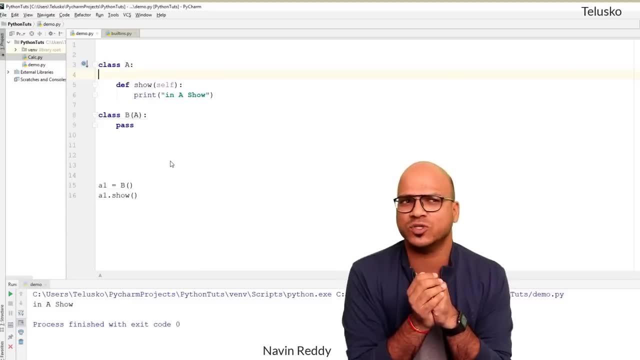 I was not having any phone. So whenever someone used to ask me which phone you have, I used to say: I got Nokia 1100.. I don't have a phone, right, But my father has a phone, So father's phone is my phone. 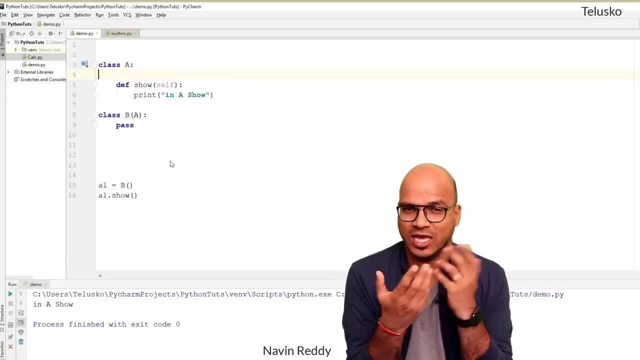 That's how I think it works right. So since B, I am B, Father is A, So B inheads A, So I got all the features. In this case, show is in A, right In B. we don't have show. 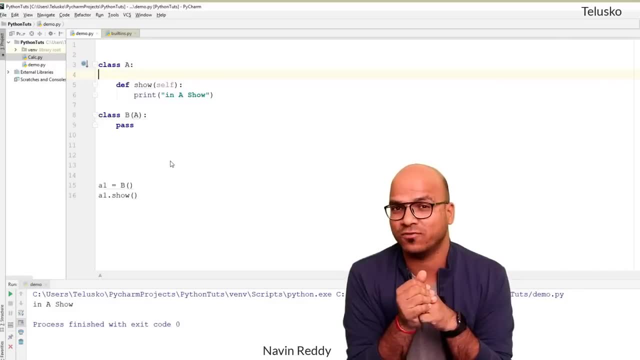 After some time, you know, after a few months- I got a new phone and that is Motorola phone. So my father has a Nokia phone and I got Motorola phone. Now, if you ask me which phone I have, of course I would say Motorola, right. 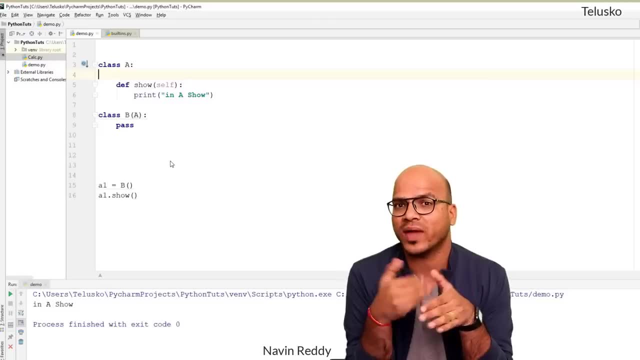 I would not say Nokia, right, Because my phone overwrites my father's phone. That's what was happening here. The moment you create a show method inside B as well, And if you try to print in B show, because when we were not having show inside B, it